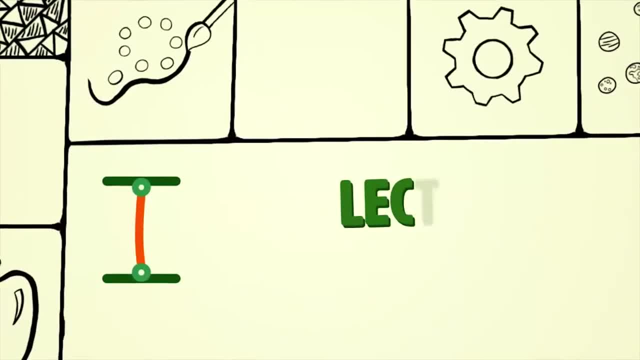 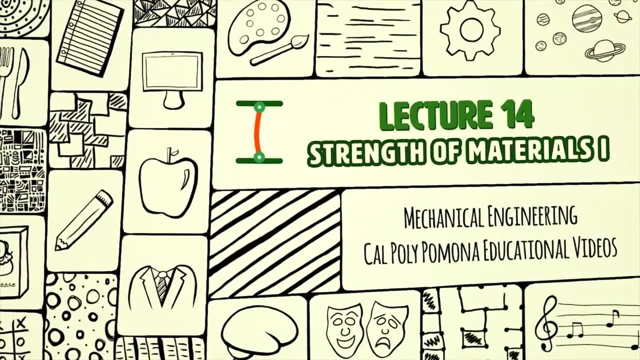 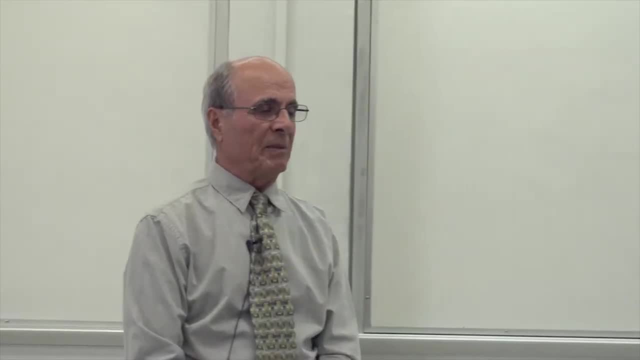 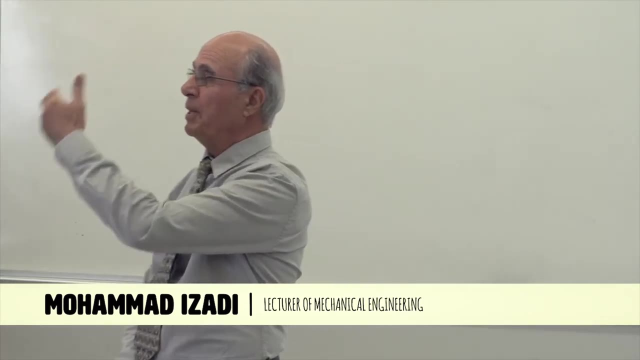 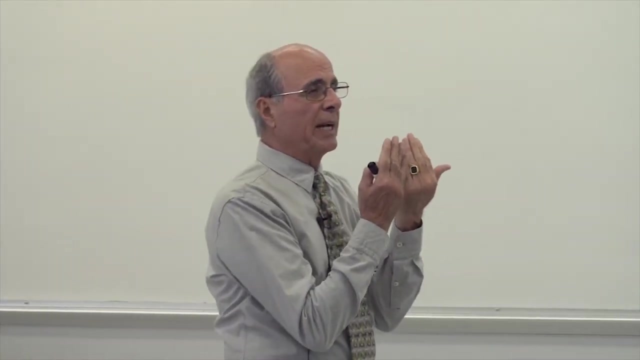 It was about composite beams. That means that there are two types of material. is there? It happens a lot. Let's say that you are trying to you have a building there or a structure there And to do that you can put two beams next to each other. That way you're only increasing. 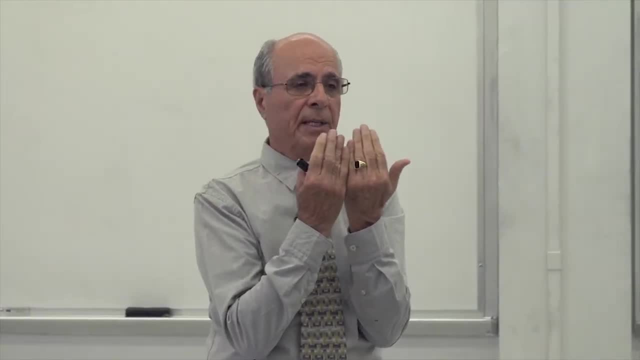 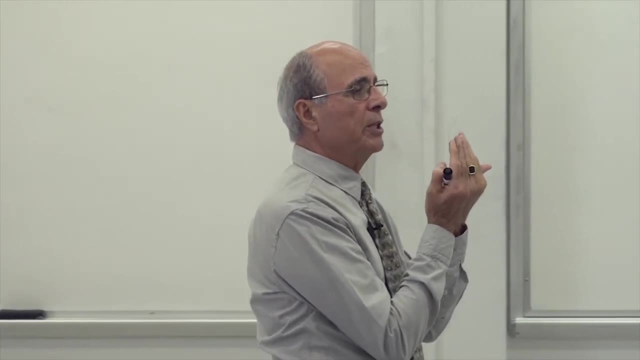 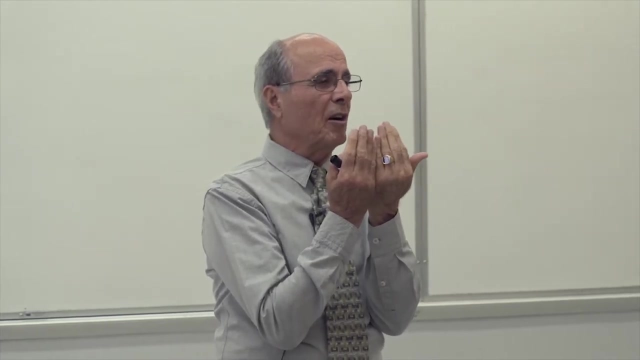 I twice. Everybody agrees on that. Why If I put one beam here has an I of so much and I put another beam next to it, like that the I become twice. only Correct or not? Why? Because I is usually is 112 of base time, height cubic, So when the base increases. so who? 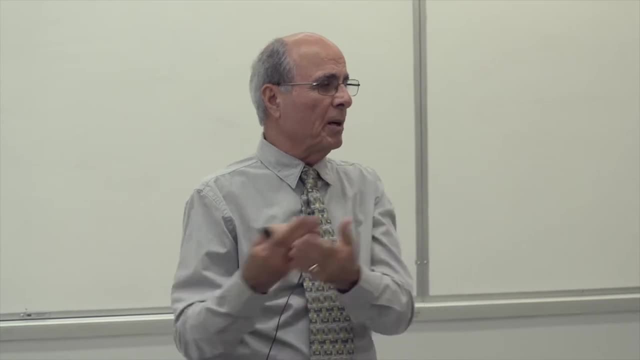 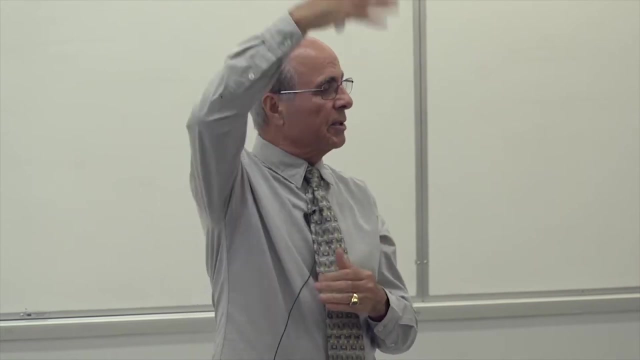 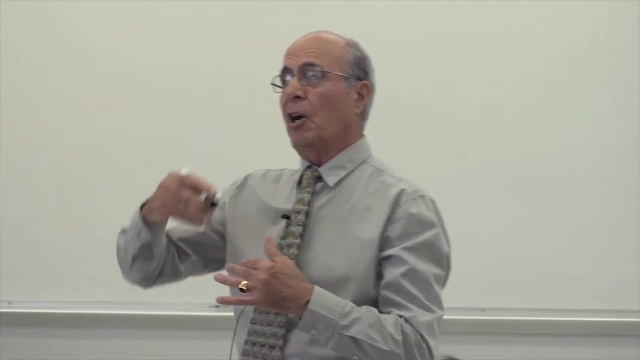 cares, It still is twice. Two B become twice. Is that correct? However, if you put the two beam on top of each other, then what happen? The I become much larger. You have to understand that from this static. So you put the two beam on top of each other, then the I become. 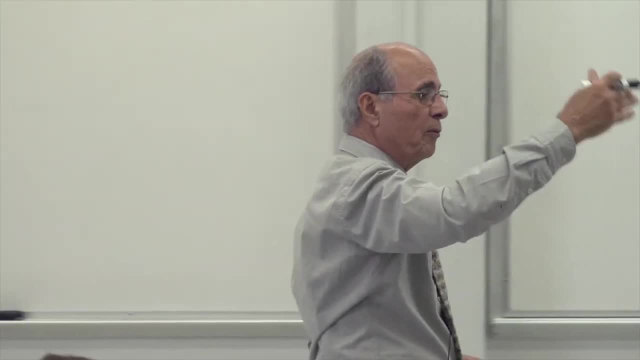 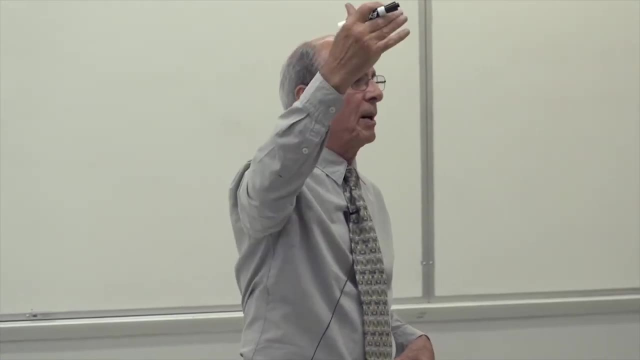 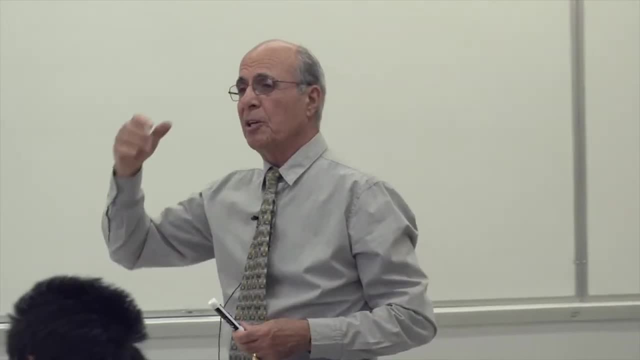 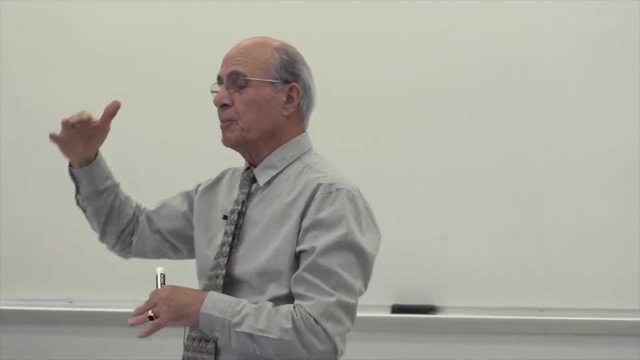 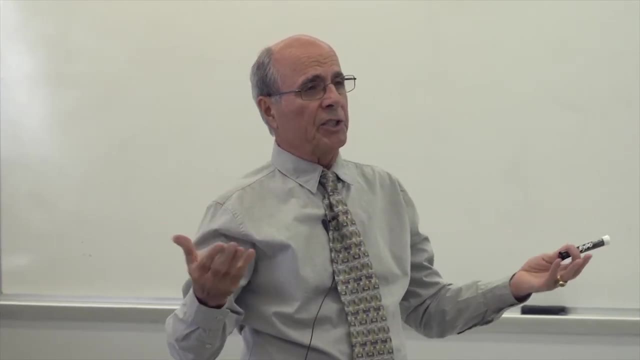 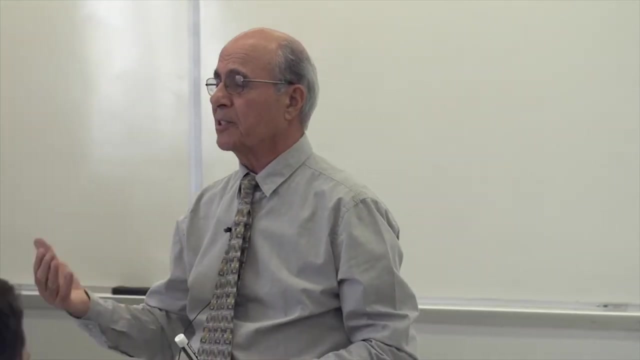 because you based first of all. you don't have sometimes the space to do that, Sometimes because of cost. so it's just not right decision because your beam strength suddenly become 10 times more. Is that correct? And you need only 50% more or 100%? In that case, you sometimes 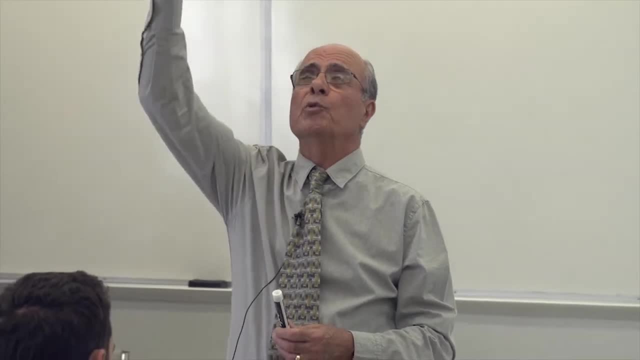 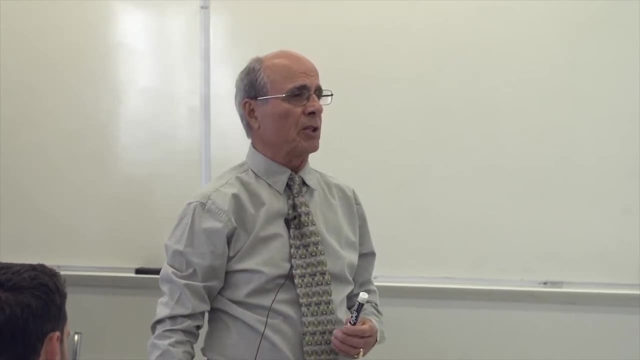 you don't even have to ruin the ceiling, but you go on the roof, You cover that one and just a piece of metal on top. for example, let's assume it is a wood structure- All you have to do put a metal on top. Is that correct or not? Therefore, it 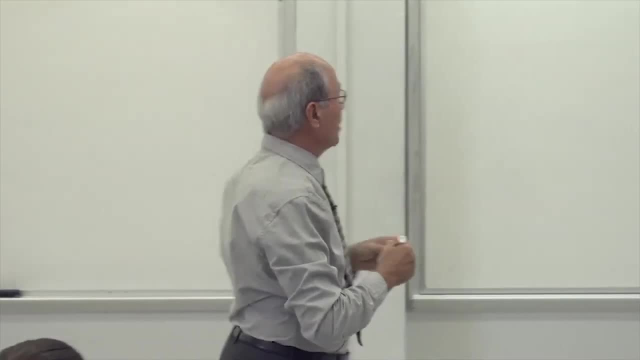 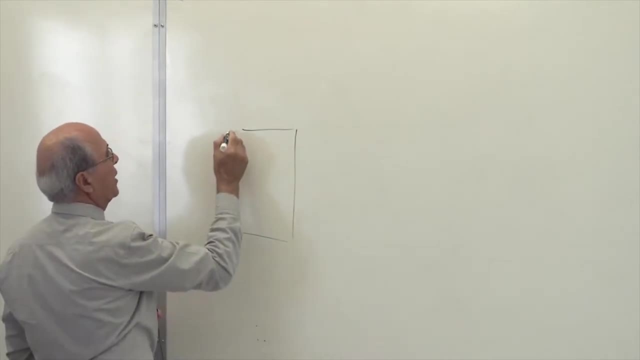 become a composite beam. It is part of a beam, is so this is what I'm saying- that the part of a beam. if you do it this way, first of all this is the wood beam And then you only put a metal on top The length we are not talking about. 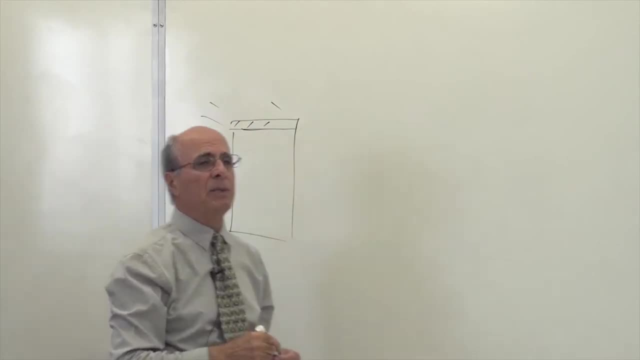 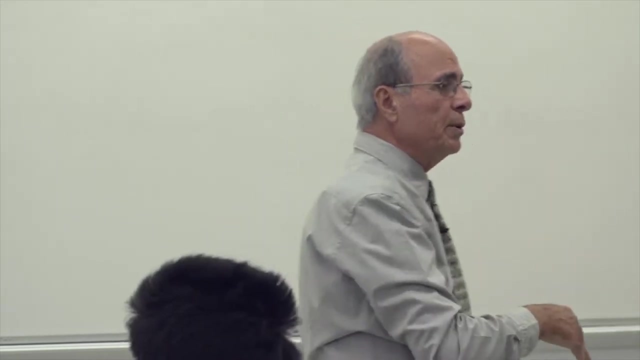 length of the beam Discover, so it become a composite beam, And I discussed that last time. How do we treat that? How we treat that? We have to change the wood into steel or steel into wood. Both options are available. Now let's do the 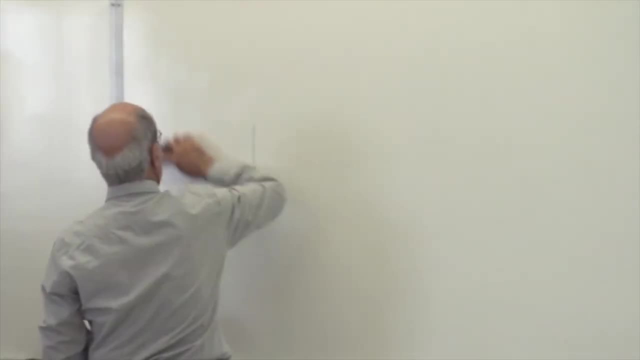 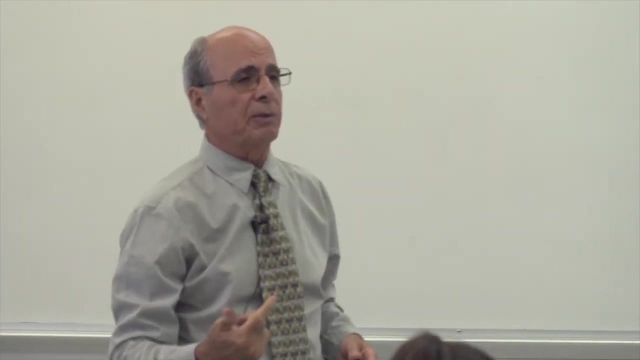 example, because I did not finish it. So the discussion. remember that at the beginning you have to change it. At the end again, you have to change it as well when you calculate the stresses. Is that understood? So for that reason, in 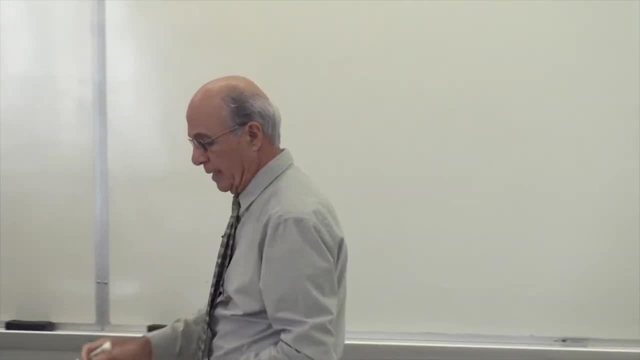 your handout. there is a problem in your handout. We are going to do that In your handout. I believe it is a problem. It is page three of your handout. There are a few more copies here in case you. 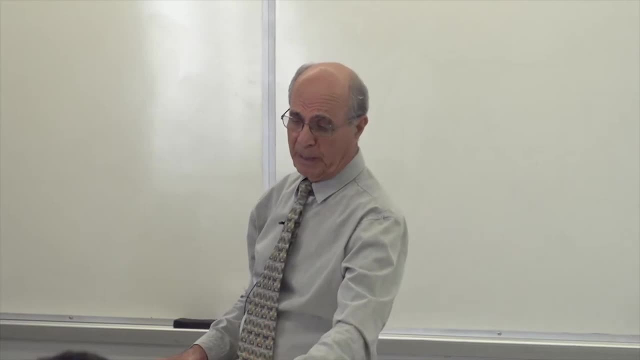 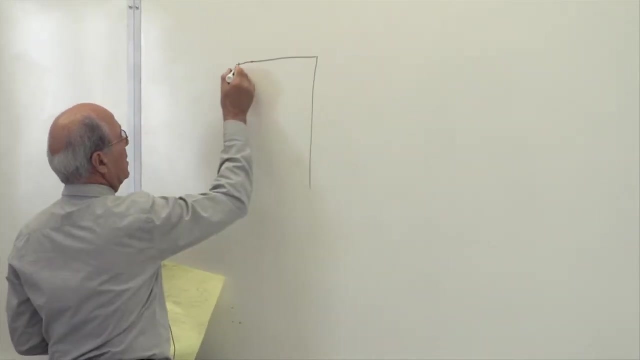 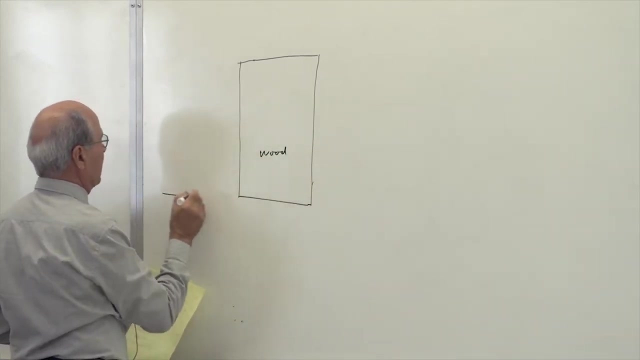 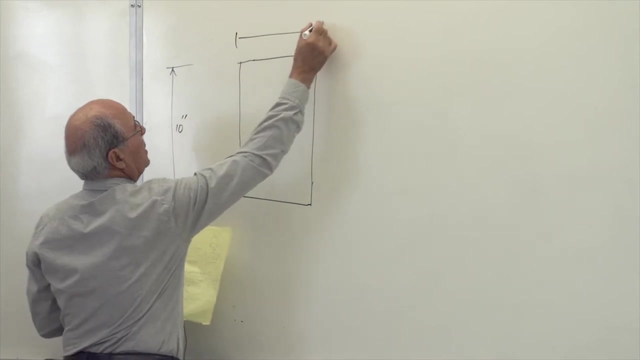 need it. So on the page of three, page three of your handout- there is a problem there- for this purpose. So it is a rectangular shape wood beam. The height of the beam is given equal to, I believe, 10 inches And the width of the beam is given 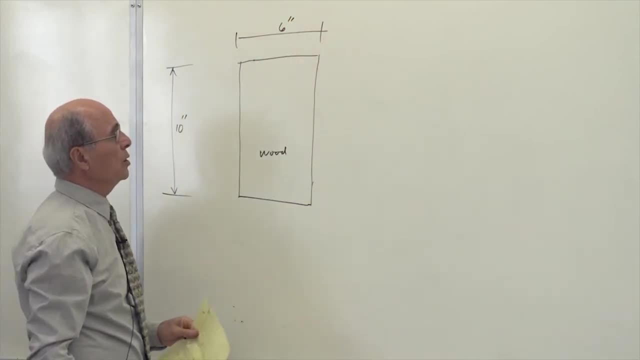 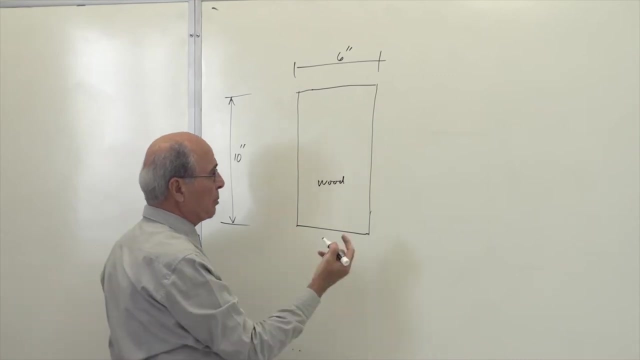 6 inches. So it's a 6 inch by 10 inch wood. This is just for practice purposes. What's the purpose of adding a steel here? It's not what I was talking about For this particular beam. they have added a little piece of metal here, a little piece of. 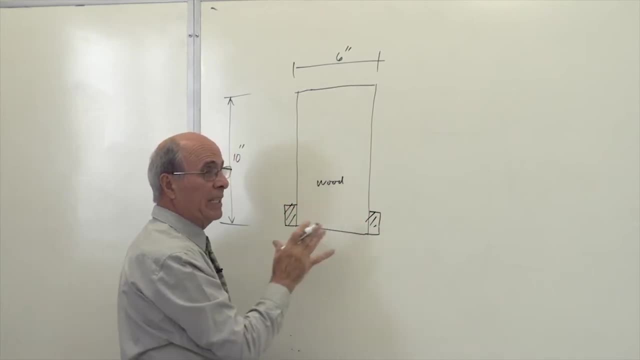 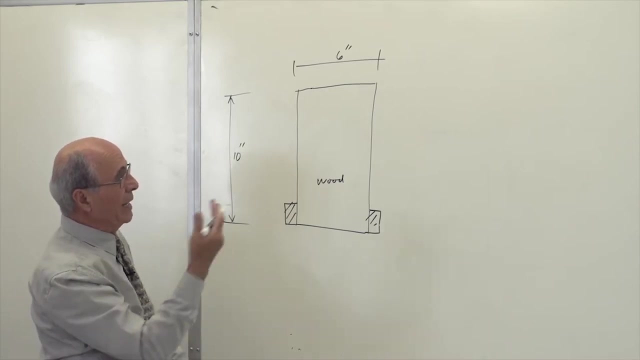 metal there or a strip of the metal. This is again is the cross section. The length goes whatever. We don't care. at this time We are not concerned about the length of the beam, So the beam goes like that. Everybody see what I'm talking. 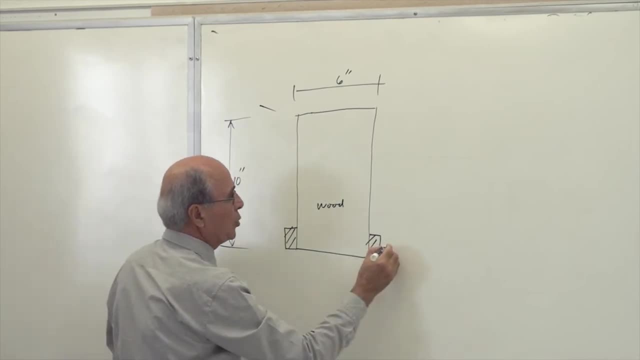 about. So here it is. And then we have added 2 inch height and 3 eighths of an inch thickness strip here. So if the beam looks something like that, so all you have to do put a little strip here and a little strip there. Everybody understand, And you. 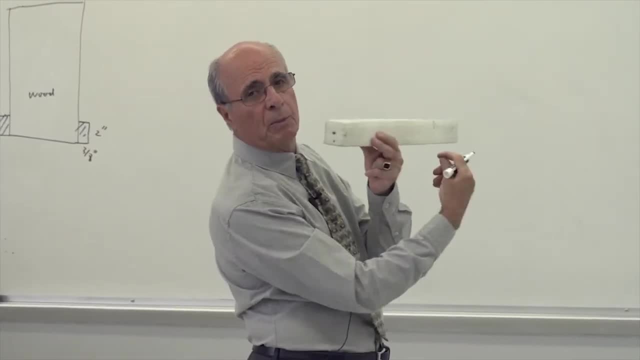 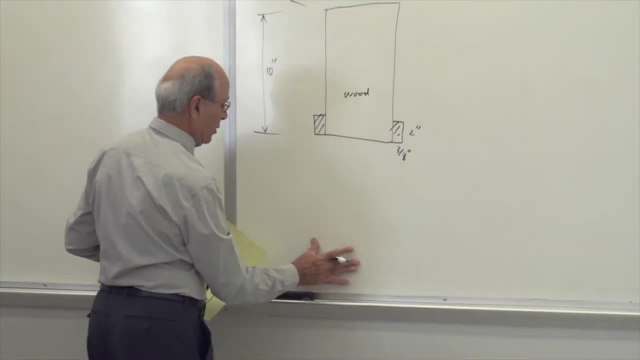 are showing it the cross section. So the strip goes like that on both sides, Correct, On the bottom of the beam. Now the data that we usually will give you is the following: I have to say this is wood and this part is wood And this part is. 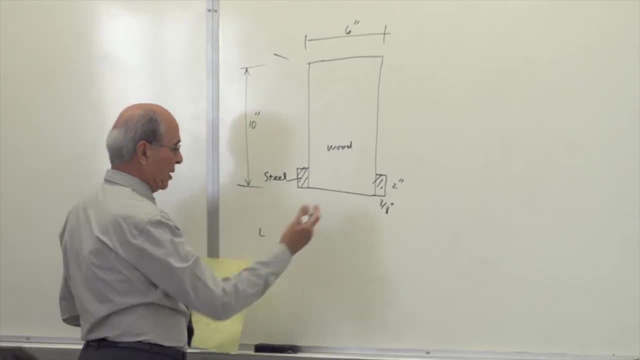 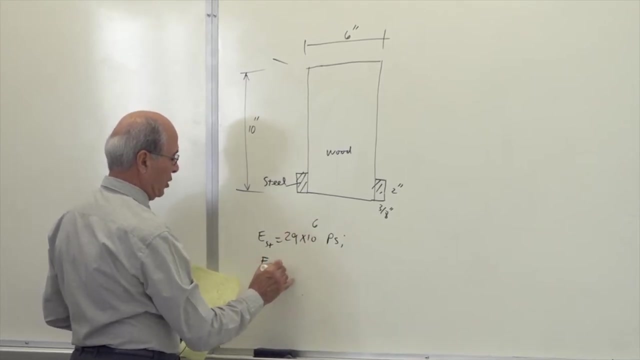 steel. The two parts are steel Symmetrical, So actually in that respect remain symmetrical. So therefore I'm going to give you E of steel equal to 29 times 10, to the power of 6 psi, And then E of the wood, which much weaker. 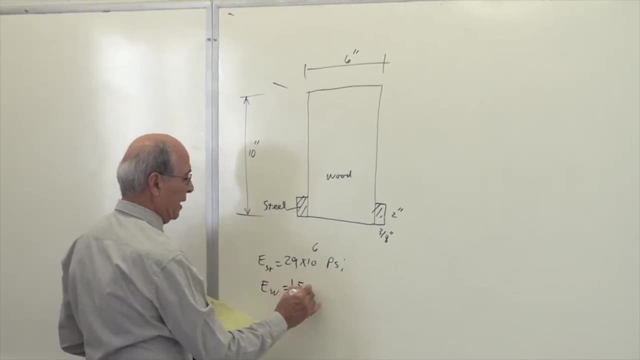 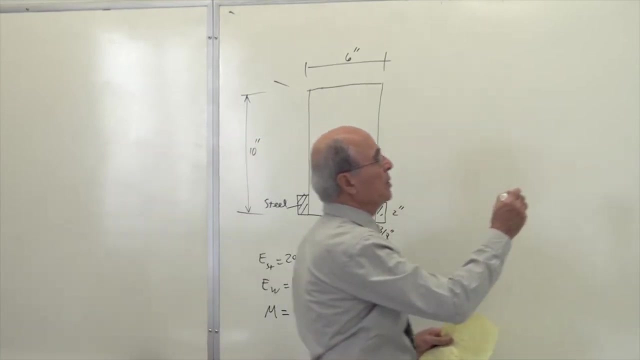 comparatively, in this problem is given 1 and 1 half times 10 to the power of 6 psi And the M is a positive M. So this is the positive M, So this is the positive M of 200 kips inch of the moment being applied to the cross section of this beam. 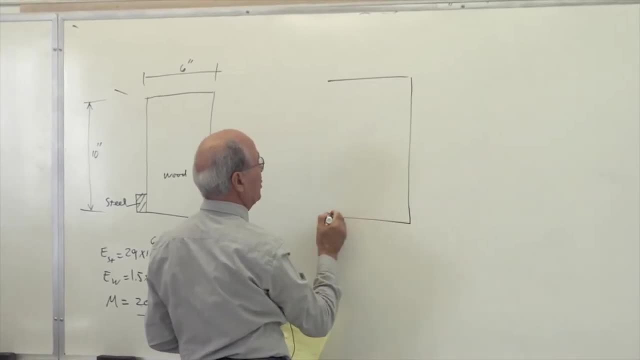 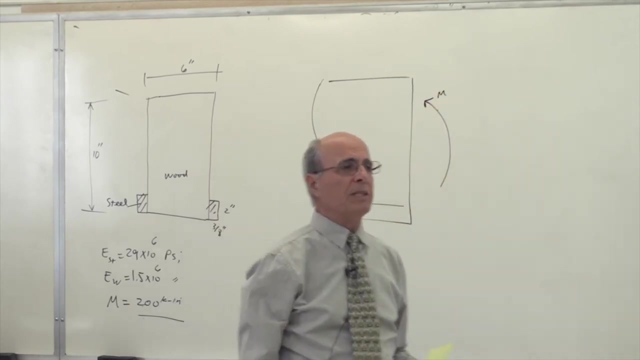 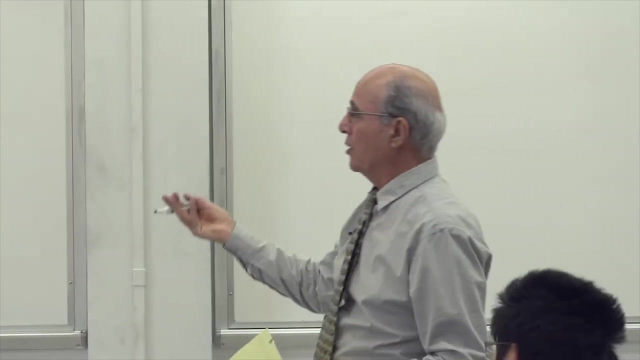 In other words the cross section of the beam. if we go side view, this is again, is the side view. This is the M, Which means compression on top, tension on the bottom. Notice: if this is the cross section, I cannot calculate the Y bar I. 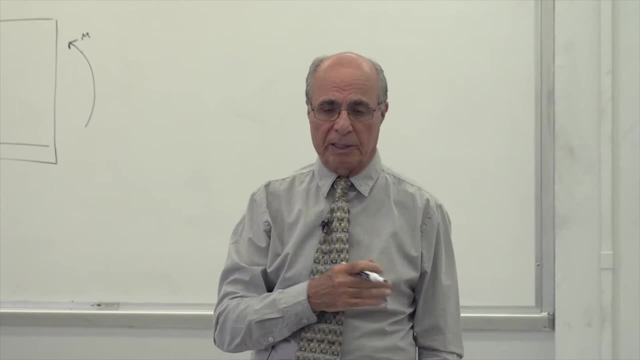 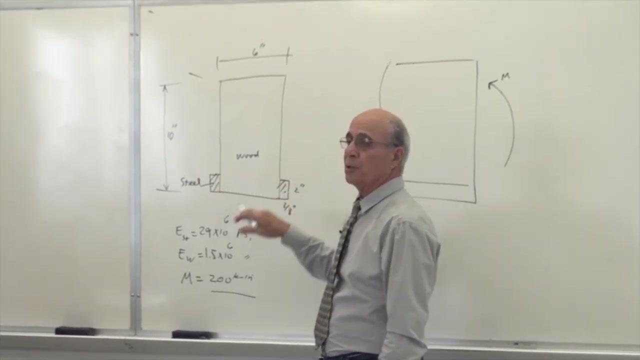 cannot calculate the I because there are two M's. So this is the cross section. There are two different material. Again, we have two option here. We can change the steel into wood or wood into steel. That all depends on how you start your. 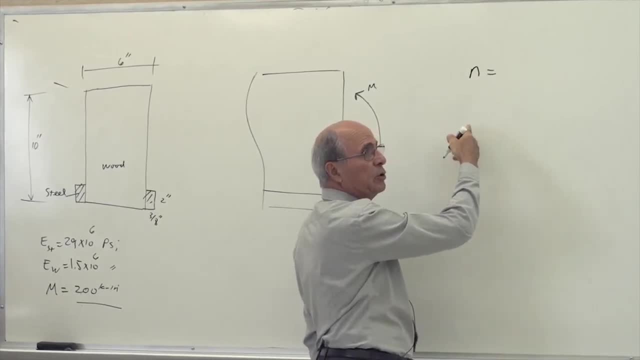 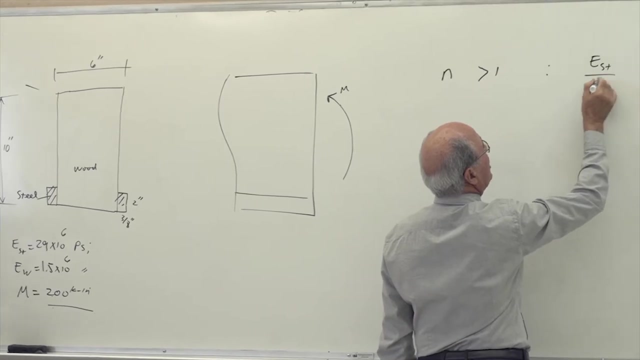 problem. I'm going to explain that again one more time here. The N usually is the ratio of the modulus of elasticity. You can take the N larger than 1.. So let's call it this way, Which gives you the following scenario: E of steel over E of. 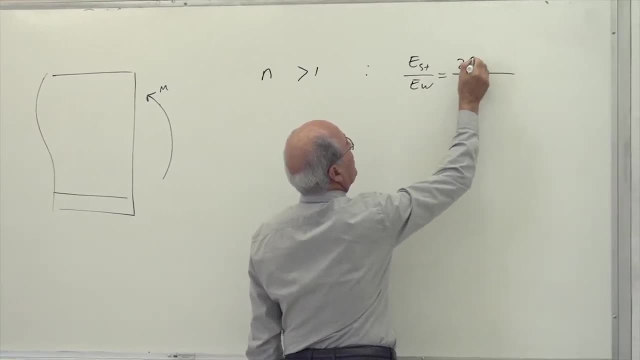 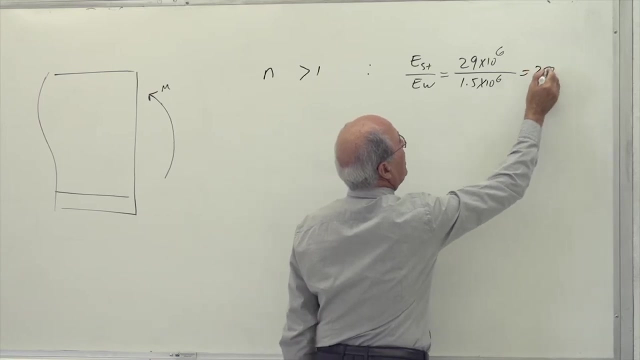 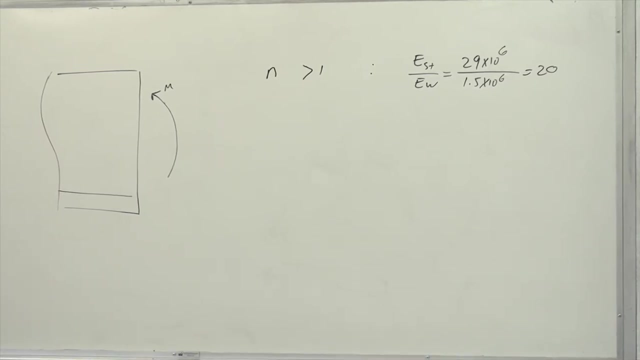 the wood Become equal to, for this problem become 29 times 10 to the power of 6, divided by 1 and a half times 10 to the power of 6.. Which, for this problem, is a ratio of 20 to 1.. Technically, in effect, E of steel is 20 times larger than E of steel. 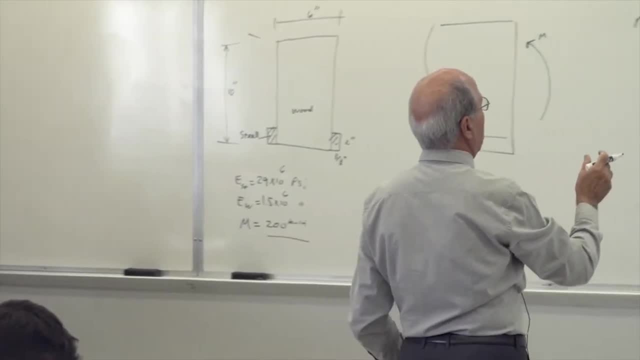 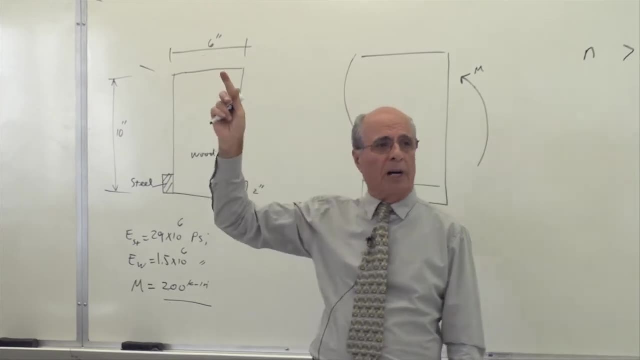 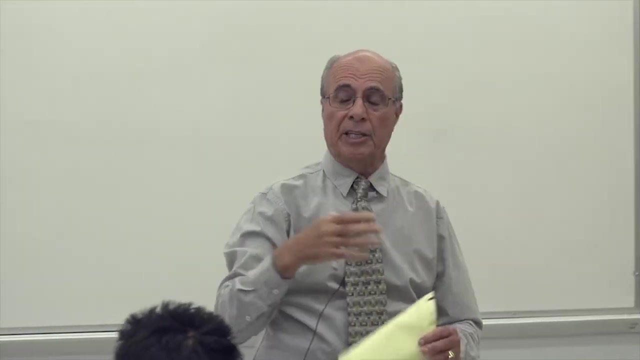 When you do that, that means I have to multiply this thickness. First of all, remember what we said here: We cannot change that Y, the height. We cannot change the height. Remember epsilon was dependent on the height, the Y. So if I change that, I cannot do that because that changes the. 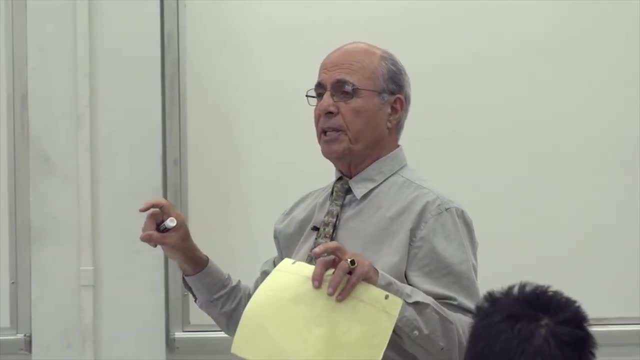 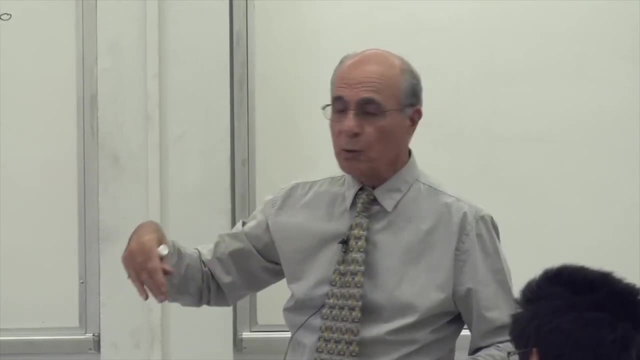 whole scenario. But I can change the width of the material. Is that correct or not? Because in the width of the material the stress was uniform, So I can do that. Therefore, when I use that ratio of 20 to 1, that means this still has to. 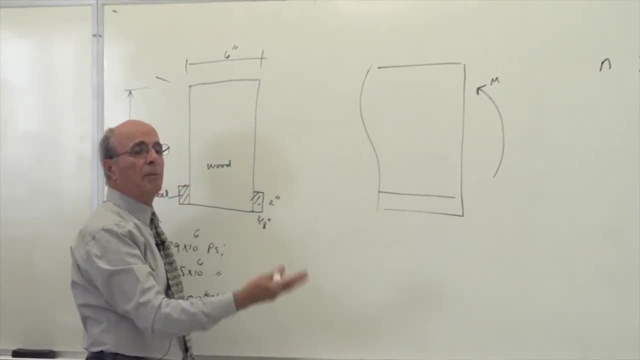 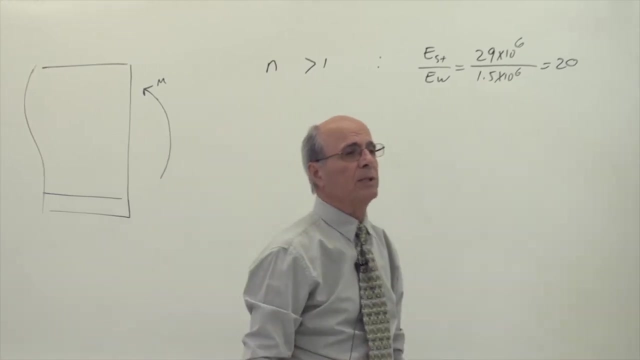 be expanded into larger And that's why I can't change the width of the material, The area, of course that become a wood. So when N is larger than 1, write it down. That become all weakest material. So it become all wood. Is that correct or not? 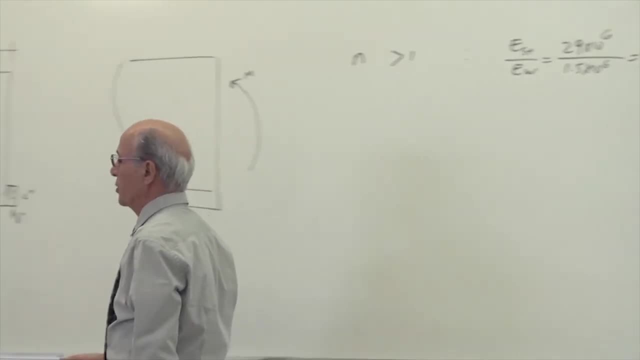 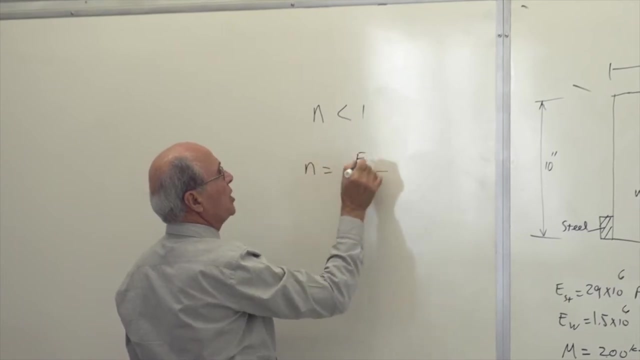 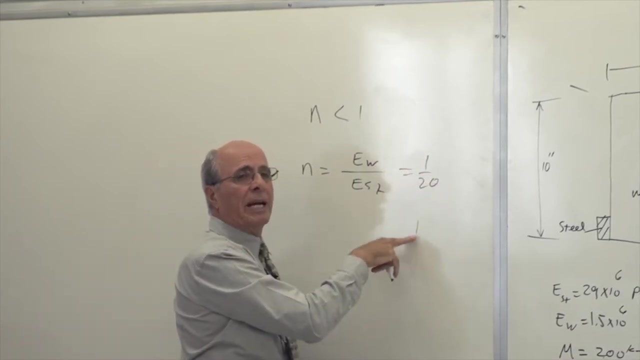 The alternative to that which we can use- but I put it on the other side because I'm not going to use that- is using N less than 1.. That means I can use E of the wood over E of steel, which become 120.. Remember, this is less than 1.. That means 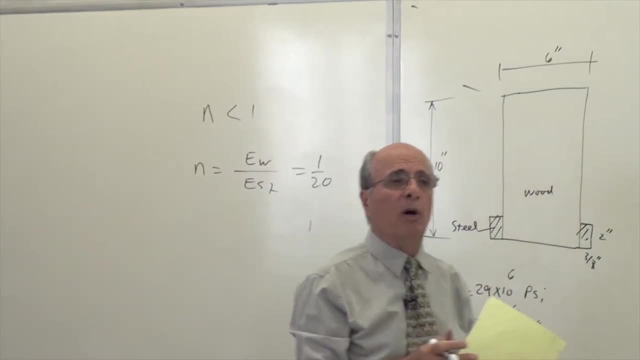 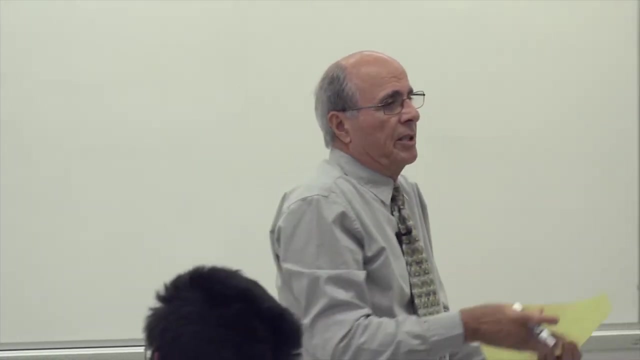 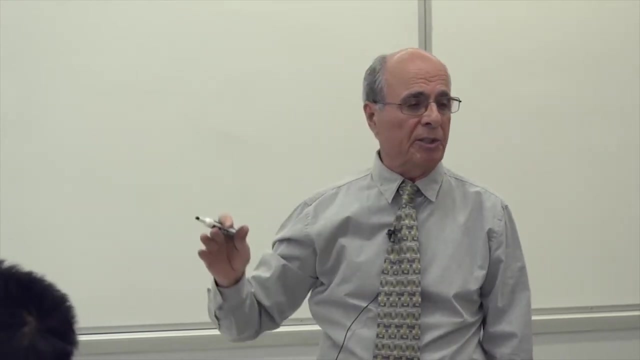 that the thickness of the wood should be shrink 120 at size in order to become equivalent to steel, because I need less steel to be replacing wood. So you have two options. So some problem. you have to look at it to see which one is easier. 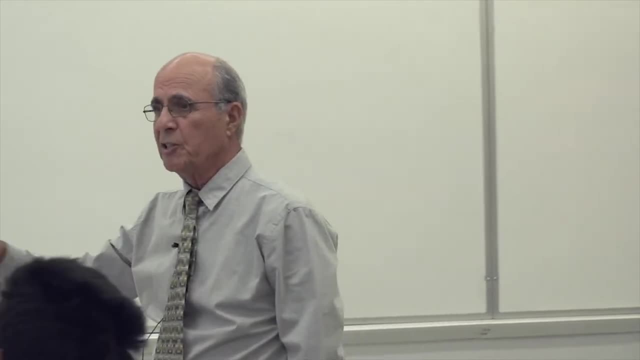 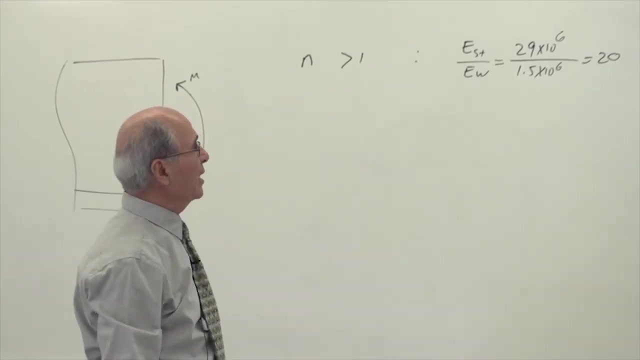 because sometimes there are more work. I'll show you at the end, after I finish this, which one is more appropriate For this problem doesn't make any difference, so I'm going to use this one. Is that correct or not? You will think that one it. 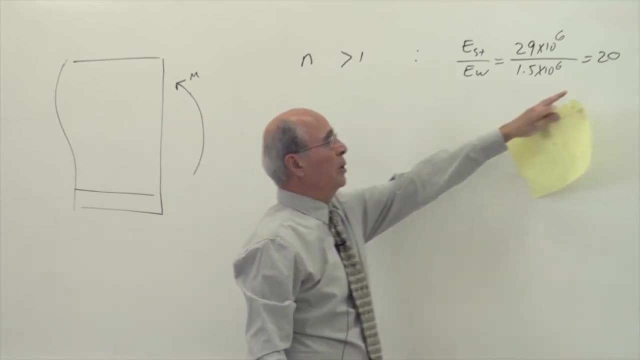 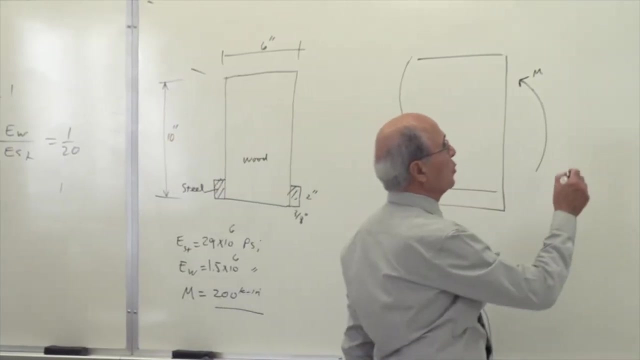 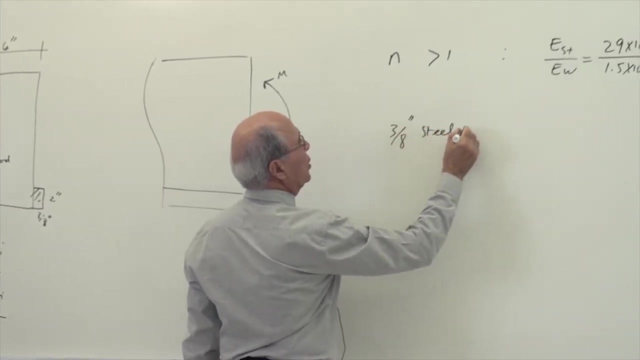 means all wood. Everybody understand that Why? Because this 20 is larger than 1, so I have to multiply this steel by that ratio. So how much wood would replace this much steel? I have 3 eighth of an inch of steel become equivalent to that's. 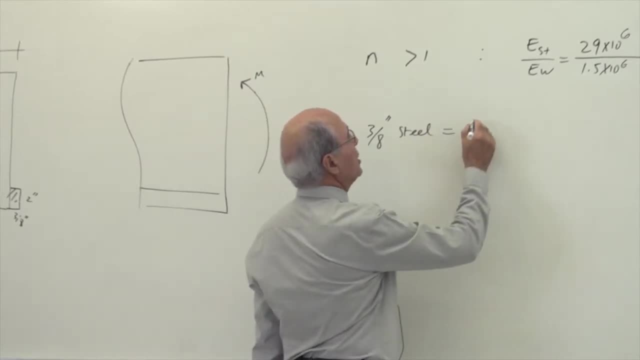 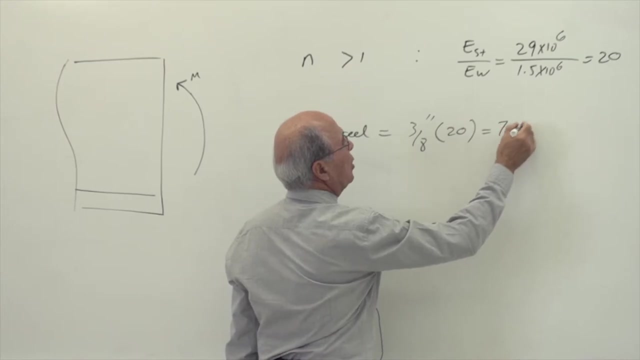 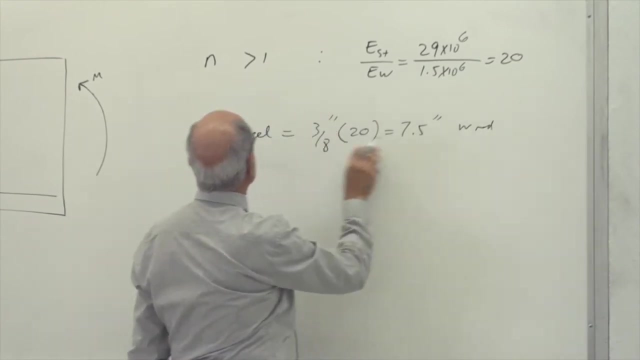 equivalent- not exactly equal equivalent- of 3 eighth of an inch multiplied by 20, so it become equal to 120.. Equivalent to 7 1⁄2 inch of wood. So another 7 1⁄2 inch of wood is equivalent to: 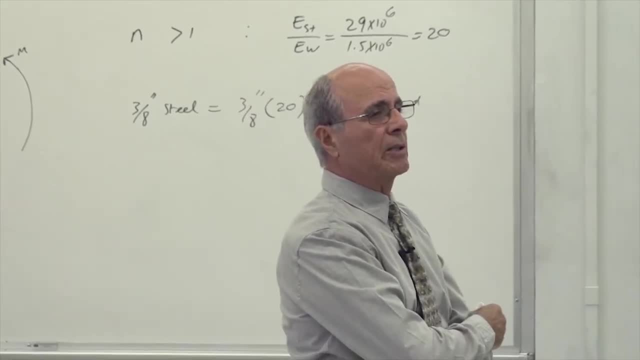 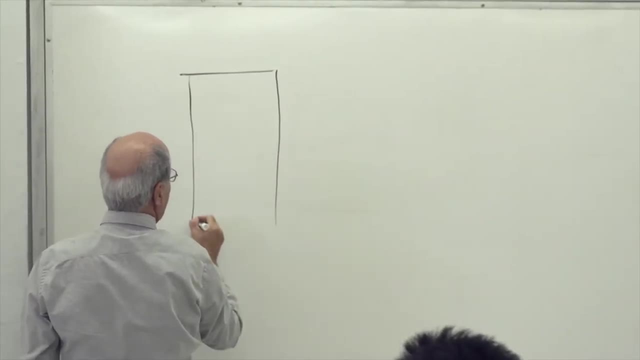 3 eighth of a steel, because the ratio was 20 to 1.. Is that correct or not? As the result, your section ends up to this section. So here is your section. The wood remain exactly the same. So this is 6 inches. The height is 10 inches. Suddenly, 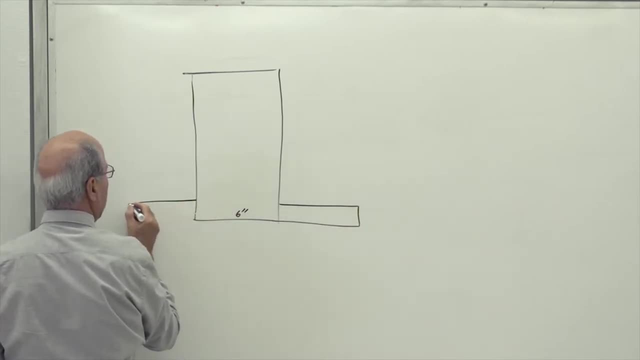 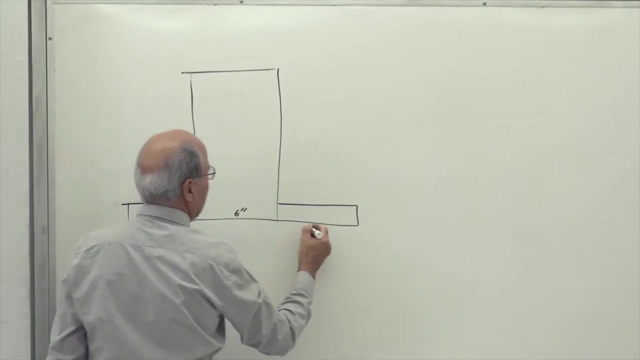 you see, here, instead of 3 quarter of an inch. you see, sorry, I have two more. I have to be on the same level. You see, there, equal to 7 1⁄2 inch, here 7 1⁄2. 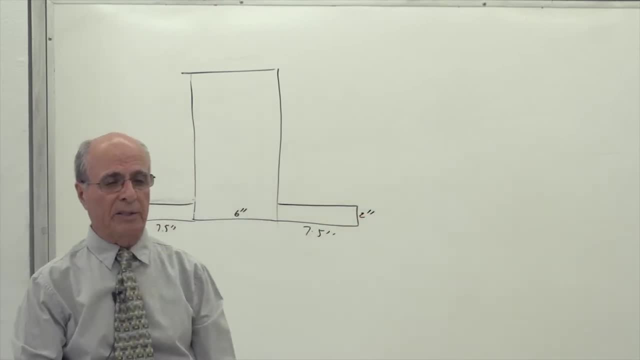 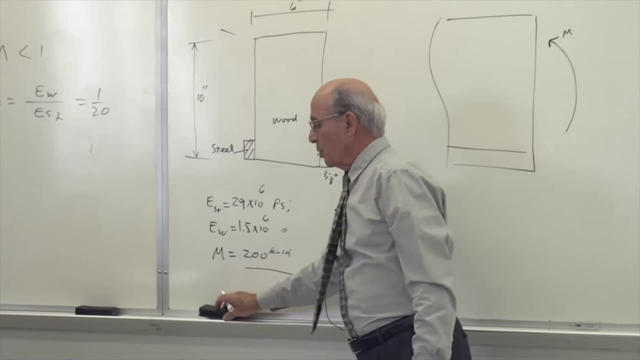 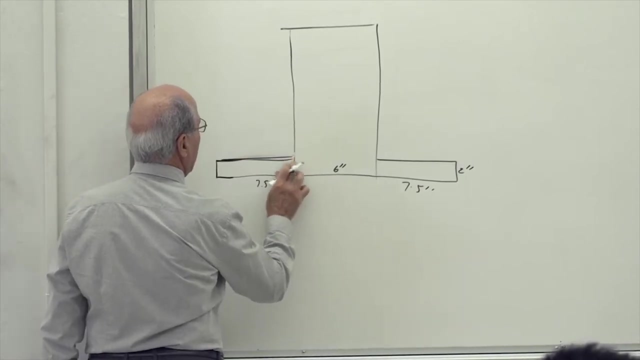 inch. here Height cannot change, As I said, the Y cannot change here. So that become this much steel. So it has to be exactly the same to be symmetrical. So should I show you this a little bit shorter? So let's assume these are this. 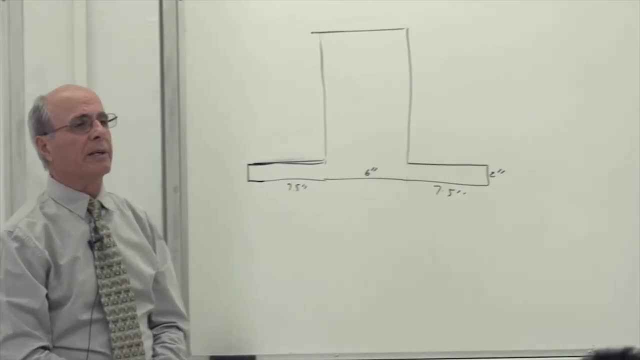 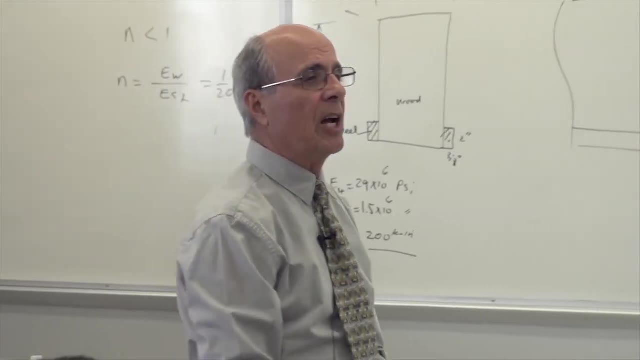 Which, back to This, is all wood. Is that correct or not? Now I can use the same technique I used before to solve it. Now notice the centroid has changed and I have to find the I. Is that correct or not? I'm not going to do that. That's a. 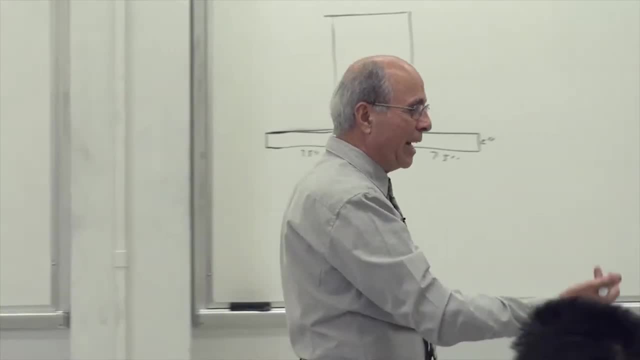 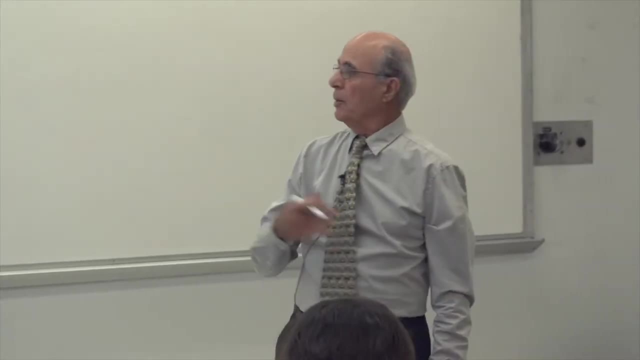 waste of time. I already did that. That's the whole idea of it. Last class, I use a T section and I calculate the Y bar and the moment of inertia. I'm not going to repeat that, But remember that this is 2 inch, This is 7: 1⁄2 and 6 and 6.. 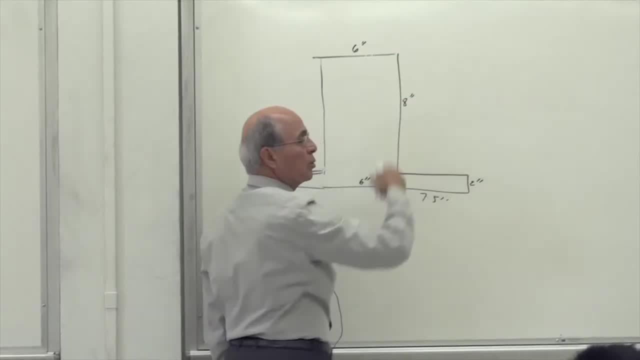 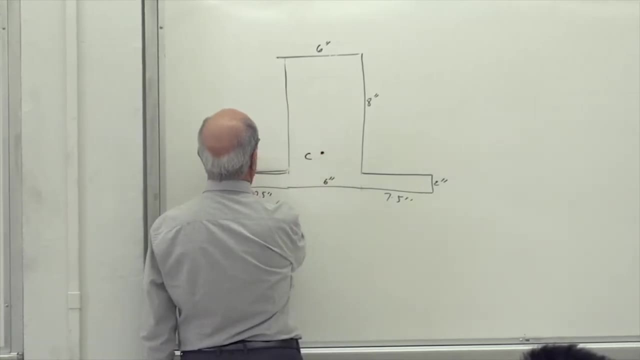 This is 6 inch And this height is 8 inch because the total was 10 inches. Is that correct or not? Therefore, you calculate first the centroid. So if I put the centroid, which will be the neutral axis, you have to use all wood. now That? 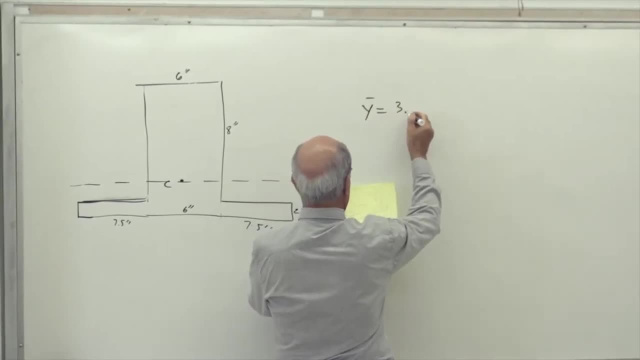 we did it, So you get 3.67, I believe, Yeah, 6, 7.. So if this become your first, you put your X here, So you call this one Y bar. That's what I did last time You. 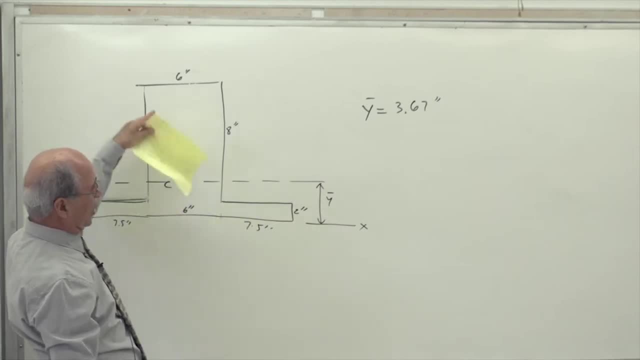 put your X axis here, You calculate all the Q's and you keep your Y bar. You and you calculate with respect to this x axis divided by area, to calculate y bar, Which is where notice what happened. again To review your static, because I need. 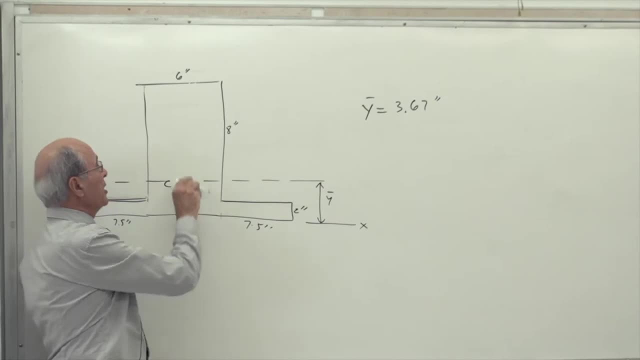 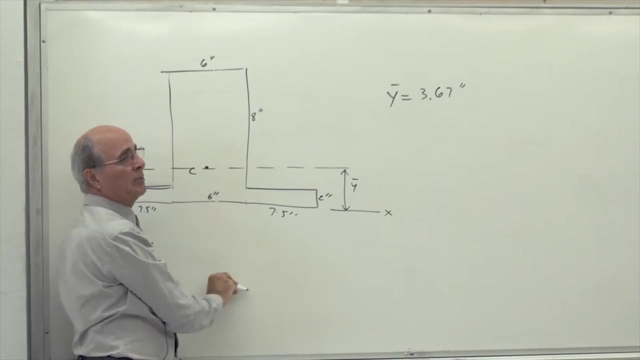 this for chapter six as well. When the x is here, this area and this area, the second area, have a q here, as I did it last time. Remember that If the x is here, then q become different. Is that correct or no? If x keep moving up here here. 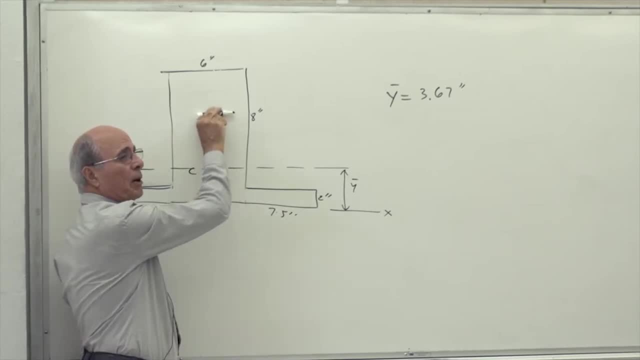 here, here, when it gets here, notice some q's are above the line, some q's are below the line, and we proved that several times in the static classes, and here I mentioned that the q of the above and q of the below become equal and opposite. 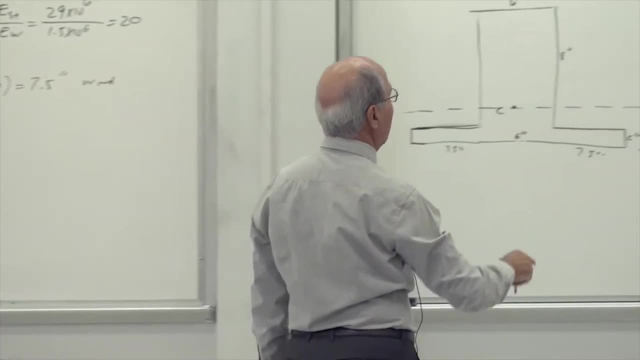 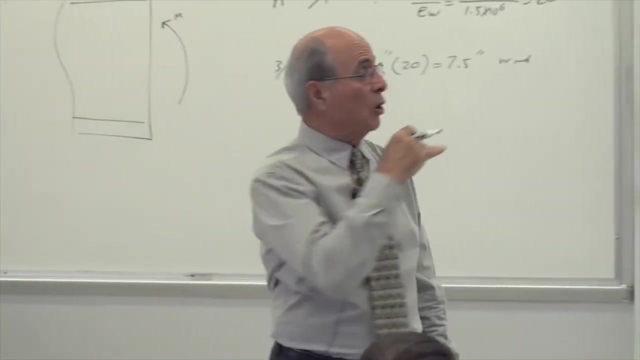 in order, total q to become equal to zero. Why? Because now I'm changing this x to this x, Everybody understand. I'm suddenly changing my force from here In order to be at that point with respect to this axis. of course I'm changing. 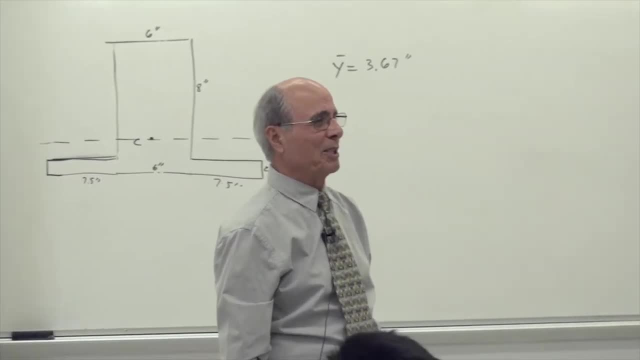 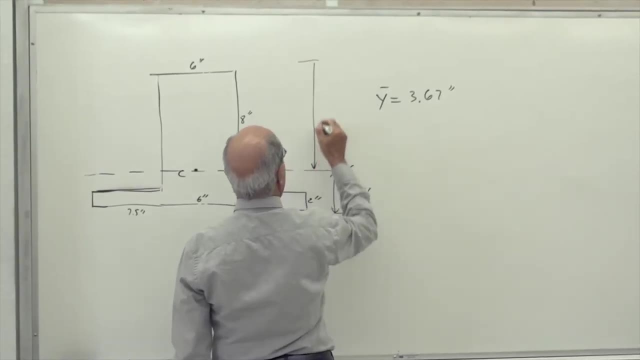 my force. Of course, y bar must be equal to zero. Is that understood what I'm saying? Therefore, after we calculate that, this is 3.67.. So this distance I need, which is the balance with respect to 10.. So it is 6.33 inches. The problem is: 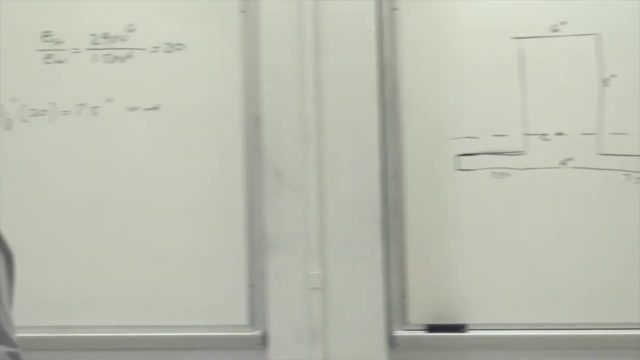 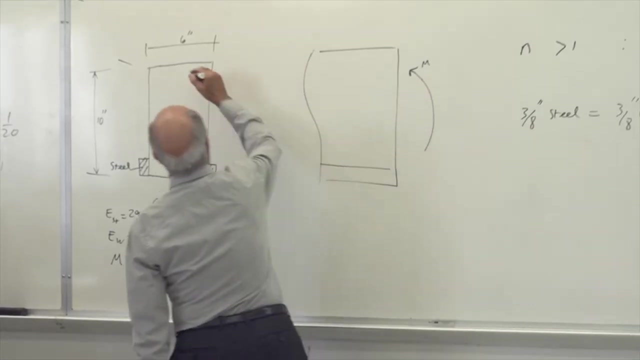 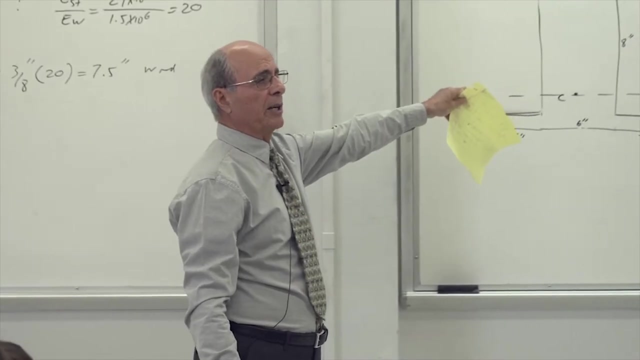 resolved. Now it's back to the exactly the same problem as I did last time. Is that correct or no? Yes, Let's calculate the sigma here. point a, That is, we would, it was wood. still is wood. Is that correct or not? Therefore, what's the? 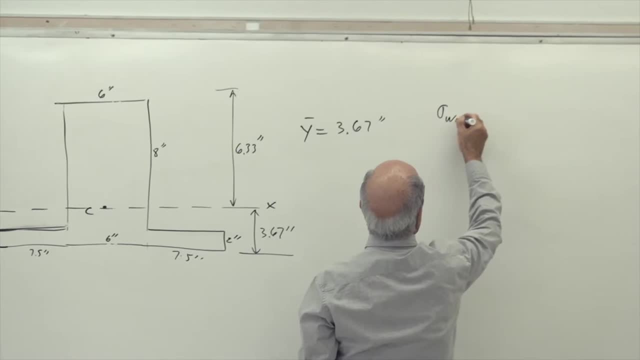 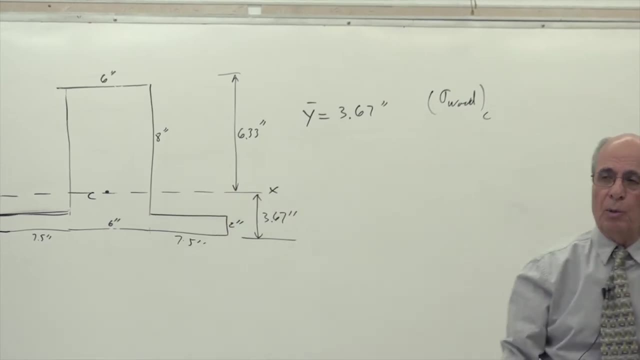 sigma. at that point Sigma, we call it wood, material wood, But it is in tension or compression, according to your moment. It is in compression, Therefore it become minus. How much moment did we have there? I have written it here: 200,. 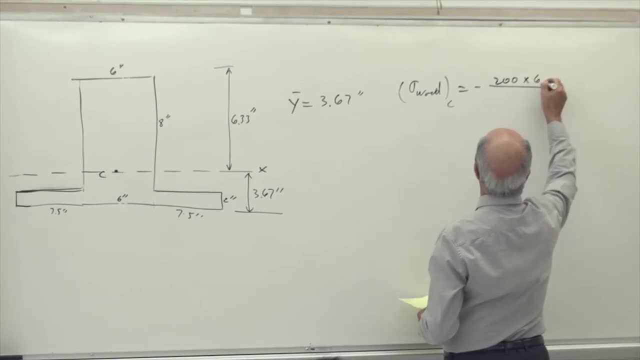 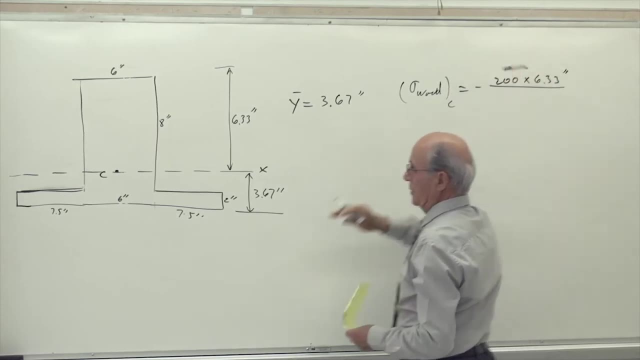 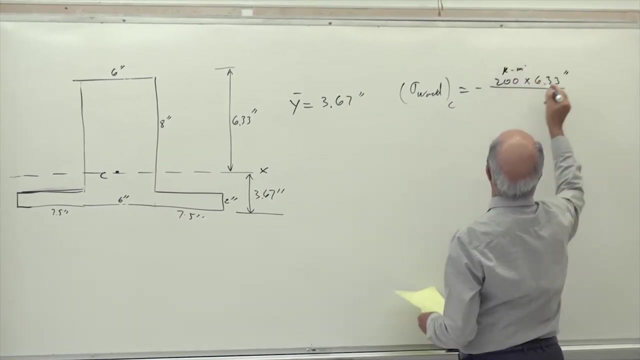 the unit work: kips inch multiplied by 6.33 inches, And this is pound inch Or kips inch. I'm sorry, Need to raise it: kips inch. So we get the answer in KSI: Kips inch And that's inch divided by. oh, I forgot to put you the i with. 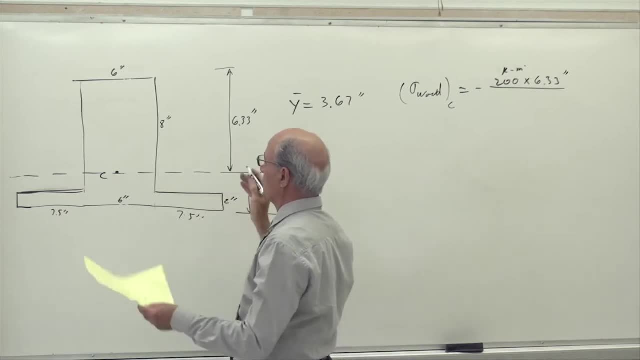 respect to the neutral axis. By the way, this axis, whether it's x or z, doesn't matter. This is the neutral axis that passes through the centroid. So i again i calculating, i, with respect to this x axis, you need parallel axis Theorem I. 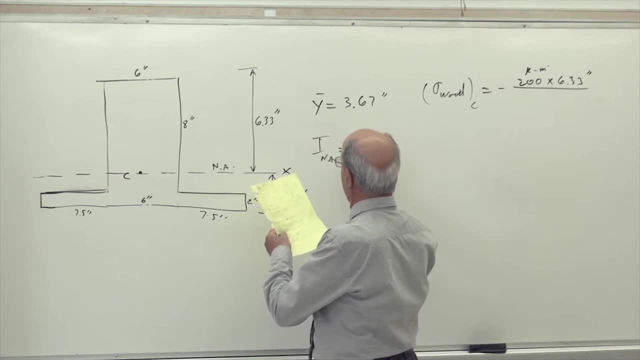 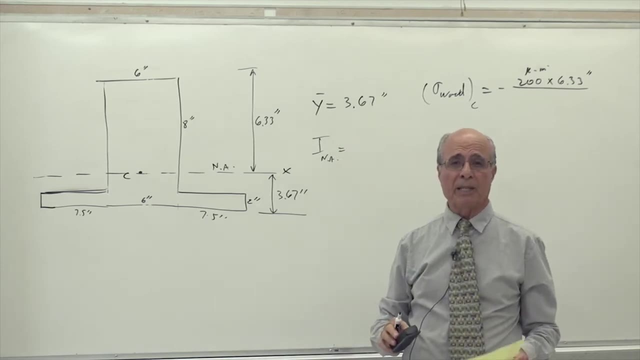 asked you to study that, So I cannot help you with that department anymore, unless you ask me question. By the way, there is no quiz today for either classes, So today office hour would be very empty, So it is good chance for you. 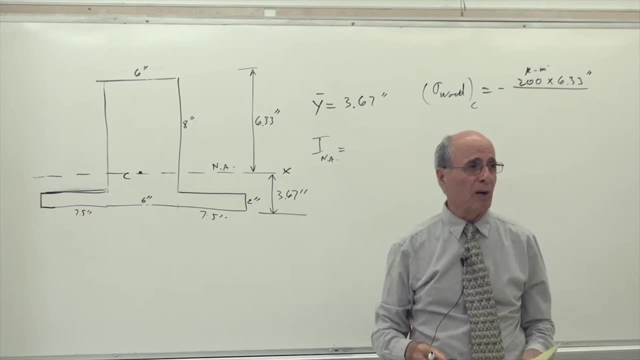 to have all your question being answered. So if you want to come to office hour, today is the day. Is that understood? Okay, Don't leave me lonely there. Don't leave me lonely there. Is that correct? Nobody showed up. If there is no quiz, 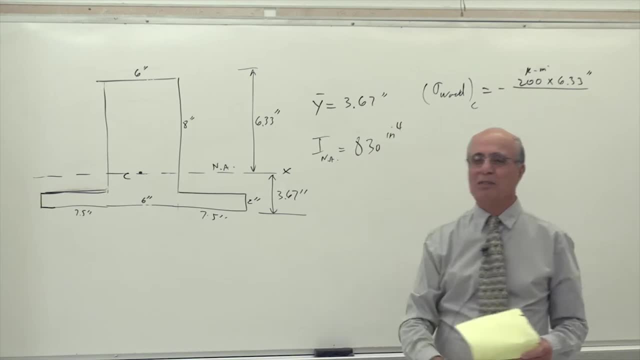 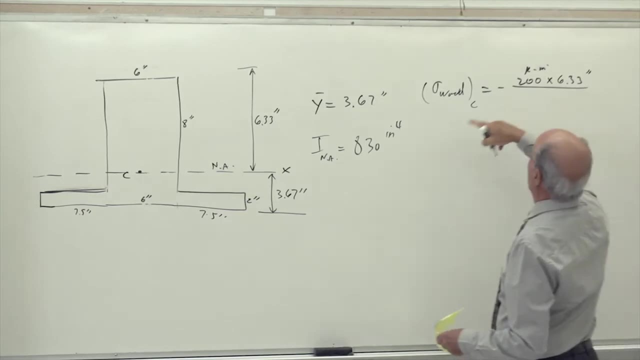 nobody shows up: 810 each to the power of 4.. So that's the answer. So that's 4.. Yes, Okay. So therefore, now we have to calculate sigma at point a, which is the old wood, So, or in this point there, And that is divided by 830.. So 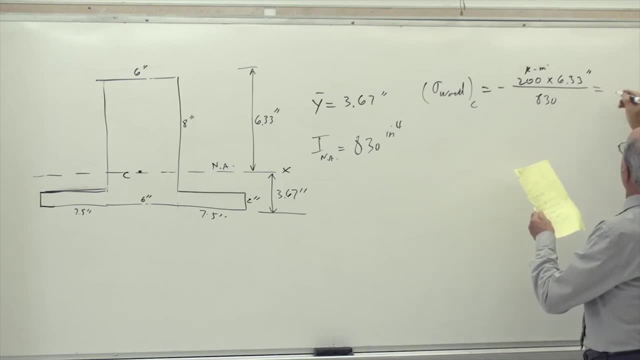 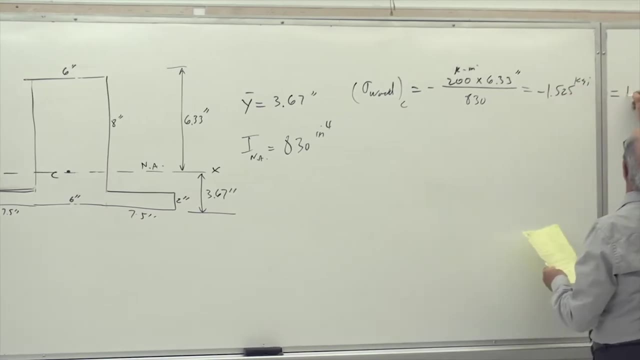 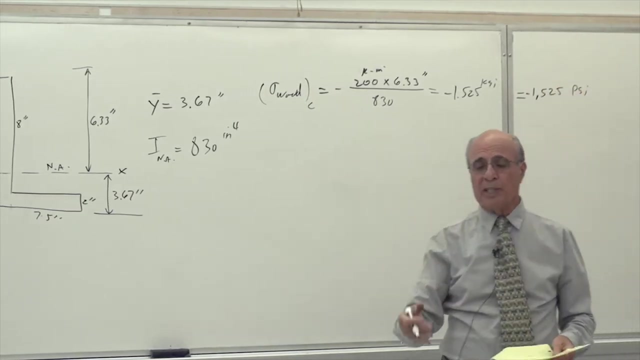 therefore each to the power of 4. So it become minus 1.525 ksi. Since it is wood, we better do it in psi. So 1,525 psi, That's the same thing. Usually, when it is wood or weaker material we say psi, when it is a steel or stronger Maybe. 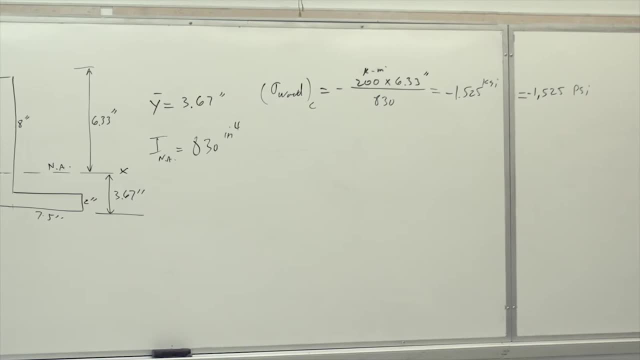 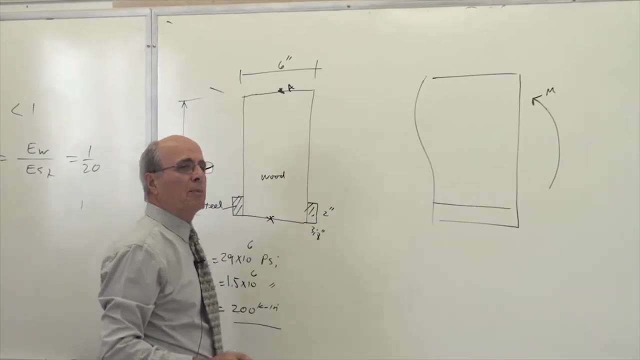 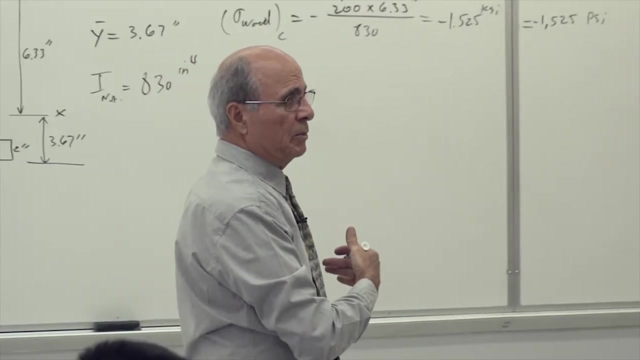 go with ksi, because that's usually the case, Yes or no. Then how about this point Point b here? That point was wood still is wood, The only difference that it is in the tension zone. Is that correct or not? So it's still sigma wood. So 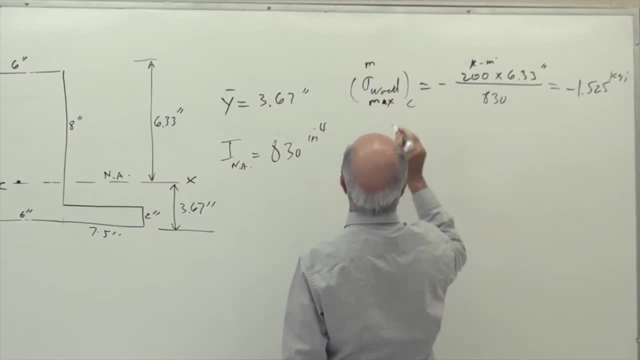 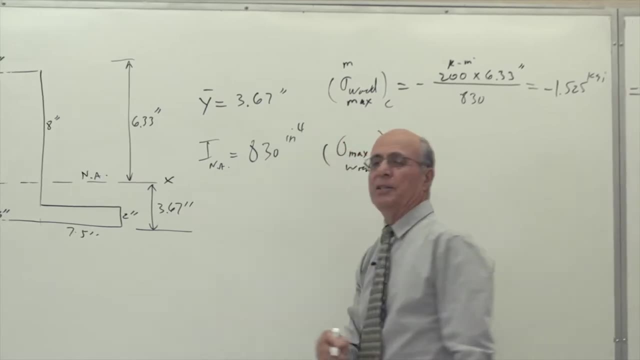 you can call it sigma max if you want. So it's wood max, Sigma max, but this time in wood, the same thing. Or however you write it, it doesn't matter, It will be in tension, Yes or no. I've calculated tension. That would be. you can use the. 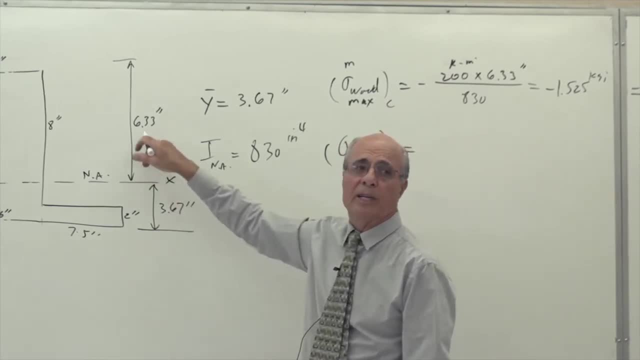 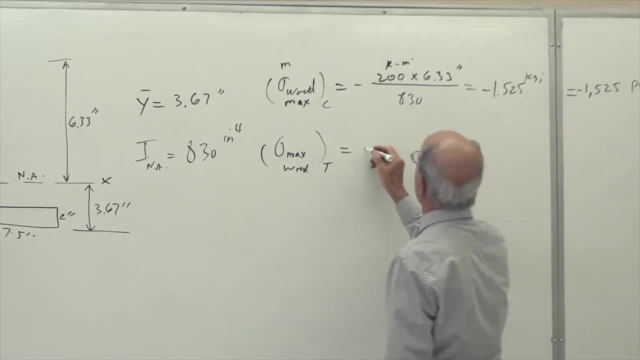 ratio. Remember, I can use the ratio of 3.67 over that one because it is linear. We talk about it because the stress is linear. I can do that Or I can recalculate that. That's the same thing. So 200 times 3.67 divided by 830.. So 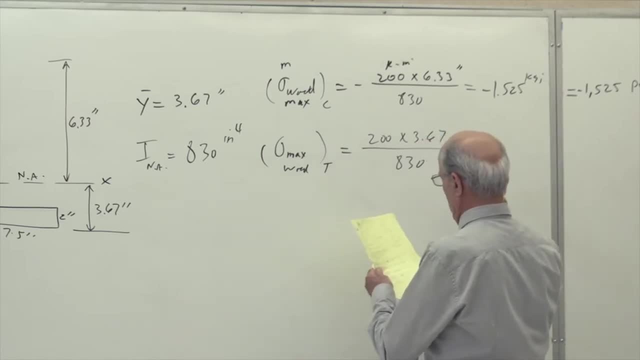 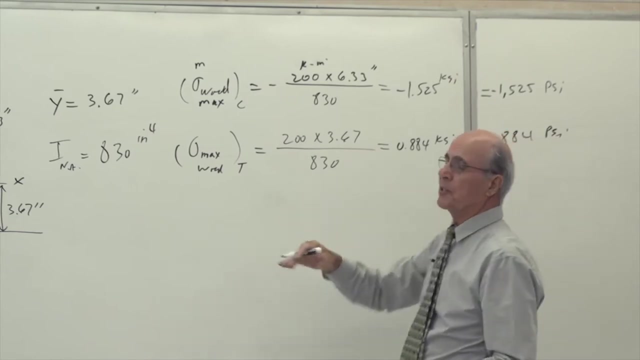 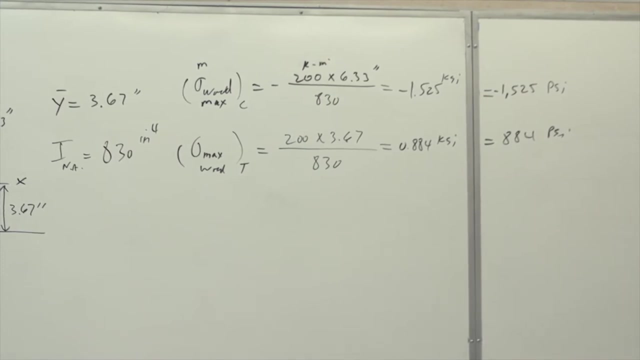 that's 3.67 divided by 830, which is equal to .884 ksi, or equal to 884 psi. Of course it is less because less distance. This distance is almost half of that, So the stress becomes half, Yes, Linear. However, how about the stress in the 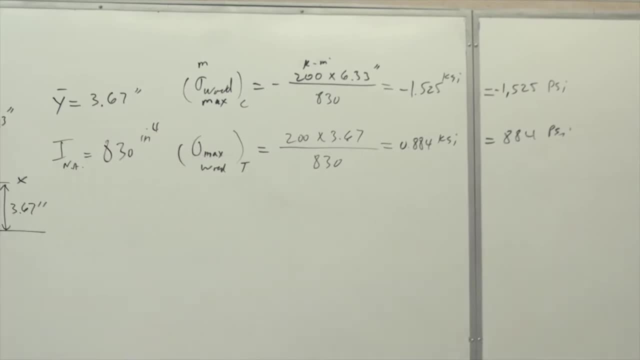 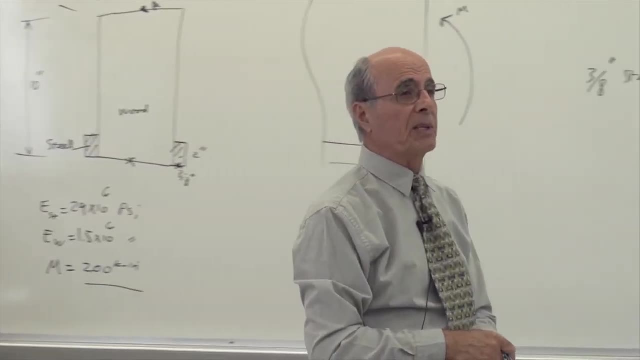 steel, Don't we? are we interested to find the stress in the steel? Yes or no Stress in the steel? I need to find stress here now. This is the maximum stress in the steel. We don't care about the top of it. Steel, all of the steel. 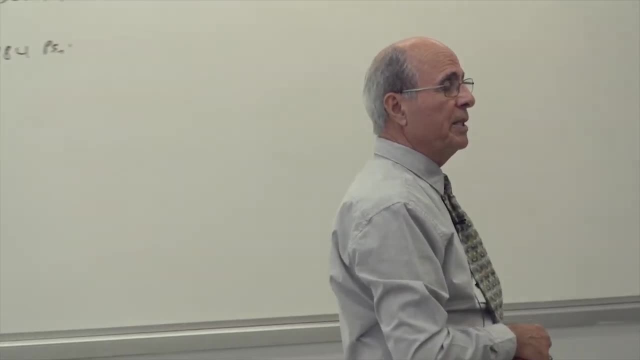 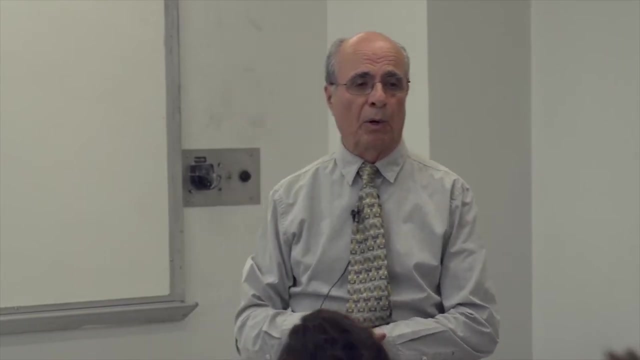 is in the tension zone. Is that correct? So the steel will be in tension zone all of it, And we want the highest value of stress in the steel. So I'll go to the furthest point. You remember that You have to go. furthest distance Is. 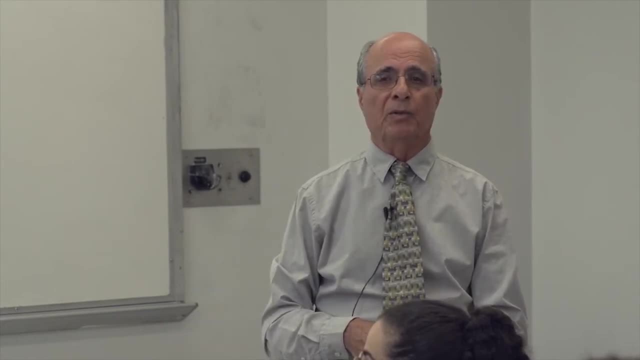 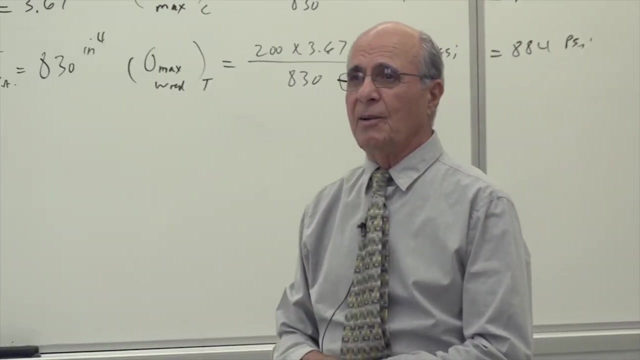 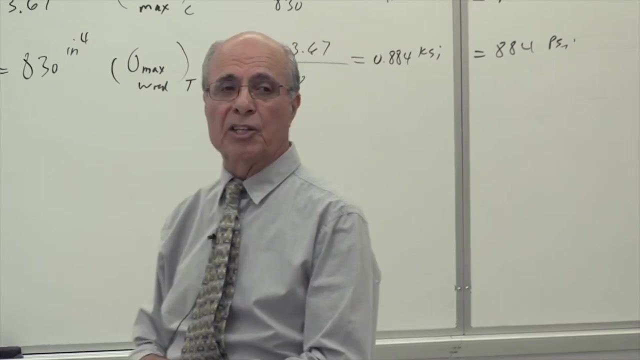 that correct. So it will be the bottom. What's that? How do we calculate that What? You should have the answer right now: What? What should I do? I already calculated without you realizing What is the stress at that level: 884 psi per. 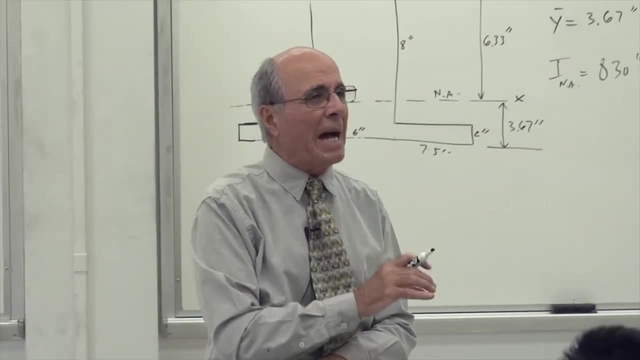 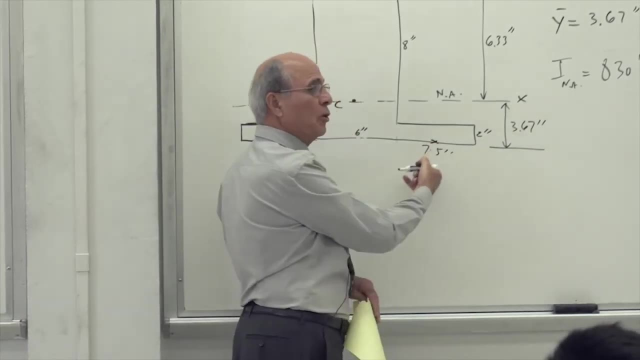 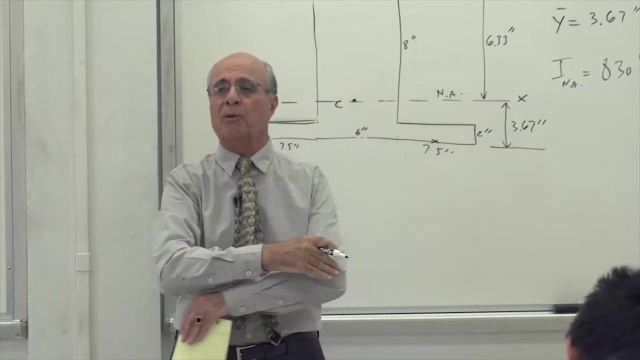 square. What is psi? It means that many pound per square inch of wood, But in this area it's. that shows Yes. So 884 pound per square inch of wood, So that's a square inch of wood. But this was not wood originally, That was. 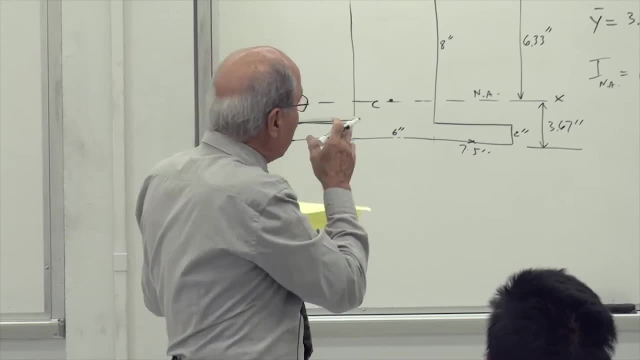 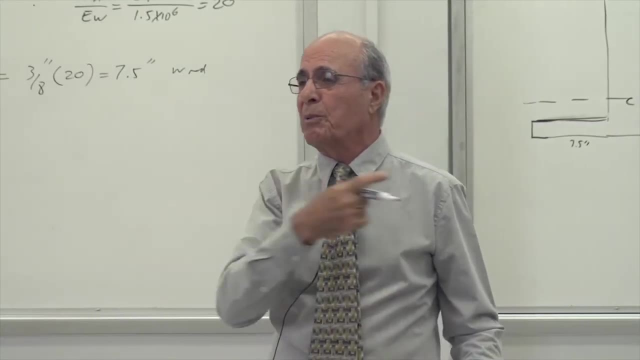 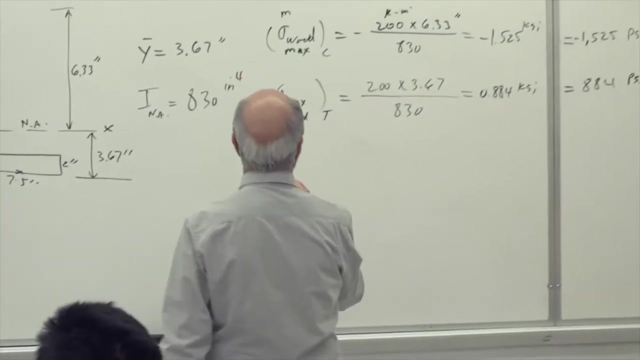 So what should I do? 20 square inches of wood equal to one square inch of steel. Is that correct or no? So I have to multiply that stress by, By 20, by N again. That's the adjustment that I mentioned last time. So sigma maximum in steel. 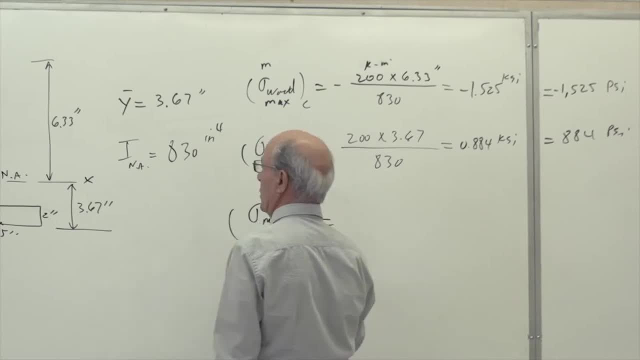 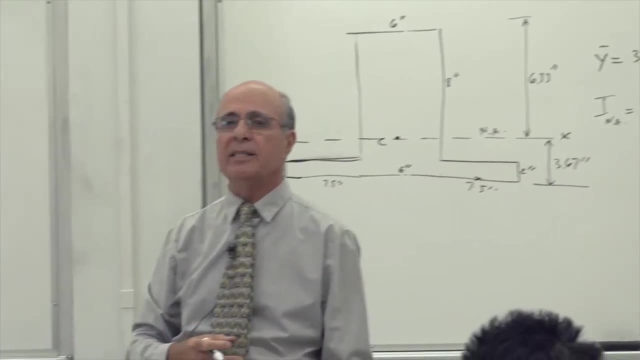 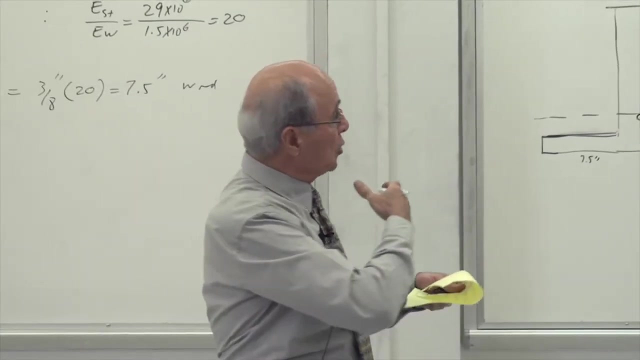 which definitely will be in tension. All you have to do, look, you have to shrink this back, So you have to bring all the stresses and put it in one square inch. if I had that Is that Because sigma is the unit, Sigma is the amount of pound per square inch, But you expanded it. 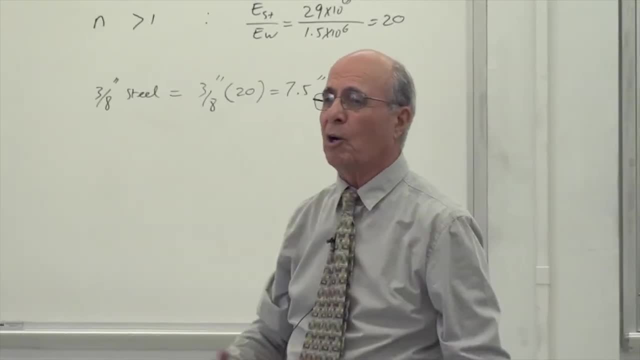 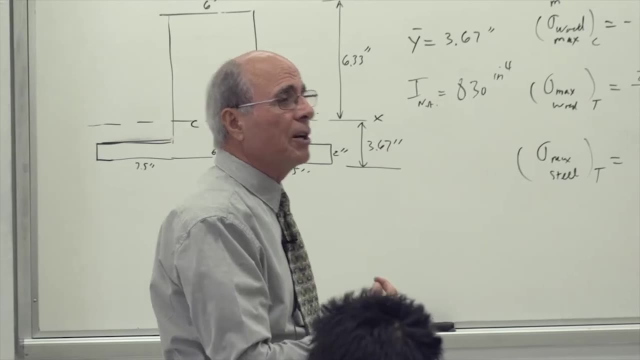 Yes or no, Then you have to bring it back. So all the stresses come together, all the forces come together. back. Is that correct or no? So 20 square inch of wood equal to one square inch of steel. Therefore, all you have to do get that point. 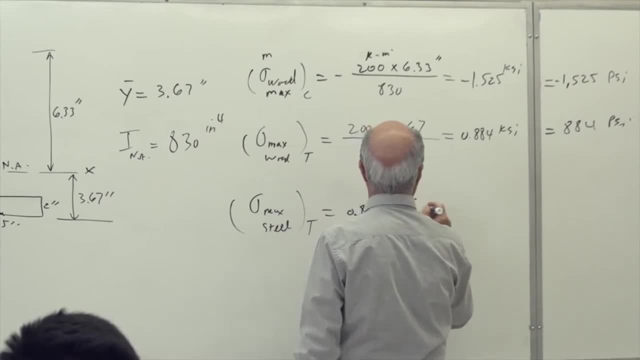 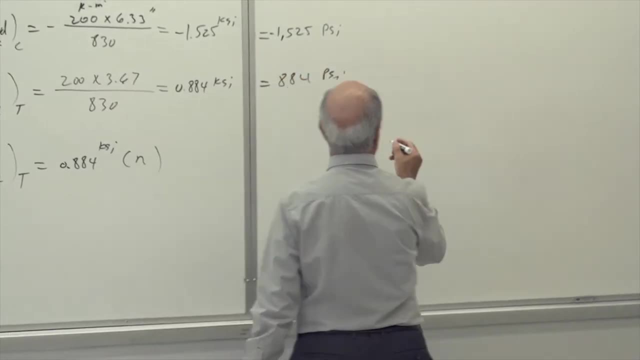 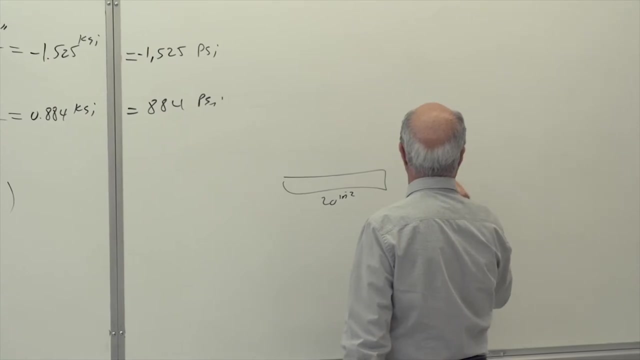 8.884 KSI. You have all you have to do. multiply it by the end, as if- as if this is what you are quite frankly doing. This is 20 square inch. 20 inch square suddenly become one inch square, But here you have 844, 884,, 20 times. 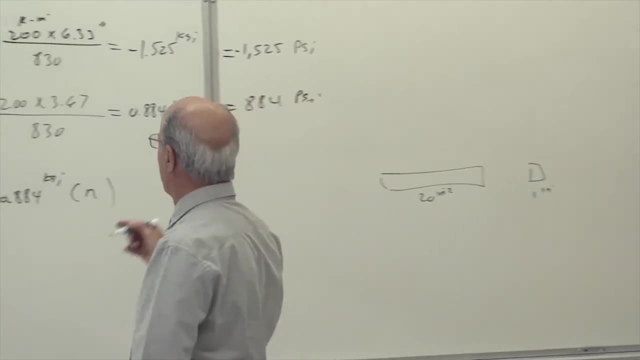 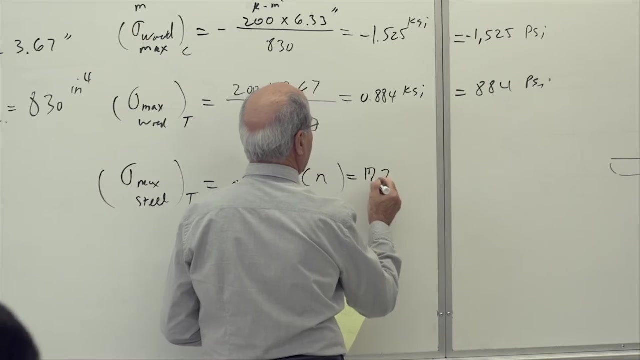 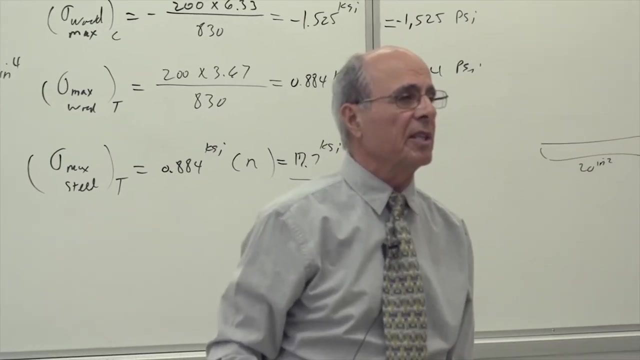 And you have to put it all there. Is that correct or no? Very simple, But I'm saying it this way. So actually you will see it become 17.7,, 17.7 KSI and almost 18 KSI, which is half the sigma yield of the steel. The steel has 36, a. 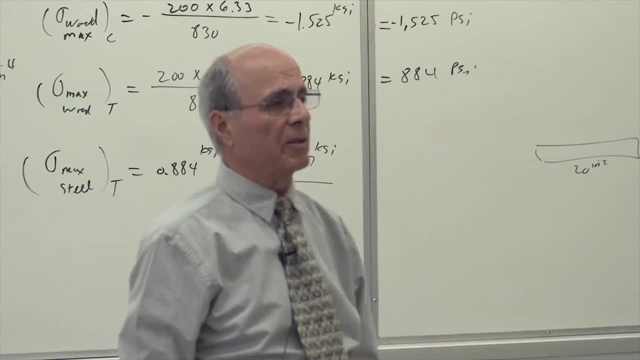 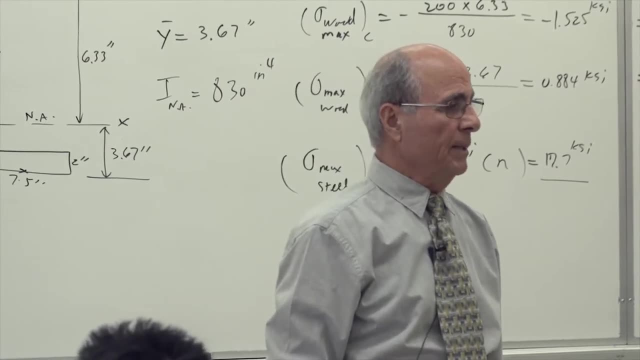 standard steel has 36 KSI units, So you have a factor of this. You see how much, how much help the steel is there. Is that correct or no? Yes, Okay, All right, Now for some of your homework. you have to decide now, So I'm just going to. 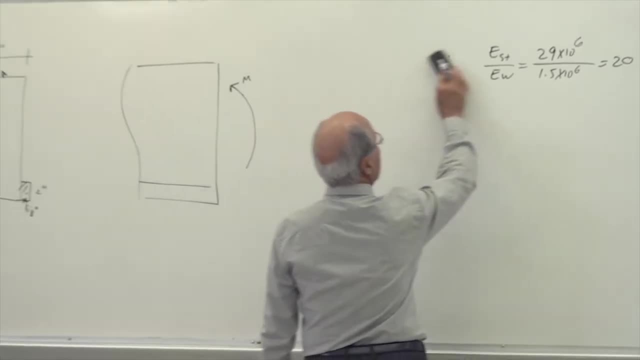 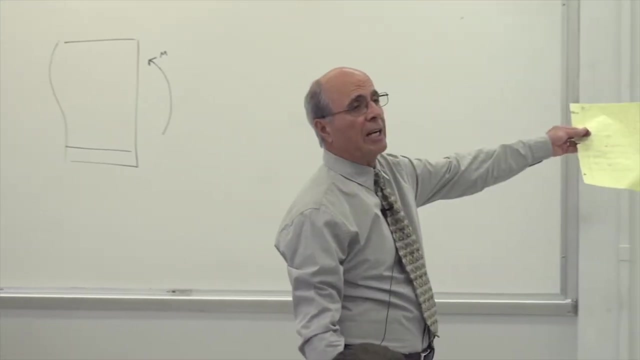 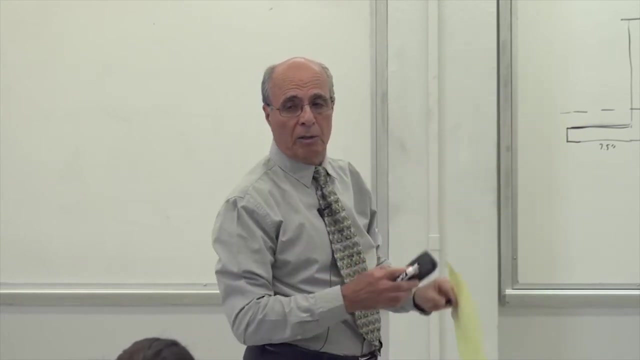 give you a few hints, because that's all you need. So you change it at the beginning. You either go from stronger material, all the stronger material, or all weaker material. Here I had all weaker material because I choose N equal to 20.. If I would have N equal to 1 over 20, then I'll make it all stronger all. 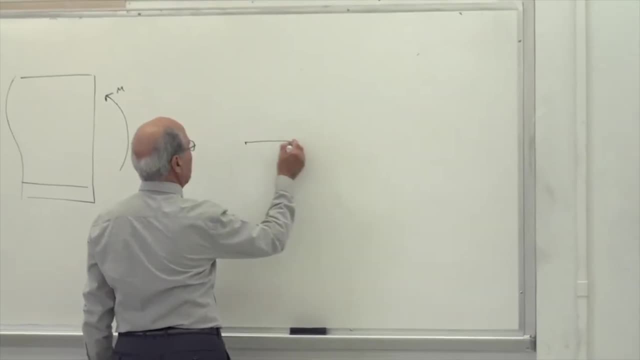 steel. So you choose your system. So if you have here, I want you to understand- if you have your homework- I don't know how many homework I gave you, maybe two or three- So if you have a plate on top, you have a plate on top, you have a. 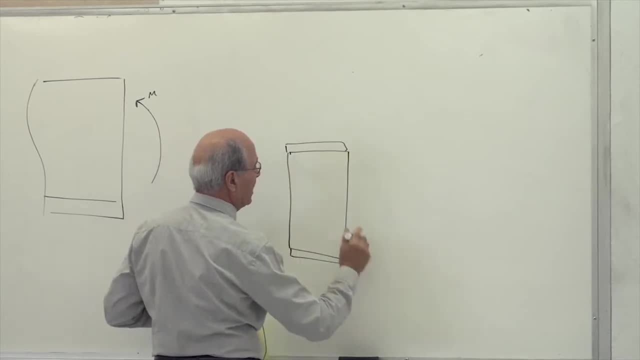 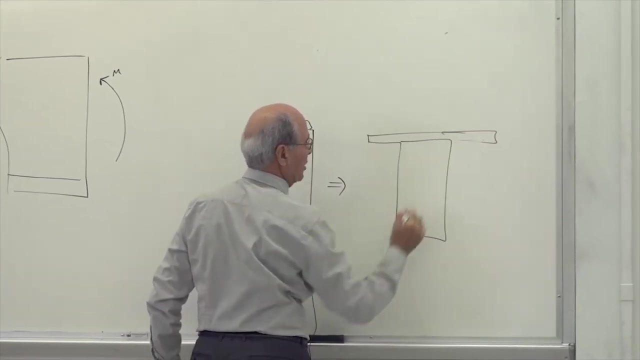 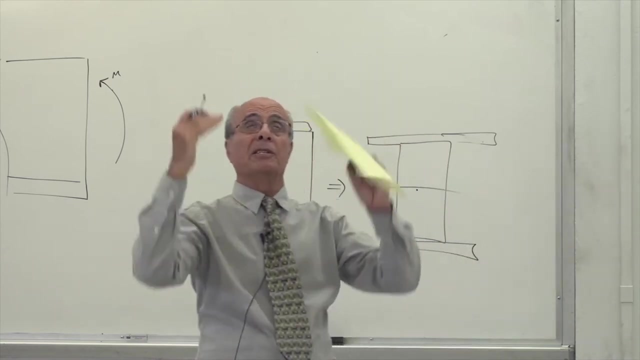 plate on top and you have a plate on the bottom and you expand it. this becomes similar to just what I did, except it becomes symmetrical. Everybody understand what I'm saying, Because both plates are going to expand. Centroid again remains the same. However, as I said it here, I don't want to touch the. 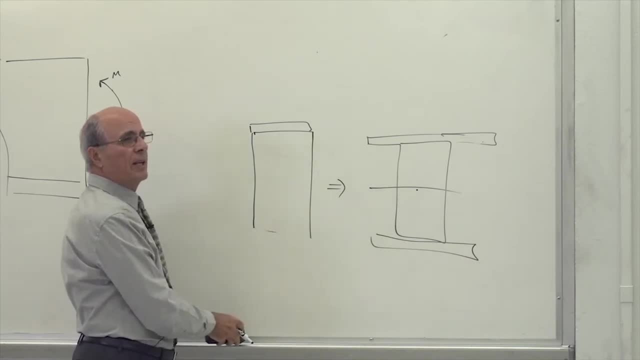 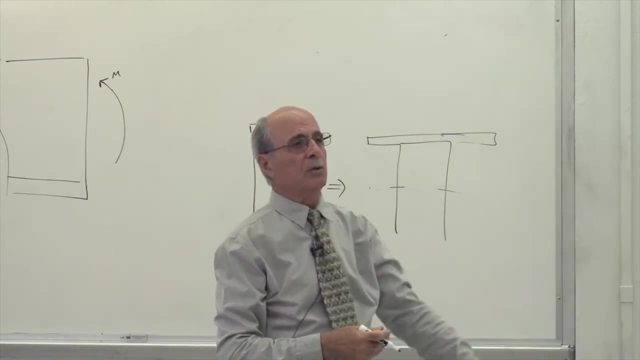 ceiling. Sometimes we do this. Yes, If we do that, then we don't have that one. Is that everybody understand? Then system become a T-shape So you have to change the T-section. I show you the T-section already. Then there are other. 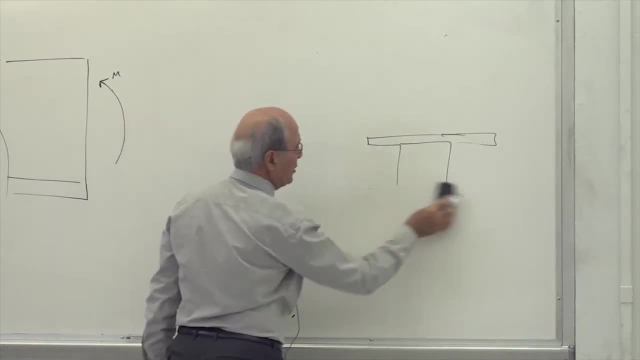 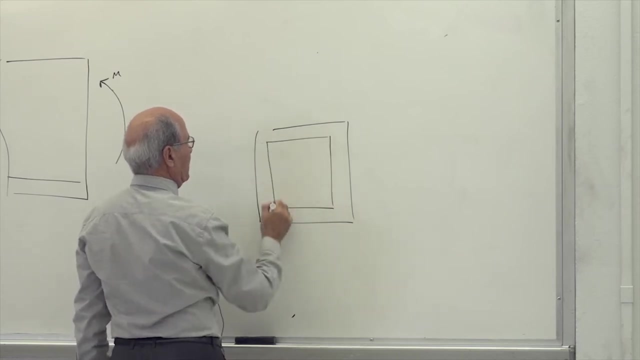 options. Sometimes you have a pile or beam or whatever. Let's say it has a hollow tube still filled with concrete. So this is concrete. I think there is a problem like that. These are all steel and concrete. Which one is easier to change? I 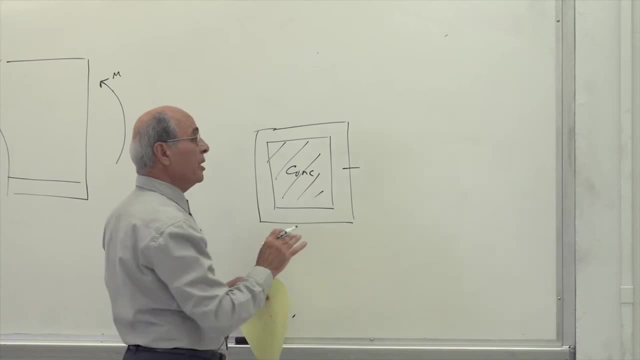 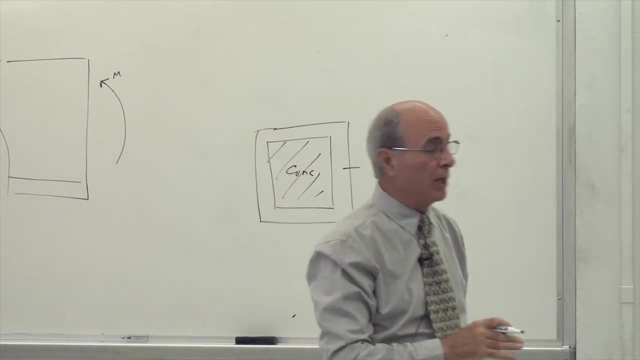 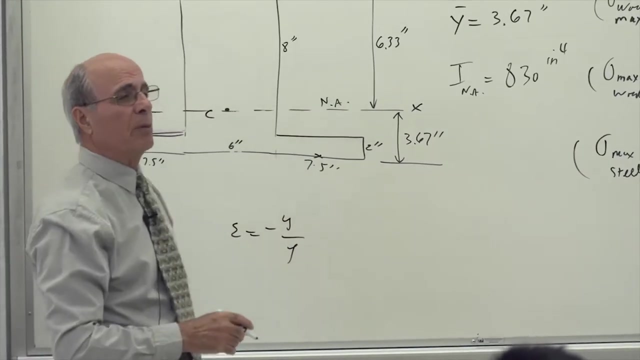 want you to understand. you cannot make a mistake here. The only thing you can change is the width, not the height. Did you make a point of that in your notes? So everybody should write that, Because you cannot change the epsilon, Epsilon was equal to minus y over rho. We cannot touch the y, Because what we can 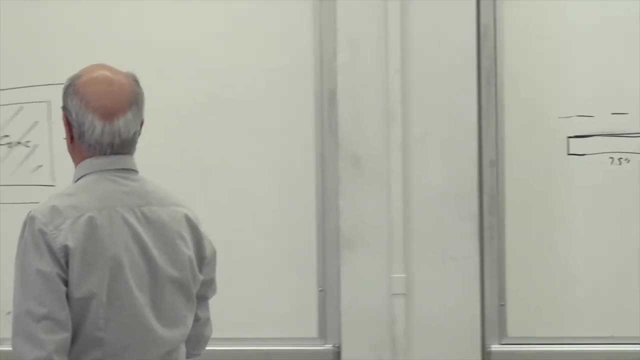 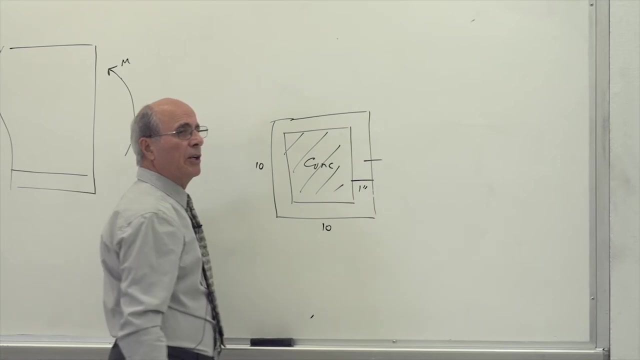 go horizontally as much as we want. Therefore, let's say that this box is 10 inches by 10 inches And let's say the thickness of one inch box. notice: if I want to increase this 10 inch, this 10 inch is going to be 10 inches by 10. 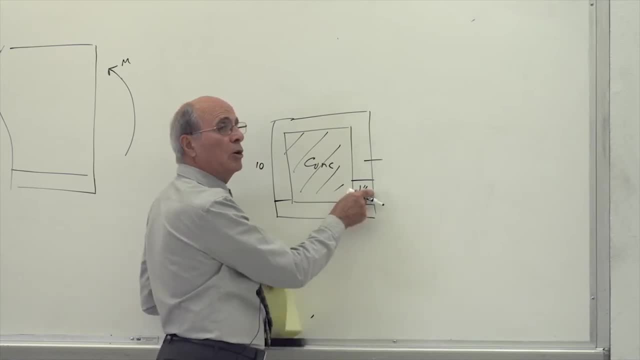 inches. This 10 inch has to be multiplied by 20,. yes, But here I only have one inch. One inch has to be multiplied by 20.. Here again I have to. So it is easier. rather than do all of that, It is easier to change the concrete into steel, Yes, or? 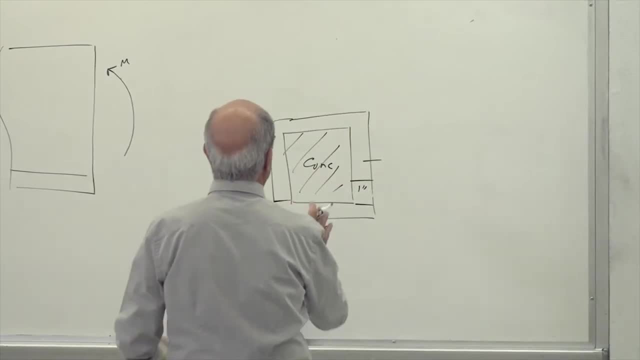 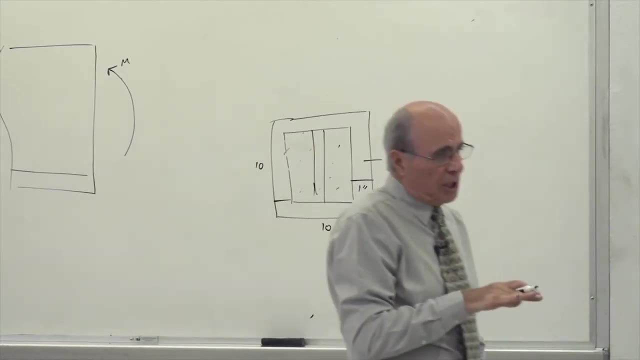 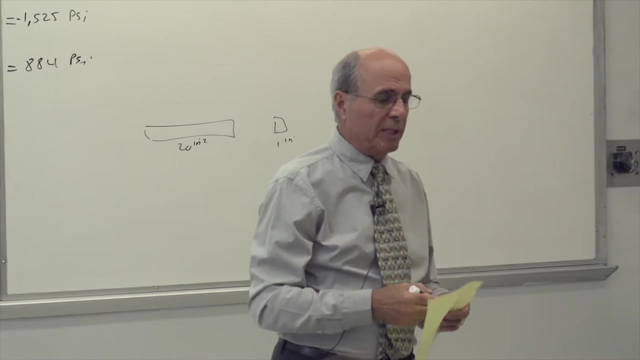 no, Because there is only one change. So in that case you shrink the concrete Depends on the ratio, Of course, because symmetrical, you put this much steel at the middle. So in each problem you decide which way is Same amount of work. At the end you end up with the same amount of work, One or 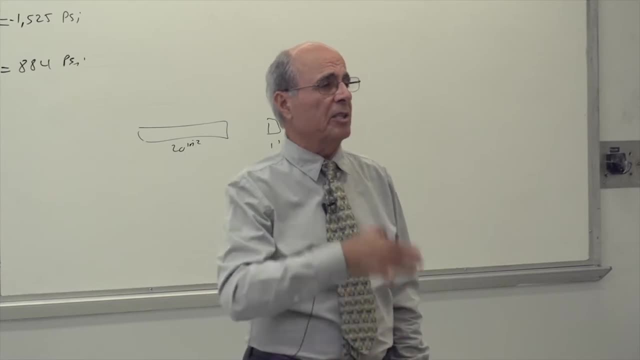 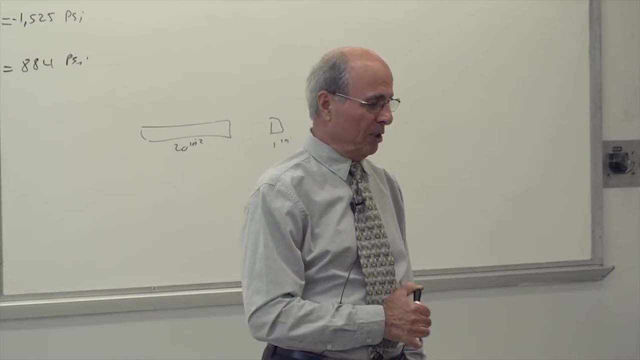 other does not have any advantage over the other. If it is a T section, it still ends up with a T section. It will be smaller or bigger. That's the only thing. 20 times bigger or 20 times smaller. Everybody understand that. However. 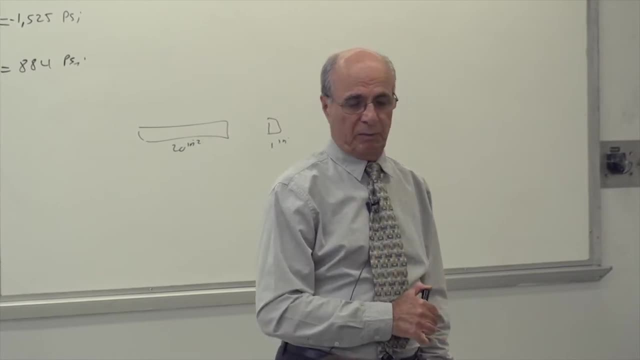 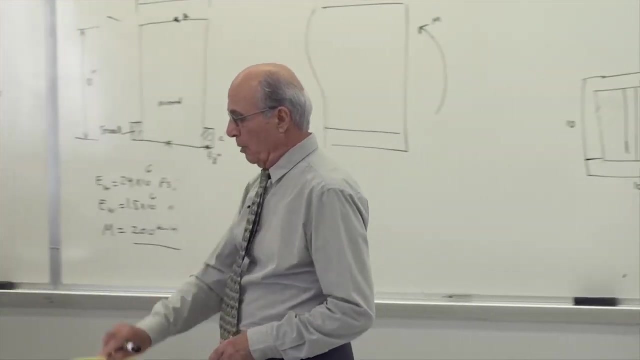 sometimes it is to your advantage to decide which method to use. Is that correct or no? Yes, Okay, So that's it. Now I have one more problem here- I'm going to put it here- which has a lot to do with your understanding of the stress. 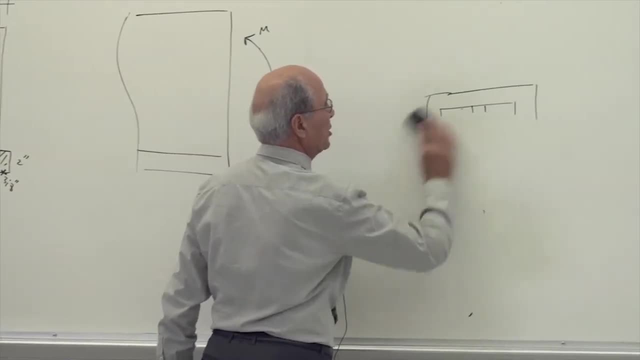 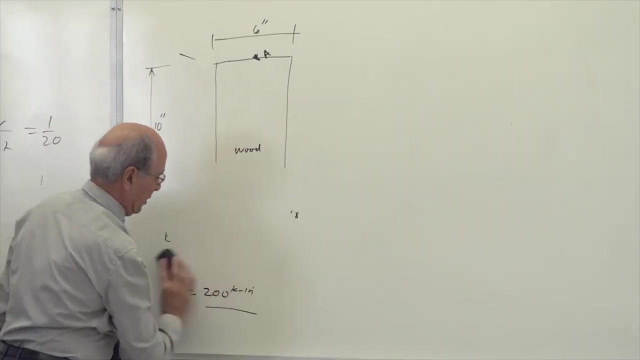 distribution. I was going to skip that, but then I decided it was a good example to discuss it with you guys. So this is not in your handout, So please write it down, So let's see what you come up with. this answer for this problem, So that's. 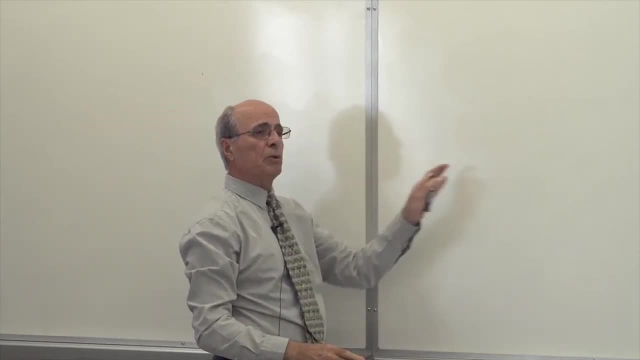 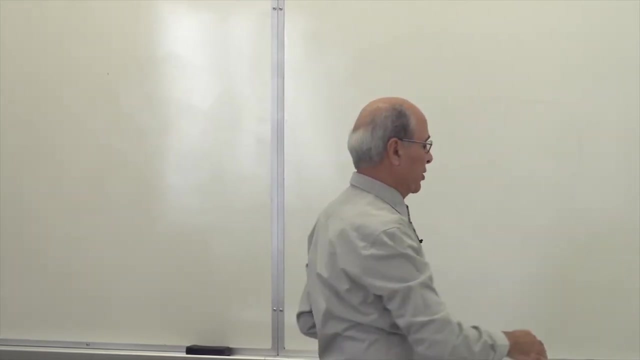 it All, the composite beam. you use this technique. It's very simple. You just change it at the beginning, You change it at the end. Don't forget to change it At the end. your stresses for the material that being changed. Now, this is: 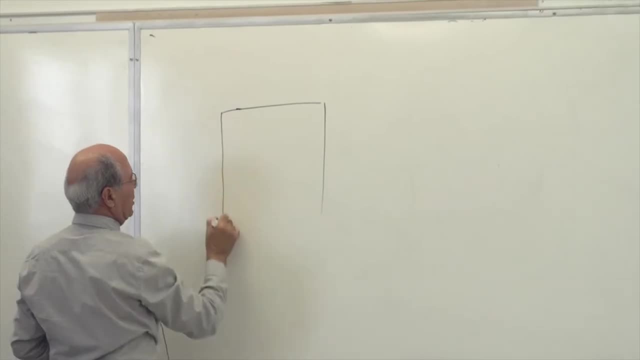 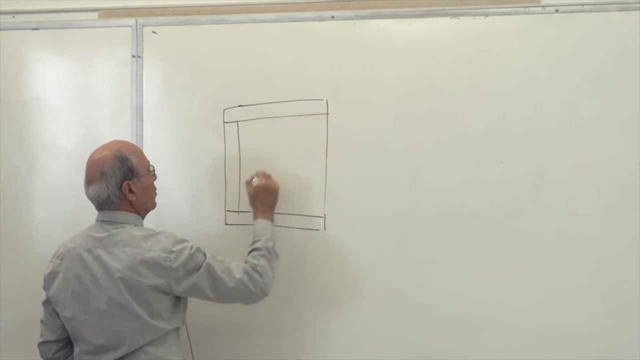 another problem. So please write it down here. This is a box. again, Let's say it is wood. So it is built like that: Four pieces of wood put together like that. This is 200 millimeter by 200 millimeter square. The thickness is 20.. Each. 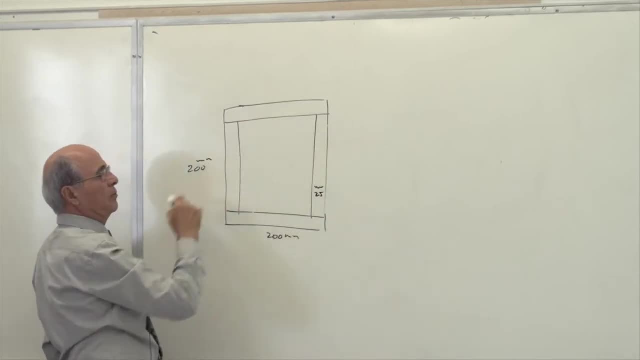 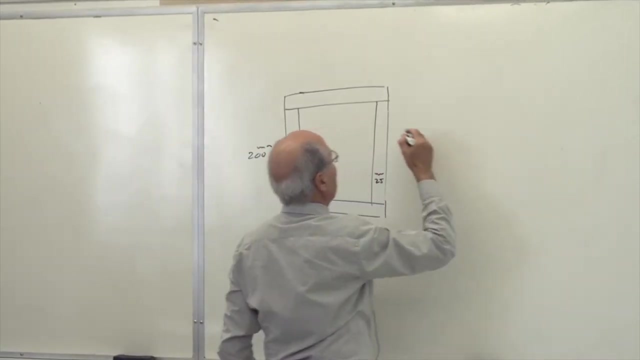 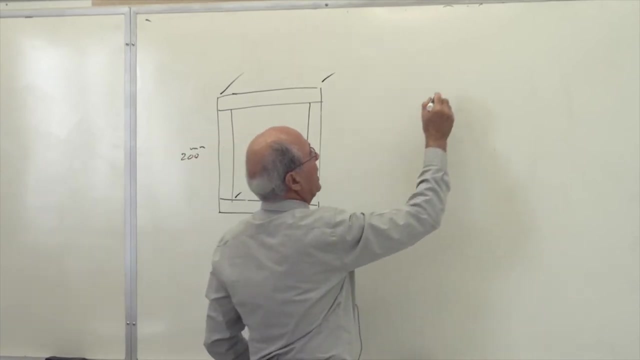 thickness is 20.. All are up: 20,, 25,, 25, 25 millimeter thickness there. And when we look at it sideway again, this is the cross section. Again, I want you to understand that this is the cross section. It's like this: It's hollow at the middle And then 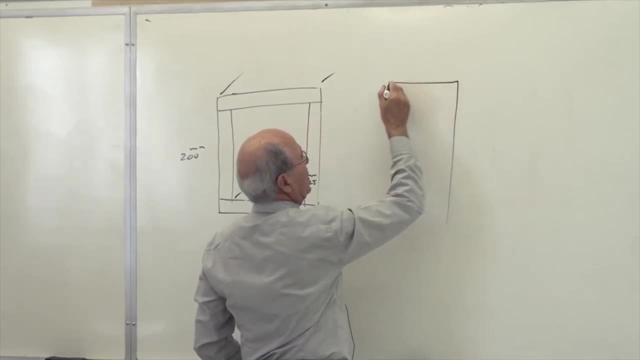 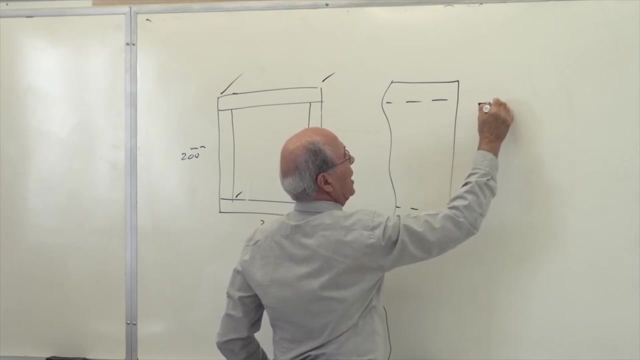 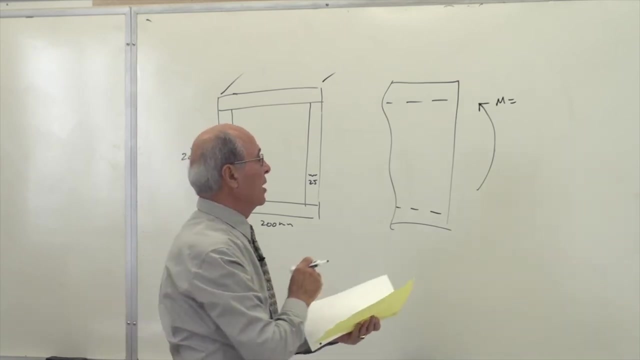 when you look at it sideway, we see this, Of course. then you see a line here, You see a line there And we have put here M equal to. I believe in this problem, we put M equal to 5,000.. 5,000 meter. I want you to answer The first. 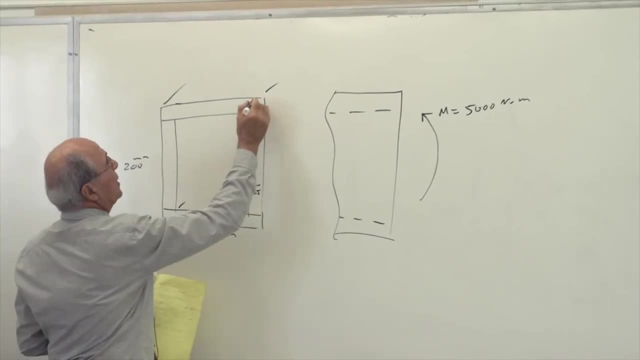 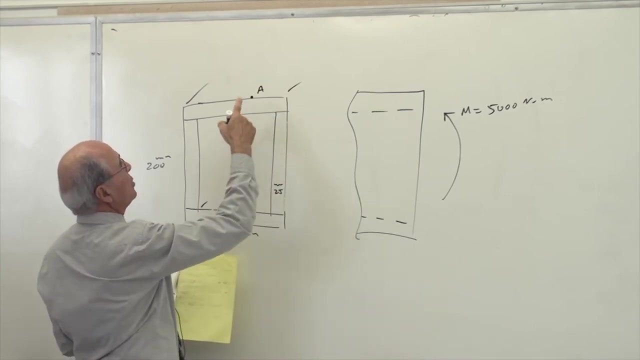 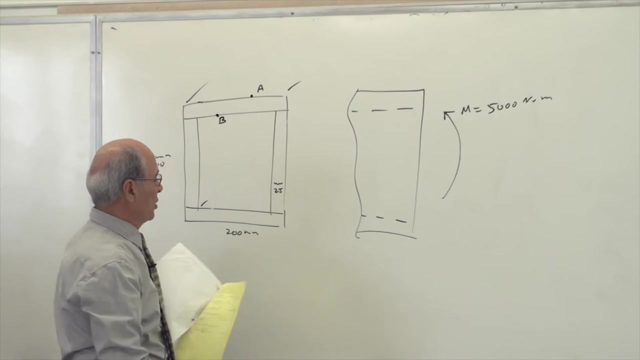 part of this question is repeat, but it just makes us to think again about the stress distribution. I want you to calculate the stress at A, Then I want you to calculate the stress at B. So these are the questions, And then I want you to. 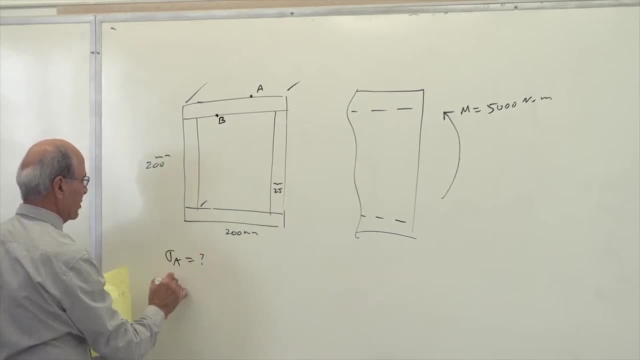 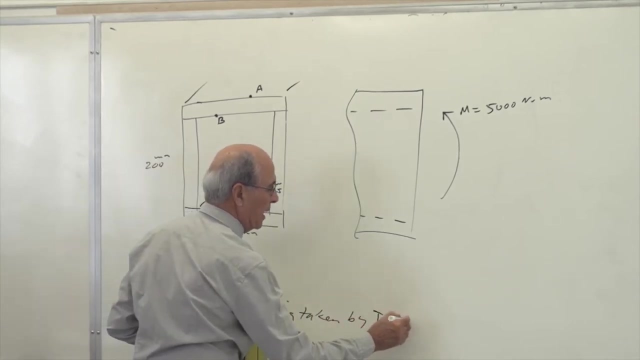 think about it. These are the question you want to answer. Sigma A very simple. Sigma B should be simple, And this is the question that I want you to think about it: What percentage of M being taken by, taken by the top and bottom? 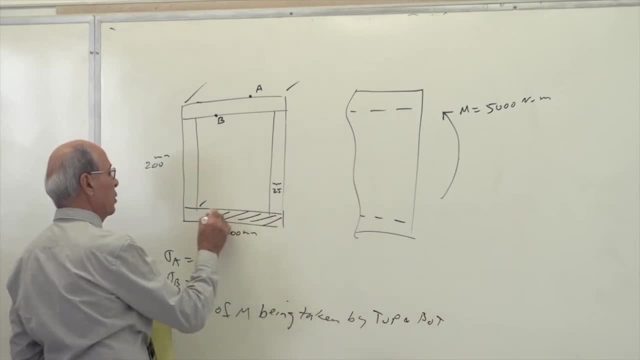 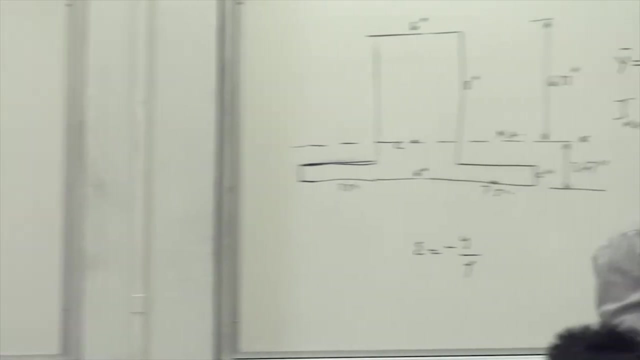 piece. So, in other words, what percentage of this moment that is taken by the that is there is taken by these two pieces? Notice, there are four pieces here. They are almost equal- not exactly They are almost equal in size, Everybody thinks at the beginning- since there are equal areas two and two. so therefore, 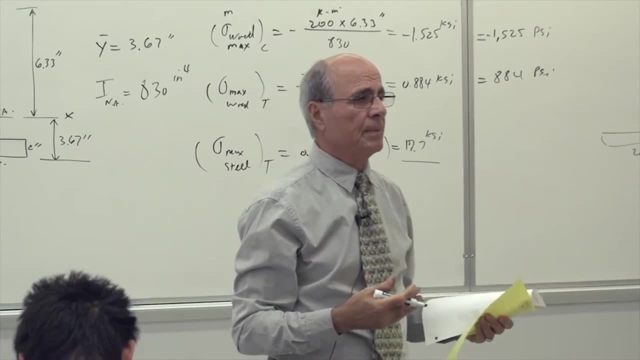 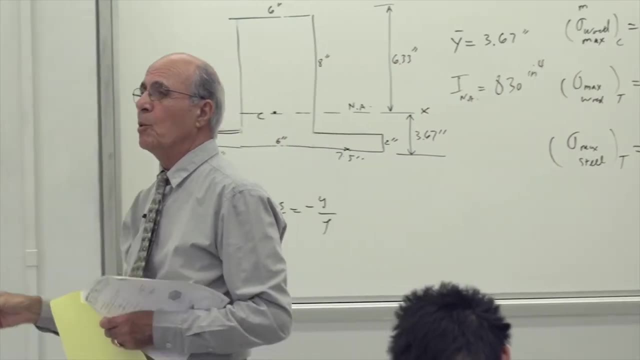 each part takes half a. Is that true or not? Do you think the top two portion that I've had- the top board and the bottom board- will take the same amount of the moment at these two? Yes or no? Before we do any calculation, No, 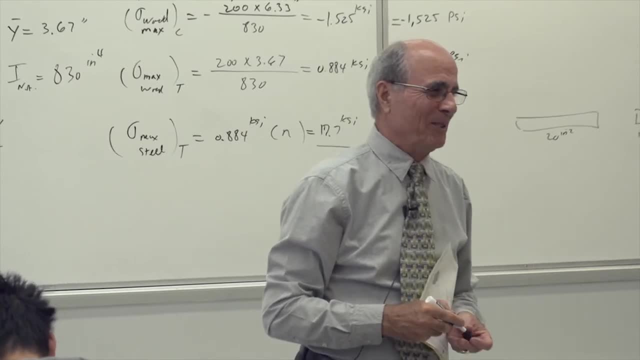 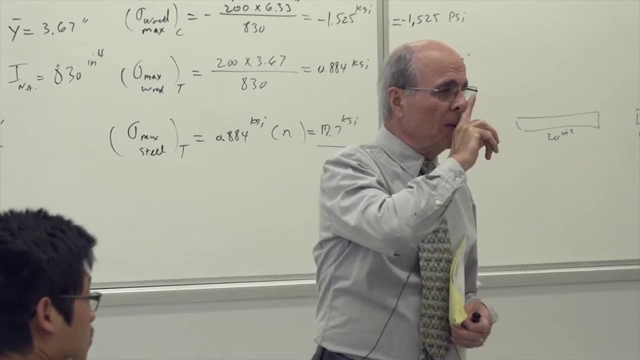 Okay, So you gave me the right answer Why. That's what we want to discuss. This is all what I think. there's one extension and one compression that's going to have a difference. No, that's not there, Of course. one part is tension, one part is compression. 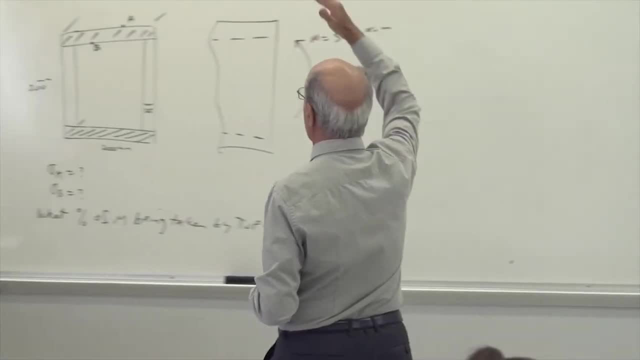 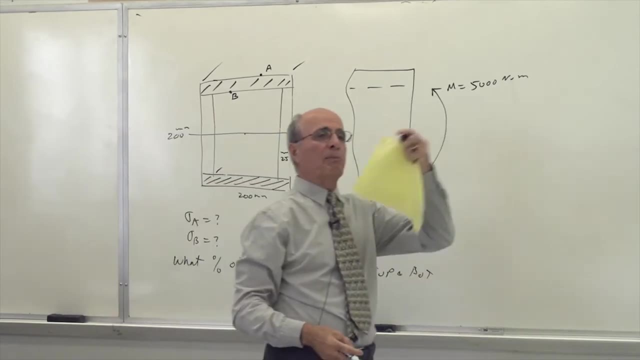 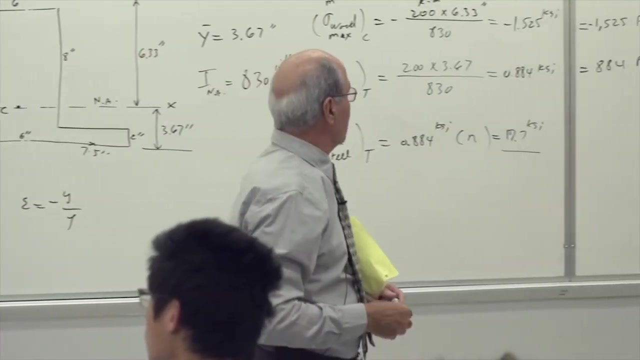 That, no, that is top part. This from here. first of all, centroid is here, Centroid. Centroid is at the middle, so that's not there. Upper part is in compression, lower part is in tension. That's not the point. Well, let's look at it later on. 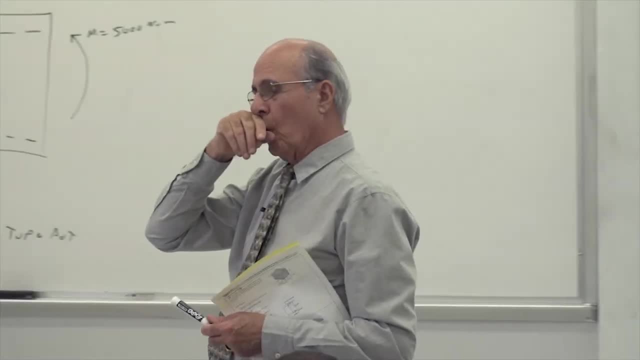 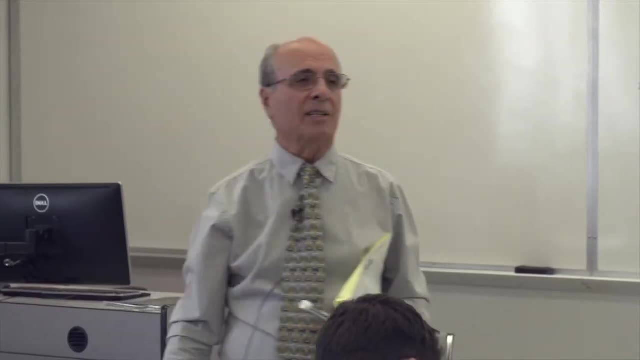 maybe as we go along? Yes, Is it because it's hollow? No, Not because it's hollow. What Is there more force at the top than the bottom? Exactly, Look at the stress distribution Guys. look at this Something. you. 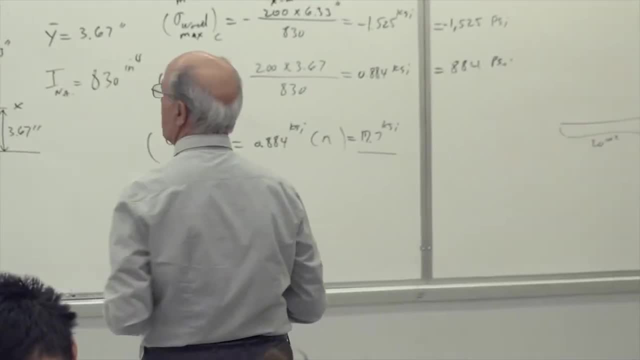 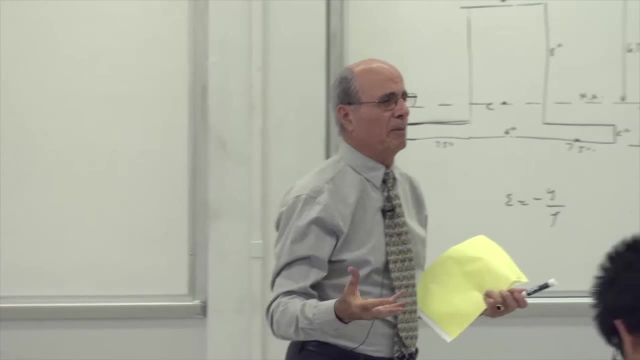 haven't looked at it, What the stress distribution looks like. What is the stress distribution? Look for the any beam. I gave it to you, Wasn't that? it was a linear? What's the stress at the center, by the way? 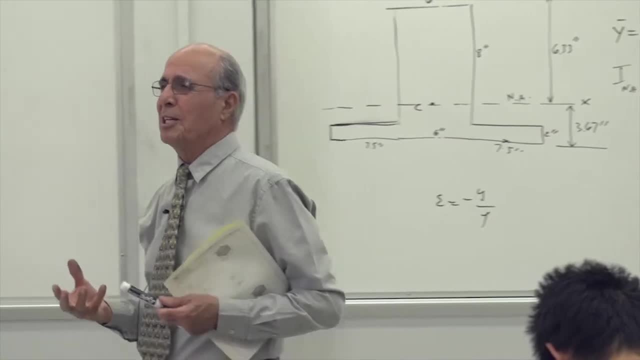 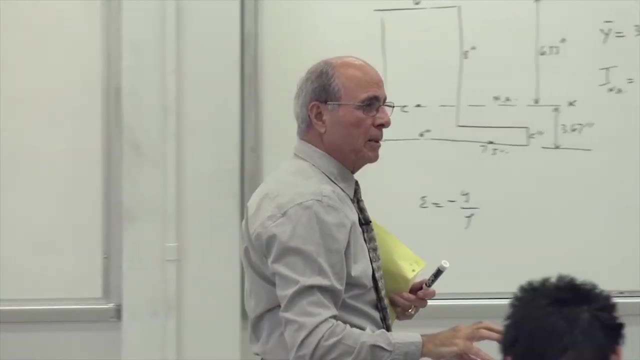 Quite frankly, you don't need any material at the center. That's why it is hollow. Is that clear? As you go up, you need more material because the stresses were concentrated on top and on the bottom. You should do the same thing for the. 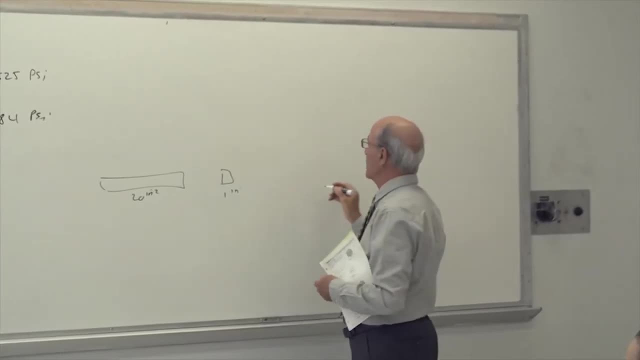 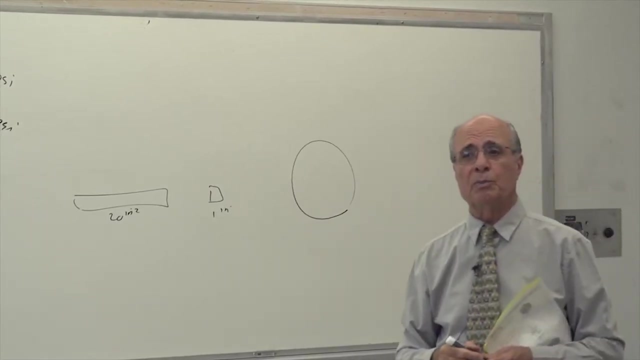 shaft. I probably didn't mention it, but it's a good time to mention it in the previous chapter. This is a shaft. yes, It is solid, It's a shaft. This is a shaft, It is solid. Do you think a shaft should be solid or should be hollow? Which one? 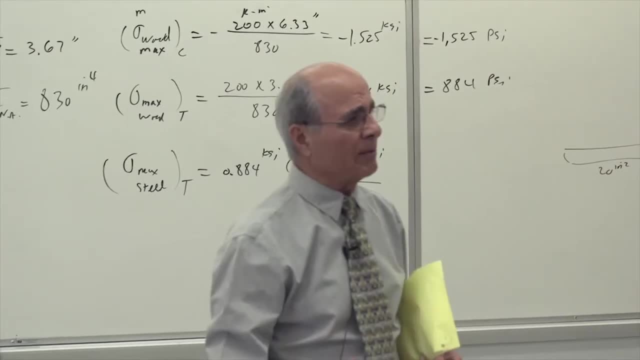 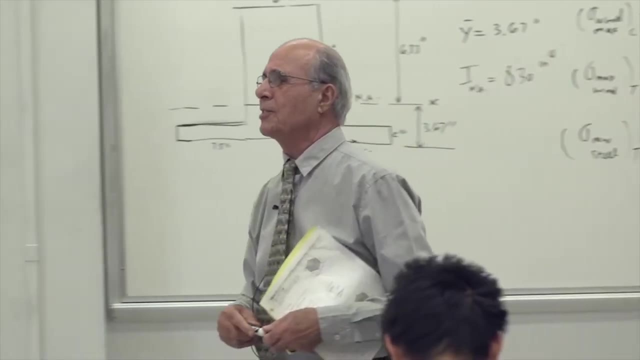 is better. What's the stress at the center of the shaft? Zero. So why do you want any material to resist it? There is nothing there to resist. Is that correct or not? Yes, So therefore the real shaft actually are hollow because the stresses 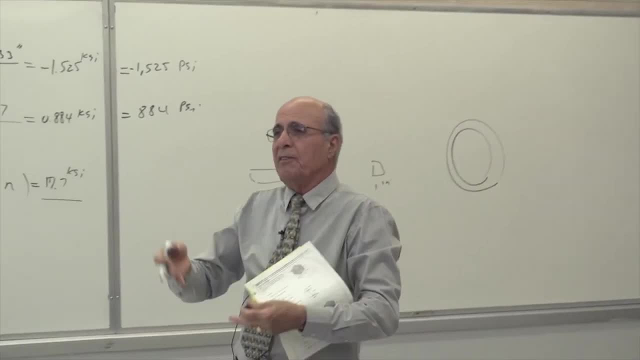 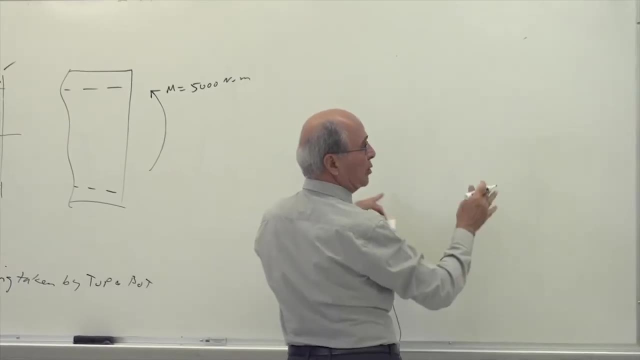 are all. maximum stresses are on the outside and we go inside. the stress become less and less. Here is the same. What is the stress at the center? It's solid. That's the same thing. guys, I'm leaving that You want to just listen, or you? 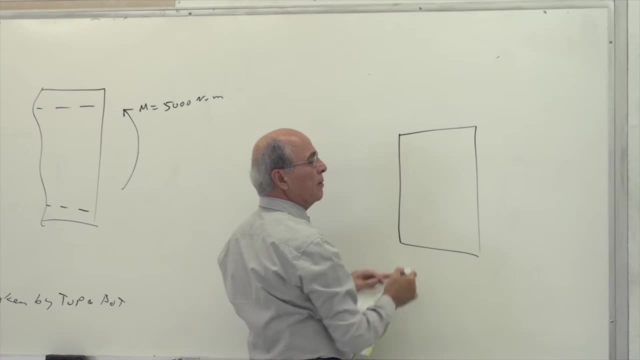 want to make a note of that. This is good for wood, because wood is less expensive, but it's not good for steel. yes or no? Because steel is very expensive and very heavy too. at the same time, You have to pay for it. yes. 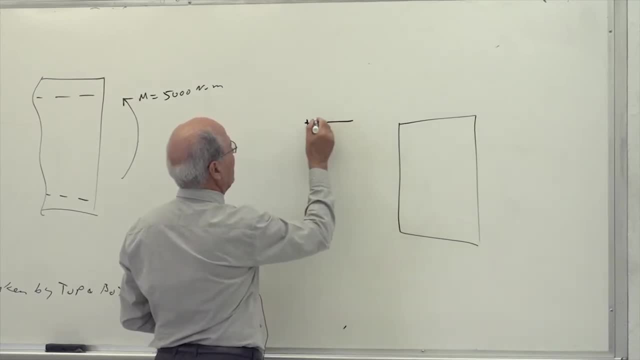 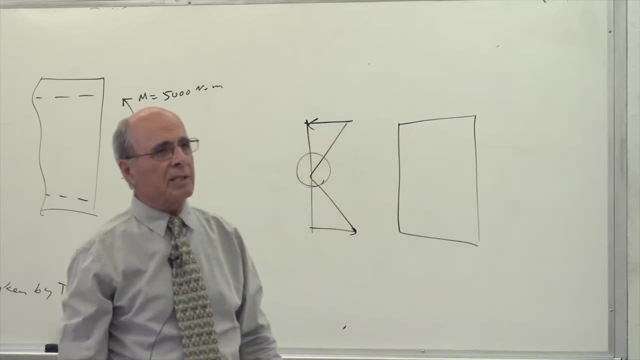 However, since the stress distribution is like this, remember that: Compression, add, That's all to do that. Look Here: there is no stress. If it is no stress, I don't need that much material. You don't need that much material, You don't. 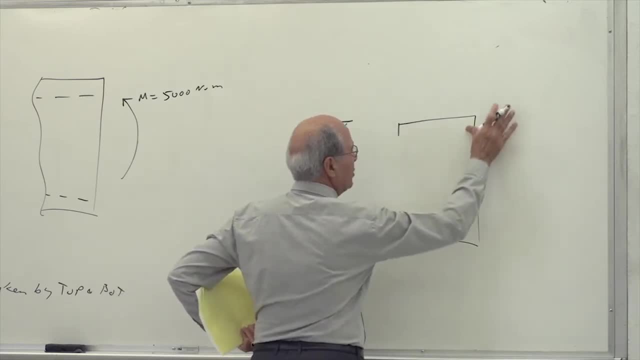 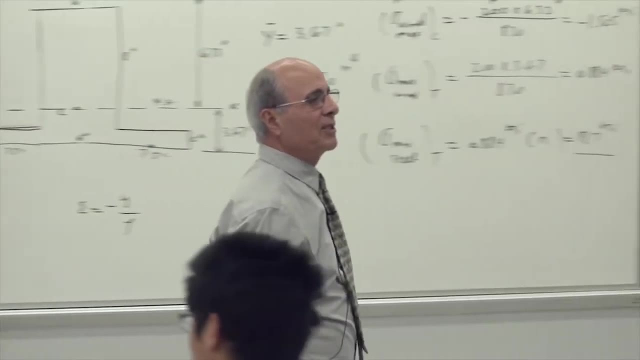 need that much material? yes, So therefore, why not cut this material to the lower? That's why it end up like that. Remember that we saw it in the static classes. yes, So all the I-beam, because you don't need any material at the. 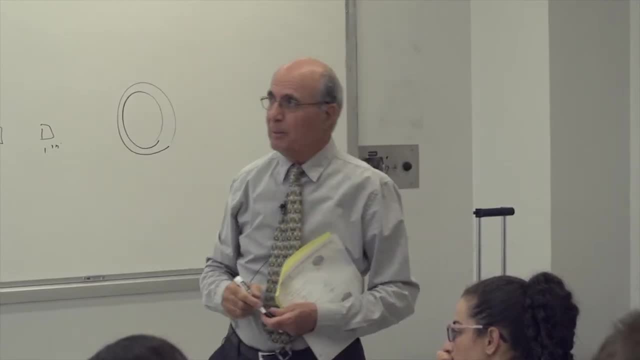 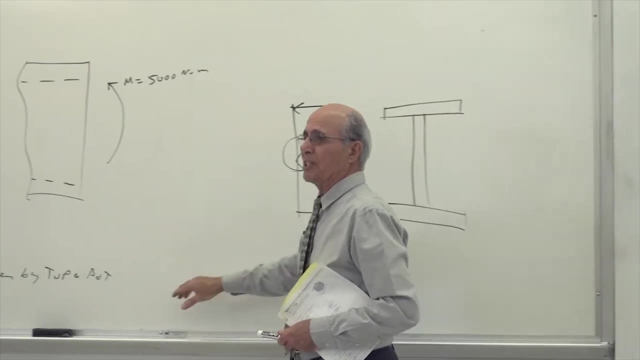 center. you need the material on top and bottom. Now that I explained that, you should have known it, because I already gave you the stress distribution, Everybody understand. This is all. This is what I'm saying. that guy, You want to become a good engineer? it's not sufficient for you just to let sigma equal. 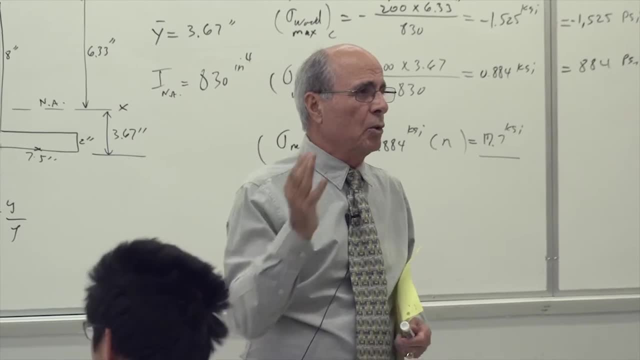 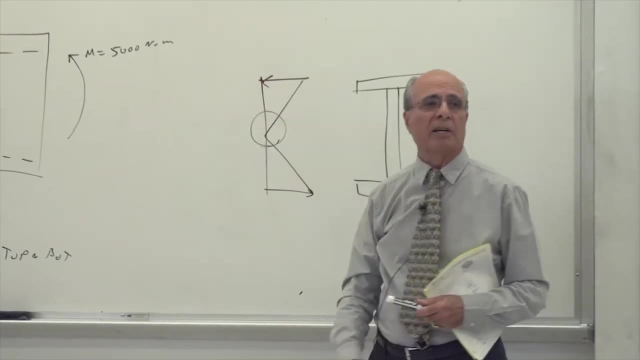 to mc over i. That doesn't do you any good, Correct? Look how much information goes through this system. This is the one you should think about all the time. Is that correct or no? That's the one I show you at the beginning through the. 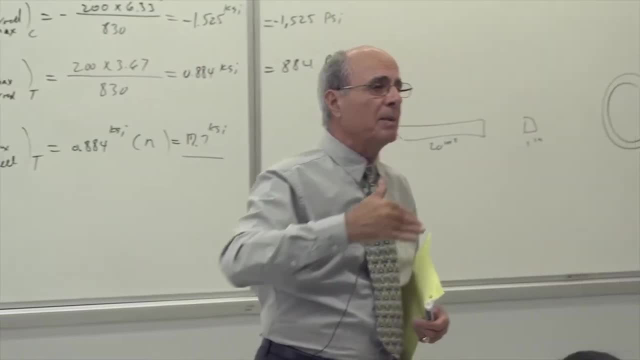 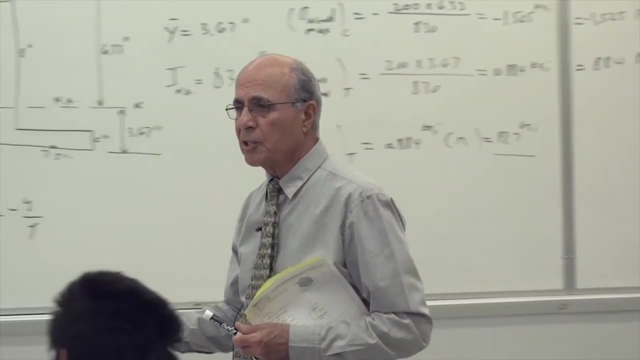 formula. I said: forget about all the formula. At least remember the stress distribution in the cross-section. That was answer to my question today. Is that understood? Yes or no? So what do you think? Do you think it's a good thing, Do you? 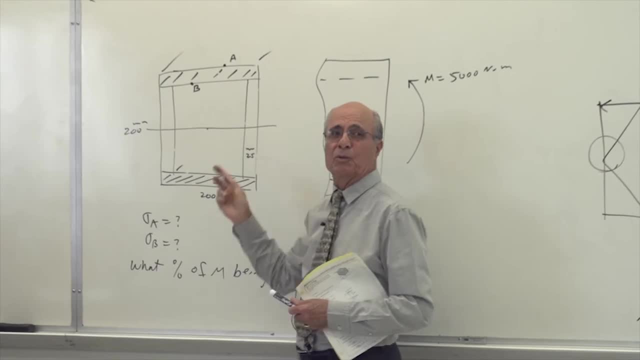 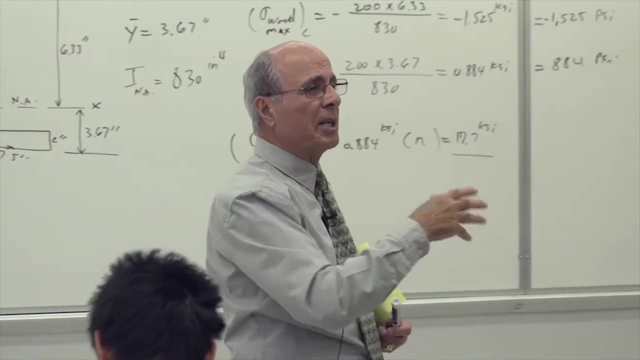 think these two are going to participate more than these two. Yes or no? Of course that's the case. That answer would be much. maybe 70% goes to the top and bottom, 30% goes to the middle because there are less stresses. there Is that. 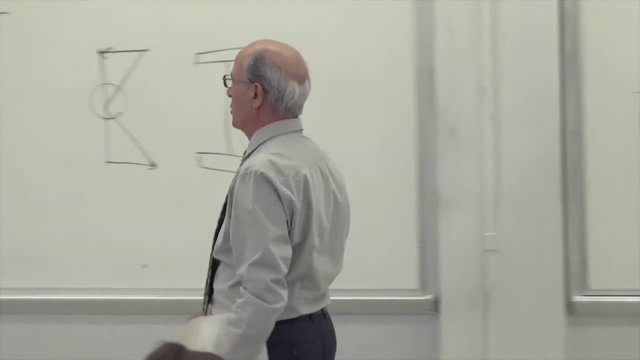 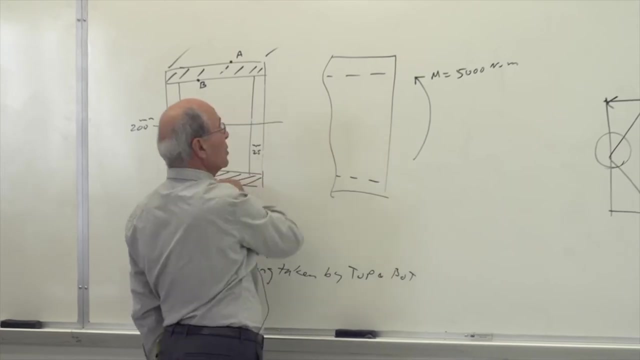 understood. So let's see whether that's the fact. That's the one. I want you to calculate. What percentage of m, which is how much m, do we have? 5,000.. Area-wise, let's assume they are equal. They are not going to get the same amount of the. 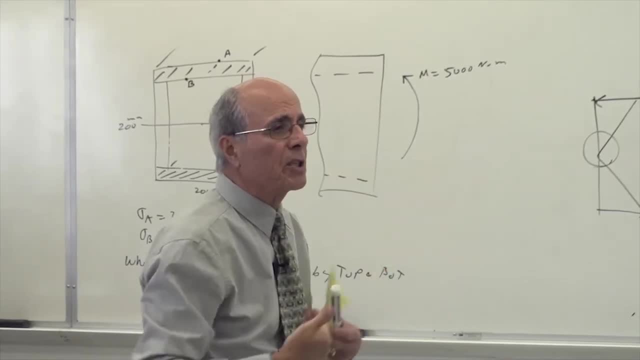 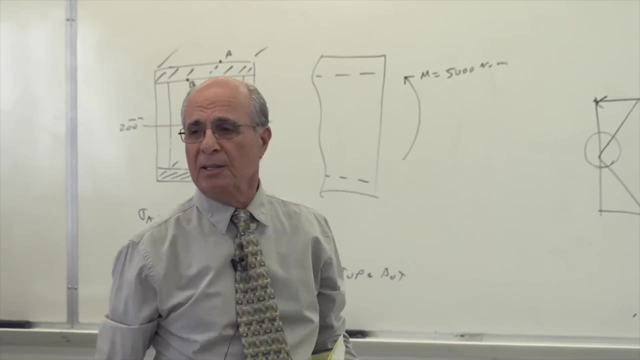 forces, as you were explaining. The force is going in, The force is coming out. The force on top is much larger than the forces at the mid. Actually, on the centroid, this force is zero. Is that correct or not? Force zero, epsilon zero, sigma zero. Nevertheless, let's finish. 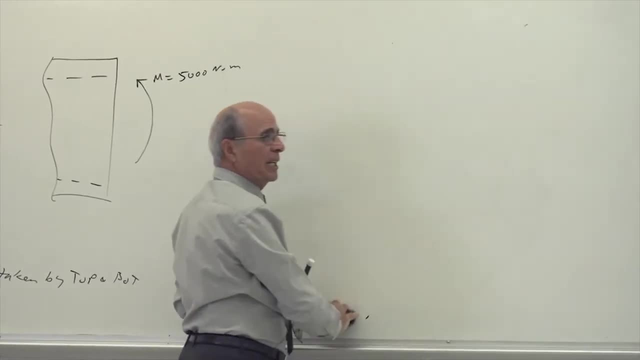 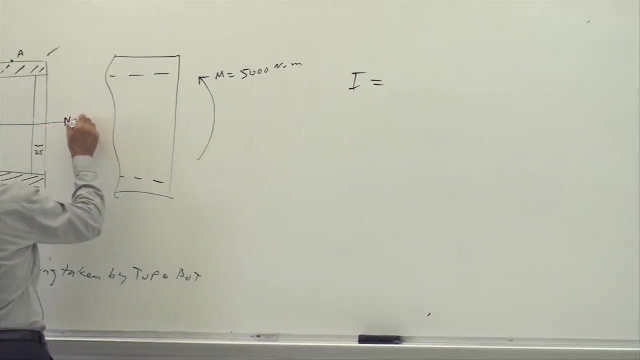 this problem. First of all, centroid is at the middle. Everybody agree This is symmetrical, yes, Next, you need to calculate the value of i with respect to neutral axis. This is the centroid and this is the neutral axis. Is this? 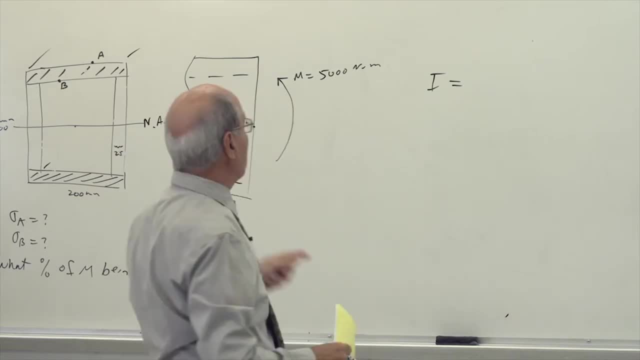 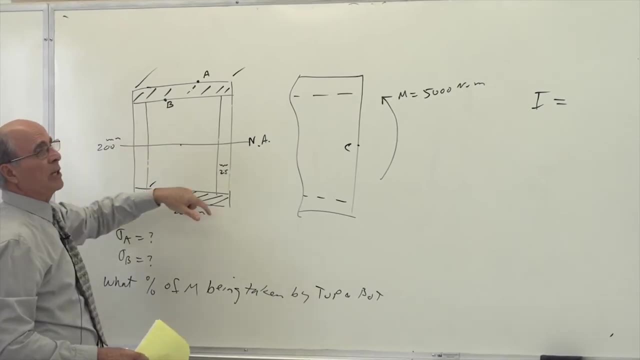 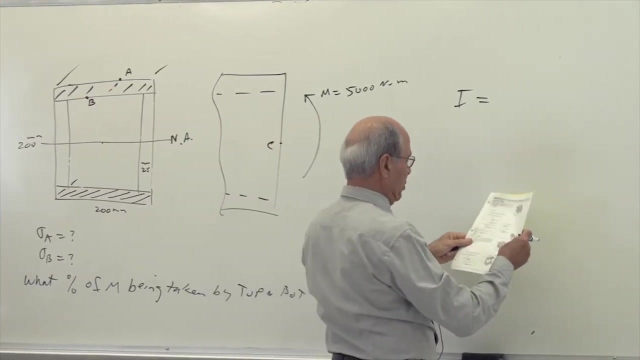 that correct or not? Which, again, you can do: parallel axis theory. For this one, actually, I'll show you another method, because you already know that, probably, And that is, since this is symmetrical, you can go i of outside minus i of inside. Don't break it into four pieces, It is easier. Nevertheless, that is your. 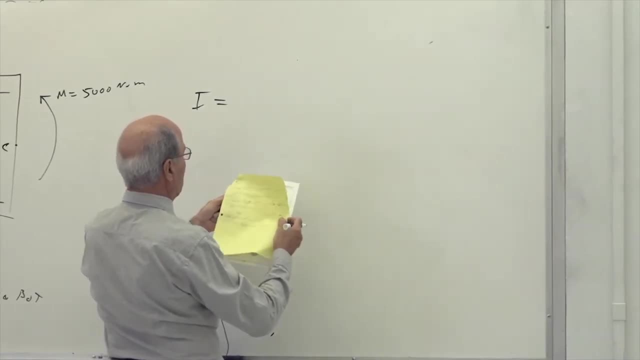 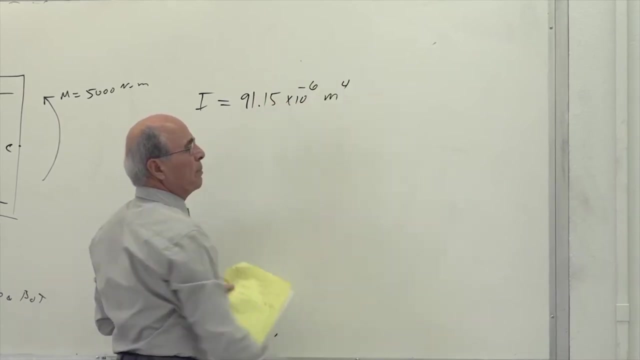 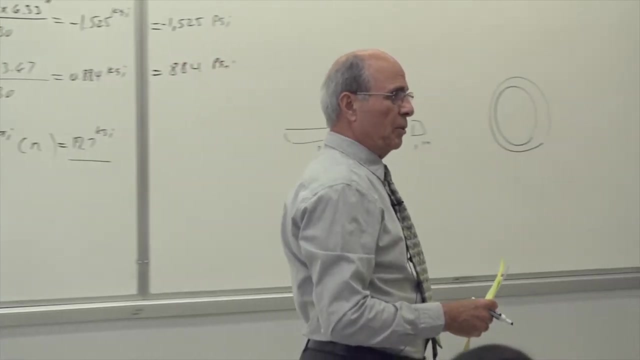 job to do, I'm not going to mention that. And i end up to be equal to 91.15 times 10, to the power of minus 6 meter, to the power of 4.. Remember last time I was showing you how to calculate it in millimeter. then convert it into meter by: 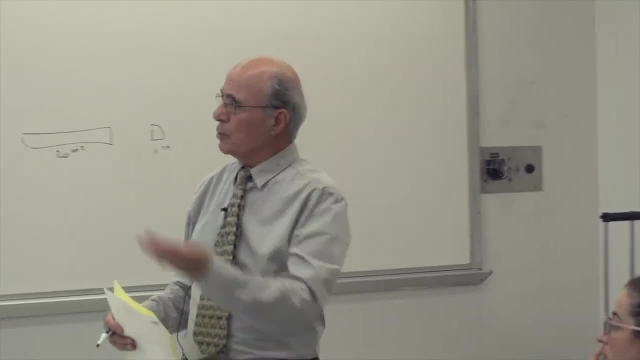 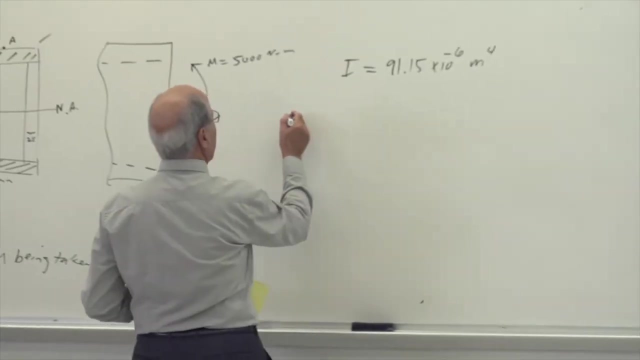 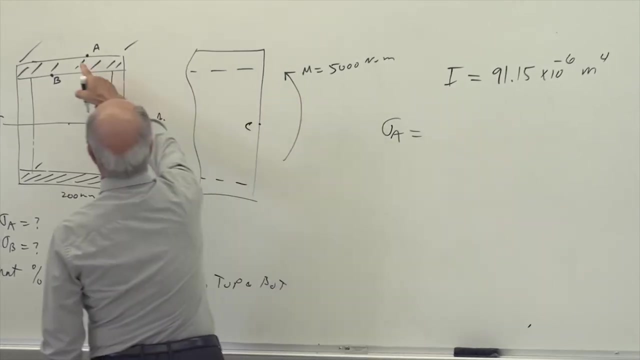 going from plus 6 to minus 6.. So that's the answer. Everybody should come up with that. Is that very simple? Then we want to calculate sigma a. These are very simple. Sigma a will be in compression mode, yes or no? Correct, This is. 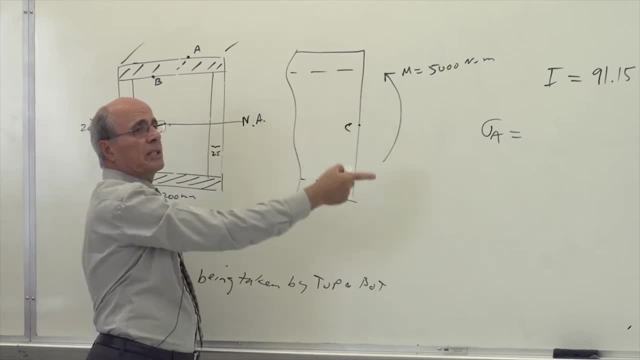 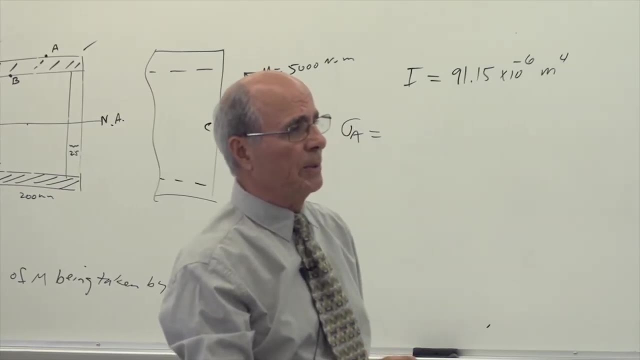 compression, compression, tension and tension. Look how the moment is there. If I change the direction of the moment, then everything changes. If I change the direction of the moment, everything changes. This all depends on the direction of the moment. The way I have given each problem, it will be given to you. So. 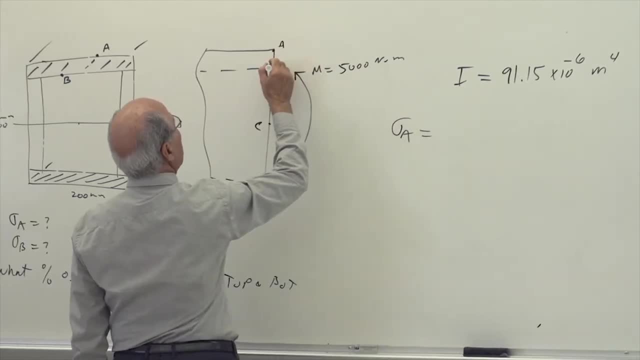 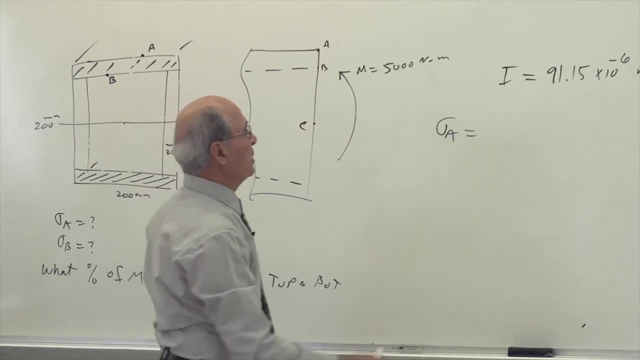 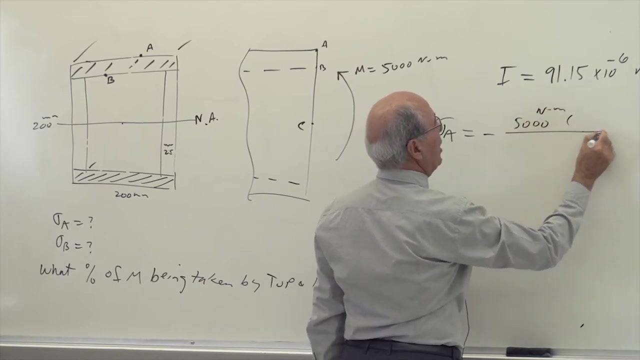 what's sigma a here? This is level of a, This is level of b. Is that correct or no? So at a we have compression and compression Correct As a and b, both of them Minus. so you put minus there 5000 Newton meter multiplied by what? 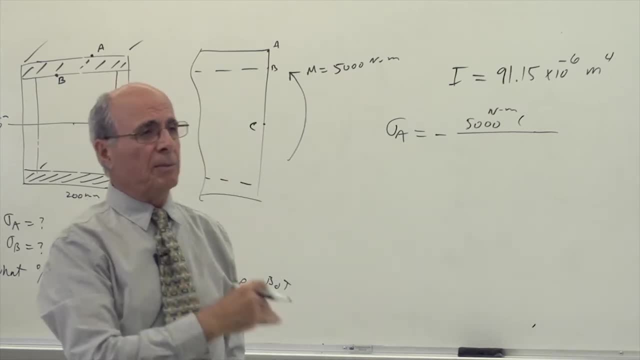 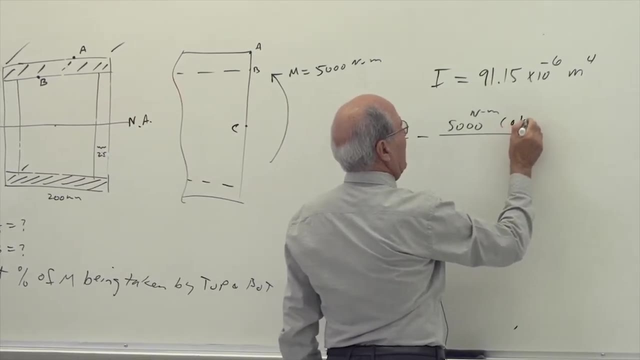 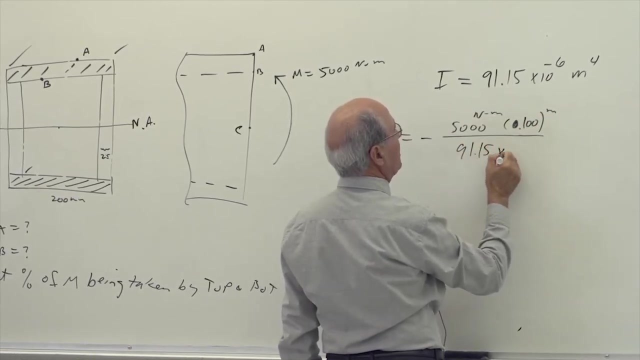 Multiplied by The cc is measured from centimeter, So you put minus there. So I'm drawing today top, which is 100 millimeter, so 0.1 meter Divided by i, which is 91.15 times 10. to the power of minus. This repeat, I said: keep this for. 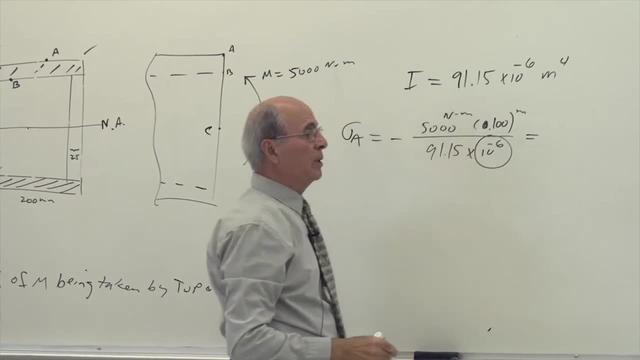 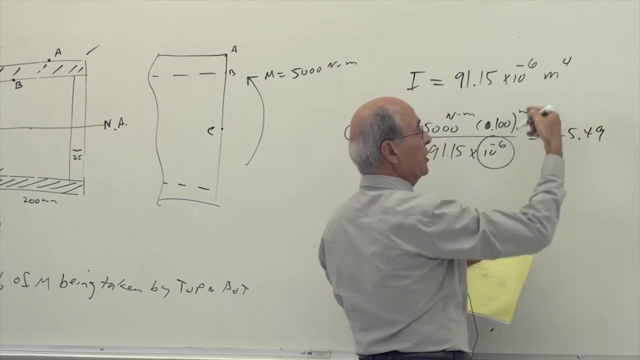 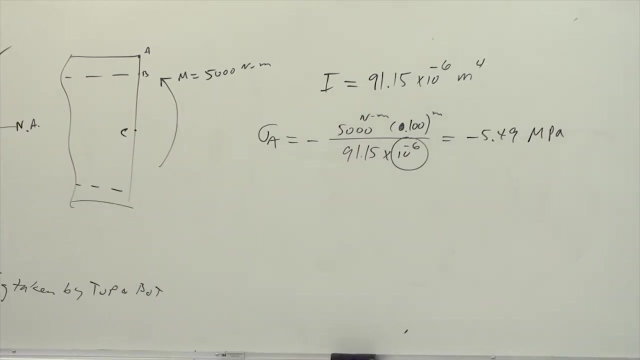 your mega. Multiplied this 3 and divide by this 2, divided by that one, So you get there minus 5.49.. This goes to the numerator and become your mega. So it becomes that many mega pascal, or that many times 10 to the power of 6.. Correct. 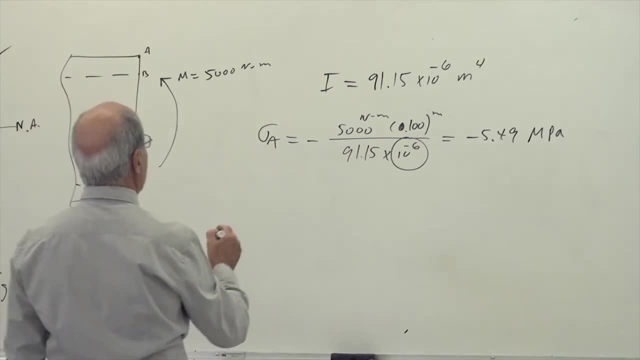 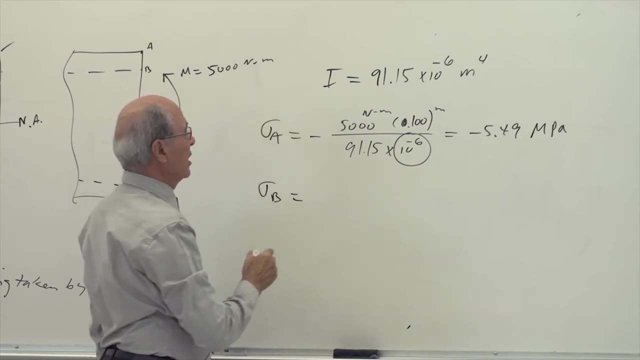 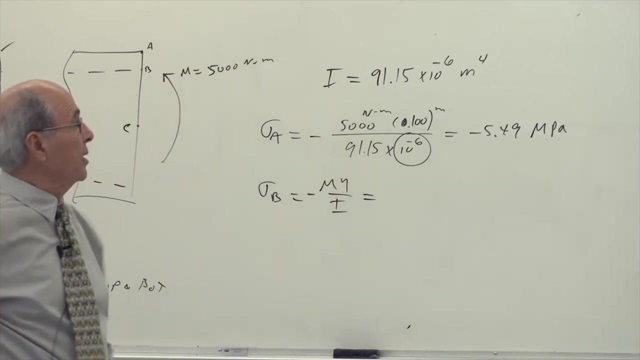 Newton per meter squared. Now we can calculate sigma b For the sigma b. obviously I cannot use mc over i. I have to use my over i Remember that. So therefore it is m. It is negative My over i. Is that correct or no? Yes, i is. 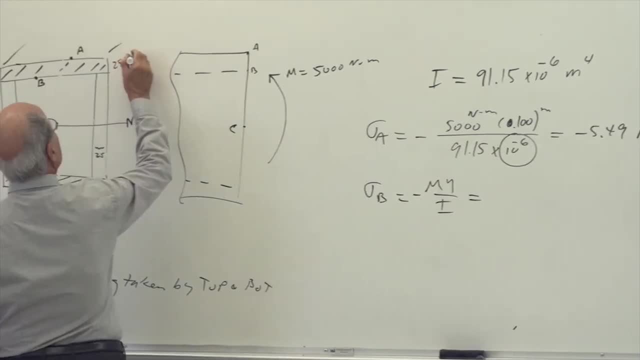 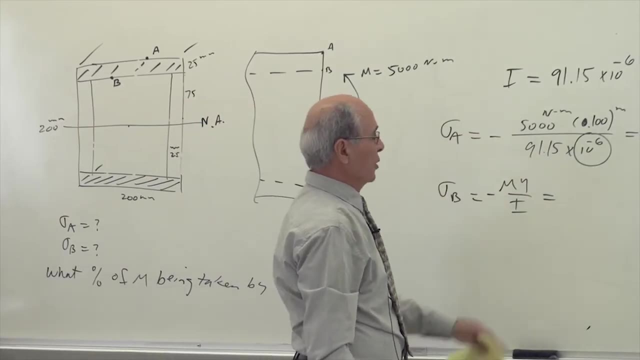 75, because this is 25 millimeter. This is 75. This is 75. This is negative. This is 75 millimeter. This is this. distance from here to here is 75 millimeter. Again, I can use the ratio if I want. So if in the solution manual they take this: 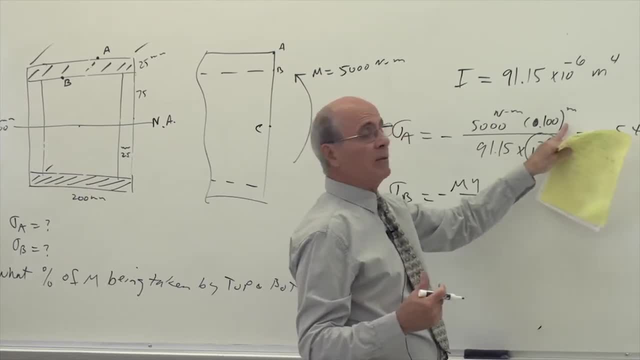 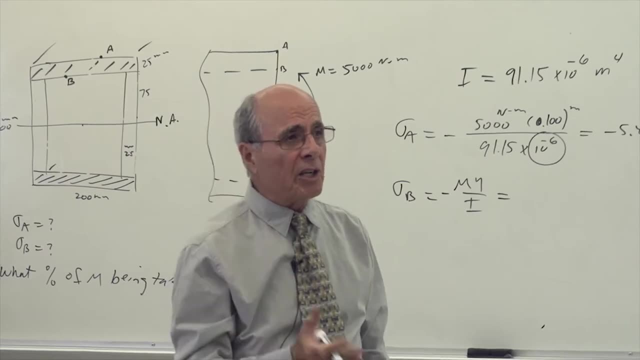 number. they multiply it by 75 millimeter divided by 100, because they are using the triangle rule. Everybody understand that, Because they're lined, therefore you can use the ratio. Is that correct or not? Yes, Some people do not. I have. 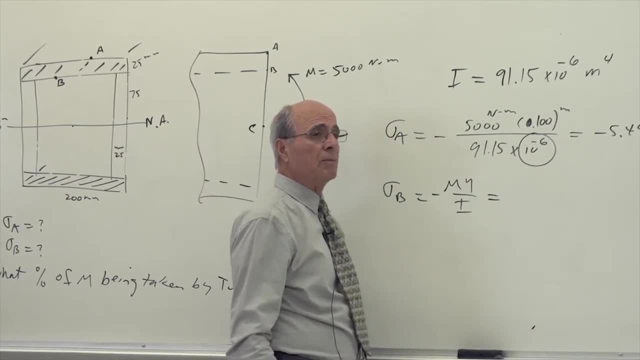 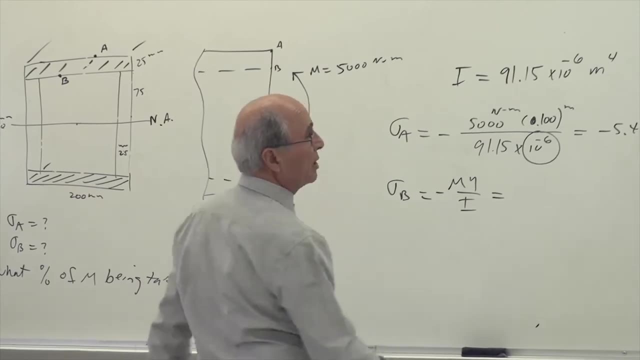 seen even the student in ME 219 come to me. They see that in the solution manual. They don't understand. So what did they come and ask me: What is this? We don't know what's coming. You're coming because the stress distribution is I. 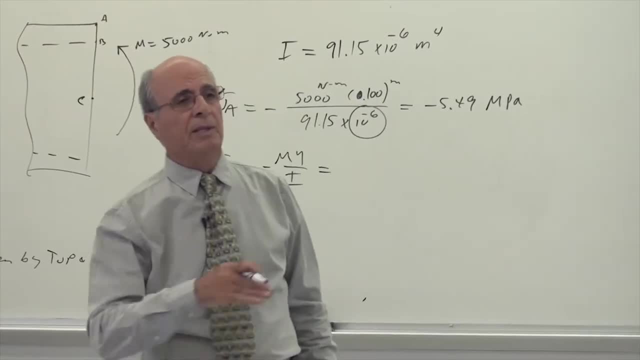 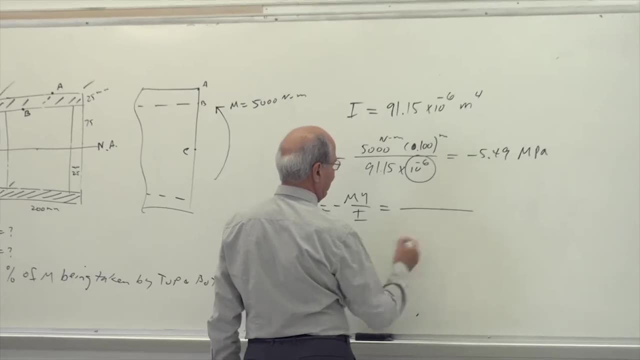 erase it there somewhere. I'll show you. The stress distribution is linear. Is that correct or no? Anyhow, Or you can recalculate that. Recalculating is more work, but that's it. So that's 5,000 times .075.. That's the only number is. 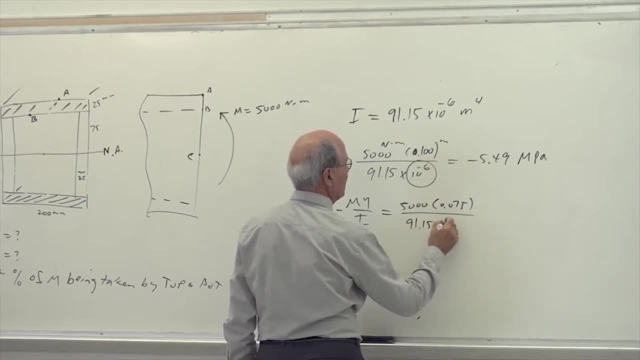 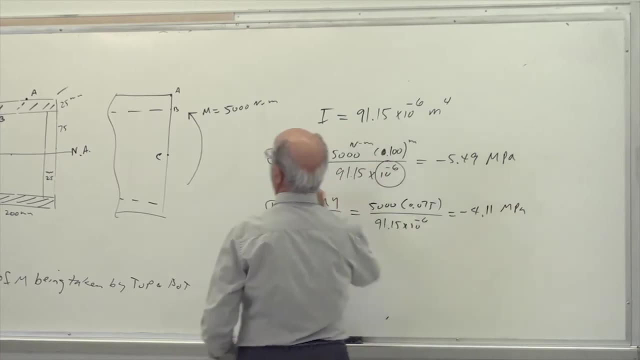 changing. Remember, divided by 91.5 times 10 to the power, which become minus 4.75.. So that's .11 mega Pascal. So I have calculated the stress at point A and B. part A and part B. answer Which, as I said, this was repeat. Is that correct or? 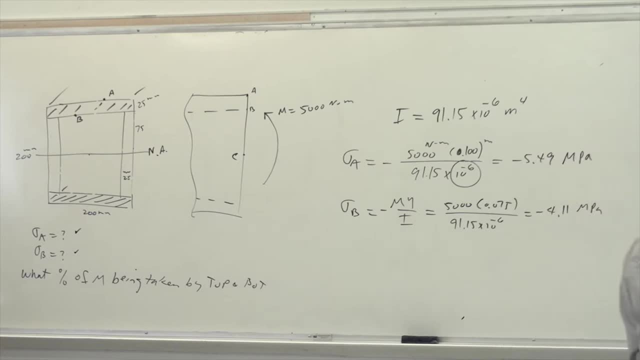 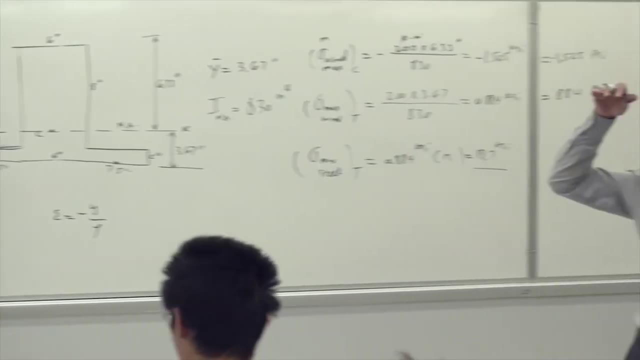 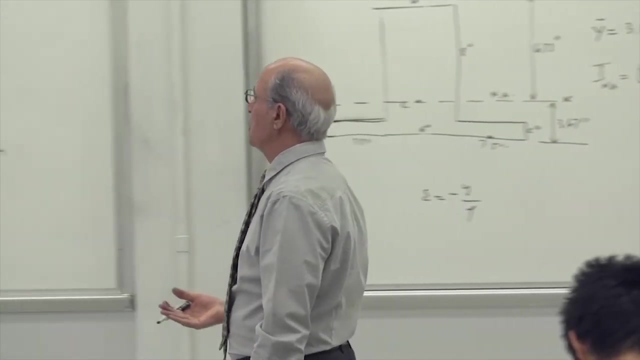 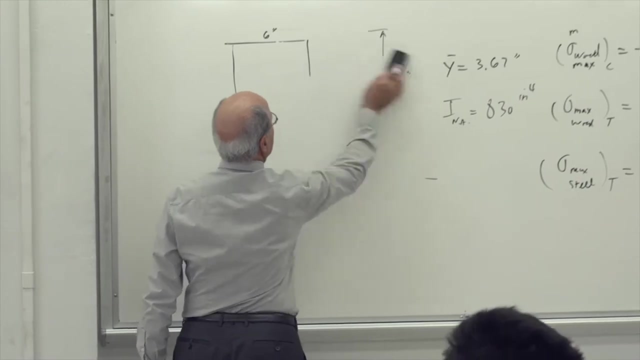 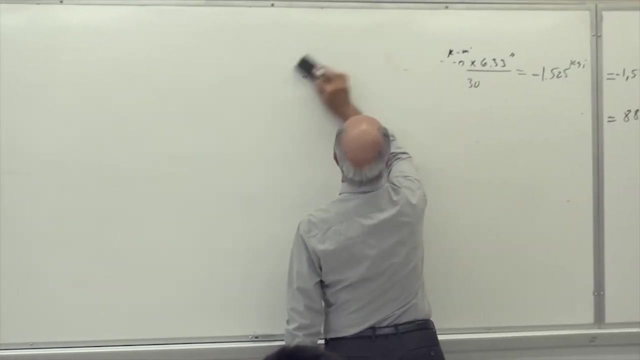 not. How do I calculate part C? What percentage of this moment being taken by the top and bottom? Obviously, I have to calculate forces going in and forces coming out, So I need again the stress distribution. Everybody see what I'm talking about, So I'm going to do it here. So this is what we are talking about. 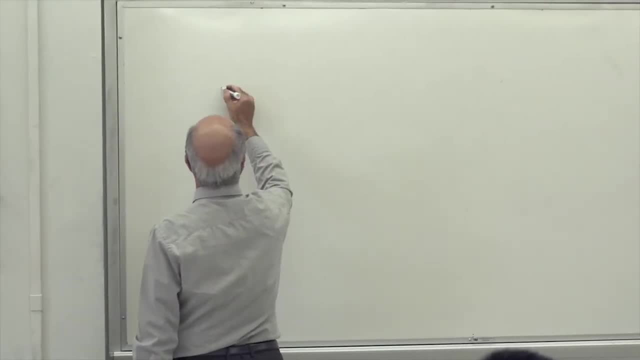 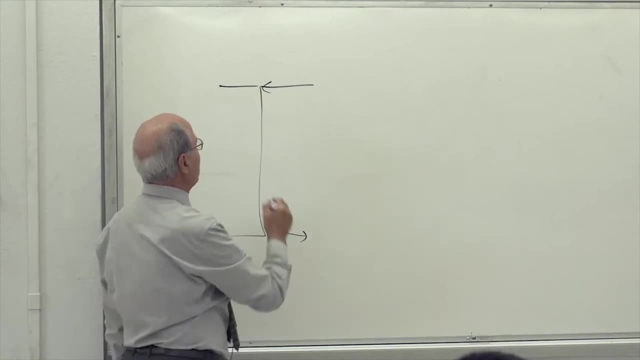 OK, In general, in any beam doesn't make any difference Of any cross section. when you have a moment like that, here is compression, Here is tension. I have drawn that many, many times just to be sure, So this is a very important point. 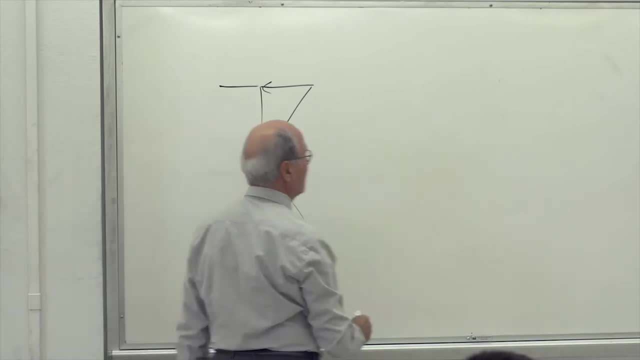 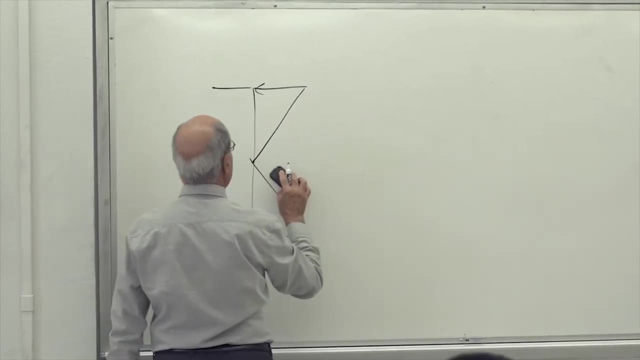 To bring to your attention Yes or no For our problem. now this changes a little bit. It's hollow or doesn't hollow doesn't make any difference, But all we want to understand is the following: I don't need this because this is my lower and 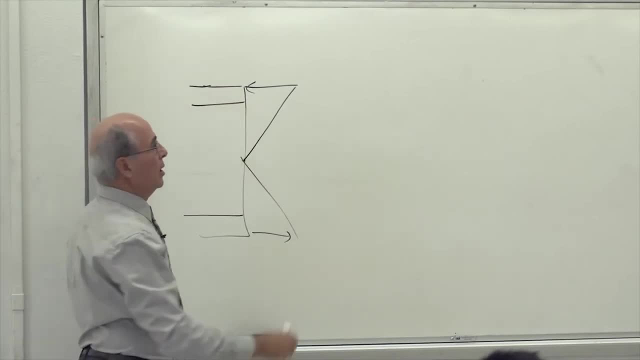 this is the upper board. This is the side view again. Yes, So we already calculated that and we already calculated that. Erase this part. You don't need that one. Is that what we are coming up? This was 5.49.. So this is the side view. 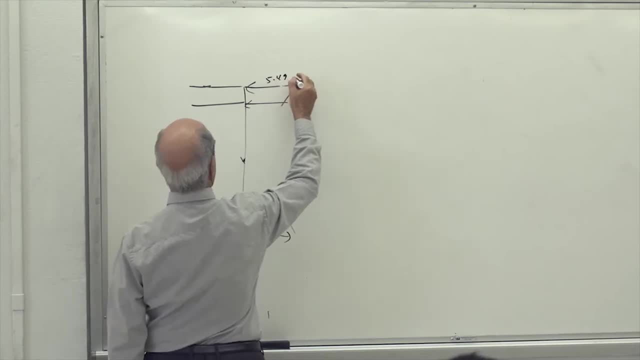 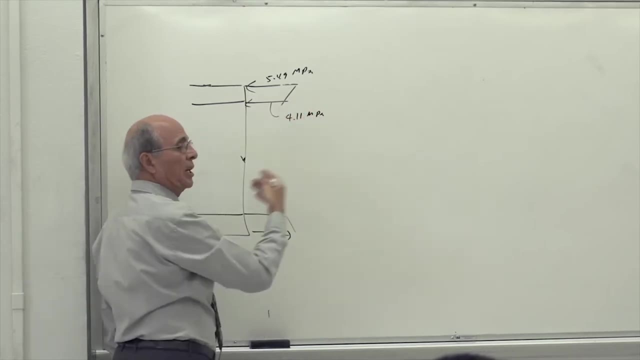 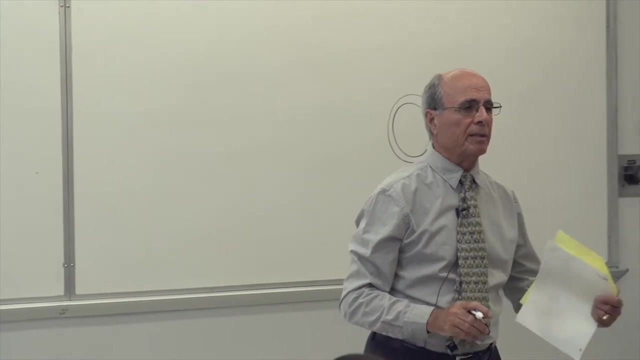 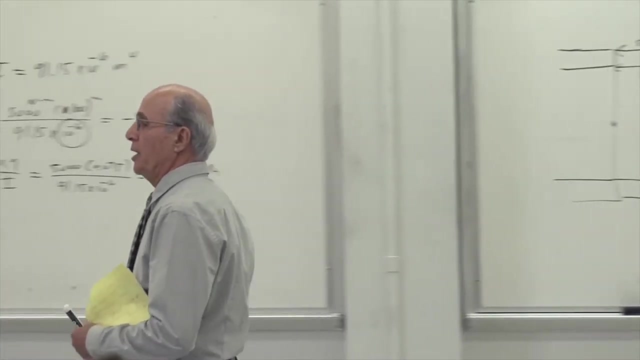 5.49 megapascal And this was 4.11 megapascal. Stress or force is going in in compression format, Yes or no? Can I calculate the amount of force there? Yes, How? Come on guys? This is lecture one, AB 218.. Force sigma equal to four. 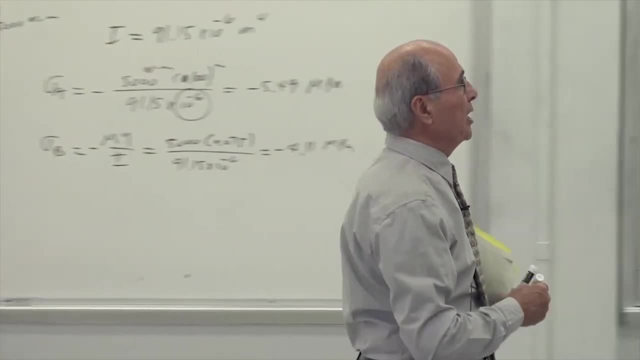 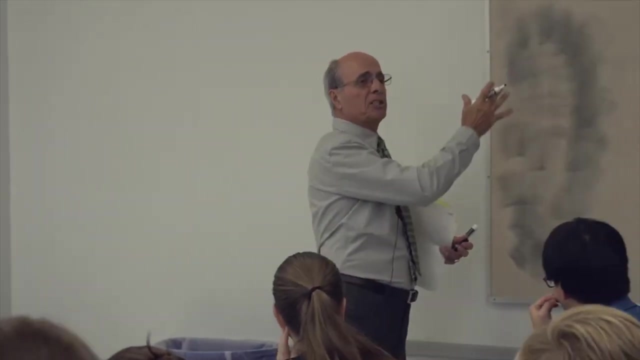 over area. It's very simple, guys: Any time you have that, you have like a pressure, Your pressure comes here. Then you want to calculate the force. You multiply this pressure by the area. Yes or no, Sigma is the same thing, because 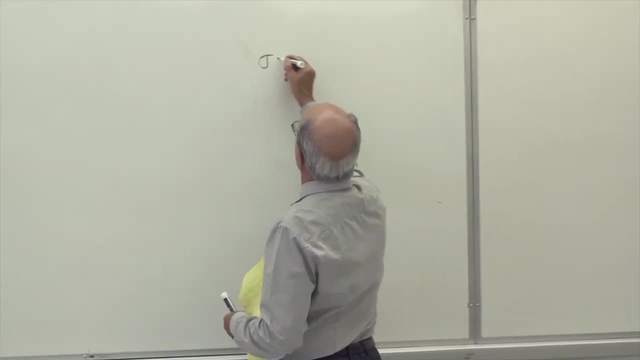 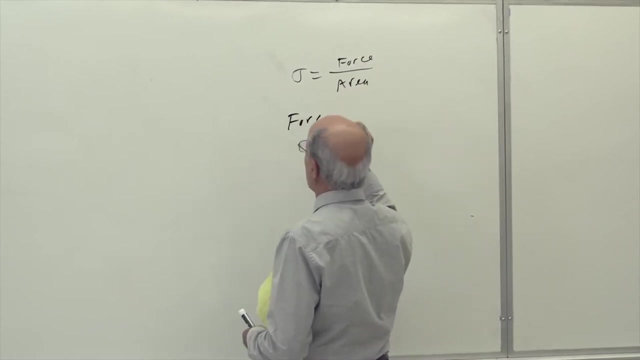 lecture, one lesson one: Sigma equal to force over area, Yes or no? So if I want the force- actually usually you have the force- then you do that- It become equal to sigma times Area. The only problem is: is sigma here is constant or is a variable? If sigma 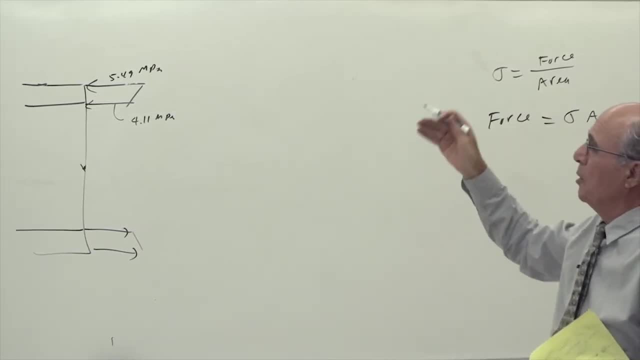 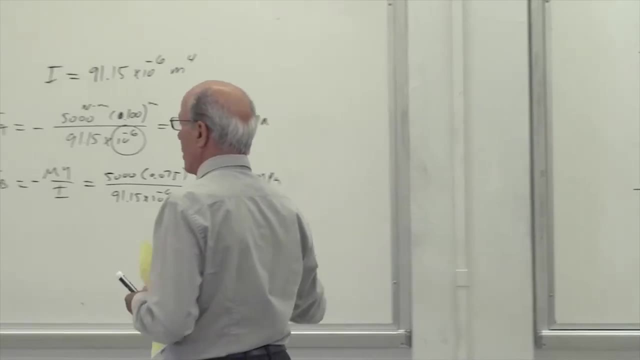 was constant. all I have to do could take that sigma, multiply it by that area. That becomes the amount of force going in. Everybody see what I'm talking about. So the result of that one is a force. I'm showing the force in color, guys, So it. 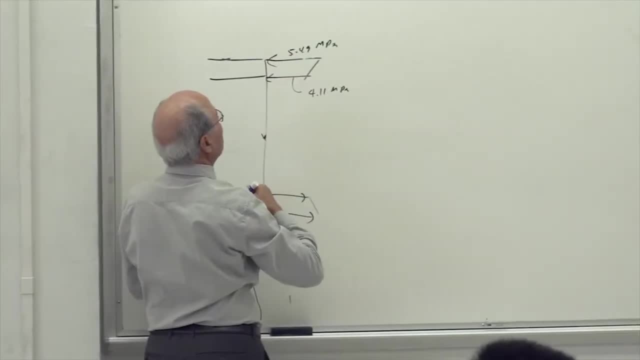 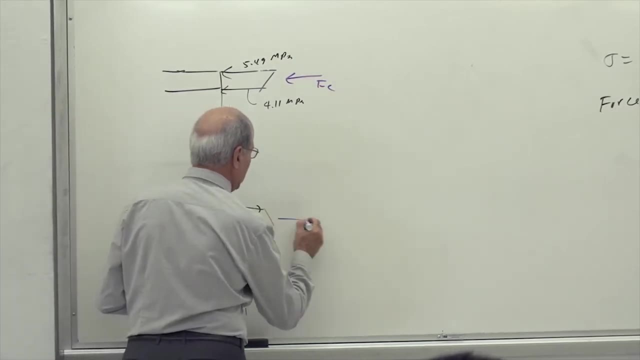 would be the resultant of all these stresses. going in is a force. I call it here FCE. Is that correct or not? I'm looking for that FCE, And the resultant of this force going out, it should be FT. The two are. 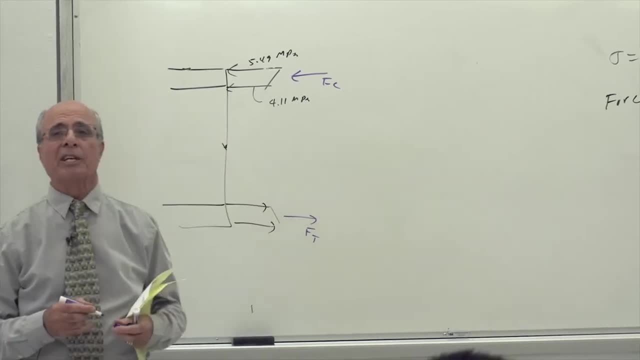 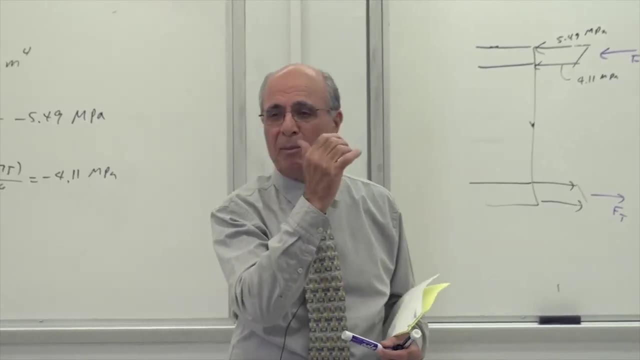 equal. and Because, in this case, because the stresses are exactly the same- Is this a couple? So if I find the distance between the two, I can find how much couple taken by these. See, this is what I want you to think When I put this. 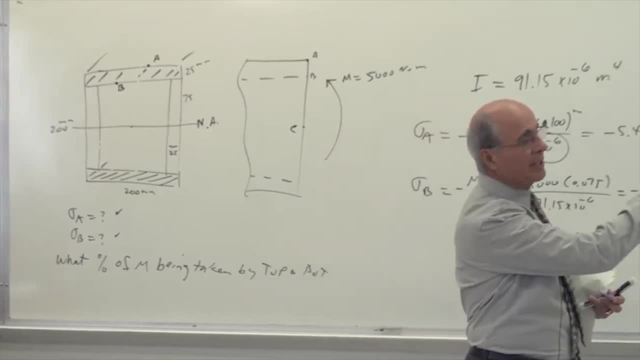 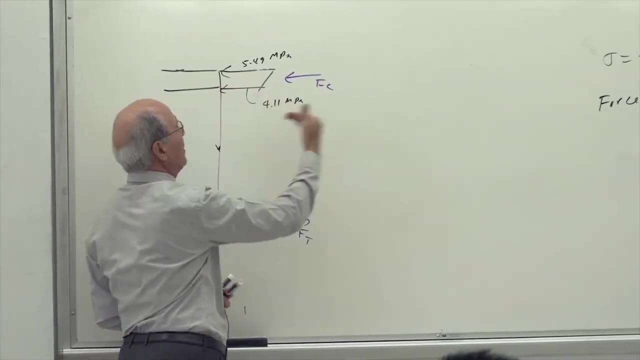 this is imaginary. This actually always is like that. Everybody understand that The formation of the stress is like this. This is imaginary. This actually always is a couple. So stress make it looks like a couple: Forces coming going in, forces coming out, or stresses because force over the area become a stress. 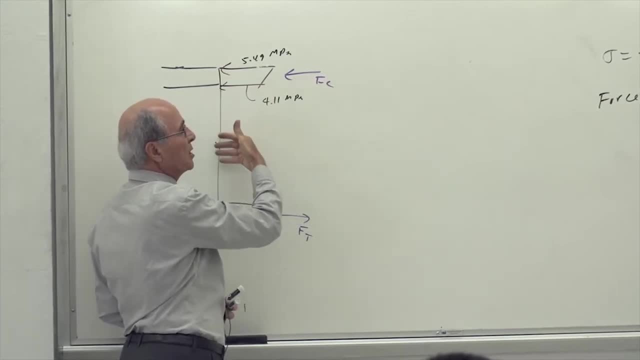 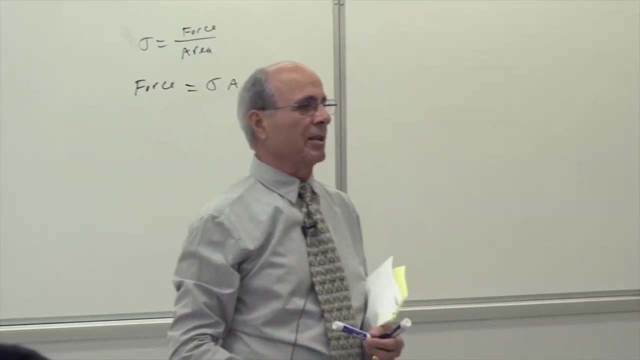 Stress is going out, Stress is going in. The only difference between this and lecture one was their sigma was always was a constant, It was uniform. Is that correct? So I can always multiply here I have if, by the way, in the book they 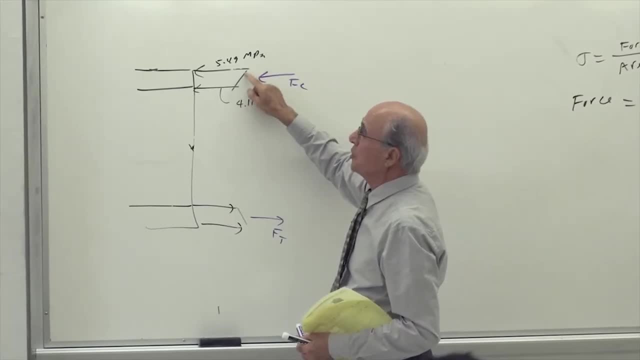 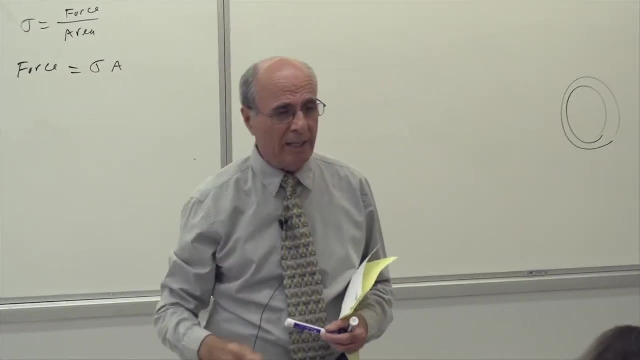 use integration It doesn't need. you don't need the integration because this is a line, so I can average it. Everybody understand that. So I can find the average sigma on top and on the bottom. Everybody see that Because linear. again. 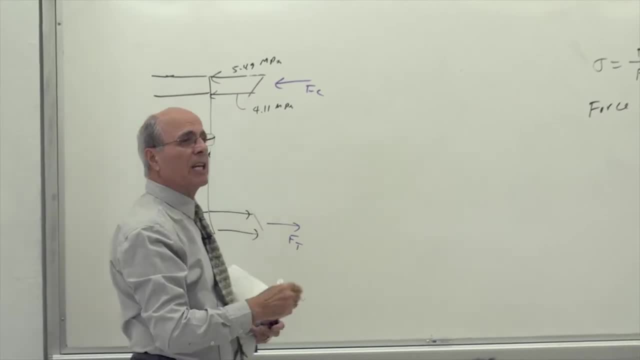 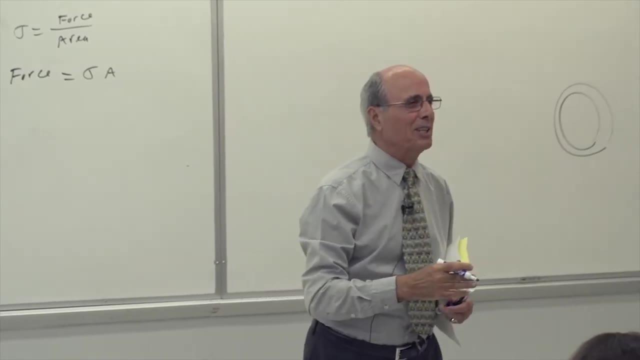 But if this was a parabola and a parabola, then I had to integrate mathematically. But we don't get that sophisticated not yet. Is that understood? Yes, But technically you can do that. Nevertheless, your this is. 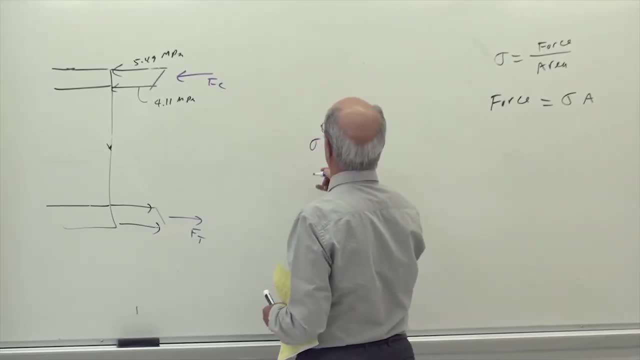 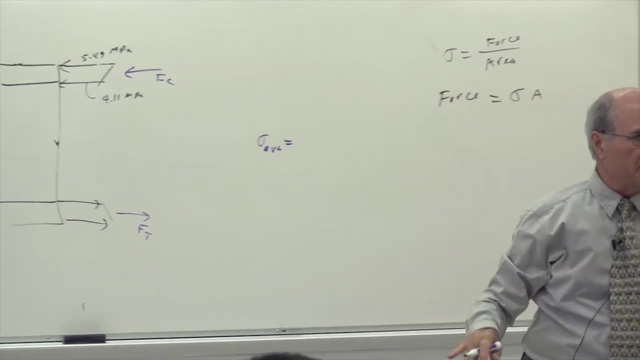 you first calculate this? Because since I'm calculating these forces, I put it in color. in this color Sigma average on top or bottom, one is in tension, one is in, one is in compression, one is in tension, Doesn't matter, You have it there. 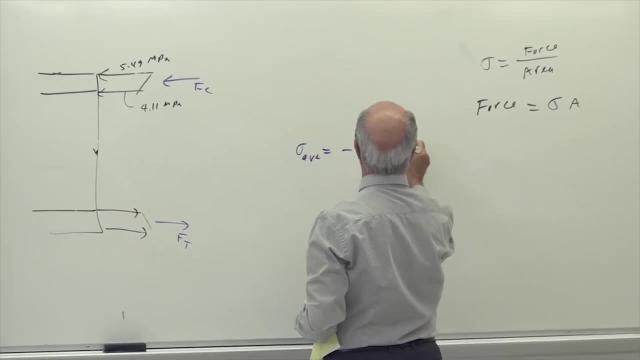 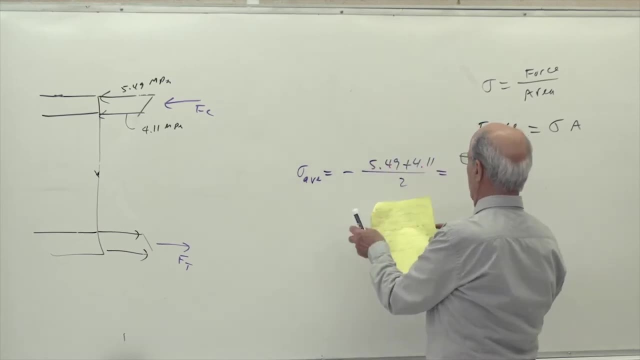 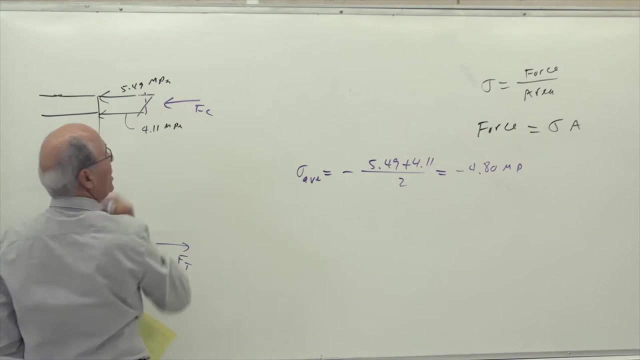 You put a minus there. You average it 5.49 plus 4.11, divided by 2 minus, because we are calculating for the top, And it become minus 4.8 megapascal Instead of these two. I'm reducing it to that. Everybody understand. Now it is a. 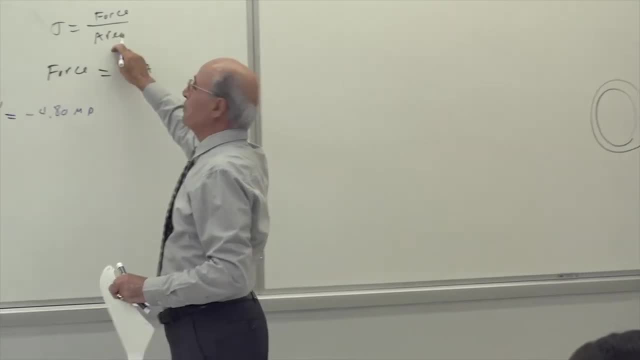 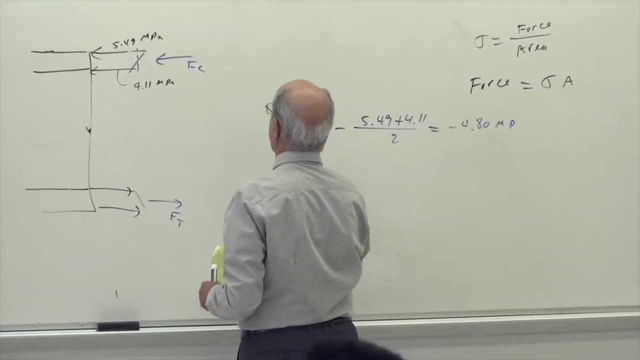 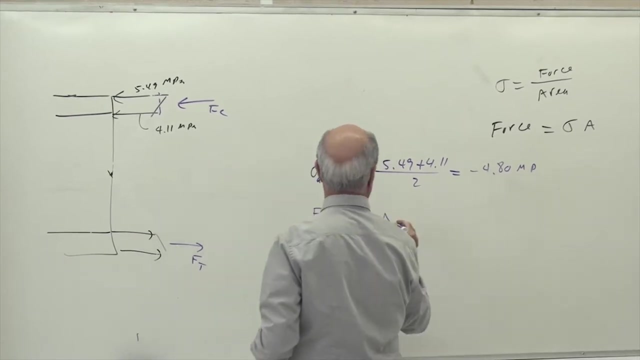 constant sigma. Constant sigma multiplied by area become the force. Is that correct or not? Therefore, then, the sigma- now I can calculate by force- FC, FC becomes sigma times A, sigma average times area on top. This is the area. So 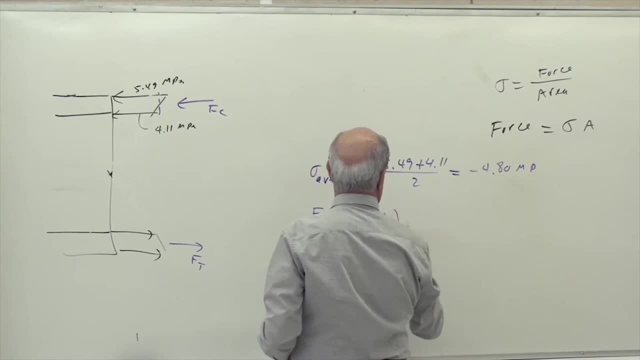 please write it down: Area A of area of the board above, Because we are only talking about this board there, So that A sigma is 4.1.. 4.1 minus 4.8 megapascal, which is 10 to the power of 6 pascal, which is: 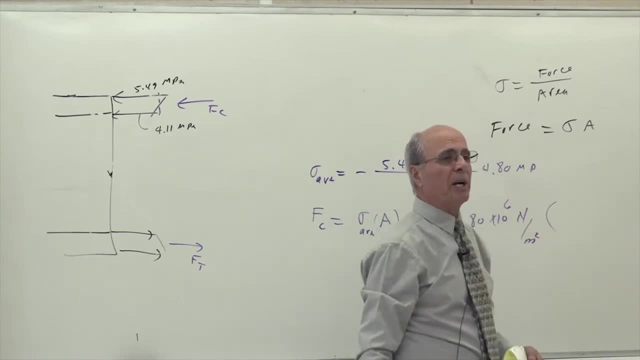 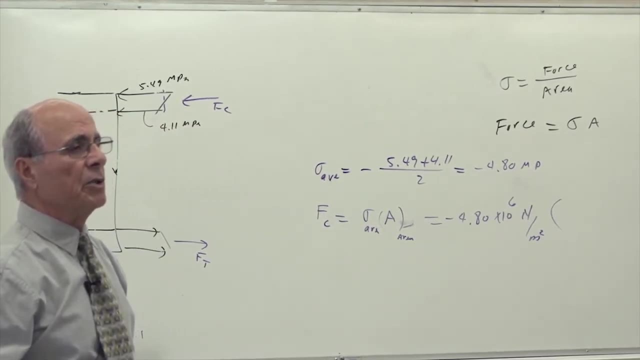 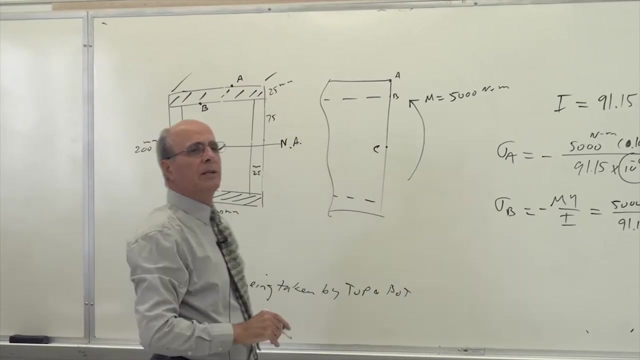 near-turn pair: meter squared multiplied by area which is meter squared, Therefore, the answer would be in near-turn, which is the unit of force. Is that correct or not? So how much area do we have there? It is 200 by 25.. That's. 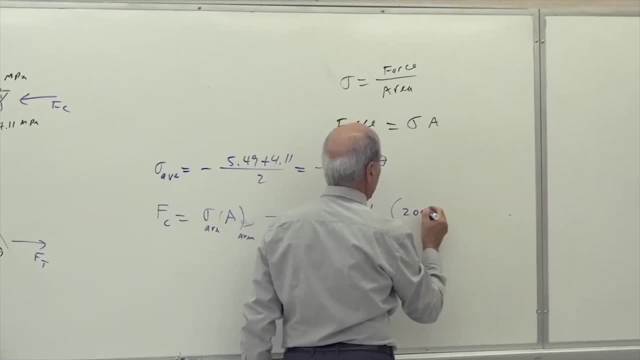 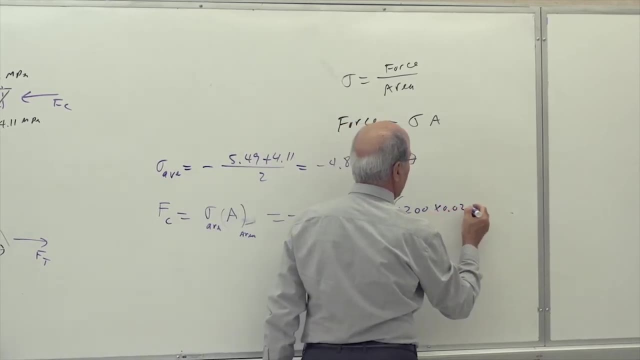 simple enough. Now that you get the idea. you understand what I'm saying there. That's 200.. Of course you have to put it in meters. So you have to put it in meter because you want to drop it meter by meter, squared multiplied by .025.. 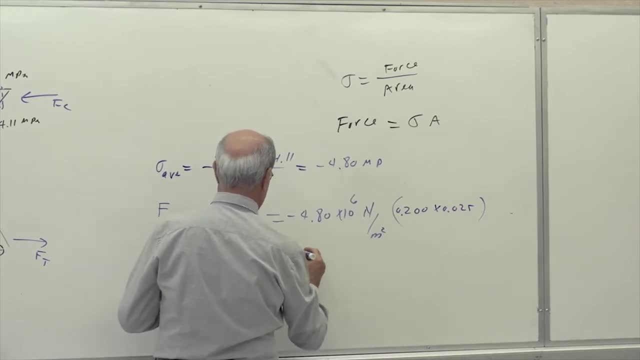 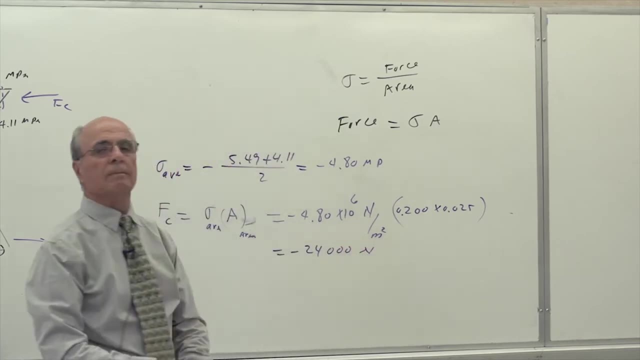 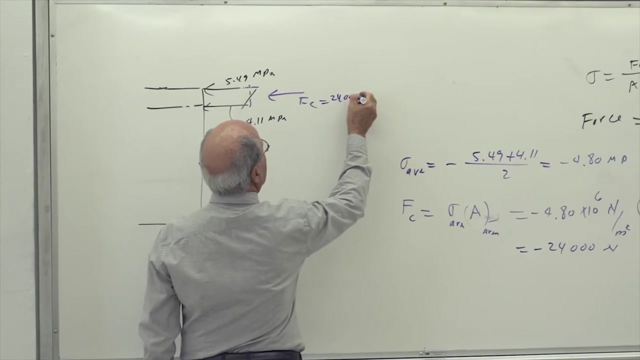 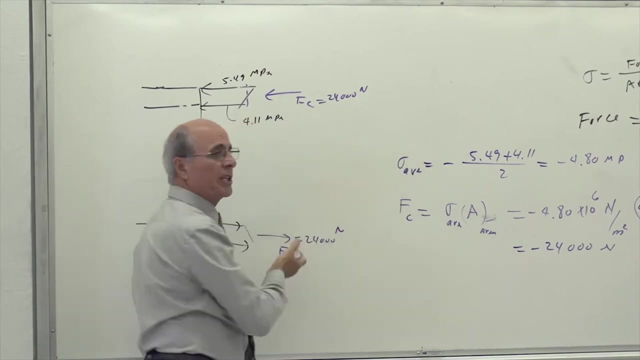 And the answer become equal to minus 24,000 near-turn, Exactly So. this force is 24,000 near-turn going in. This force is 24,000 coming out. Notice, this is a couple, Yes or no? That couple is part of that couple, But not. 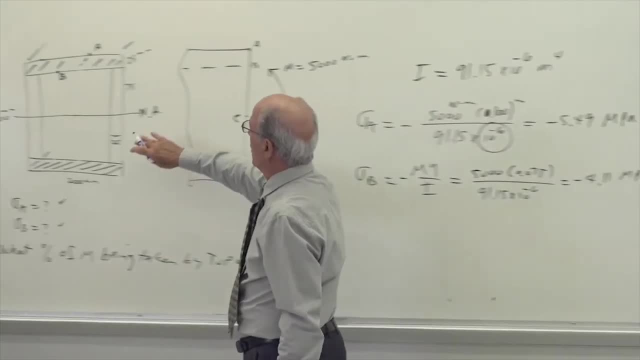 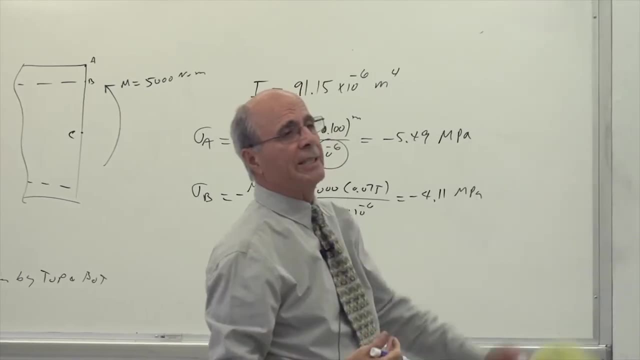 the entire couple, because this part also participates to a certain degree. But this is the highest load because the stress is on top and bottom. That's what I was saying earlier. If the stress is on top and bottom, Now all you have to do. 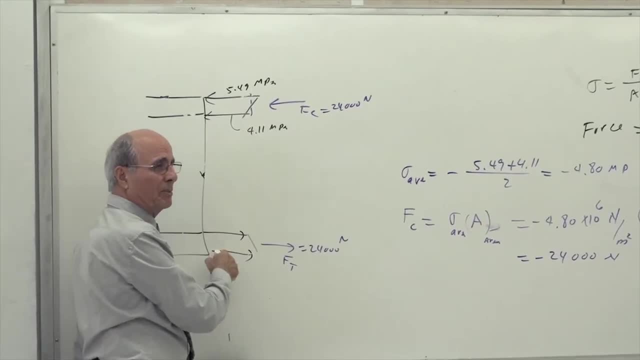 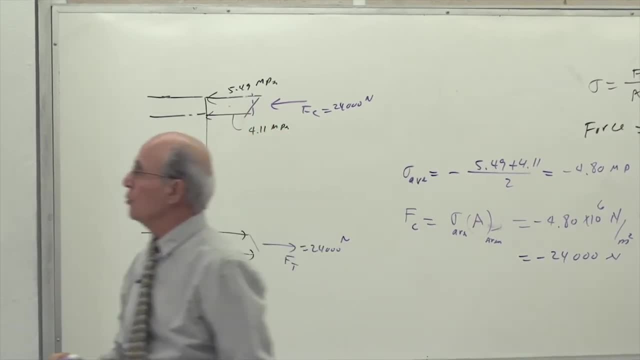 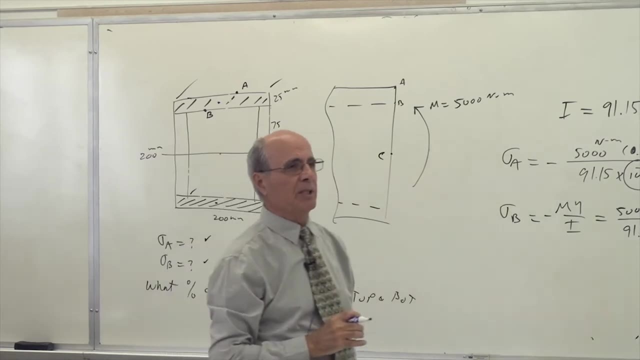 from here to here become 175.. So we are talking about from middle of this, middle of this, which is not the correct answer, not the exact answer. Everybody understand, But since this is a trapezoid, and then here is there. if this was a 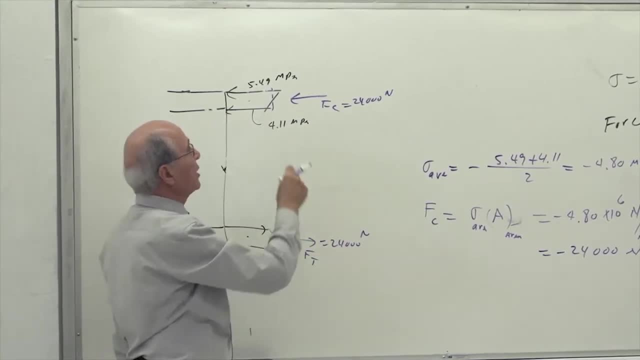 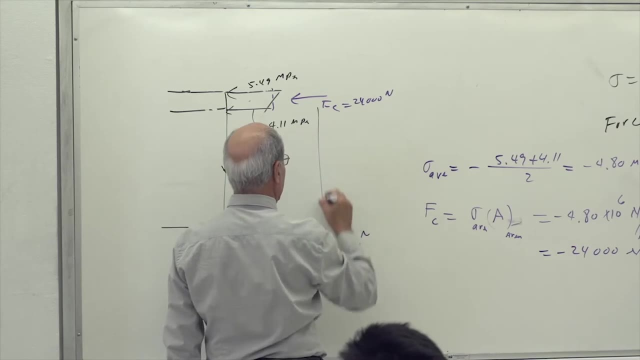 class exercise. you did not. I don't give you enough time to do that. So you assume the centroid is at the middle, which is not. Everybody understand that. So, however, I can give you the distance, to you, the exact distance, This exact. 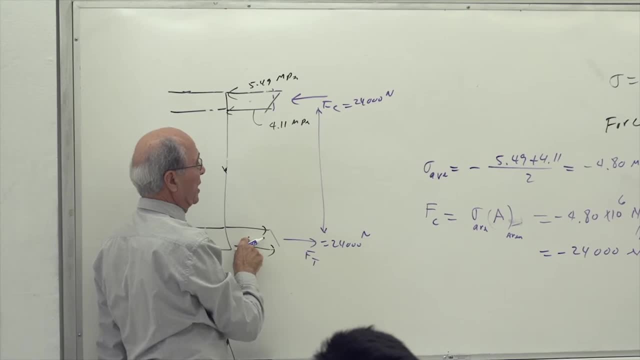 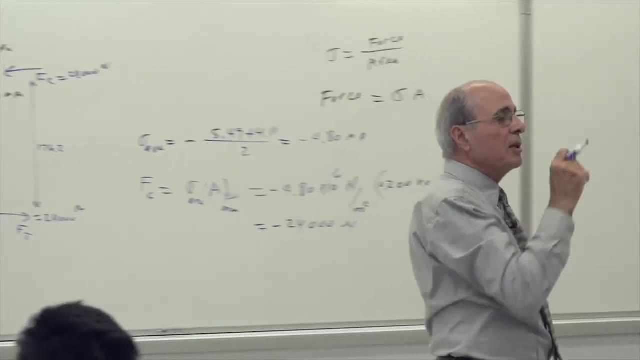 distance. if you use the centroid of trapezoid here and here, become 176.2, only one millimeter extra. Everybody understand, Because centroid is a little bit higher. Everybody understand what I'm saying. Nevertheless, the amount of M. 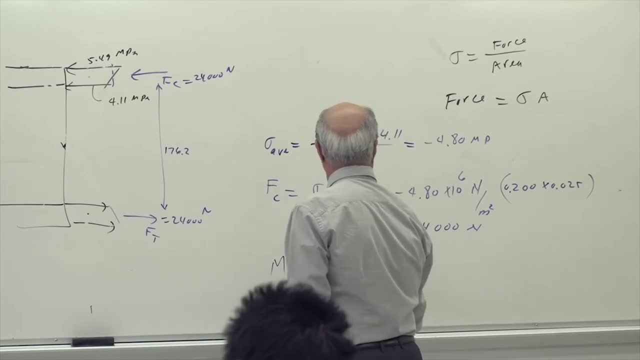 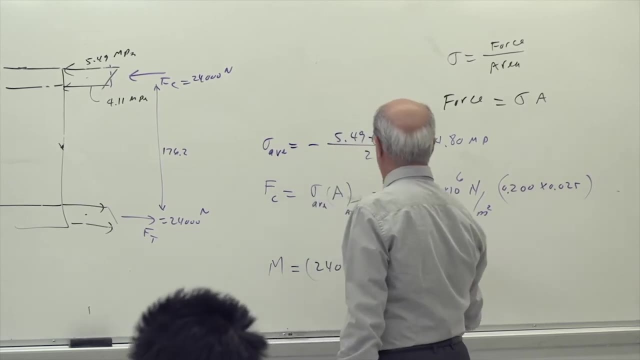 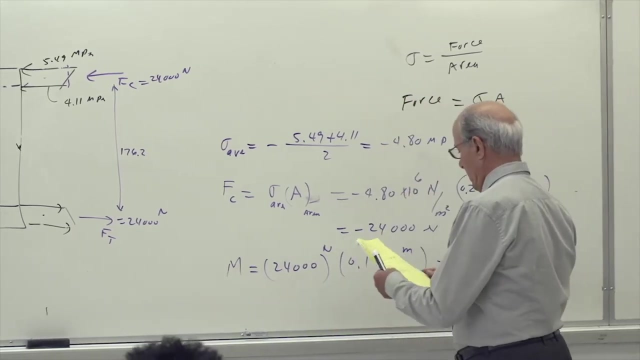 taken by the top and the bottom, as I said, that here become 24,000.. We need the magnitude Newton multiplied by .1762 meters. So this is the distance from here to here: 176.2 meter. When you calculate that one, it end up to be 4,222. 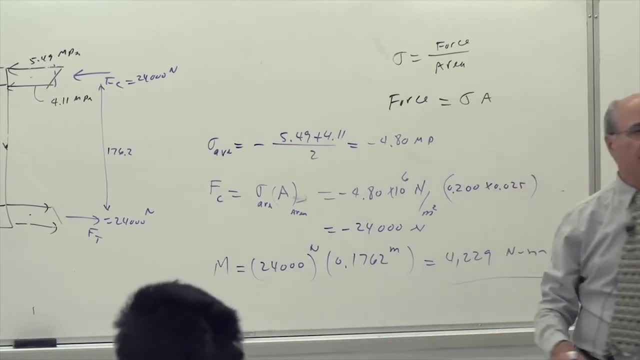 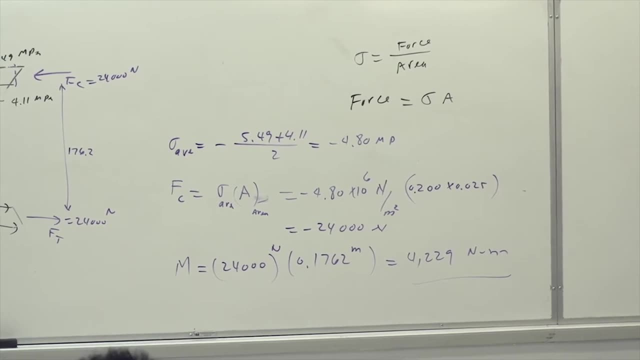 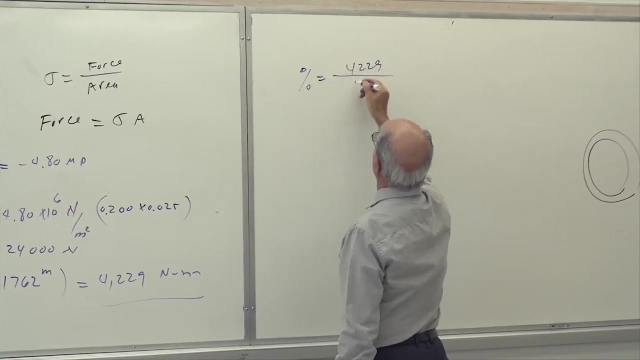 Newton meter. How much of that moment is that? More than 80%. Everybody see that. Yes, The percentage. if you want to calculate the percentage, the percentage would be equal to 4.229 over 5,000 multiplied by 100.. So that's the percentage. 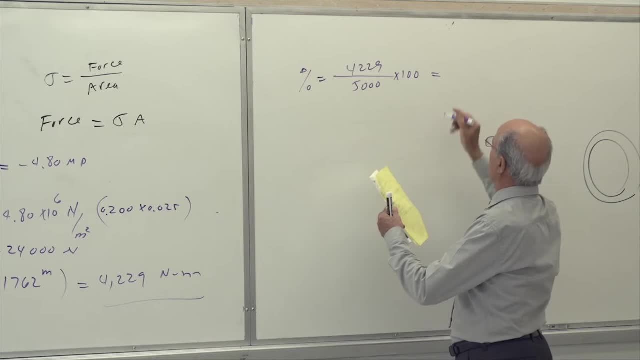 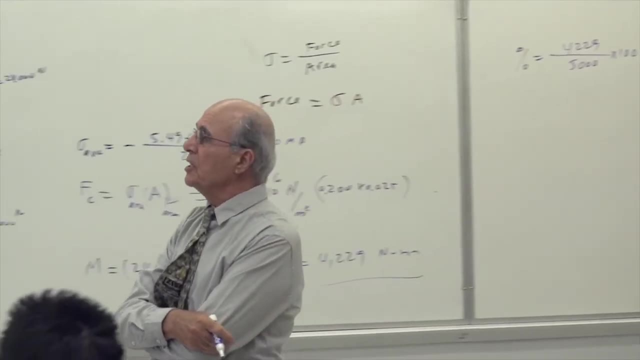 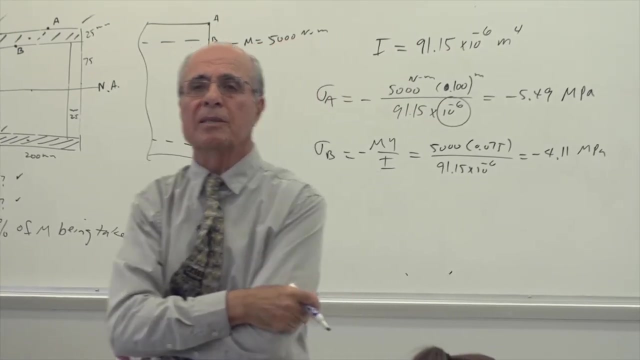 Multiplied by 100.. So it is become equal to actually 84.6%, Almost 85% of this moment. in other words, I do not need those middle pieces. If this was a still, I just connect that with a little piece in between. Is that correct or no? Yes, Of. 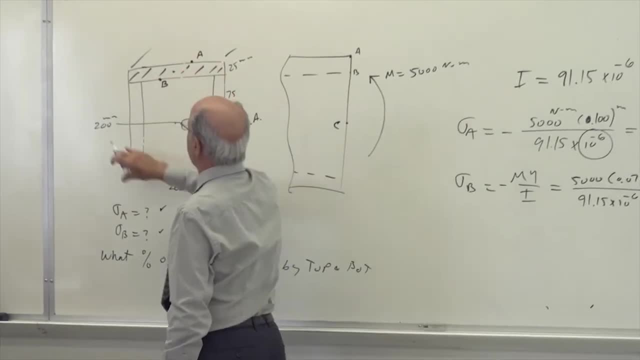 course, the ideal beam would be material here, material here, nothing in between, a string between. But that doesn't work because we have to also think about shear stresses which come into play. So that's the difference. So that's the difference. 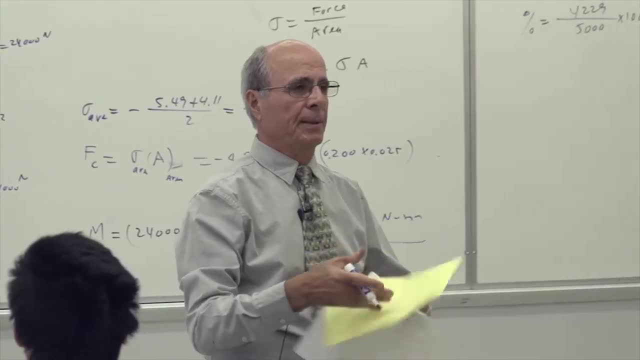 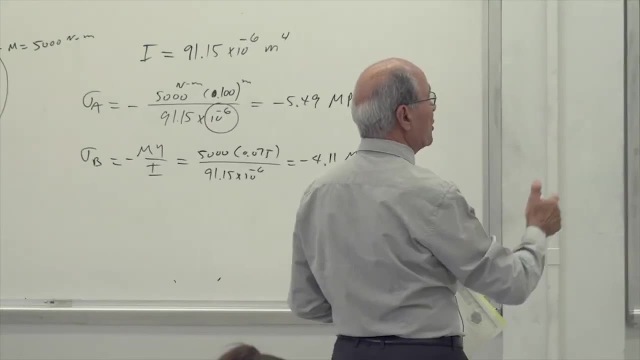 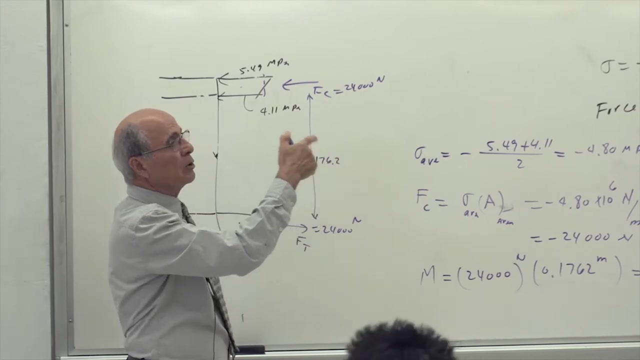 Stresses which come in chapter 6.. Is that understood? Yes, Any question That gives you again another insight into this stress. The most important part of your system again is not thinking about sigma equal to P over A or sigma equal to MC. 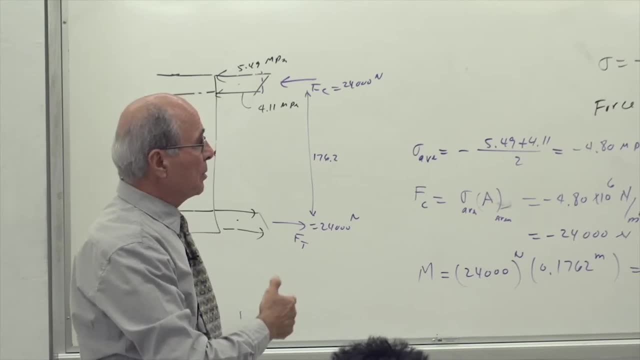 over I, et cetera. It is the stress distribution for the shaft. I mentioned that Here for the beam. Is that correct or not? Now we come to the stress distribution for the shaft, Here for the beam. Is that correct or not? Now we come to the 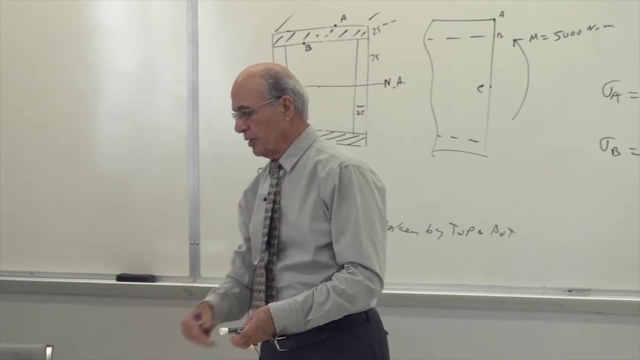 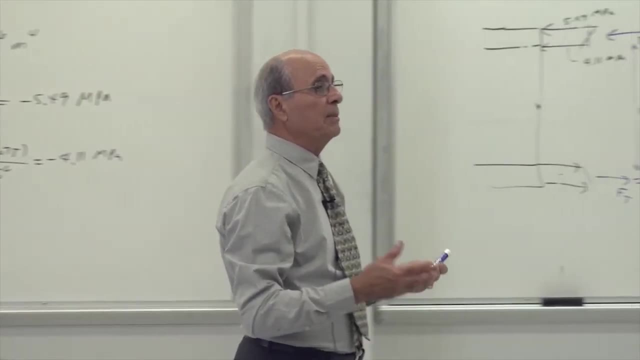 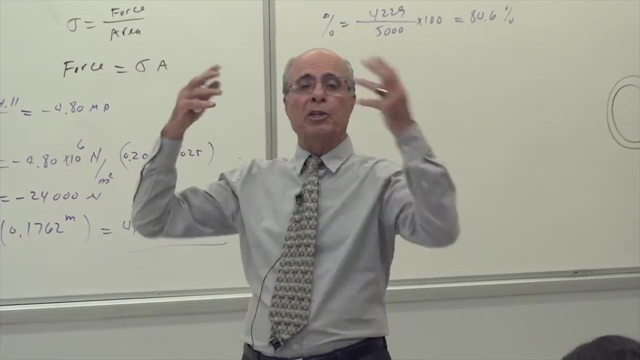 last part of this chapter, which is eccentric loading, Please write it down. And the combined loading or eccentric, which is the most misunderstood part of this chapter by a student. The reason is they don't think this way. They always want to get the answer from sigma equal to MC over I and the answer is not. 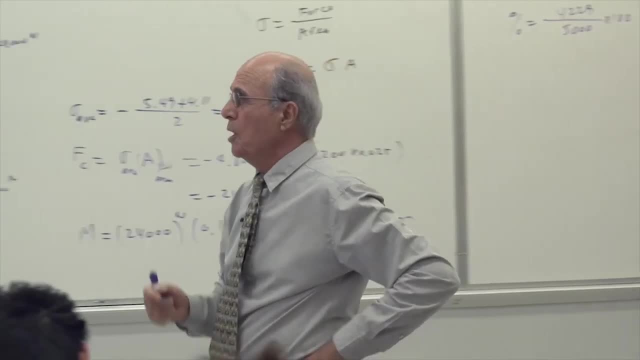 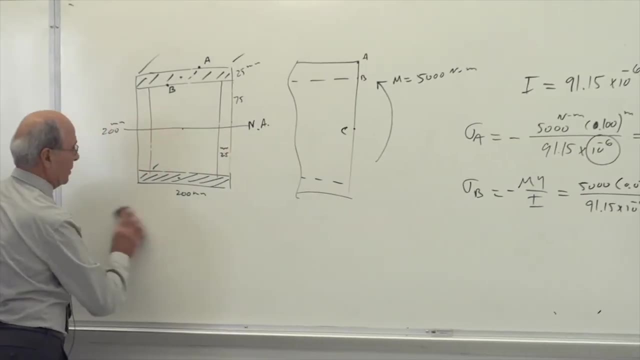 there. Everybody understand. Now I'm going to make it very clear for you, because I have seen a student usually have lots of problem with this, So I'm going to use this system. However, look at it. I want to repeat some of the material that. 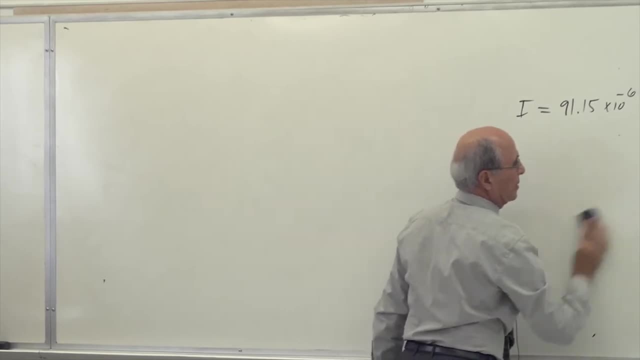 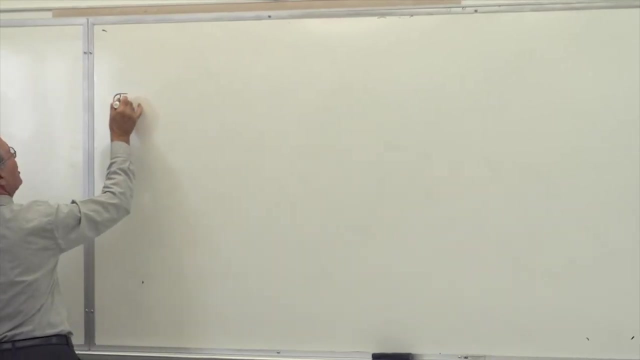 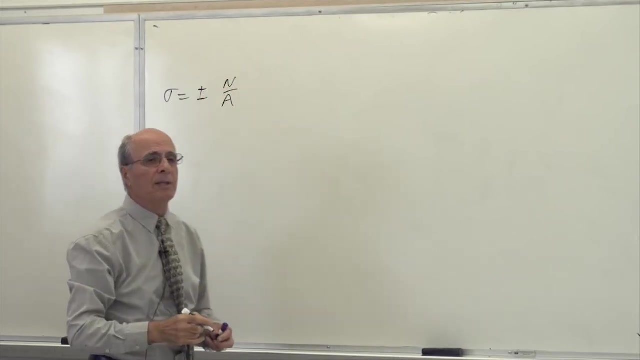 we already did in the last three chapters. So before we go any further, notice: in chapter one and two we were talking about sigma equal to plus minus N over A. What was N? I purposely did not put P over A. I put N over A because N is the. 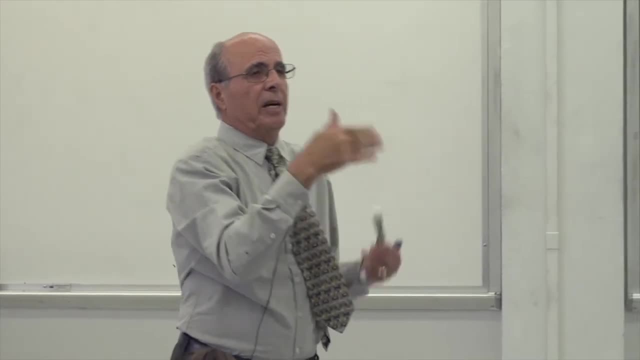 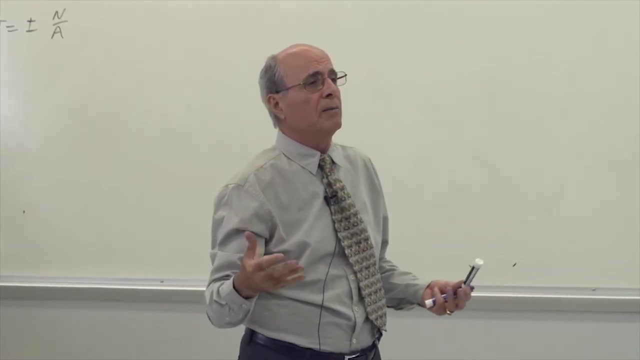 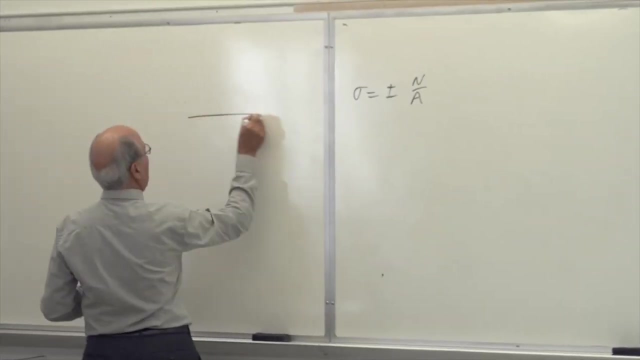 normal force to the cross section. Now why I'm saying that? It's very obvious. I give a quiz to the ME 219 at the beginning to test their knowledge of ME 218. in my class this quarter I give them this, of course, this rod, And I put here a. 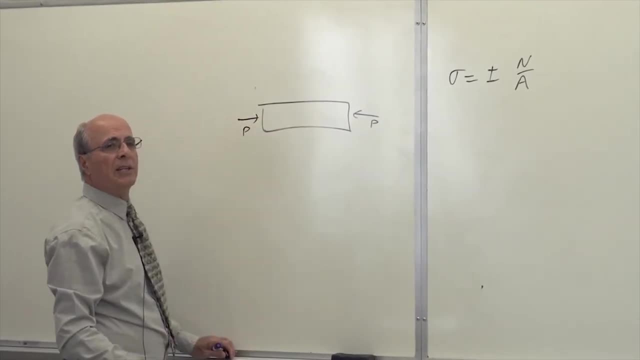 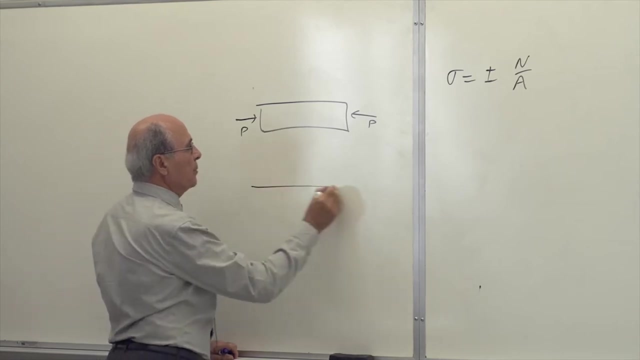 P here. Is that correct? P here? So everybody knows that is sigma equal to P over A, because that's the. I change it to N for that. Then I give them this problem And I put a P here. Is that correct or not? Is this problem? 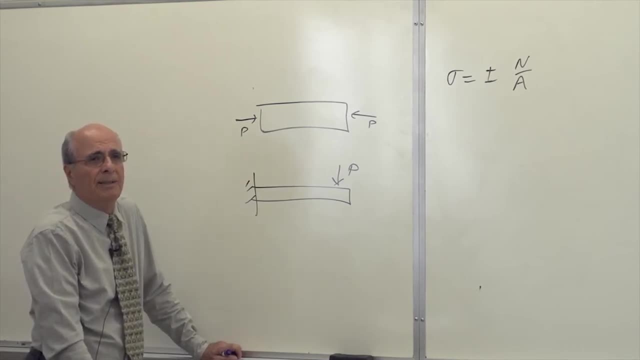 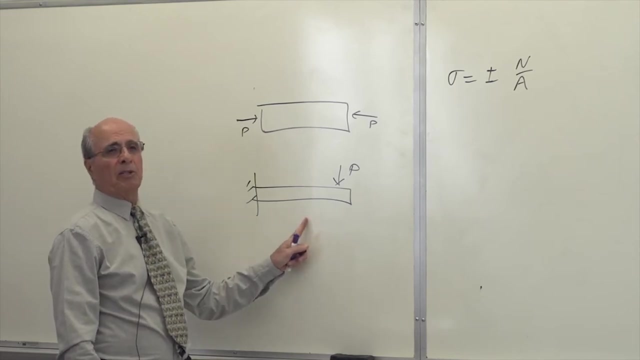 has a sigma equal to P over A. you think, Come on, guys, I don't see anything. You're not seeing the difference between the two. Is this axially loaded Ten, 15 people out of the 40 people, or 45 people put here? sigma equal to P over A. 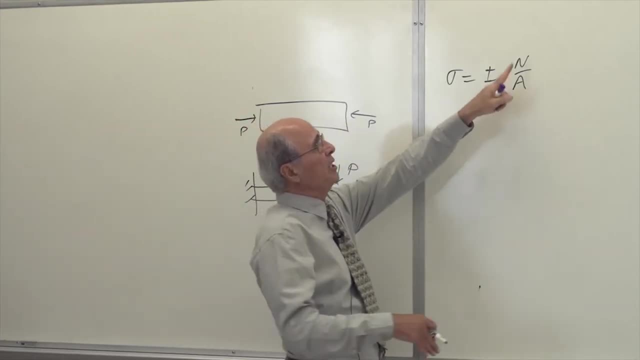 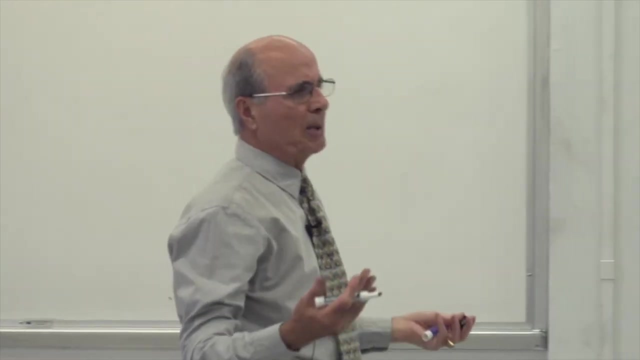 because they are not thinking. They are already seeing, So they are not thinking. No, First of all, they didn't see it this way, They saw it this way. Do you understand what I'm saying there? Since they saw it this way, they saw a P. Okay, sigma must. 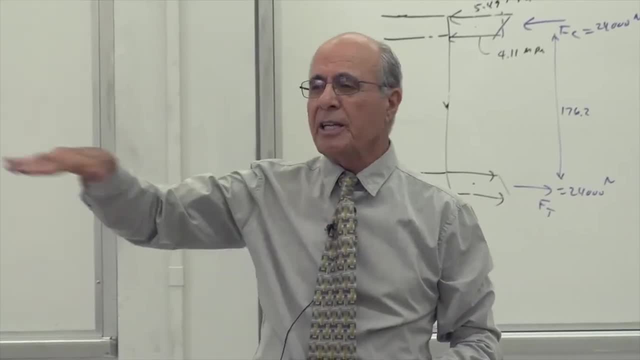 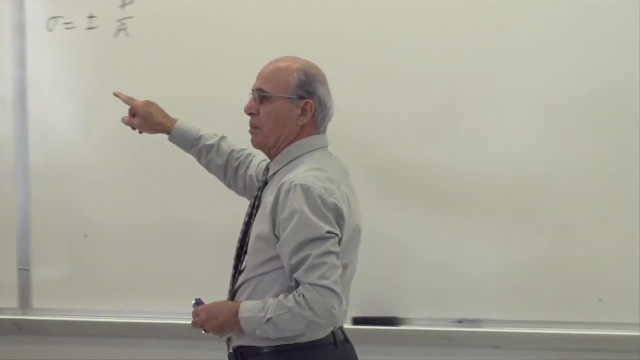 be P over? Absolutely wrong. If they are there, they have to take ME 218 one more time. Is that correct or not? Look what is there. That one is axially loaded, Remember, because when you cut it here, the force is right at the centroid Is. 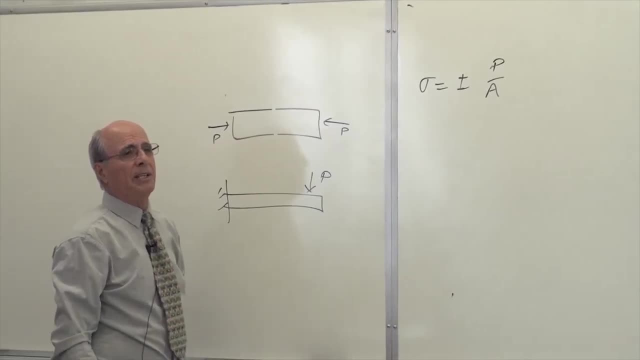 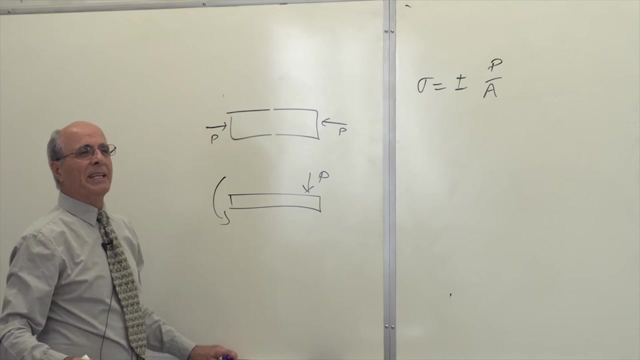 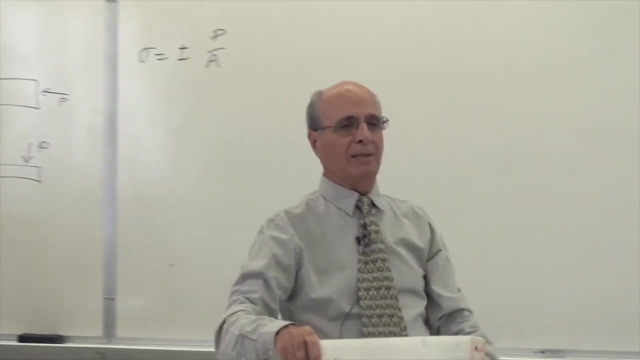 that correct? Actually, if it is not at the centroid, we have a problem there. Is that correct? This one actually is A bending. That's what chapter four is all about. This load causes here a bending. Look at it. Put a load at that end, my friend. You see that This is bending Has. 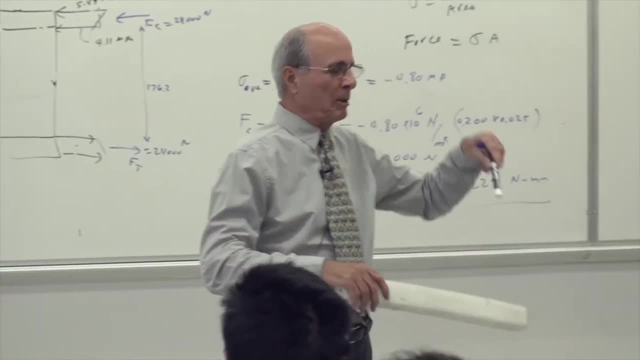 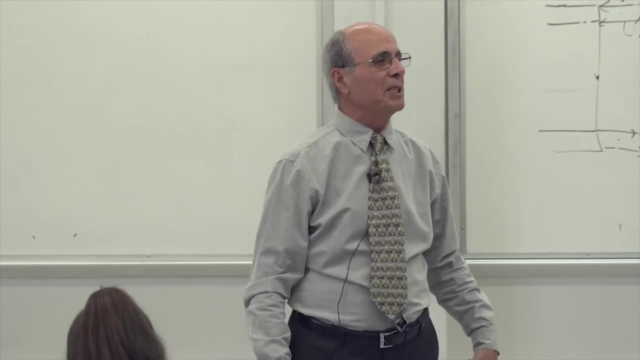 nothing to do with P over A. Everybody see what I'm talking about. We call it P because there is a vertical force. So be it. Not every P is sigma equal to P over A. Everybody getting the answer to that. So you should not make that kind of mistake. 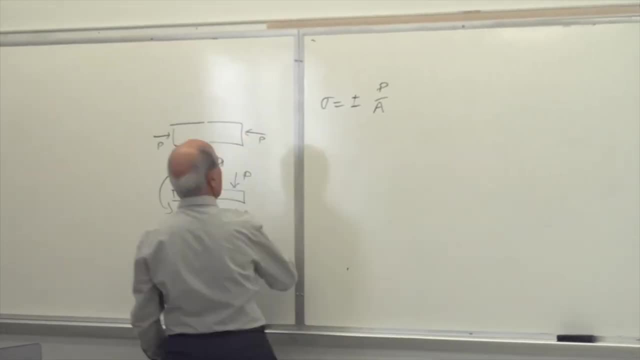 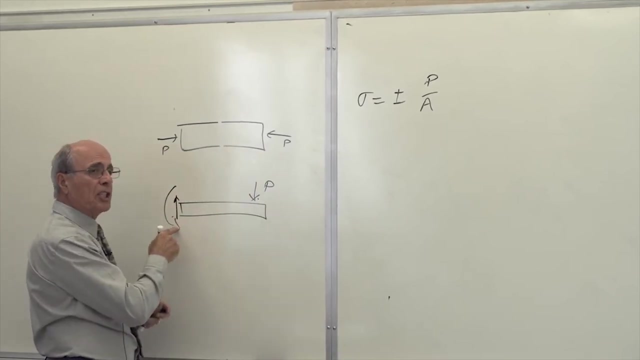 in this class or ever. So this is a bending problem. This is a. As a matter of fact, there is a force also going up this way because, again, that which become a shear problem, which is chapter six, by the way, We are going to. 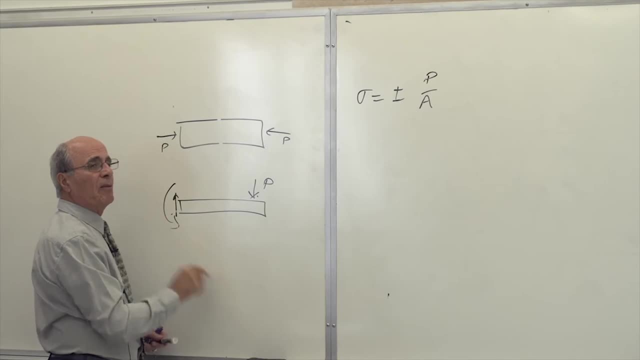 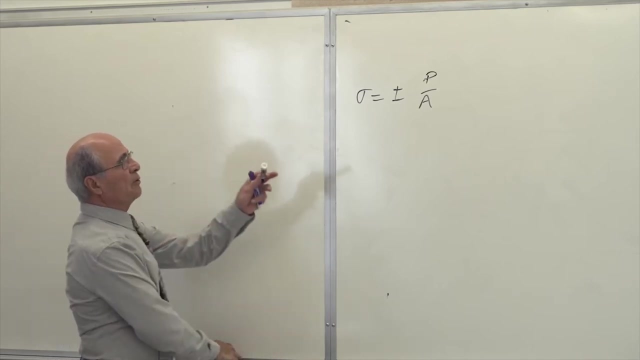 go to chapter six for this one Again, one more time. This is the one we are talking about right now at the bending Has nothing to do with this problem. Everybody understand that. Therefore, this is what I'm going to change, that in. 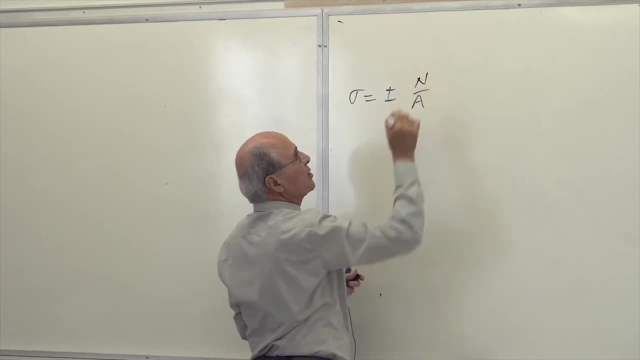 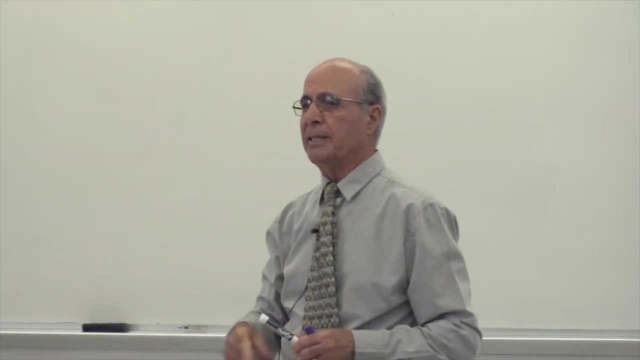 order as the beginning. I knew this problem. That's why I change it to the P. I change it from P to N in order. You do not make that mistake. Hopefully everybody understand what I'm saying there. Then in chapter two or three: sorry, 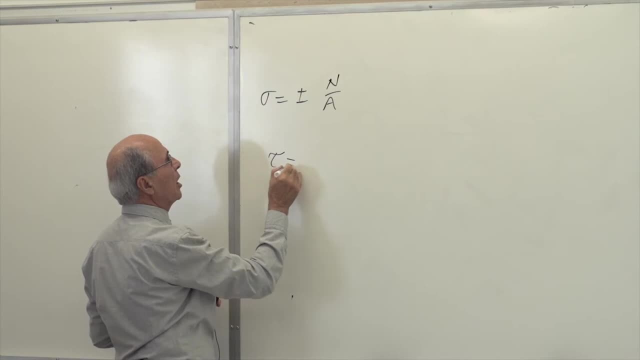 We went to the shaft design. We already talked about it. We end up with tau equal to plus minus TC over J. Is that correct or no? Yep, And then in chapter four- we just were talking finishing that- Sigma was become equal to this. This: 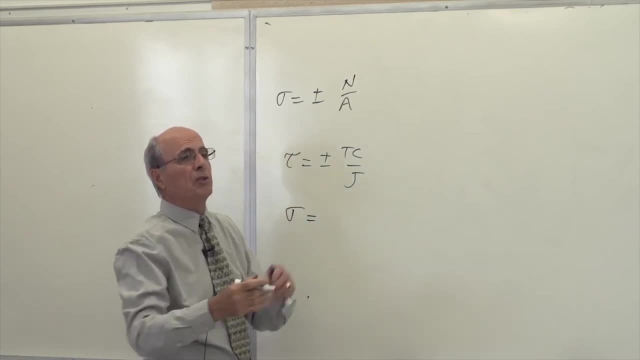 sigma. is this sigma, everybody This sigma, but coming from different source. Is that correct or no? That sigma was equal to what Plus minus? you just saw it. MC over or MY? in general You are right, MY over I, But on the top, 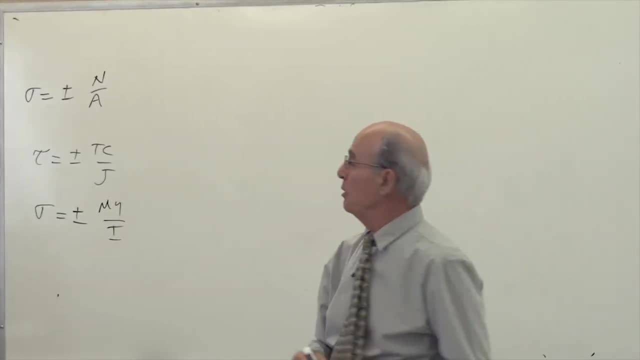 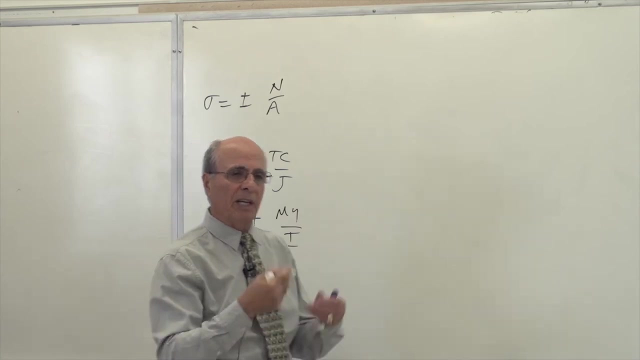 we call it MC over I, the sigma max. Is that correct or no? By the way, this was also max. So if I put here a max, if I put a max here, I'd have to change Y to C. But that's okay. That's the distribution of a stress. You are right, MC. Now. 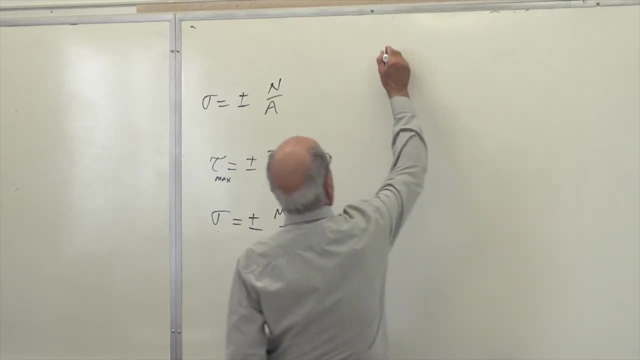 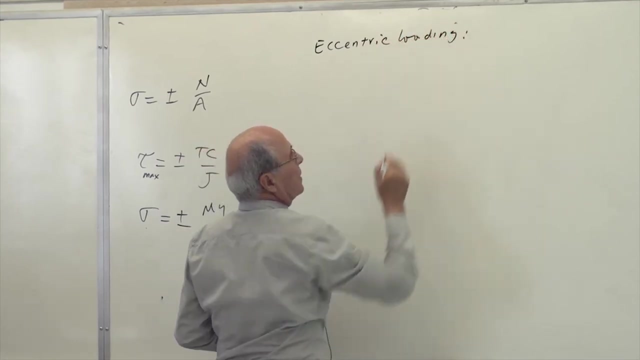 look what happened in this series of problem, which we call it eccentricity, Eccentric loading. Now, if the load, look at it. I just show it this way for everybody to understand that If I put here a plate, here a larger plate, here, 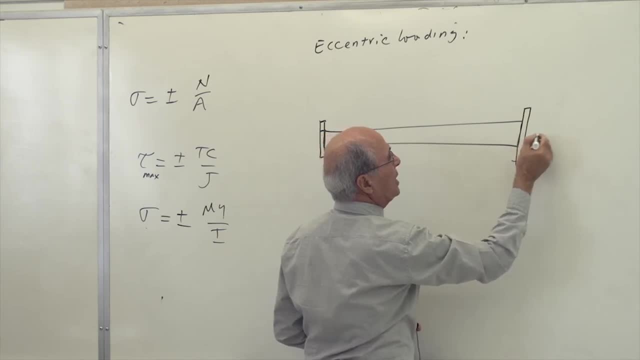 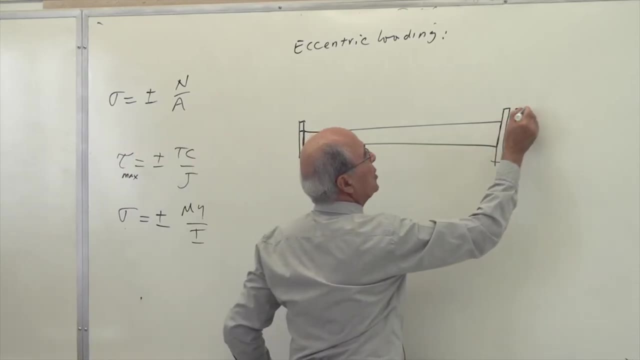 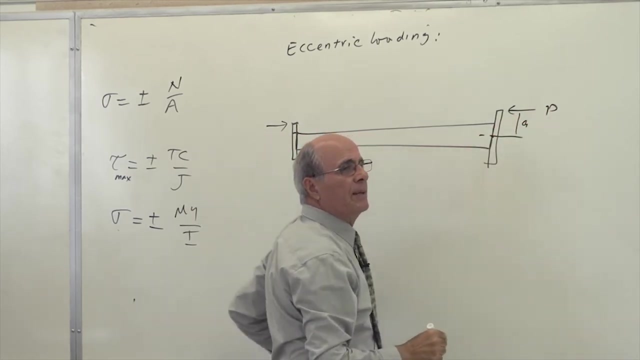 and a larger plate here. if I put here P at the centroid of this rod, that become this one, Yes or no, Correct, But I'm going to put this P here and I'm going to put this P here which has a distance of A from the centroid, Is this: 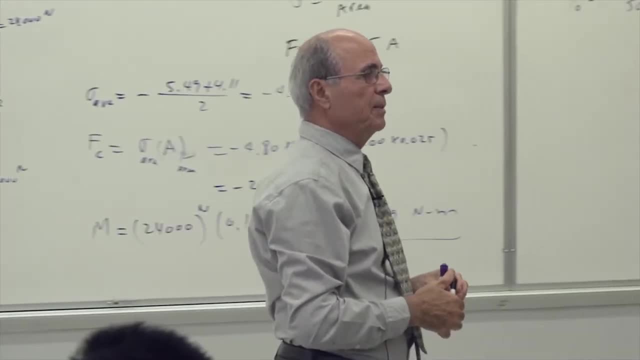 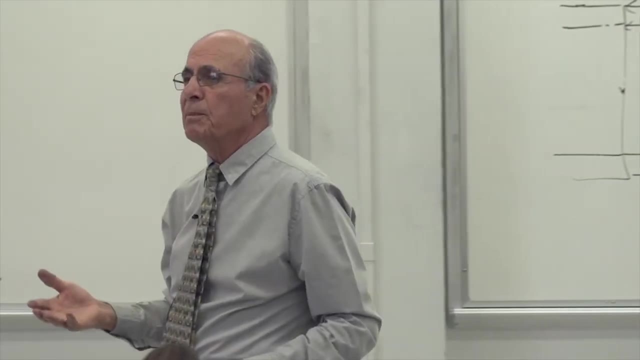 sigma equal to P over A. What's going to happen to this item? It's going to bend, And this is very simple. So there should not be really any problem. but people do not see that because this become basically an ecstatic problem or either become 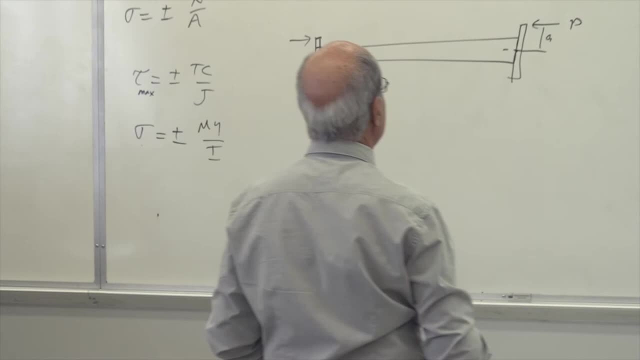 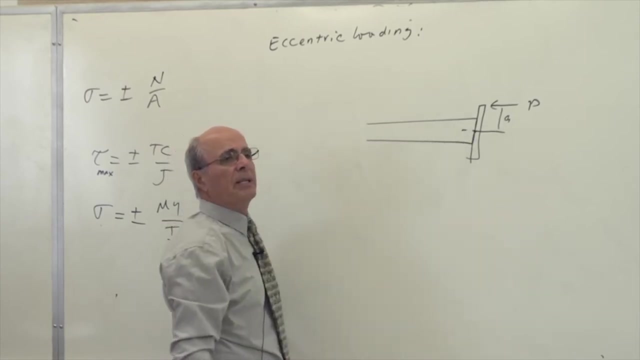 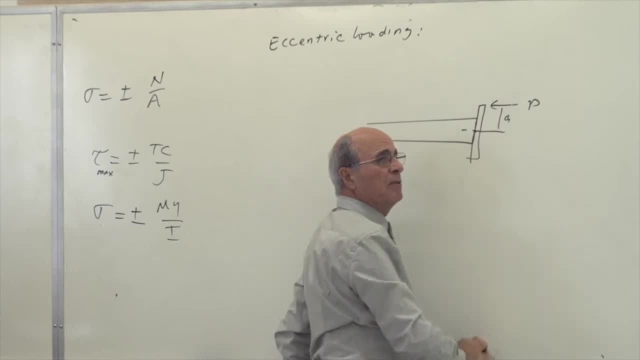 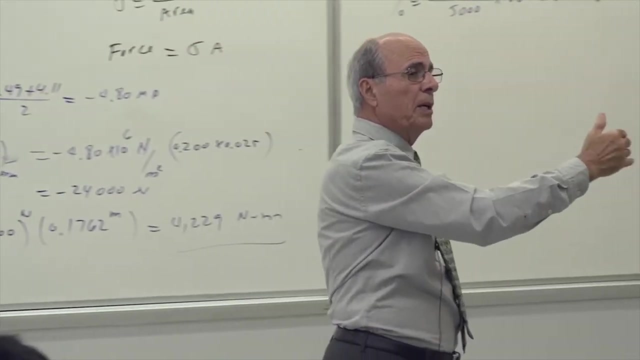 correct or not, Or you can shift this from here to here, which is the equivalent. Remember, in static we learned that if you move a force from point A to point B, you have to add a couple to it. The force become a force and a couple. That's the. 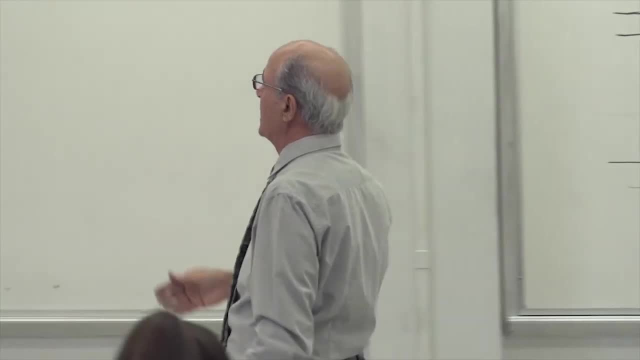 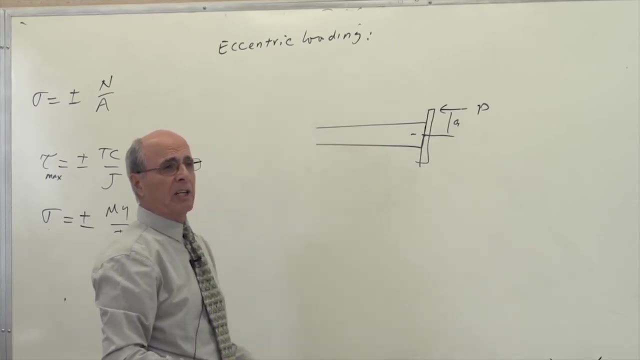 reason everybody know. the detail of it doesn't matter. That's exactly what I thought. These are the action, Here are the react. This is internal, This is external. I'm going to do both of them in order for you not to make mistake. If 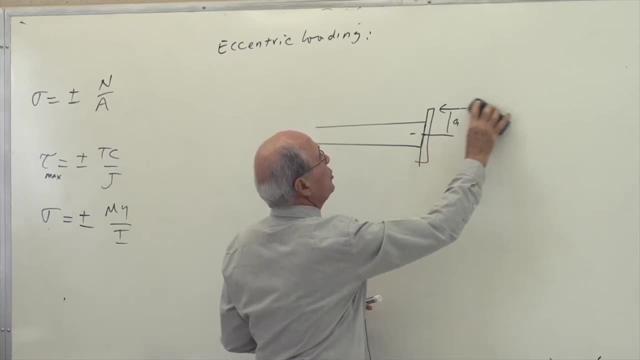 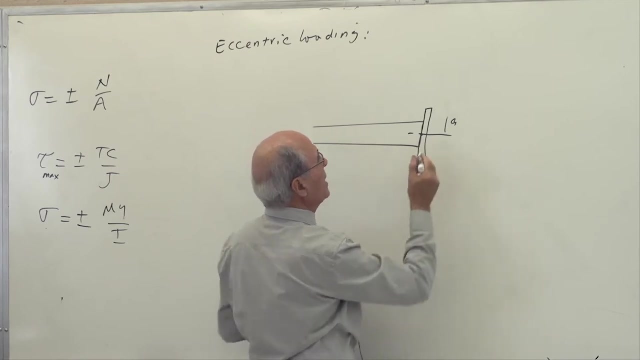 you change this because some of your homework you have to do that. If you change here to this force, this is equivalent. Is that correct or not? So that is equivalent to a force like that It was pushing, like that. You need this M Is. 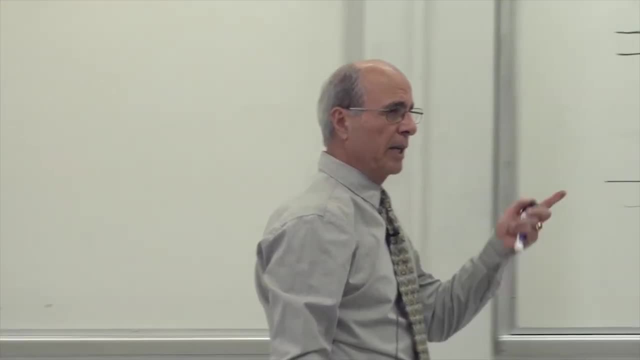 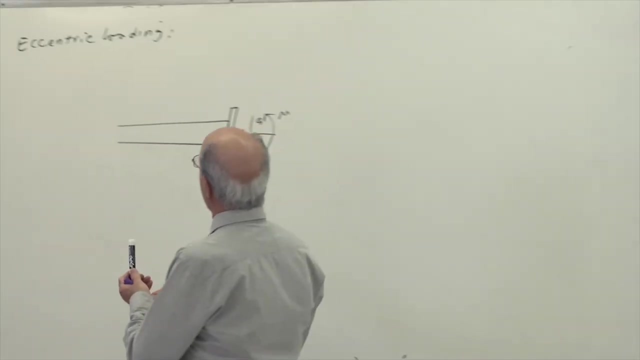 that correct And that M become P times A. That's what we had in the static. Is that correct or not? Yes, That's one option. That's one option. That's one option. Then, when you come here, look what happened When you come to this. 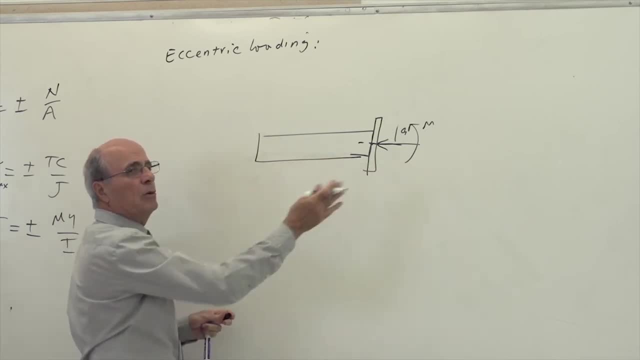 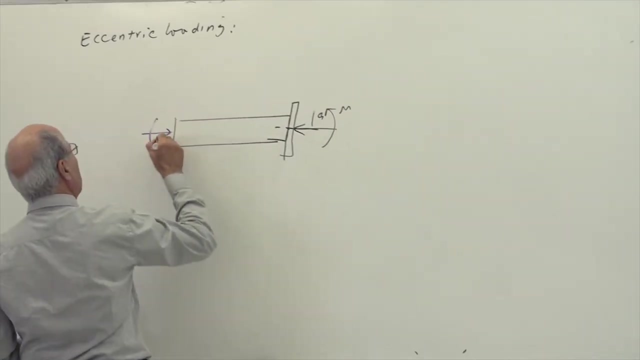 part of a beam, which is the internal part. now you have to balance this. Is that correct or not? Therefore, it become here A Look: these two together become chapter one, Yes or no? Correct? And then, since I have a couple here, I have to. 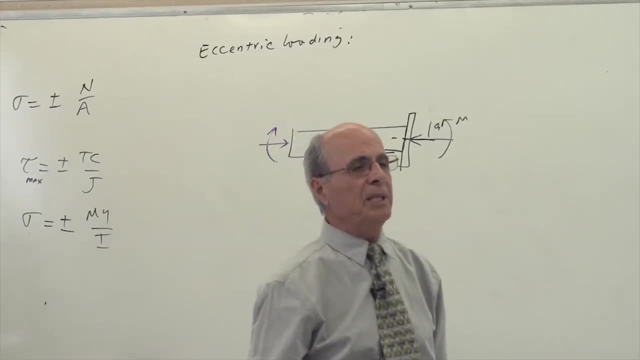 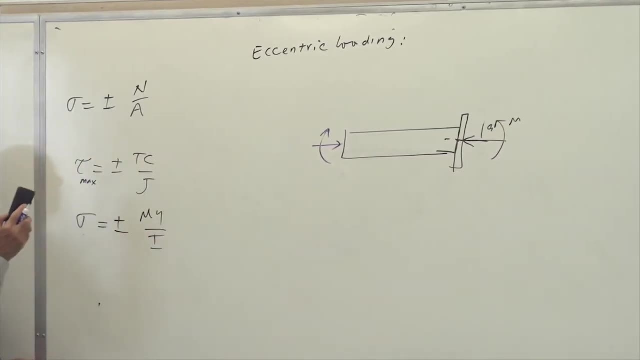 put a couple there. Is that correct or not? This is the system in equilibrium. So what do you have I have now? of course, we don't talk about equilibrium. We are not talking about this. First of all, you have to understand that You. 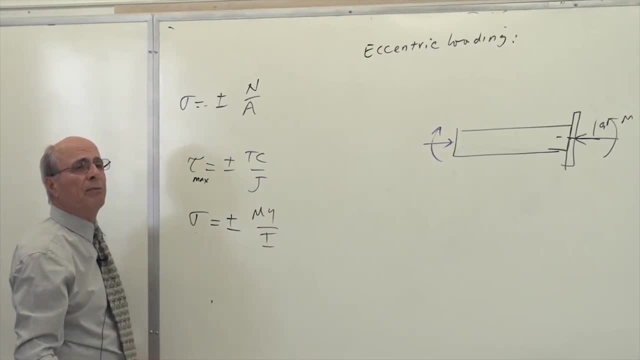 never add this to this two, because they are two different nature. These are perpendicular to the section, This is in the section, So that's out. But these two can happen together. That's what we are talking about, Yes or no? It just. 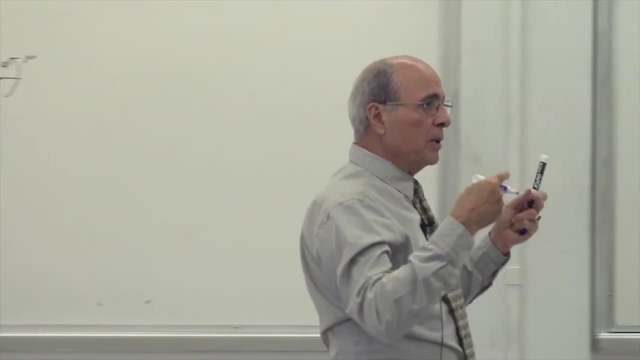 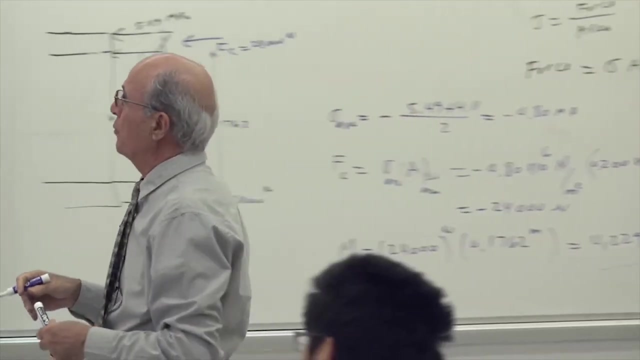 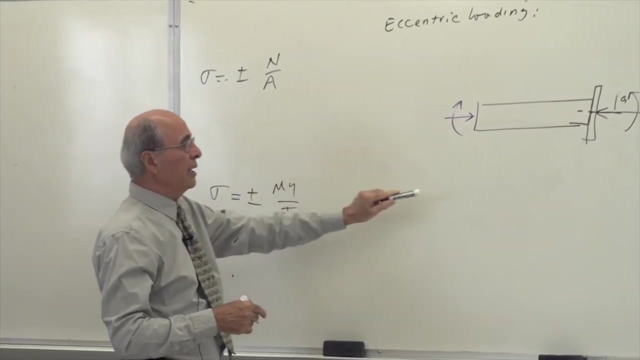 happened there. Yes, You have a centric loading plus a moment. Yes, So you have to add this together. So, therefore, your stress is here. This is the moment. This is chapter one or two. This is chapter four. Write it down Here, the. 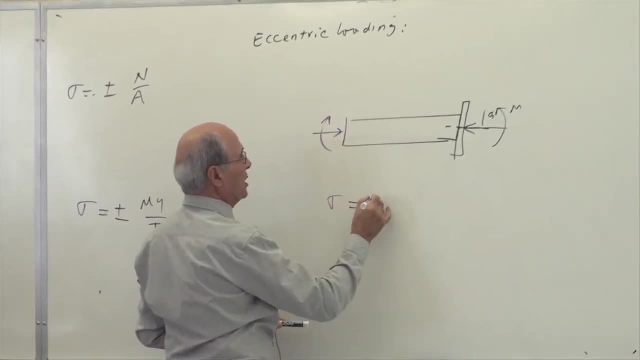 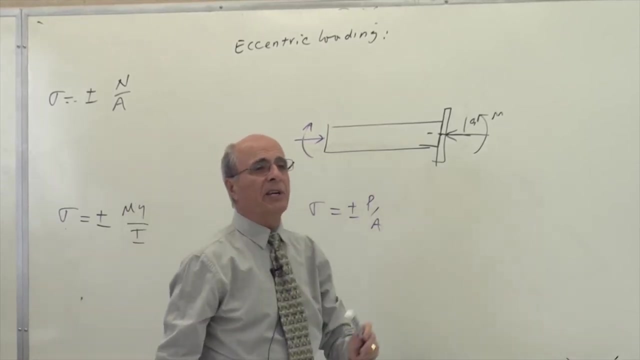 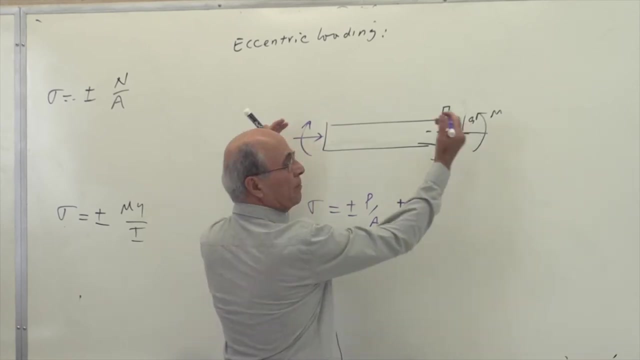 stress, is sigma at this cross section become either plus, minus. Of course you have to decide that P over A, which is the result of centric loading, Yes or no, And then plus and minus. what Plus minus of bending? Is that correct? The 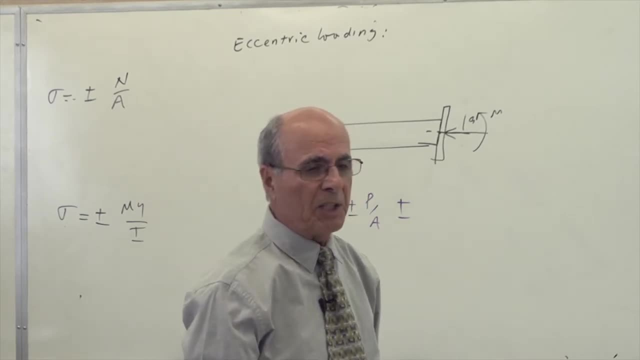 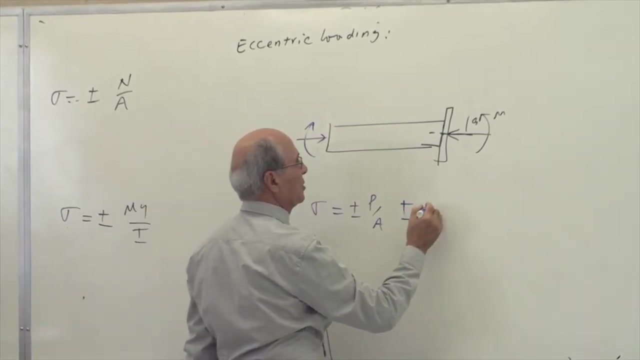 bending causes that to become a moment. So MC over I don't know, I don't know I, they are the same type. Remember, I cannot add the shear stress to these two, but I can add these stresses together, MC or MY over I Depends whether you are. 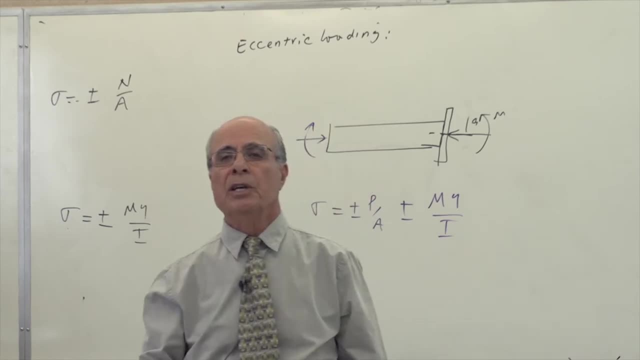 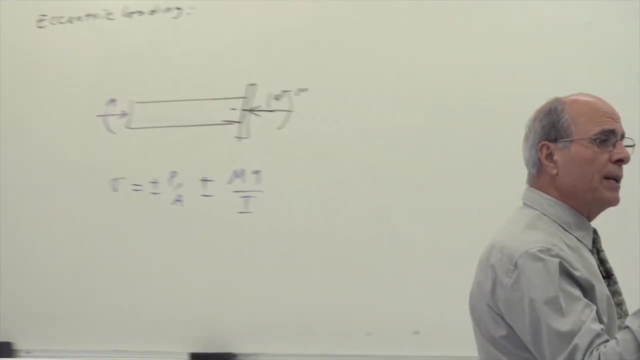 outside, inside, et cetera, et cetera. That's how you do it, So we call it eccentric loading. So all you have to do take your load to the all the load, to the centroid of the cross section and decide whether you have that or not. 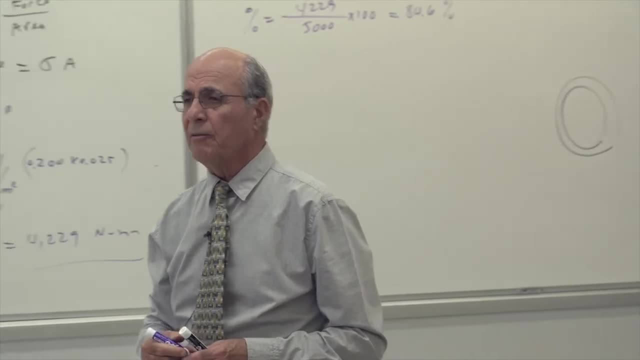 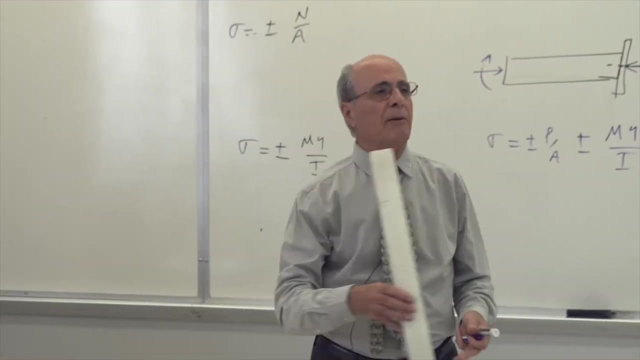 whether they are in tension or they are in compression. Everybody understood the static part of it. yes, Okay, So this happened a lot, by the way, This is very simple. You don't have to go any further than this. This is a column. You put the. 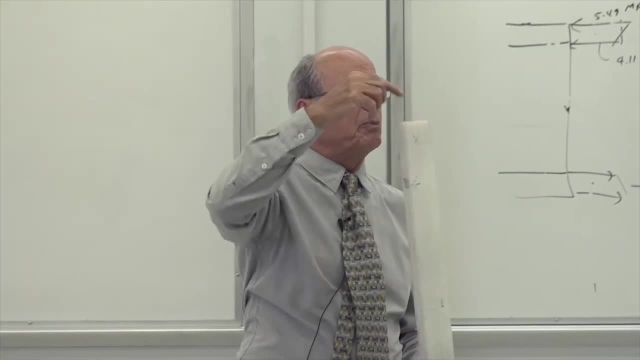 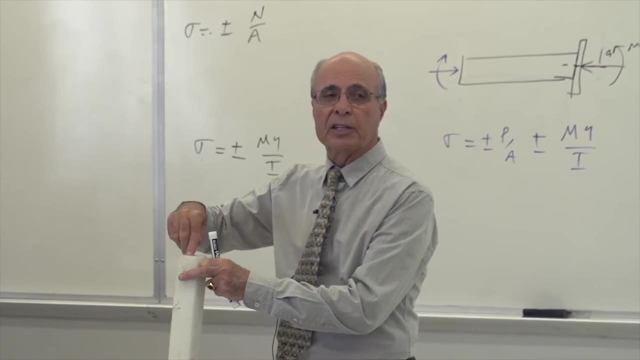 load at the right, at the centroid. The sigma here become force over area. As soon as I put my force here, for example, or here on the side, Remember I'm not at the center. Look what happened to this: It's going to bend, Is that correct? I? 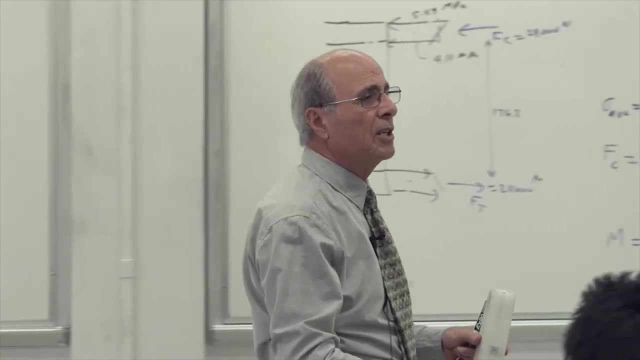 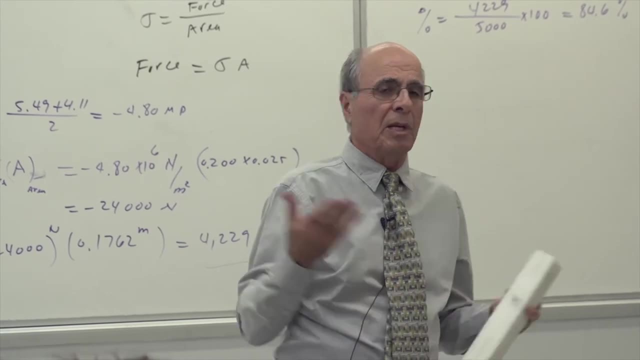 have the force there still, but aside from the force, I have a. I have a force Causing a eccentric moment. Is that correct or not? Because I have to push everything back to the centroid. It's a very simple operation, but the student, I 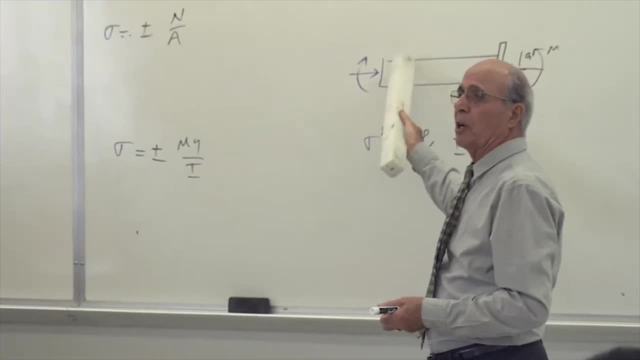 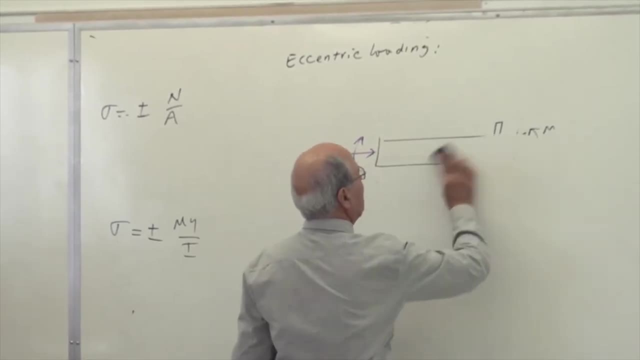 don't know whether, because maybe if I jump suddenly into do I do not explain all of that, You will not get it right. Is that understood what I'm talking? So let's go to a couple of examples Now. the examples are now very simple. Now we 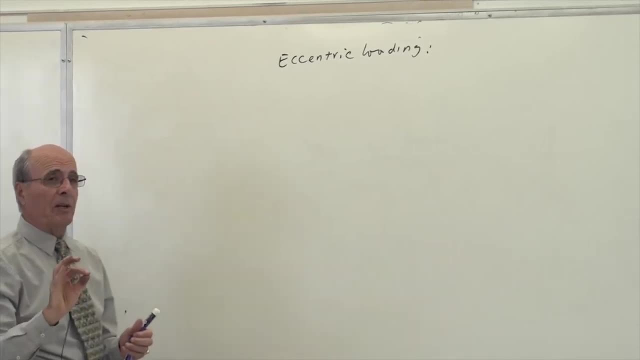 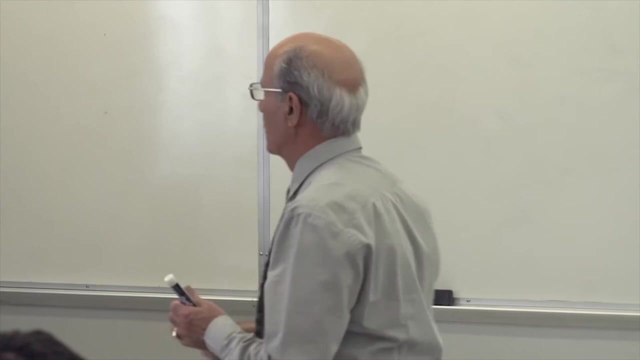 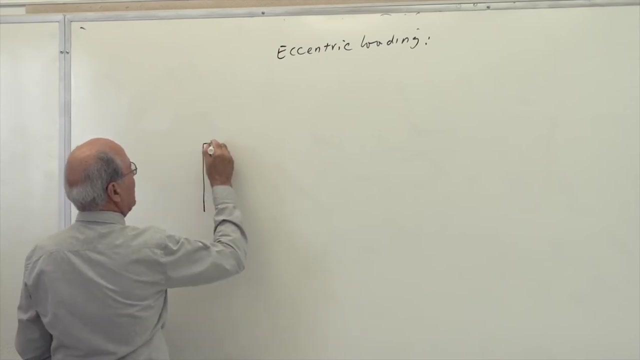 are talking eccentric loading. Now remember all the aspects of that. Everything should look what I said. Everything should go to there: Centroid, yes or no of the cross section. So here it is. Here is a clamp type structure, So here it is like this. So we have this Symmetrical again. This is. 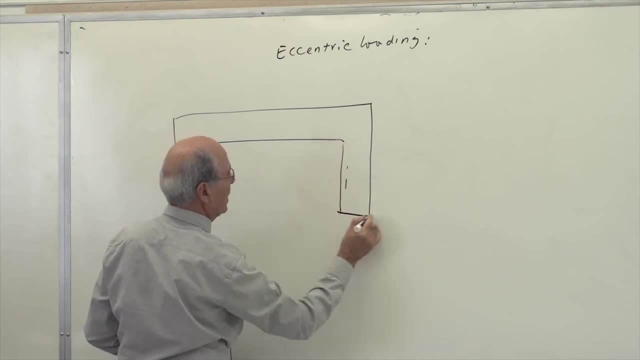 symmetrical, whether it's the same thickness or not. That. And here we put in the cable, here We put it with a force. here We have the force. here This force is given equal to 500 pound, I believe. Let me get my numbers so we know we are. 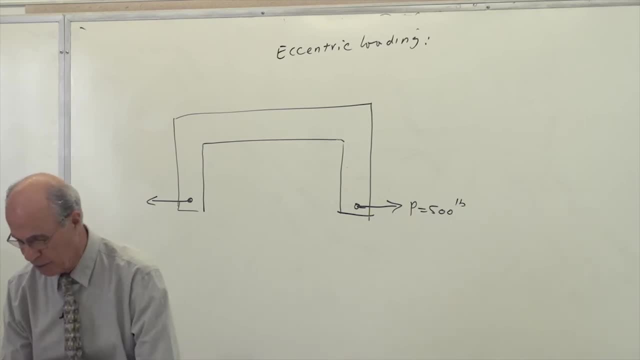 talking about the same question. So we have finished this. we have finished this. OK, 500 pound force is given there. So, OK, the distance from here to here is 2 inches, Let's say. I ask you to calculate the stresses at point A and B in this. 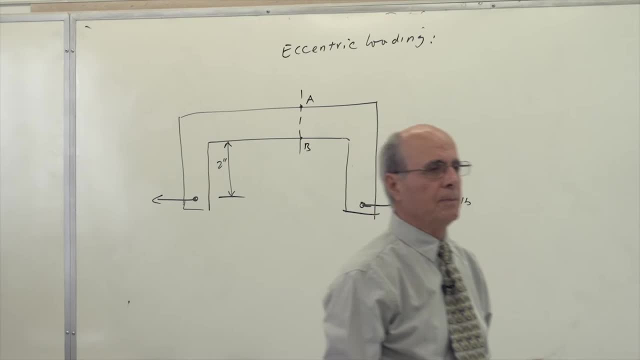 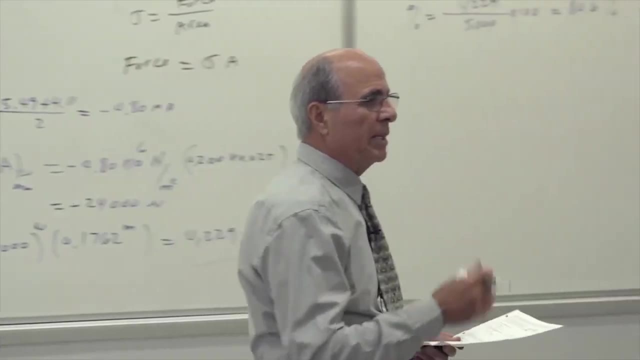 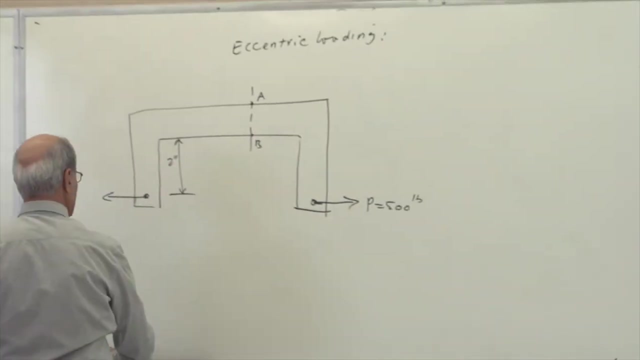 section here, Finding- that's the question. the stresses at point A and B, somewhere between the two, because it's the same, doesn't make any difference. OK, And now the cross section there. the cross section of that part is something like this: Everybody, it has a height and it is a thickness. the 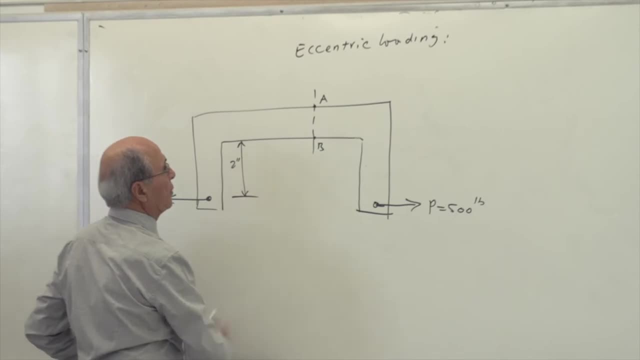 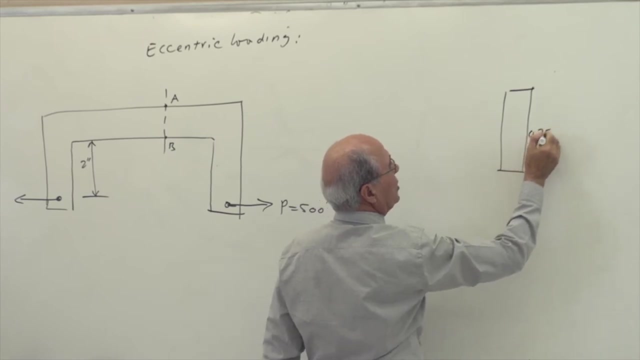 thickness. you don't see. Is that correct or not? Yeah, So therefore, is the blade. so, in other words, the cross section is 0.70 or 3 quarter of an inch by half an inch, maybe a little bit wider than. 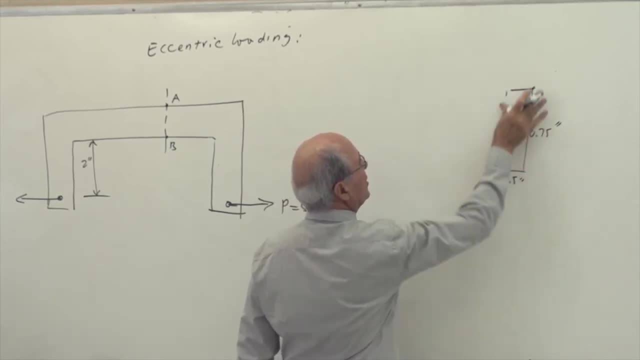 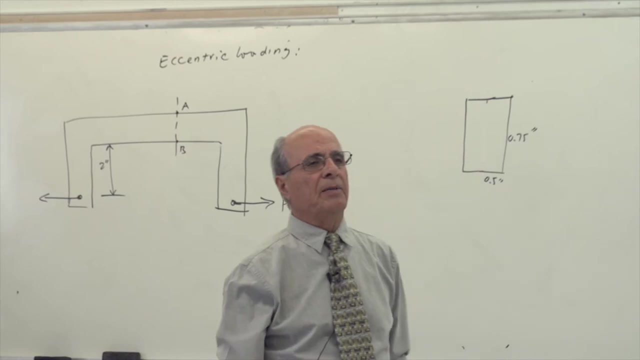 that Should be wider. if that's the case, 3 quarter of an inch by half an inch. Is that correct or not? Yes, How do we do that? The first step is the static. I just told you the problem is with the static. people are reluctant to draw free. 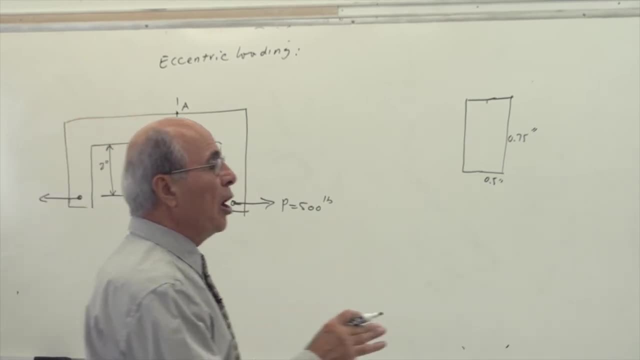 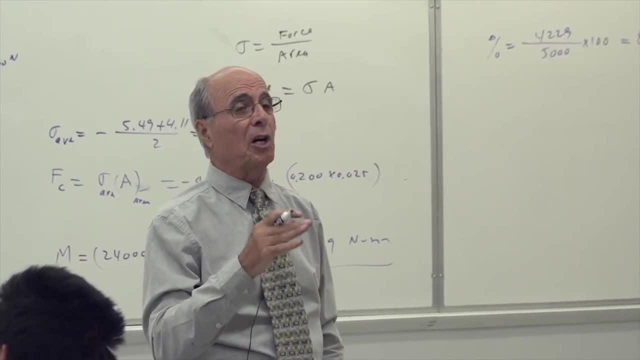 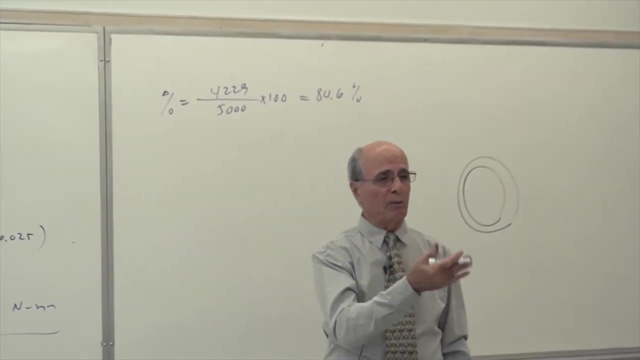 next, which is funny at the same time. but you will be surprised how much progress we have made. Look, let's look at this. every day, every you are driving to school or coming, we are one way or another. you are seeing all the traffic. 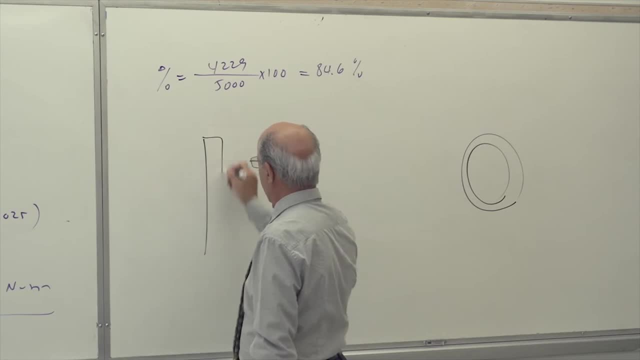 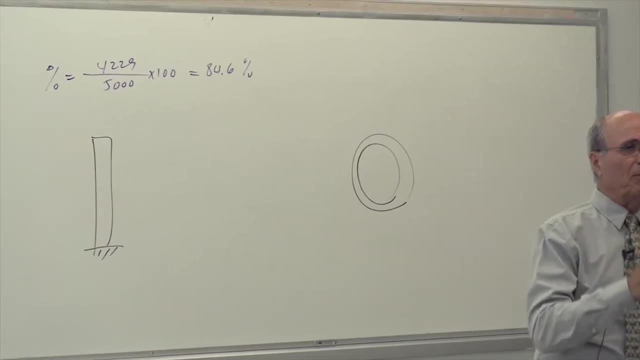 light, Yes or no? Let's look at one of this traffic light. I can give you at the end this problem, which covers chapter 1 to chapter 7, maybe even more. Is that not correct? One problem only. Look what happened there. There is a light here. 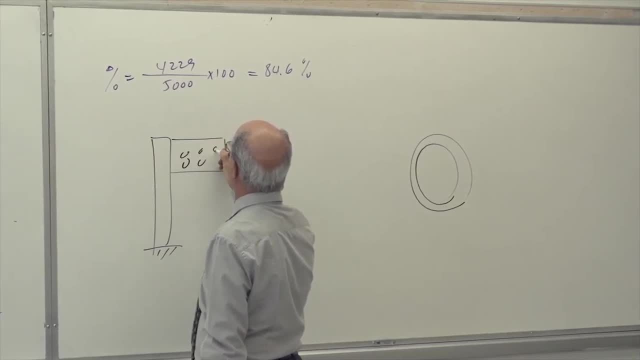 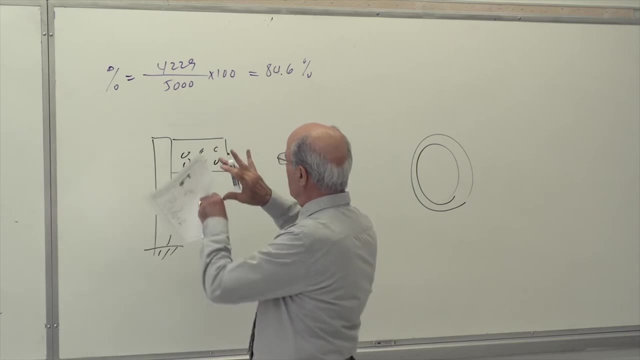 this way, this way, I don't know how the light here. OK, Yes, This has a weight, correct? You don't have to write anything down. And then the wind blows. this way, we have a horizontal force here. F Yes or no, This is also have a W. Now, when I 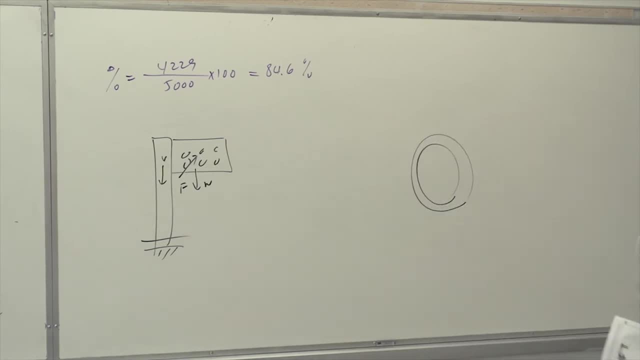 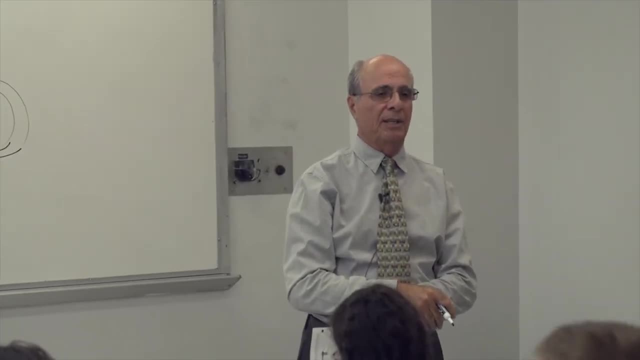 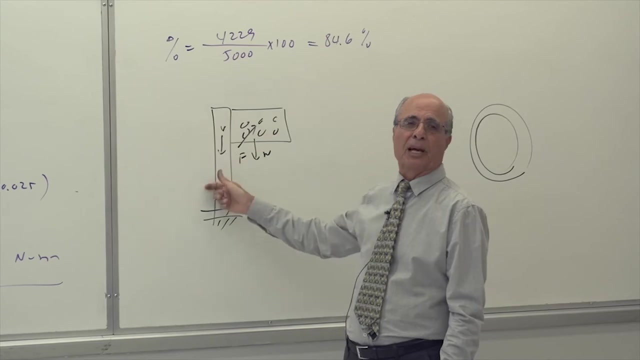 come here. do I have axial force there, Yes or no? This is also have a W Now when I pushing down, Of course it does Yes. So it is chapter one: Does it create this force? Does it create a torsion here? Chapter three: Does it disband this way? 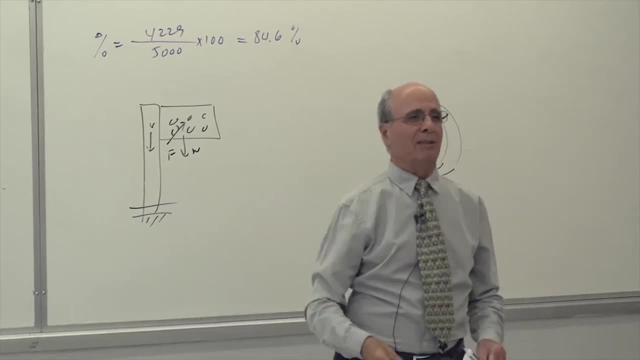 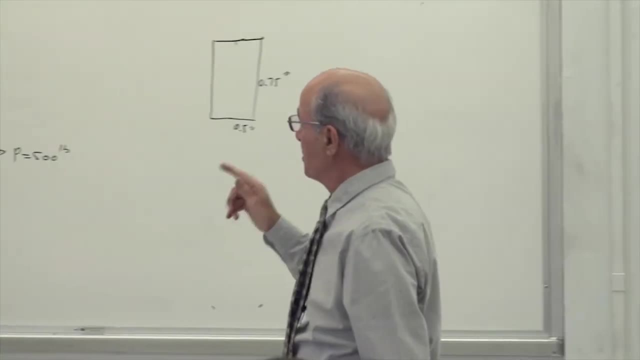 Chapter four. Does it bend actually this way? There's more than even chapter four, So we have to do So. everything that you want to know is happening. that one simple problem. Pretty soon, we are going to put all of this together, So do. 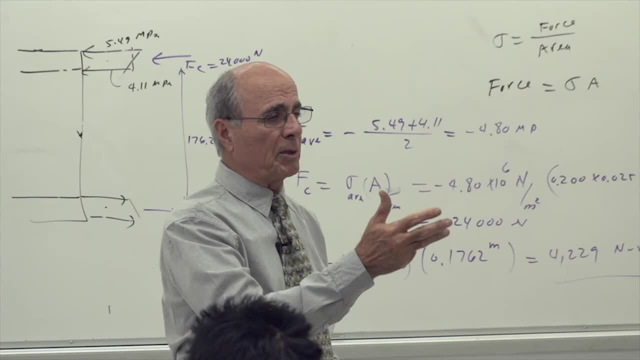 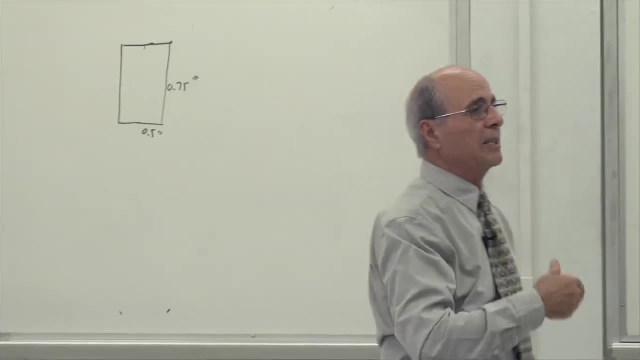 problem like that, Everybody. but first we have to go through chapter one, two, three, four, five and six- Everybody. we have two more chapters to finish all the detail. Chapter seven is all about that and more. Is that understood? Yes, So. 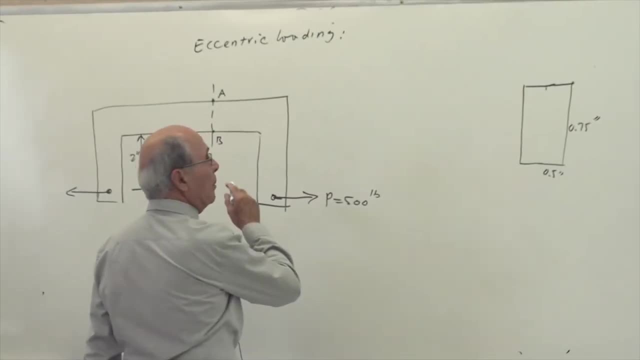 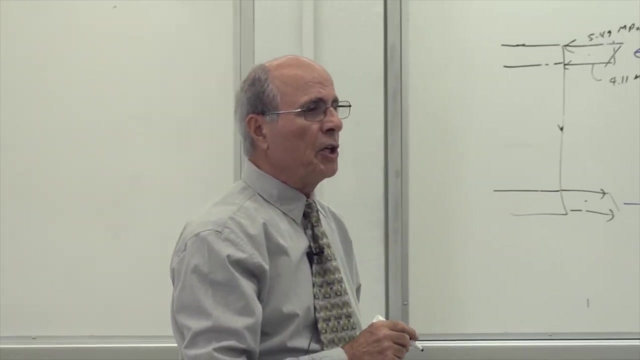 therefore, for the first time, we are combining chapter one by chapter four. Did you see the equation I gave you? One was sigma equal to what P over A. The other one, sigma was equal to MC over I. They are from the same type. so we have. 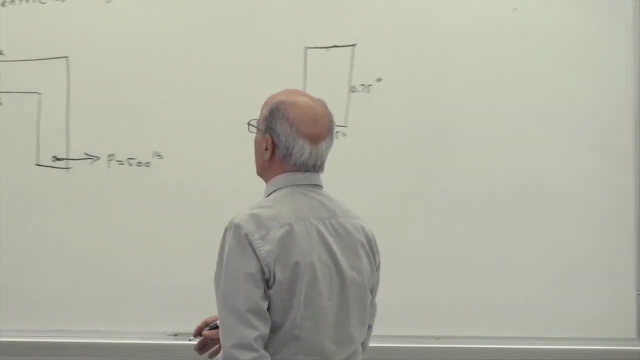 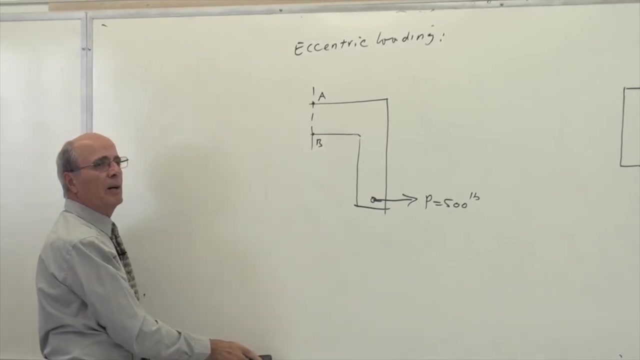 to add it together. Is that understood? Okay, fine, So now let's go here. Draw the free body diagram, So you can draw the free body diagram of the left-hand side or free body diagram of the right-hand side. Where should I put my internal forces now? 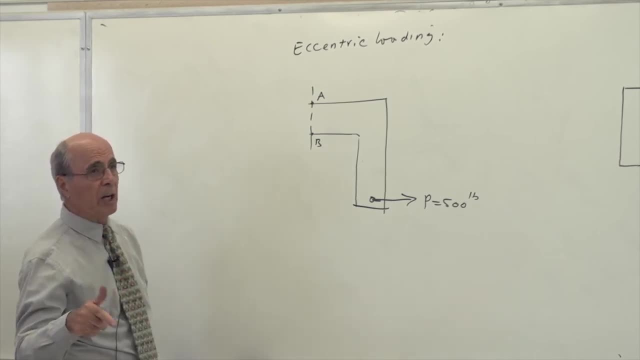 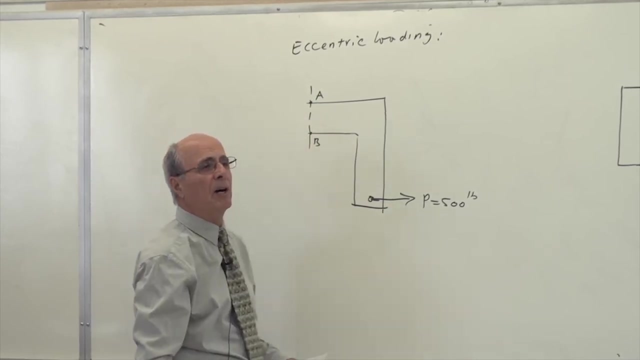 No Many people. when I give this problem, if they don't hear me like this, they put first of all: they don't know. They say: okay, there is here force equal to 500.. Yes or no? In the form of tension or compression? 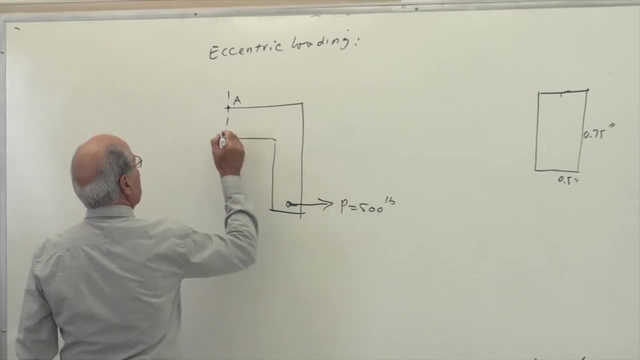 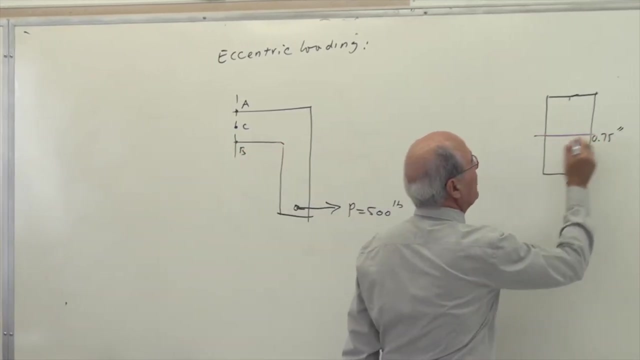 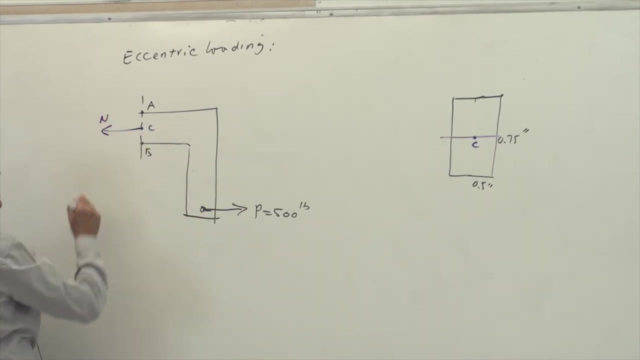 First of all, I should not put it at A, I should not put it at B, I should put that at C, which is the centroid of the cross-section. Is that correct or not? Okay, so I have here a P. going that way, I have to have here a N. The value of N. 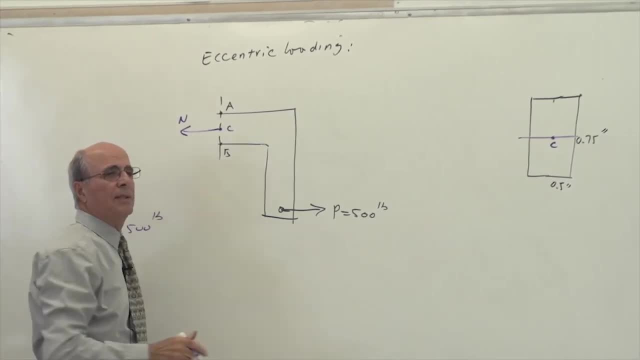 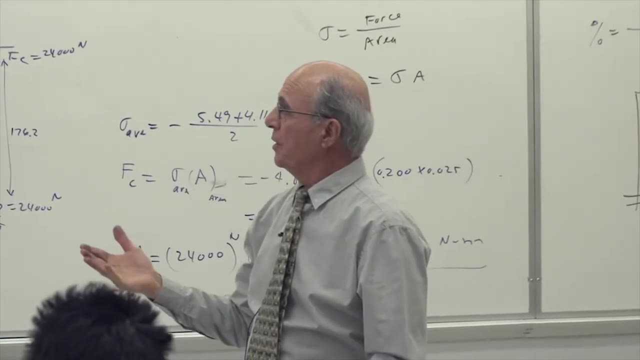 is equal to 500 pounds. This is internal, That is External, Yes or no? So I have chapter one there, Yes or no? Correct Do I have it? Is this: This is the equivalent A couple. Everybody can see that this is already a couple, So this: 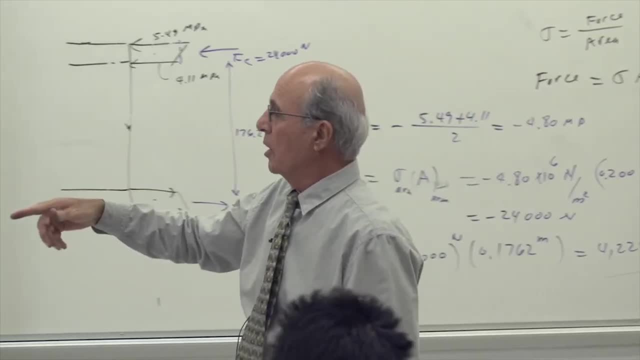 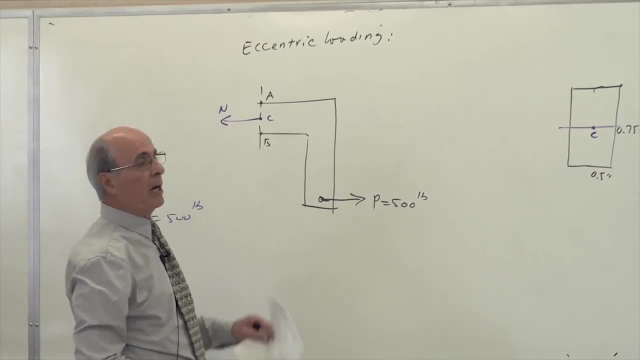 cannot stay like that unless I add a moment. I cannot add a moment here, but I can add a moment into the cross-section to make it in equilibrium. Now, this one, the first one that I show you, was equivalent, But this one is equilibrium. 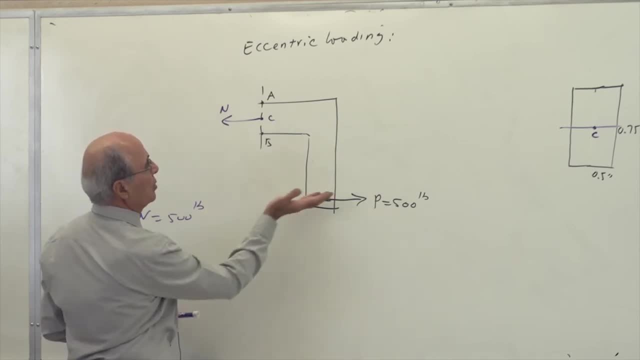 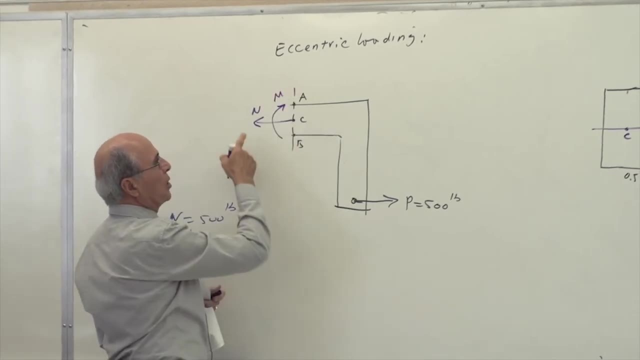 Whatever action you see here, you have to reverse it. So the action is going that way, So the reaction is there, Or you can use any other method. This is your M, because the sum of the moment now about this point become equal to zero. 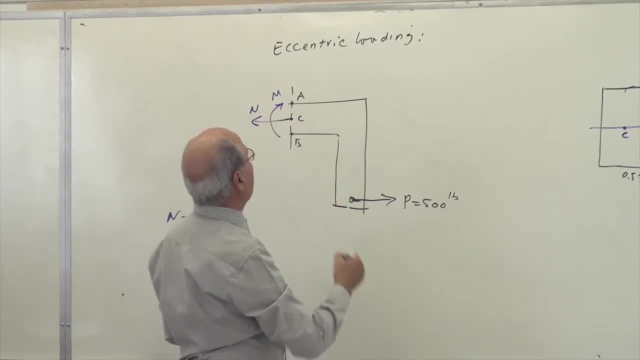 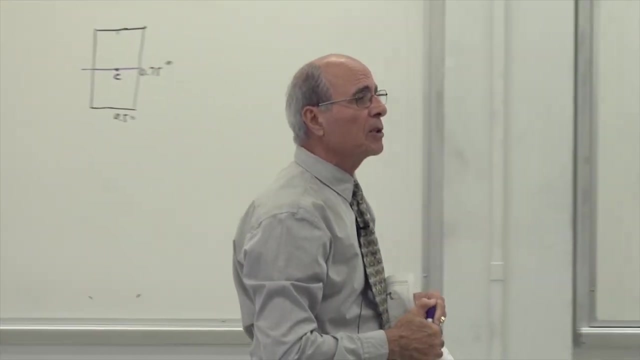 everybody, Because this going over this way, that one over that way And that M equal to what? This is a static part of it. As I said, many people have problem with the static part of it because they don't know. first of all, distinguish. 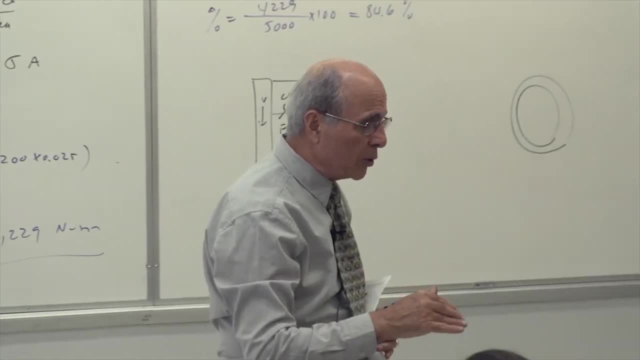 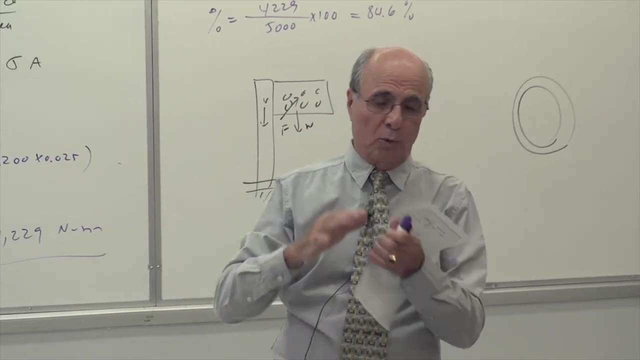 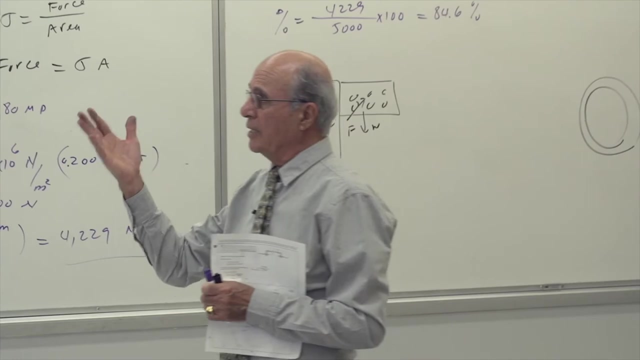 between equilibrium and equivalent. That's the two difference. Right now I use equilibrium. Everybody understand The whole system has to be in. when you do the entire free body diagram, the whole system has to be in equilibrium. That's right. So the action. look at it. If I take the moment about here, for example about 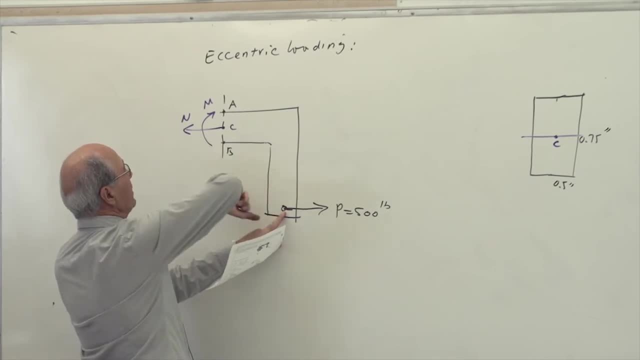 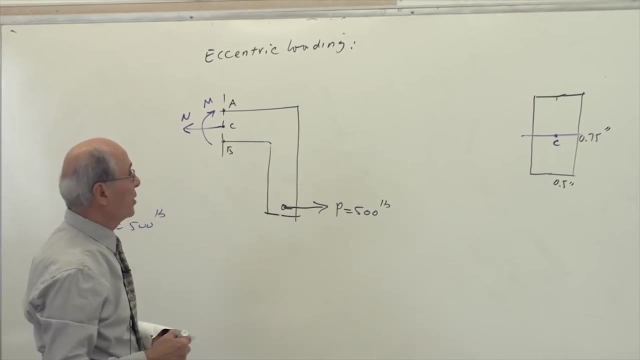 this one. this one has a moment. This moment is positive, This moment is negative. They cancel each other. However, what's the value of M? now? Exactly, You see, Like what you said, That's what I don't want you to do. You said: 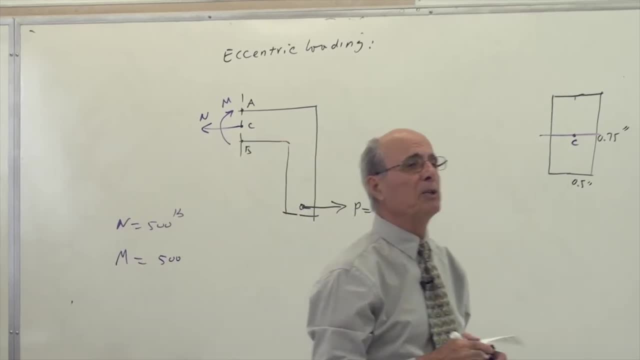 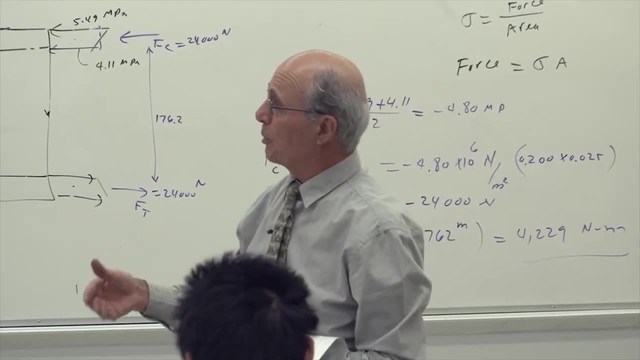 thousand because you multiply. Look at your picture. You multiply it by two, Yes Or no, Correct? If you multiply it by two for point B, what do you multiply it by two and .75 for point A? Both of them absolutely wrong. You should take. 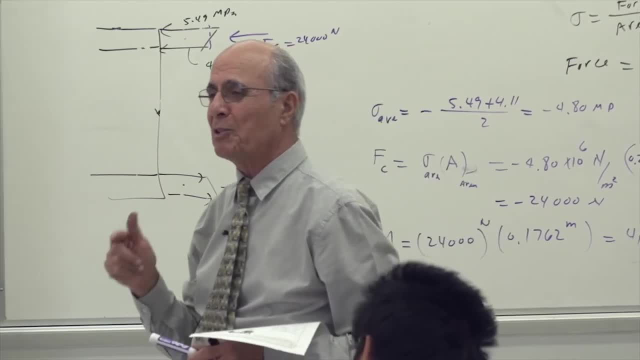 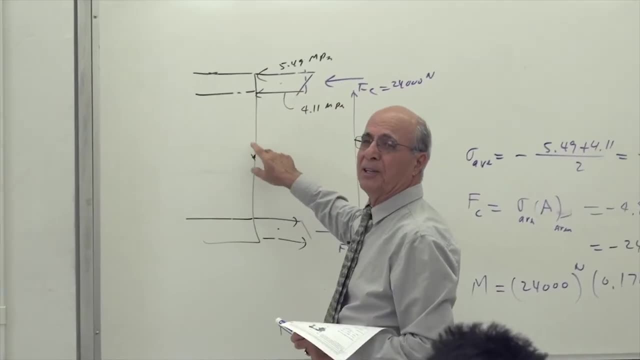 everything to look how many times I'm repeating that You should take everything to the Centroid, Yes or no? The moment, everything that we did here, everything start from Centroid. This is the biggest mistake. everybody makes Point A and B. 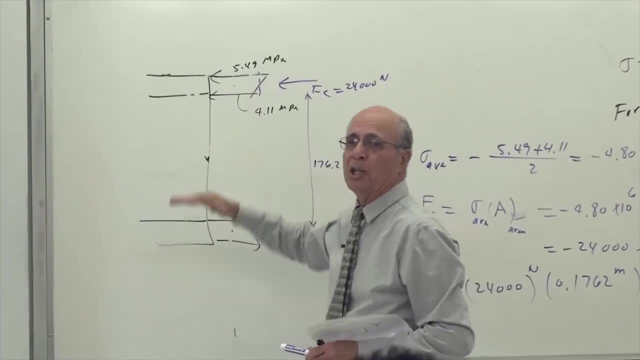 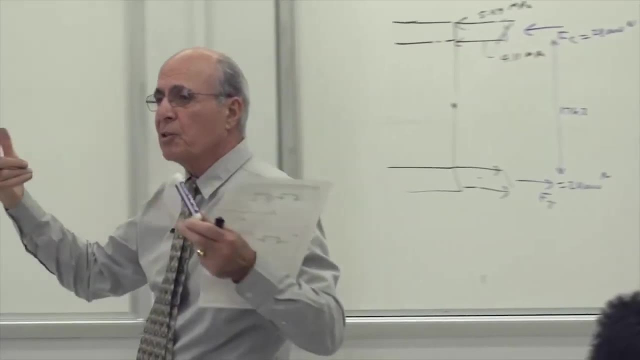 Point A and B has something to do with the distribution of the stress. You should move it everything to center. I said many times we showed the beam as a line. That line is the centroid line. Is that correct or not? So what should I? 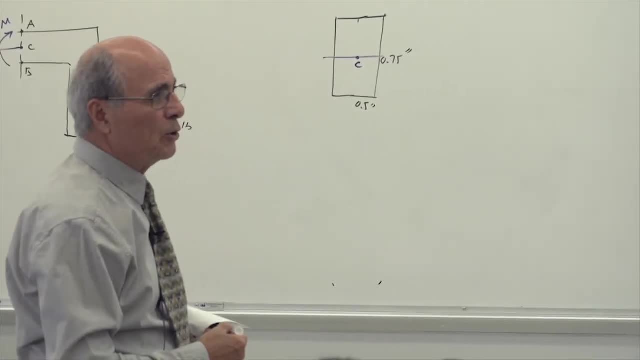 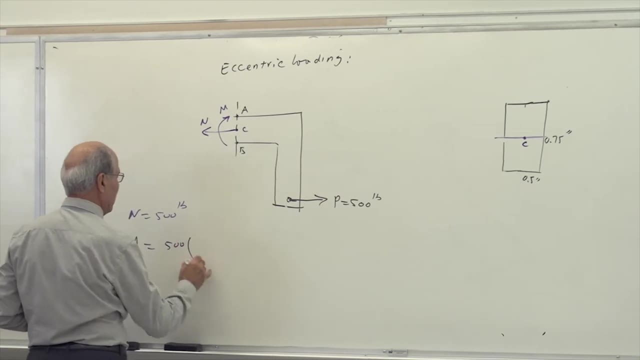 multiply that 500 by Two, plus what? Half a distance. That's right. So please do not make that mistake. That's exactly the one I don't want you to do. Time two inches, because from here to here it's going to be the same, It's going to. 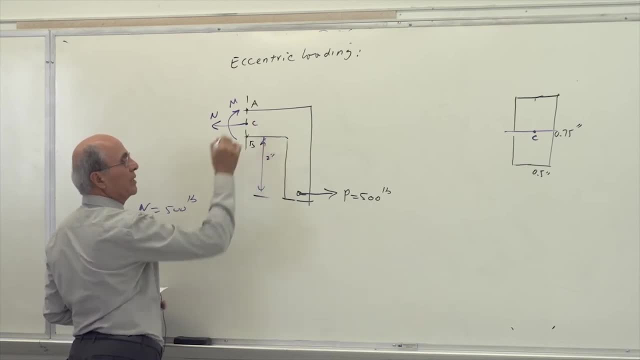 be the same. Mine is a quarter of an inch, So the one to here is two inches, correct. then I have to add this much to it. So, because we are taking moment about C, remember that which is the centroid. So two inches time plus .75. 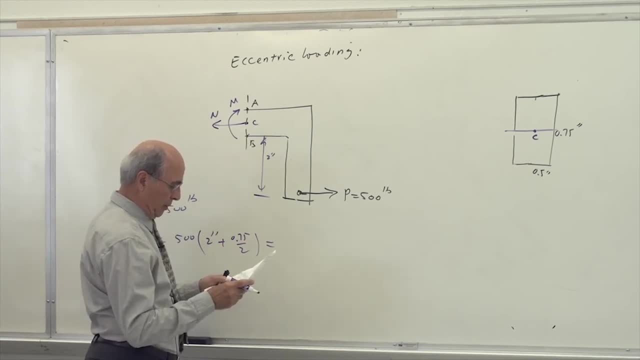 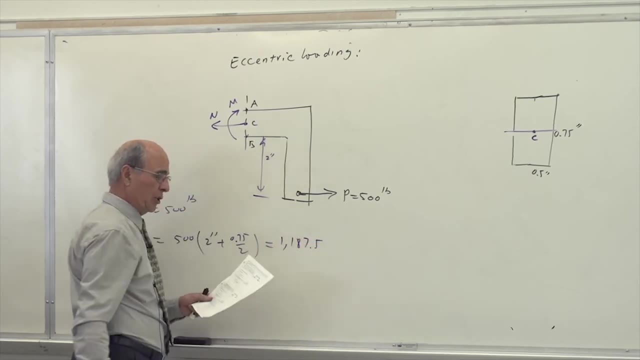 divided by two. Okay, great, So we did that part. So that become equal to the moment, become 1187 and half. I can reduce it to less digits if you want to, But that's the way they did it here, So I keep it like that pound inch of moment. 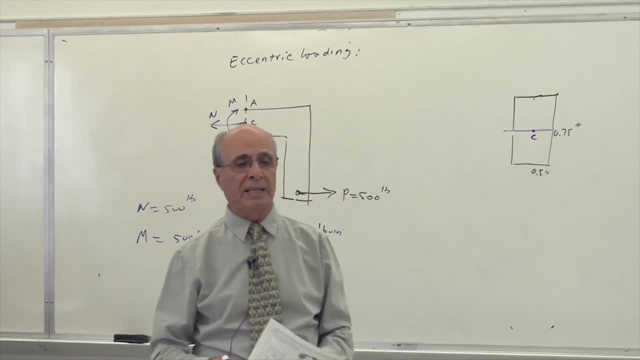 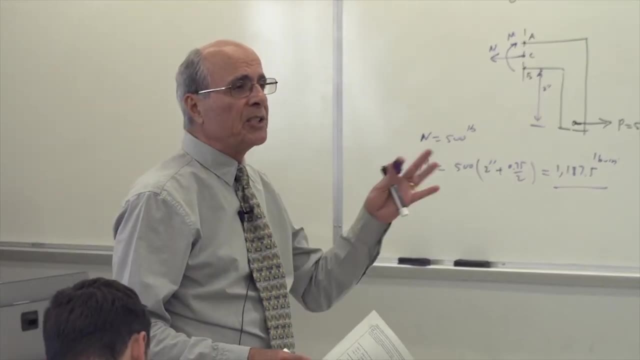 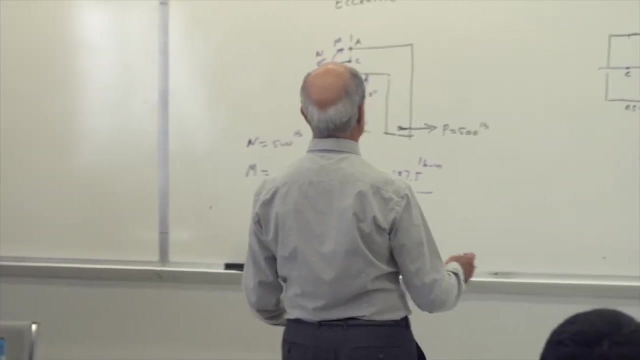 very important key. I hope that you do not make that mistake. Point A and B doesn't matter. You have to move everything to the Centroid. In other words, the system doesn't work for every problem. from now on, Is that understood? Yes, Okay, so now the system become very simple. 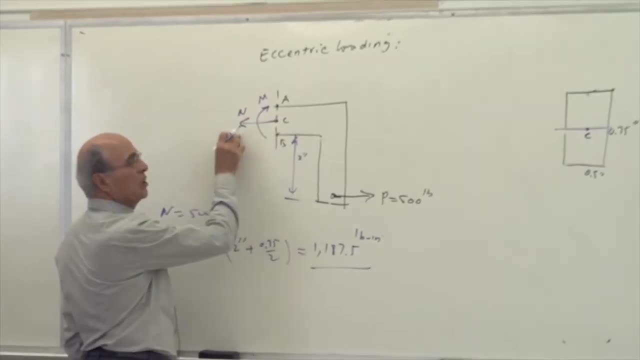 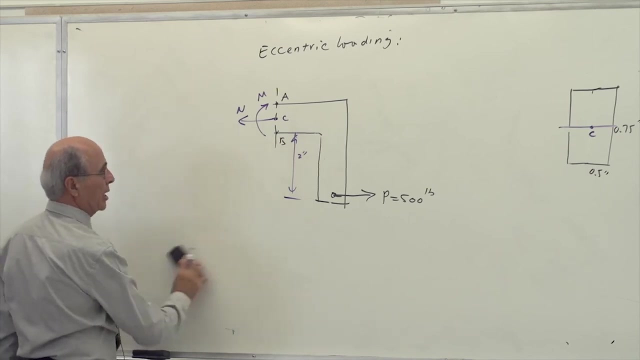 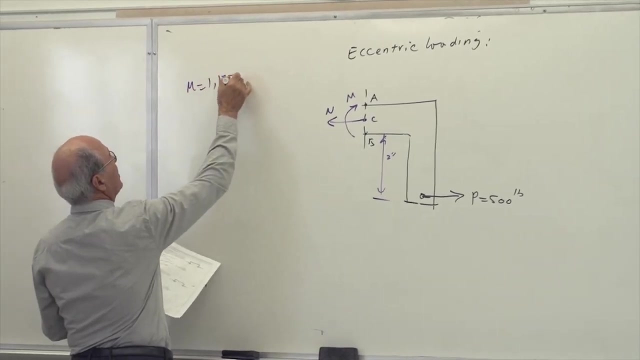 Now I have this much moment, which is chapter four. I have this much force, which is Chapter Again. now for point A. What do you think for what I'm going to erase that? do all the calculation here underneath here? So let's say M was equal to 1,187.5.. Rewrite it. 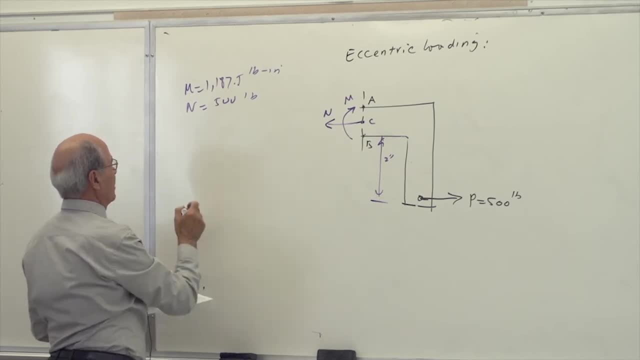 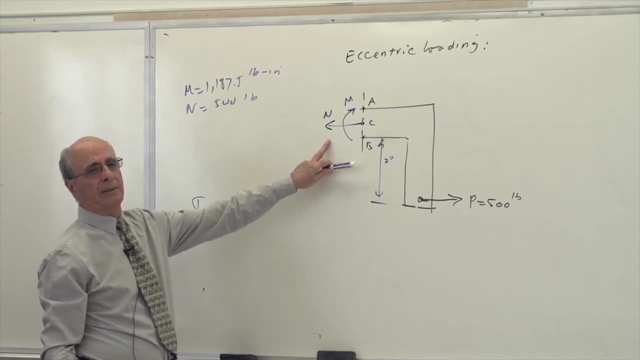 there, But okay, so here it is Sigma A. So can you see it? or should I give more explanation? Sigma A due to this. Is it tension or compression? Forget about it. Look at this one. This is chapter one. Due to this, it's purely tension, Yes or no? 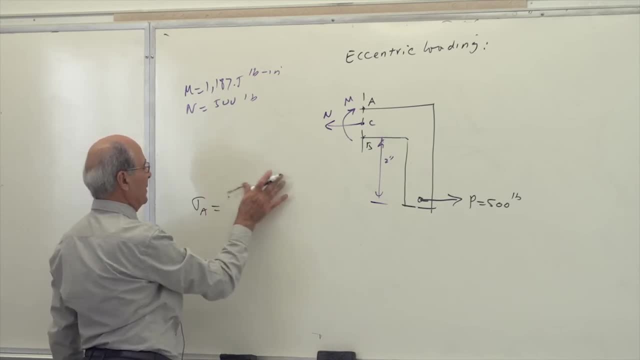 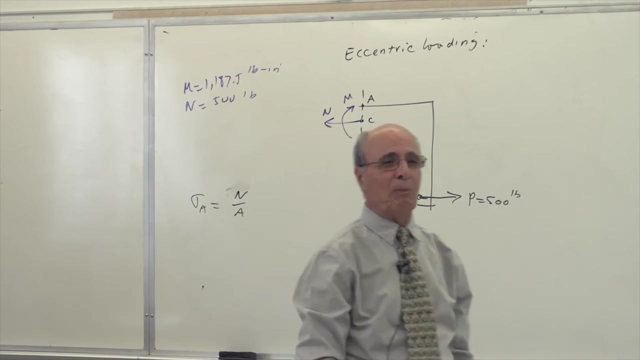 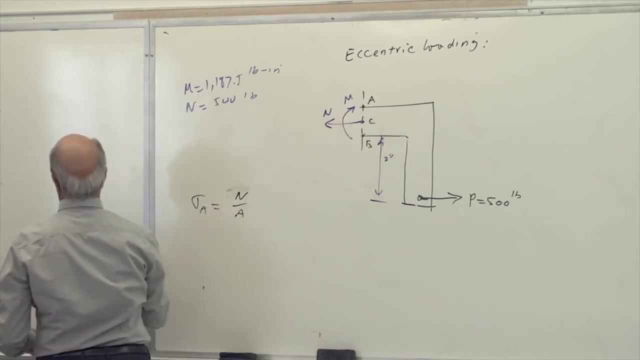 Yes, So it is P over or N over A, correct, Because of the bending. is it tension or compression? Look at the head of that. Which one is compression. Come on guys. Compression, Yes or no? Yes, It's sitting there This. All right, guys, I don't know what to do with you, guys. Anyhow. 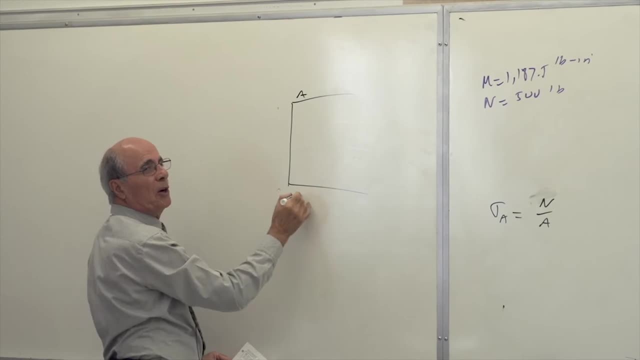 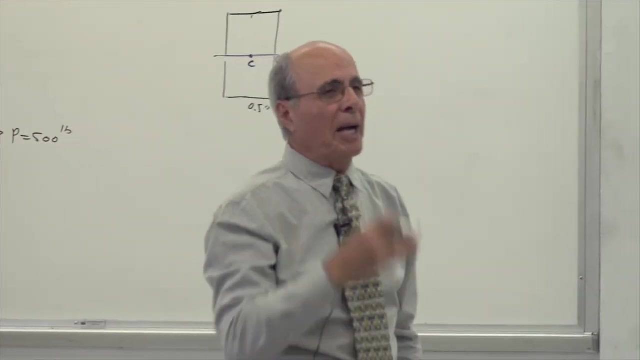 this is chapter four. Chapter one, Yes or no? This is point A. This is point B. You have a force there. You always thinking of force. I ask you not to think about the force. Think about the stress, Yes or no? The stress is uniformly distributed from top to bottom. Exactly what I ask you. 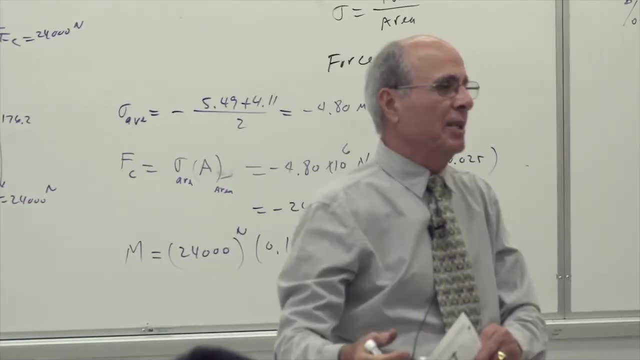 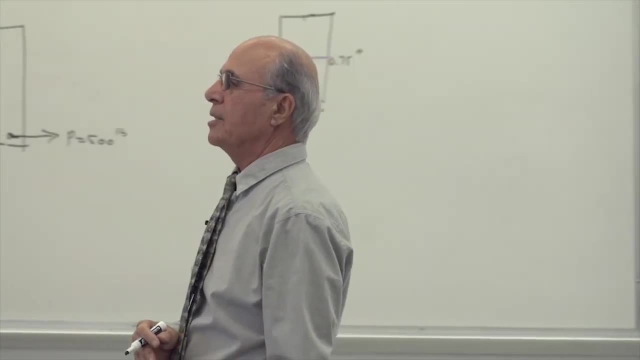 not to do. Forget about the formula. Think about the stress distribution, Then everything will become resolved, Yes or no, That is, stress is due to the P or N, P or N. Is that correct or not, Doesn't matter. On top, bottom, center, everything is uniformly. 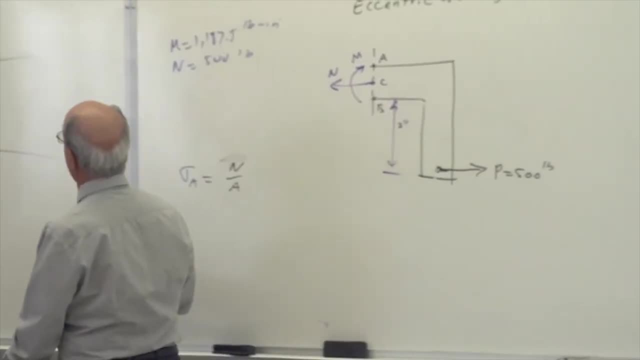 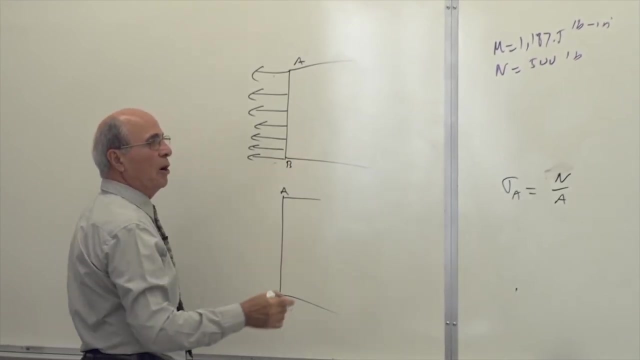 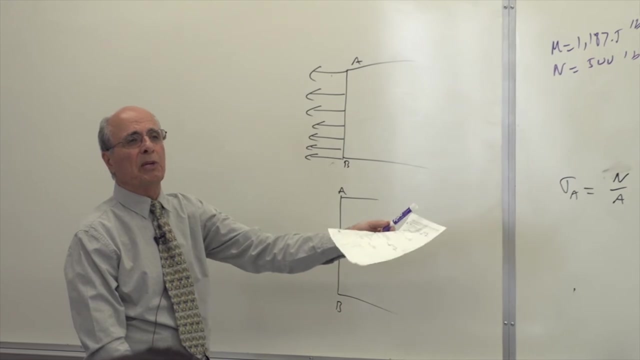 distributed stress. Then, at the same section, I have: this is the same section, This is again point A and this is point B. What do I have this time? I have a bending moment. I already, we already know that. So let's put the two and two together. What's the effect? 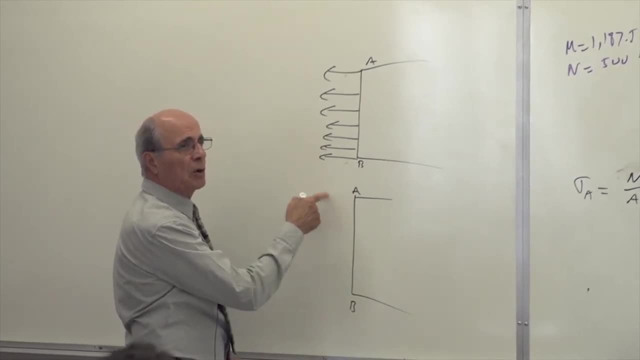 Which way the bending goes. The bending goes like that, Yes. So here is compression, Here is Compression. Compression is this, which is a little bit larger, because we'll see the- and this is the tension, Yes or no. On the centroid, the stress is: 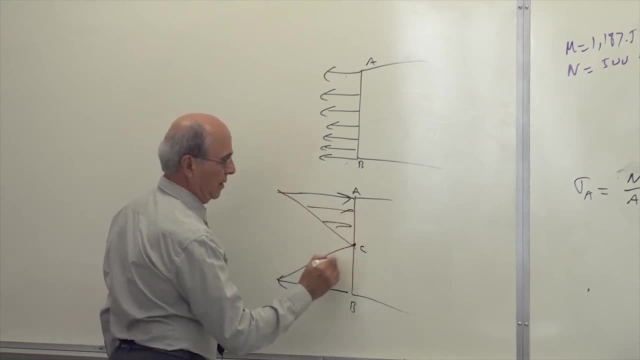 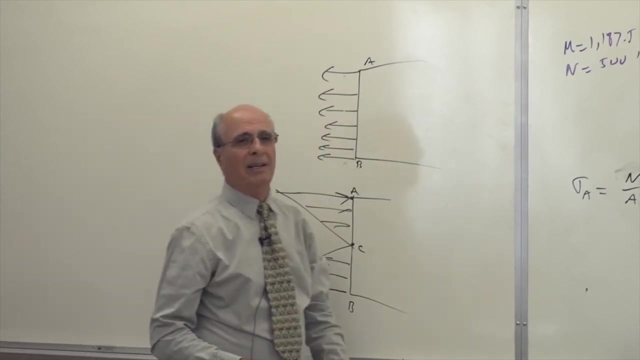 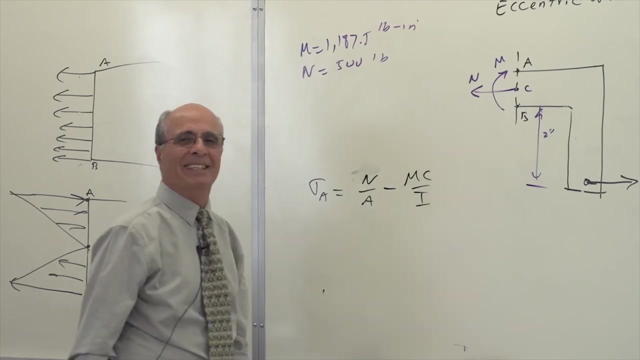 Zero, Zero. So therefore, this is it. What stress do I have at A Plus N over A minus MC over I, Yes or no? Come on guys. Okay, Yes, Some of you are still not happy. I can see it there. 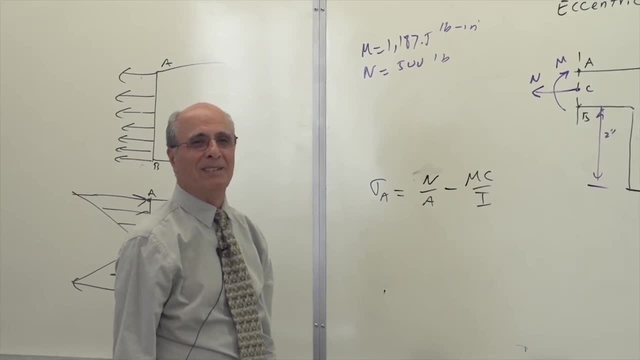 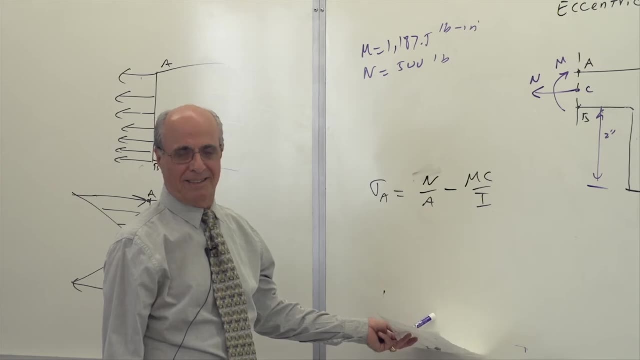 I can see it right in front row. Okay, Not looking at me, The person in chat. Okay, Did you get it? Yes, Yes, Good, Okay, Sigma B, then what? because sigma B equal to, Sigma B equal to. 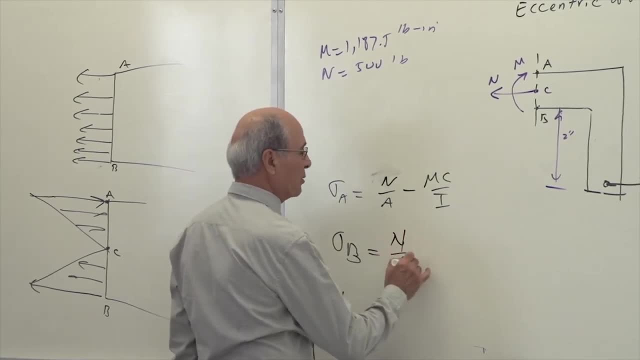 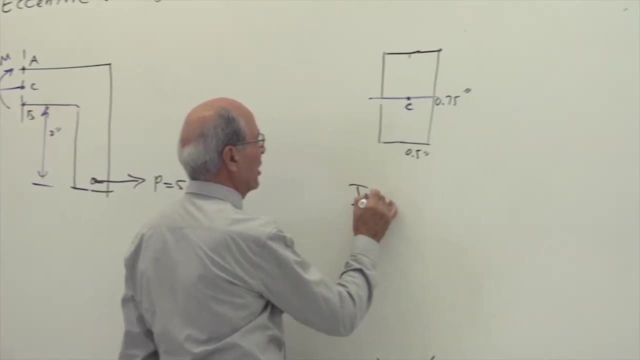 N over A N over A. Good, You have to write it your own. Then what? Plus MC over, Plus MC over. That's it All I need now the I of this cross section. I of this cross section. 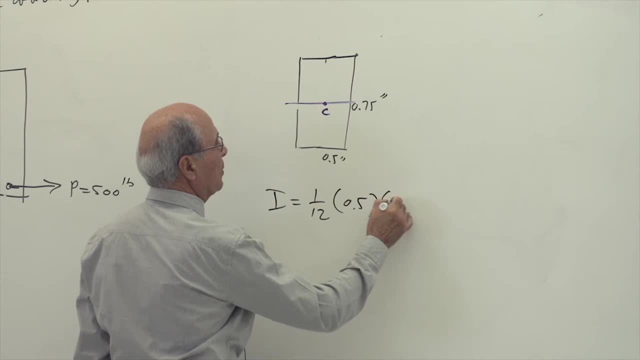 is 112 of 12, of 0.5 times 0.75 to the power of 2. Area I need, which is 0.5 times 0.75.. I leave the rest to you because that's the number. we have done it many times. Is that correct? I give. 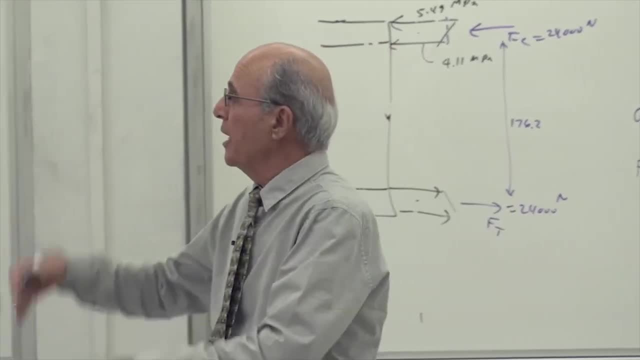 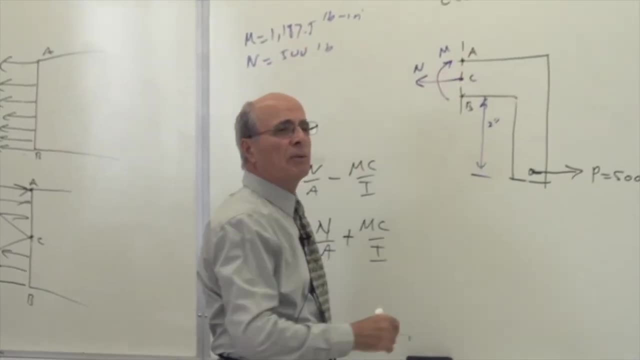 you. the result Is that understood? I is there, A is there, M is there, N is there, everything is there. Is that correct? And the C, of course, is The C is the half a distance from the C to the top. We already know about that. Is that correct or not? Yes, So this one. 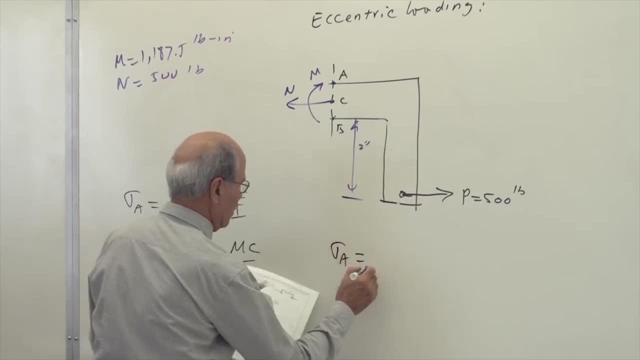 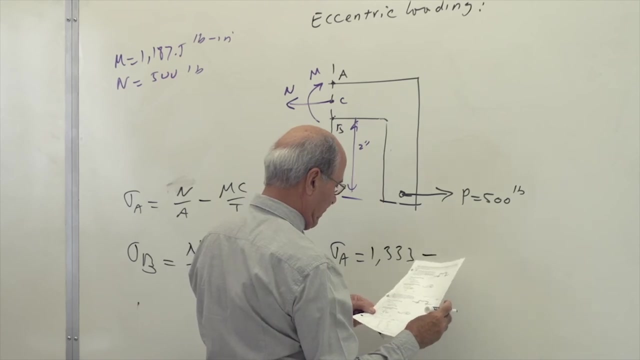 let's write it down. So this one sigma A, Sigma A, become equal to 1,000, as I recall. so it has become 1,333 positive PSI And minus, because this is repeat, minus 25,330.. This is much larger than the other one, for this. 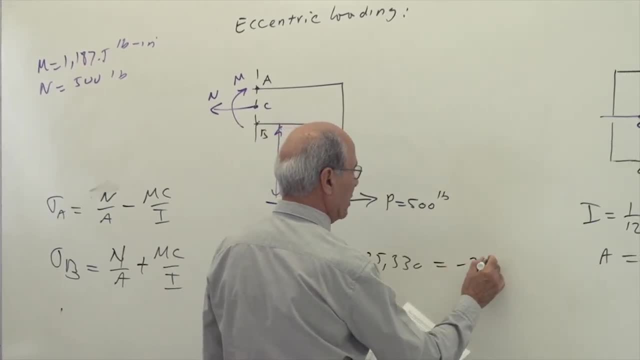 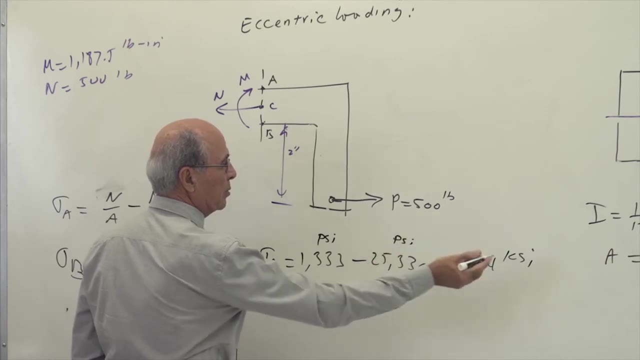 problem. So it ends up to be equal to minus 24 KSI. So on the top, of course, this is PSI. I want you to read it out. I'll change it to PSI 24,000.. Because 1,330 of that and that one drops out, There is 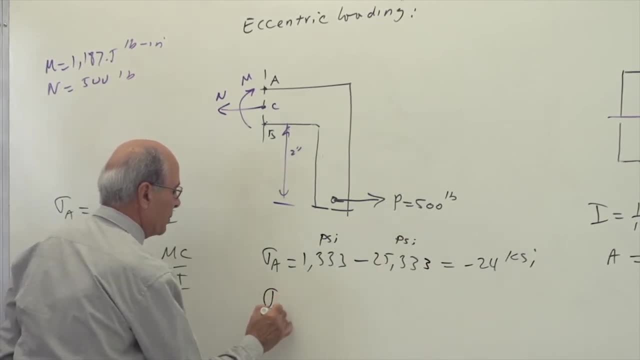 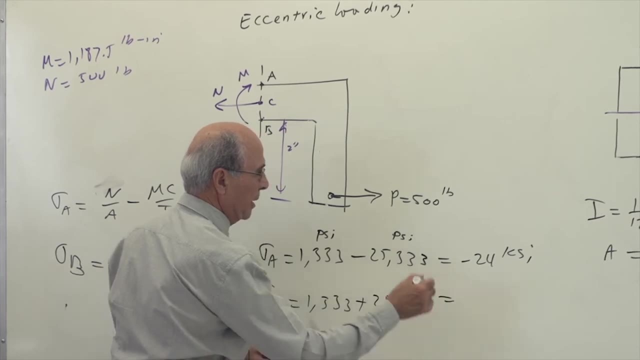 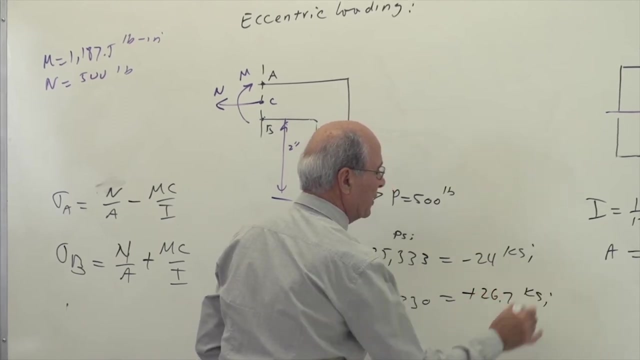 a three here, if you want to be exact, And the other one, sigma B, become equal to 1,330 T plus 25,330 approximately, So that one become equal to plus 26.7 KSI. So that's the combination. of the We have for the first time we have an eccentric load. So that's the combination of the We have for the first time we have an eccentric load. So that's the combination of the We have for the first time we have an eccentric. 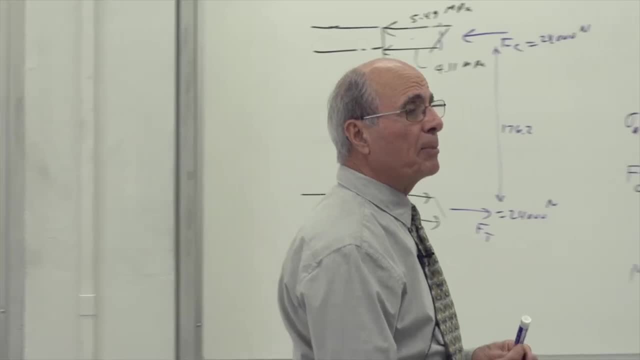 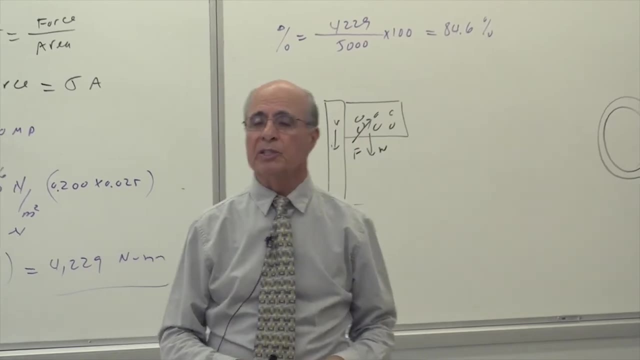 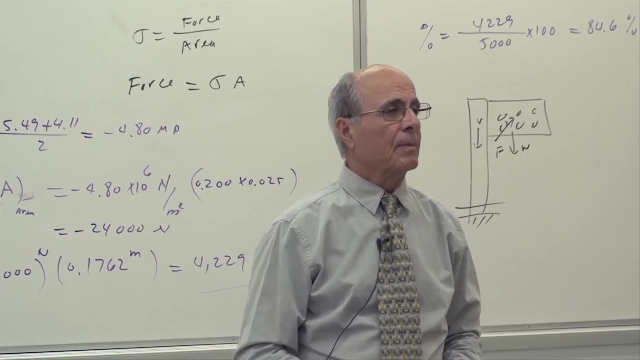 loading And eccentric loading is the combination of chapter one and chapter four. Here it has the chapter combination of all the chapter together, which we'll talk about it later on. Is that understood Now? what's the sigma at the centroid? What's the sigma at the centroid? 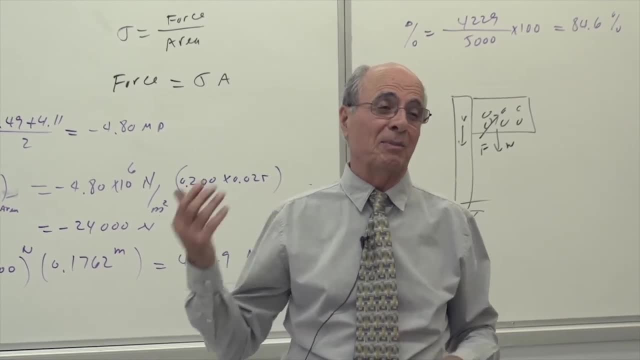 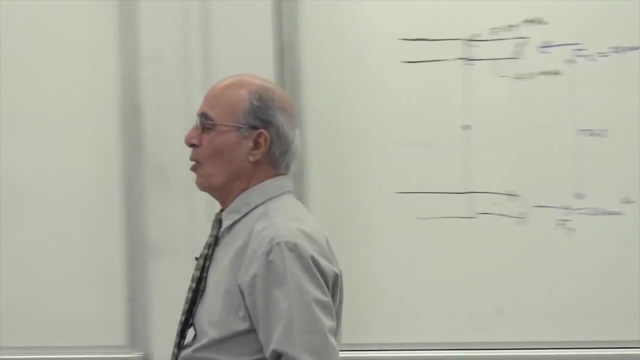 Zero. You see many people, is the sigma at the centroid zero? Look at it, Look at the picture. Is the sigma at centroid equal to zero? No, That's exactly my point, Because, just before you answer, think, think, think This. 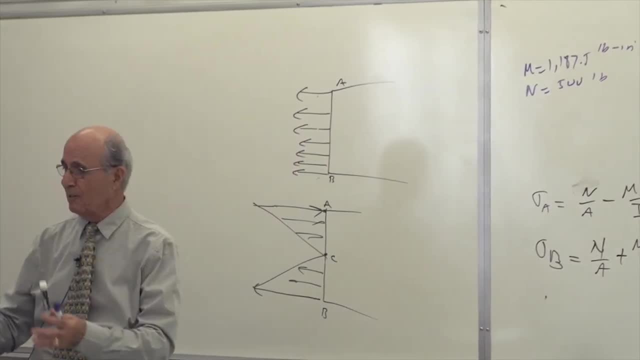 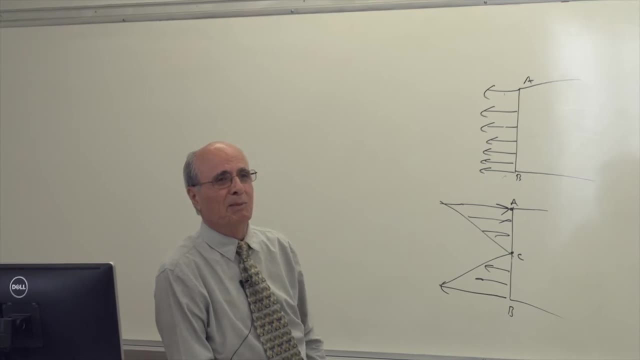 is what? when I was in IBM, working for IBM, everyone in front of us we have this sign and it was saying: think, think. That was the load, But at that time you weren't bored, so you don't know what we were talking about. At that time, computer was a huge computer. 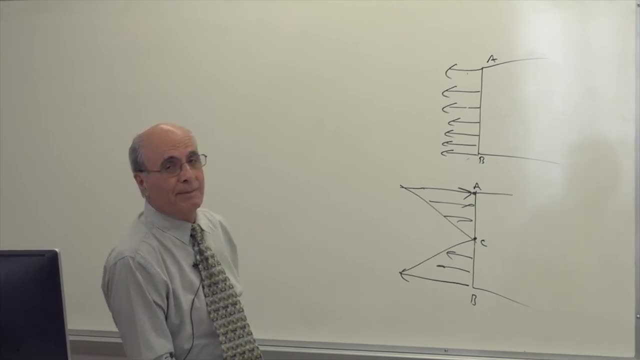 with little memory, Is that anyhow? So punch card, We have the data We have to punch card and then put it there, push it there. Tape, Tape was coming out, all those tapes In the old movie. you'll see it Anyhow before. 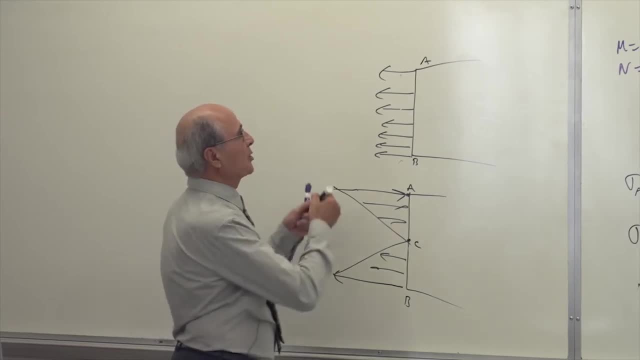 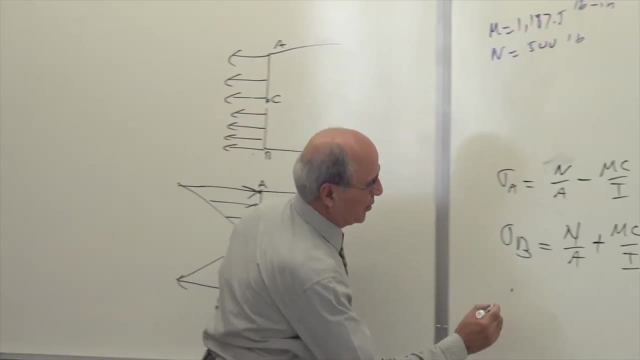 you do saying anything. think about this. Is that correct or no? What's the stress at this point? C, Here is Zero, Here is Okay, Glad, Okay. Sigma at C equal to N over A, Because you have it zero if it is moment. 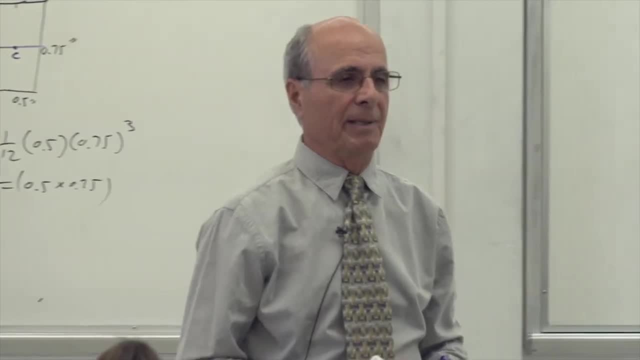 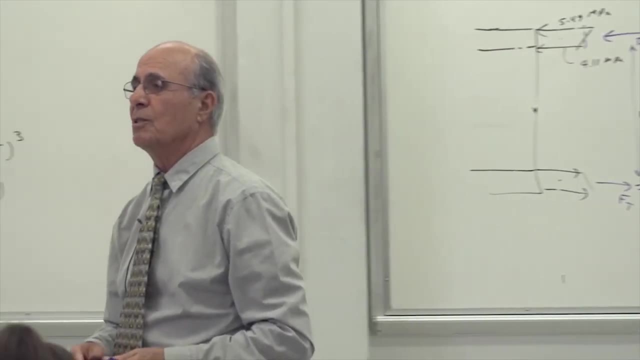 You were right. in a way, It was moment only. Is that correct or no? But it's not the moment only, It is the combination. So can you tell me where the stress is zero? I don't know. Okay, That's the question in the quizzes: Can you find where the stress is zero First of all? 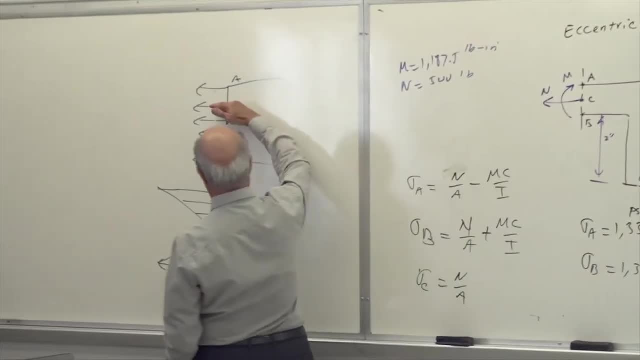 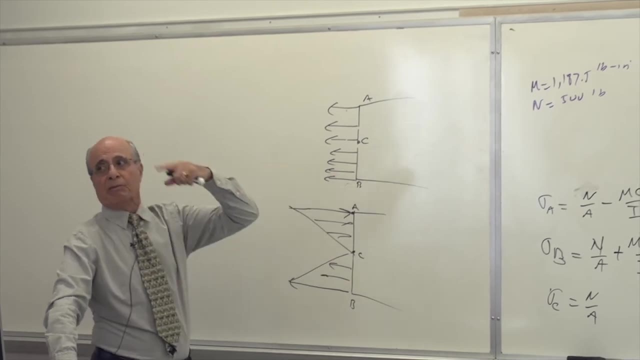 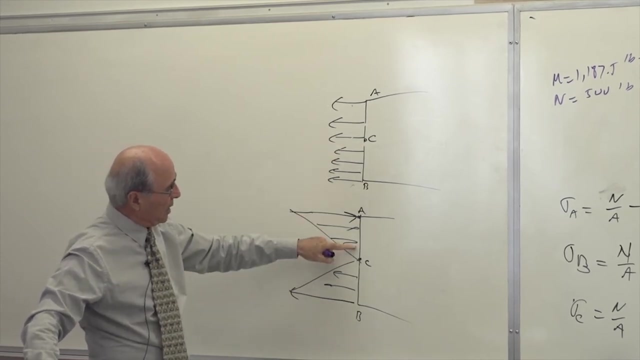 let's say that if this is the section the stress zero is here or here, Lower than C, or upper than C, Upper Upper than C. Absolutely correct. Why? Because they have to cancel each other. Everybody understand. You have this much, 1,300.. You have to go up here to get. this is the tension. 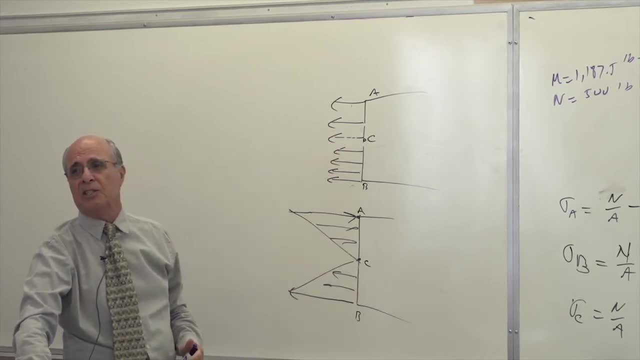 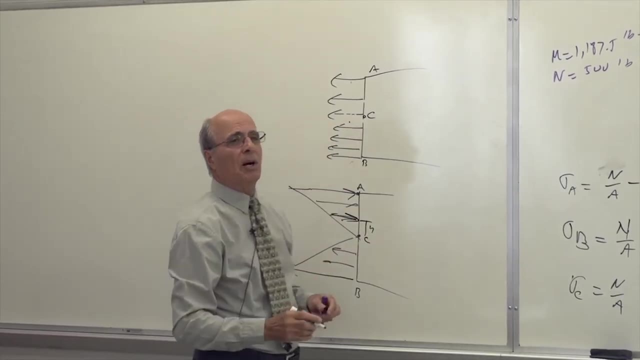 You have to get that much compression. The two together must cancel each other. yes, So actually this becomes a generalization. Yes, This is a geometry problem. How much? why should I go there that this sigma and this sigma become equal, the sum become equal to. 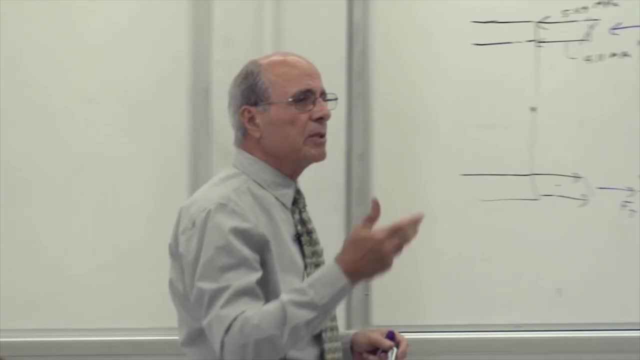 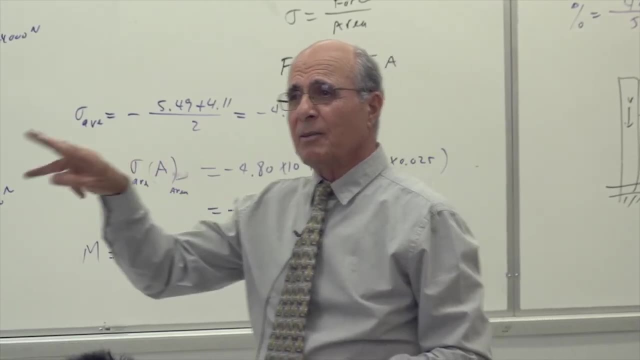 Zero, Zero. So you calculate the location of the Y Or you can use similar triangle geometry. Is that understood? I have asked that question before. Just to throw in for two, three points at the end of the final to see the difference between you guys. Different A and A minus. 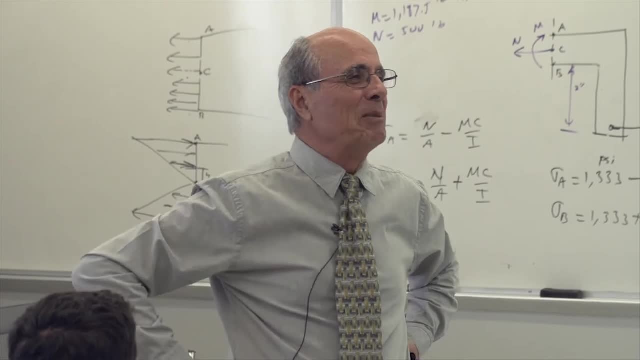 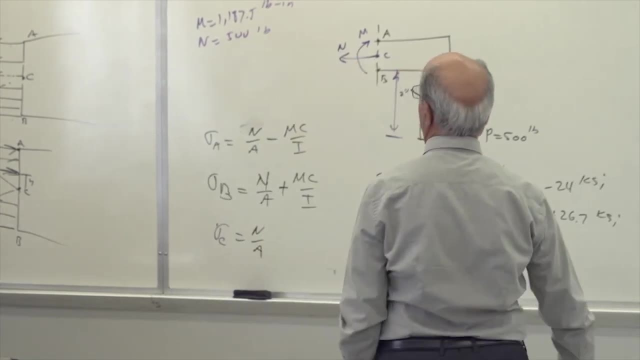 So let's put it this way: Everybody see what I'm talking about, Because you're going to get the same thing. Yes, Yes, You understand what I'm talking about, Because it's important to understand what we are talking about. Is that understood? Yes, Since the stress here is, some of you are still looking. 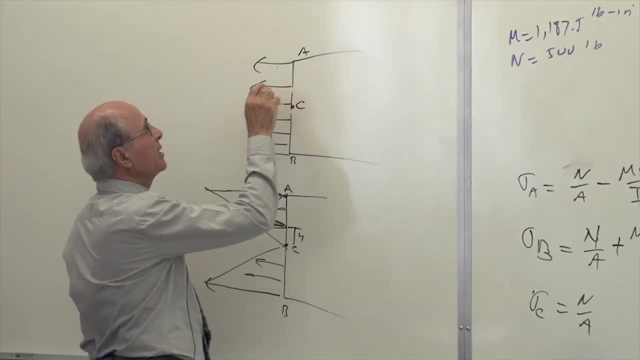 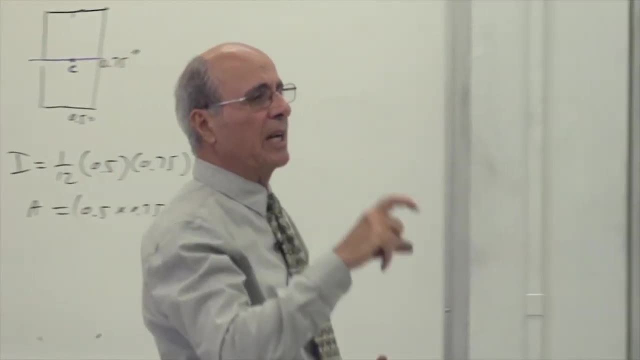 zero. Therefore- and this is the tension, So I have to go higher here to get this tension and this compression cancel each other to sum become equal to zero. Based on that, you can calculate, because it become MY over I. So you calculate the value of that, Or you. 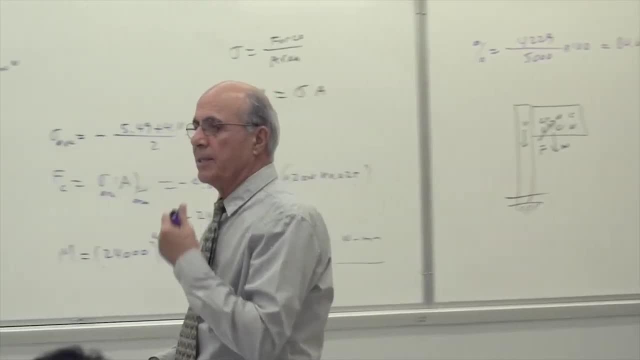 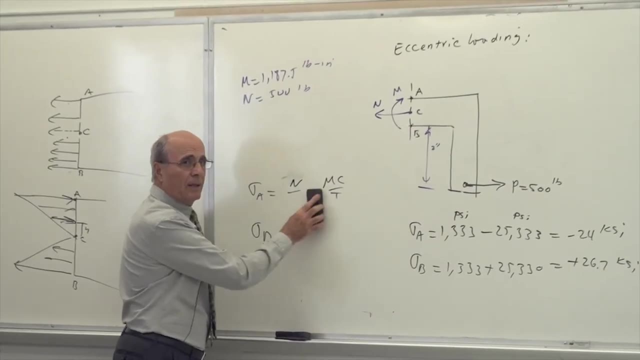 can use the similar triangle to get that height. Is that understood? Because there are two triangles. Now there is one more problem I want to discuss. How much time do I have? Eight minutes, Eight minutes, Good, So I have enough time to discuss a few things with you. 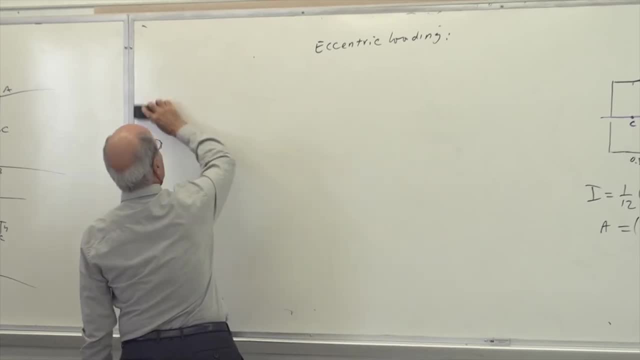 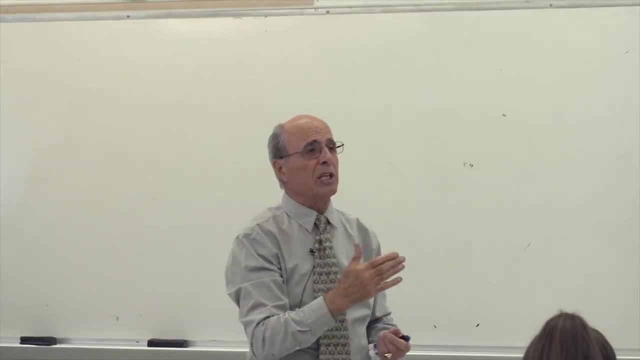 Now there are a couple of homework given to you that the student usually panic when they look at it there. Many of them is at that source, So all you have to do go to the cross section in question, draw your free body diagram, find the 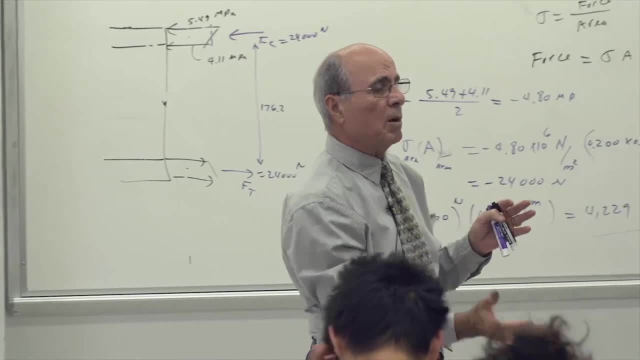 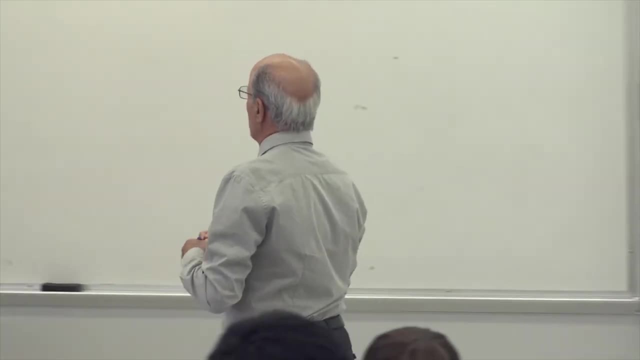 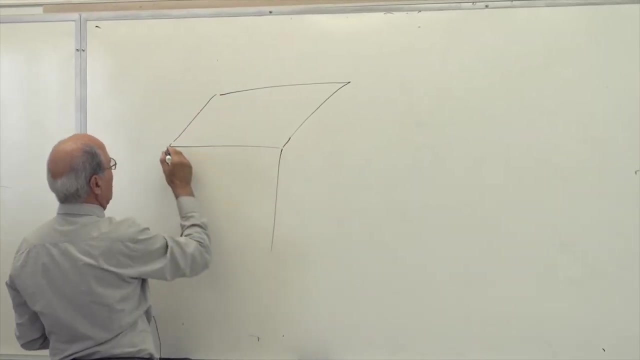 direction of your force and the direction of the moment. Sometimes moment is this way, sometimes moment is that way. That just changes your plus and minuses, nothing else. Is that correct or not? However, to just understand what we are doing here, let's say that we have here a column, and this column also this: 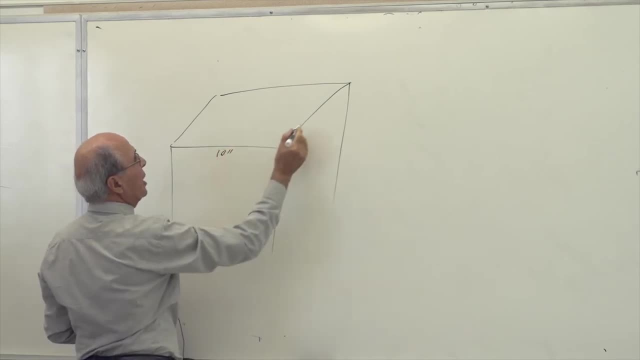 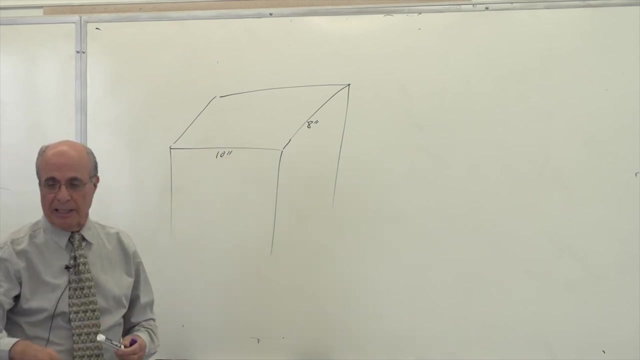 problem is in your book. it has a 10 inch by 8 inch cross section. I want you to understand the system. rather than having it like that, Let's assume this side and that side are different from each other. The ratio of 10 to 8 is 10 to 8. So 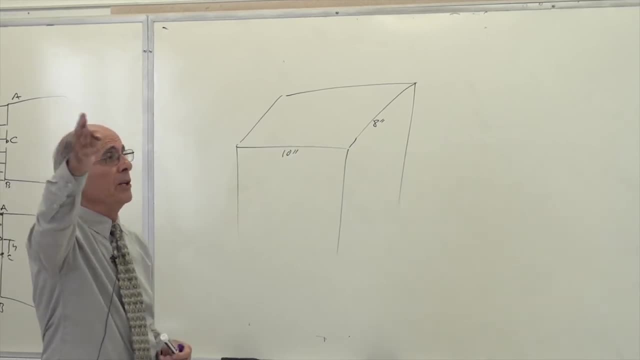 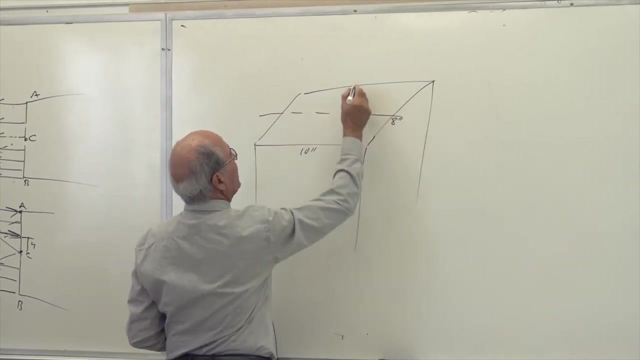 it's 10 to 8 inch. Is that correct or not? Yeah, Like any column. You see that behind you this column. Yeah, almost like that. Is that correct or not? Now, if the load, so there is a center here, The center is the everything center. So if I 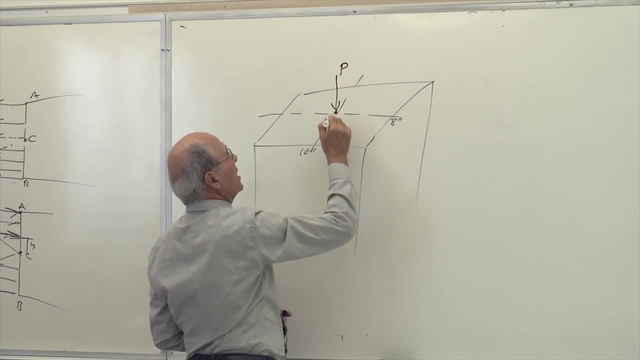 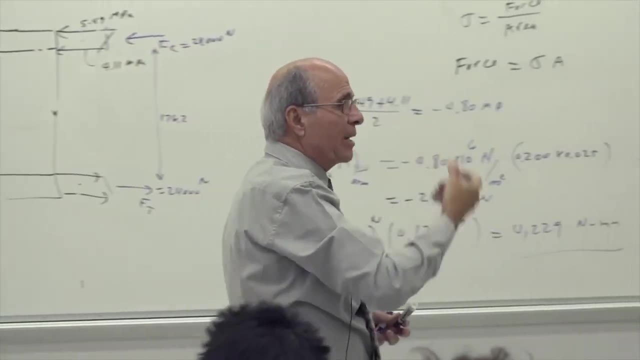 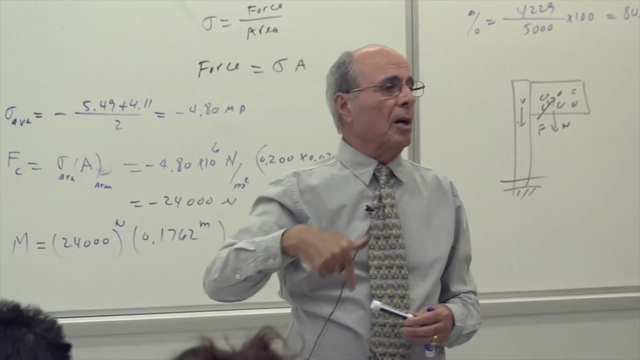 put a load here, P, at the center of this column. this is chapter one. This become axially load. Actually, the name axially loaded member, you should pay attention to that, It means where the load is on there, Centroid of the cross section. Is that correct? Otherwise it will not. it will. 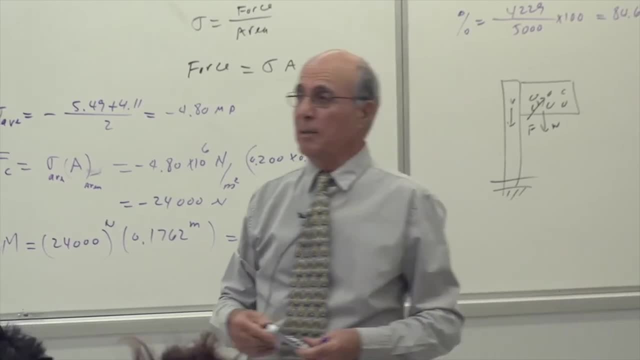 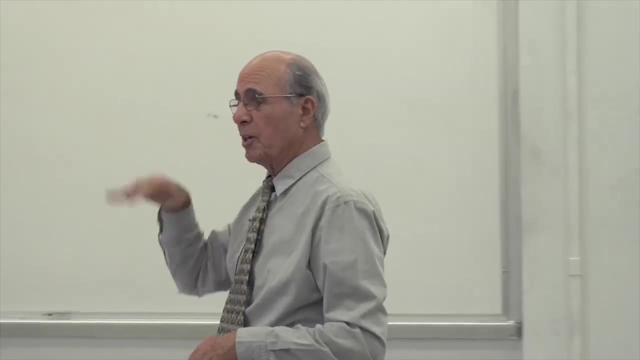 be eccentric, Otherwise it create moment as similar as that. And, by the way, we never have axially loaded member. It's impossible to put the load right at the center. If you go by real design in the code always say: take this much. 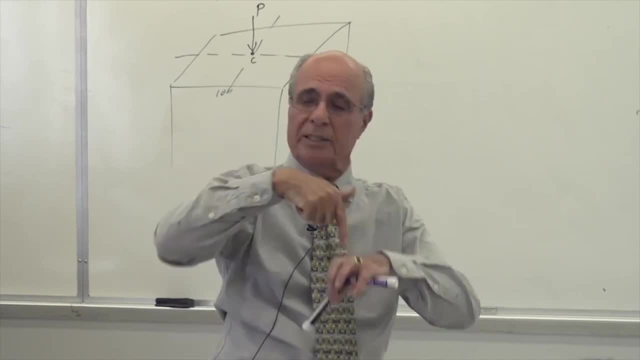 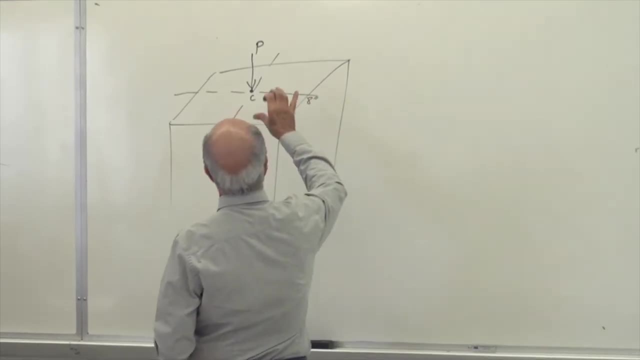 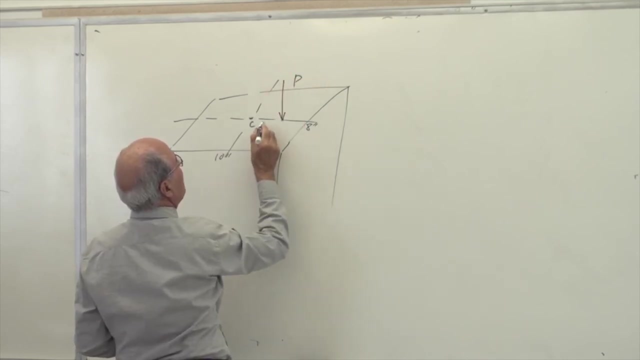 eccentricity, Because who can guarantee that your load goes right at the center, exactly the point? Obviously there is some variation there. Now, if I put the load here, P and this distance is given, let's say one and a half inches, What? 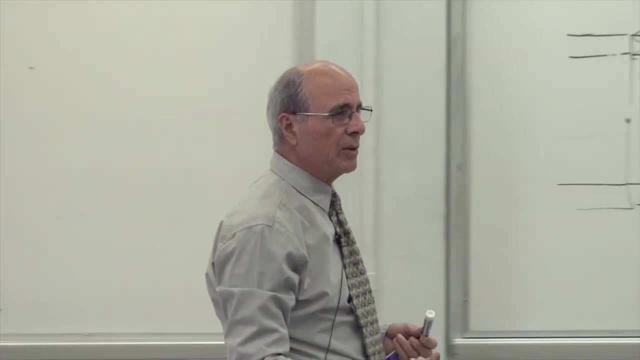 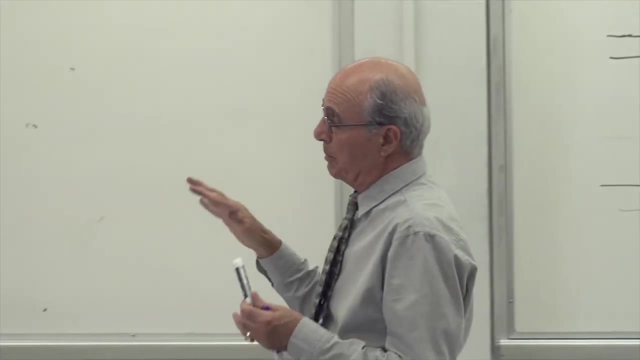 have I done here? Is this centric load or is it eccentric load, Eccentric, Eccentric. Now, how much moment do I have? You see, this is the static part that some people, many people, do it correctly, but I have to review it with you one. 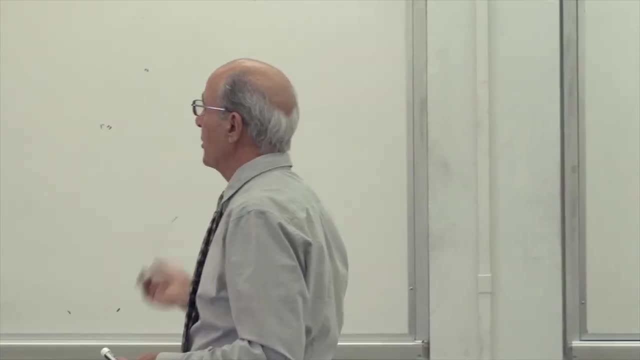 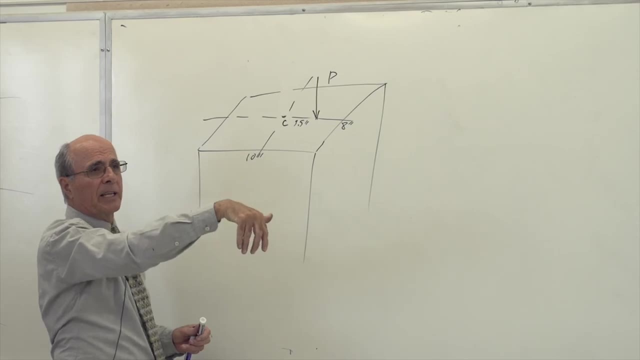 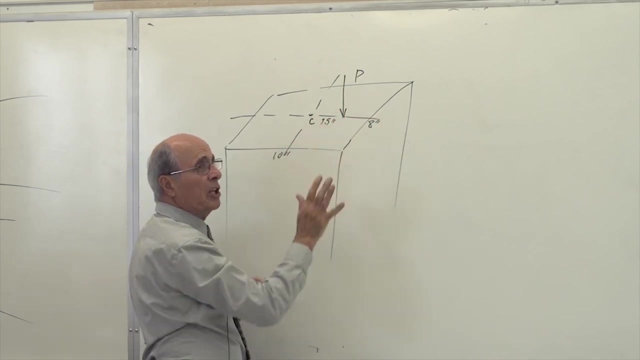 more time hoping that everybody will be doing it. Which direction is the moment? Should I put the moment like that or should I put the moment like that? I should put the moment like that. In other words, this is equivalent system. Before you go here underneath showing anything, this is equivalent. This is not. 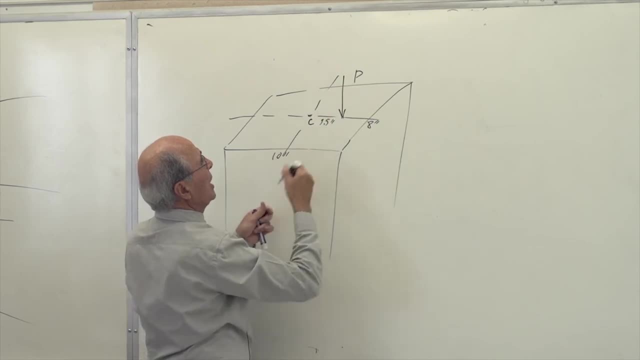 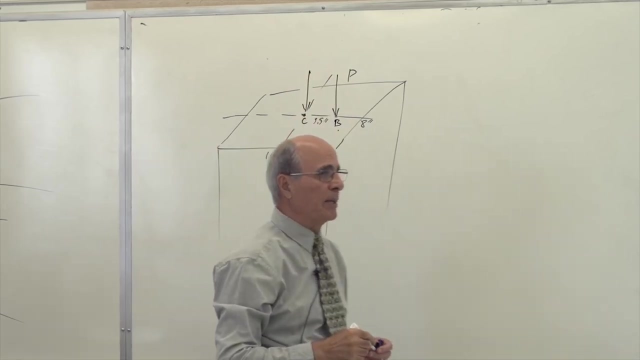 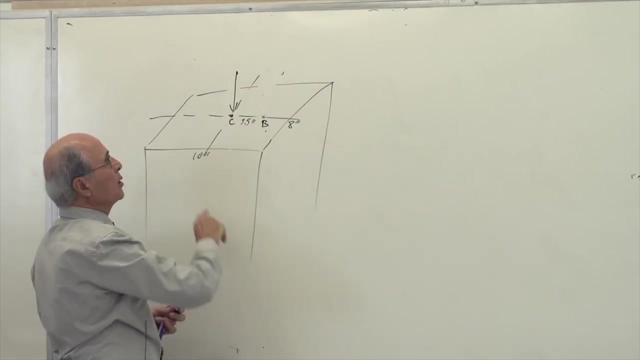 equilibrium, I have to move this P, which is applied at point B, bring it to point C. So if I do that, this is an equivalent. Remember that I do not have to reverse it. Notice, I take the P exactly, put it there. Is that correct or not? But 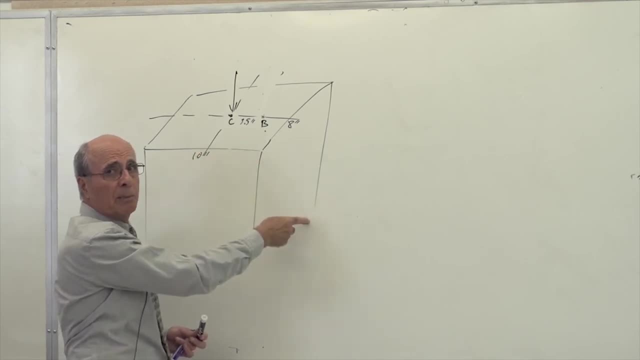 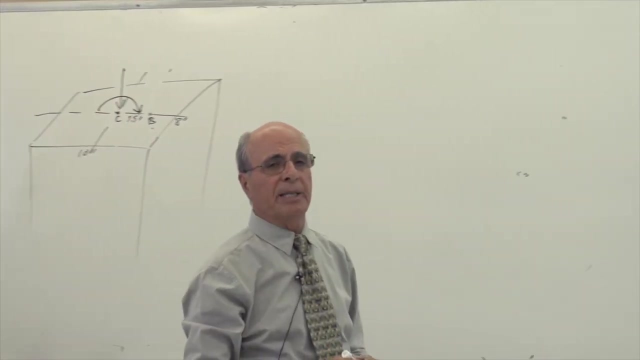 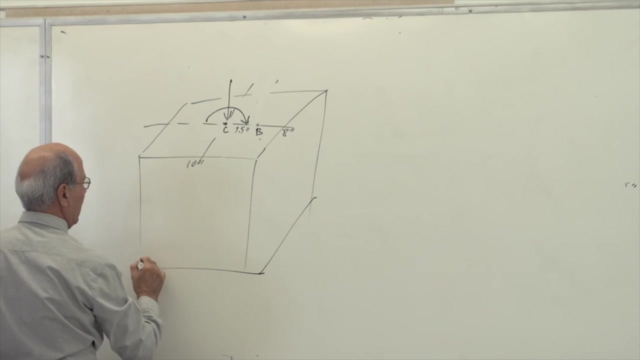 which side was the push, Which side was the pull? This side was the push, This side was the pulling up. So the moment goes like that: Is that correct or not? Yes, Correct, All right. So in this, if I'm here, I have here a cross section, I put B 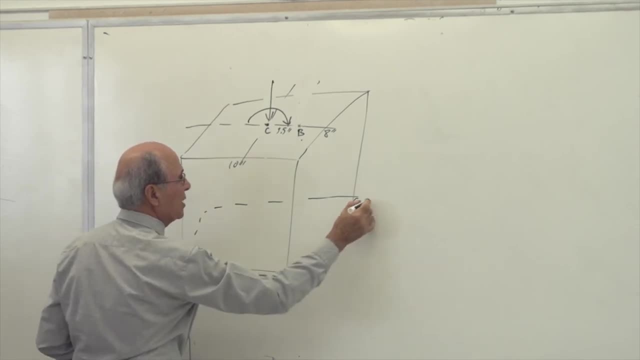 here. so I cannot use B here, So I can use A, C, D, E. Which line is under compression? Because of the bend? First of all because of this point: A, B, C, A's, I'm. 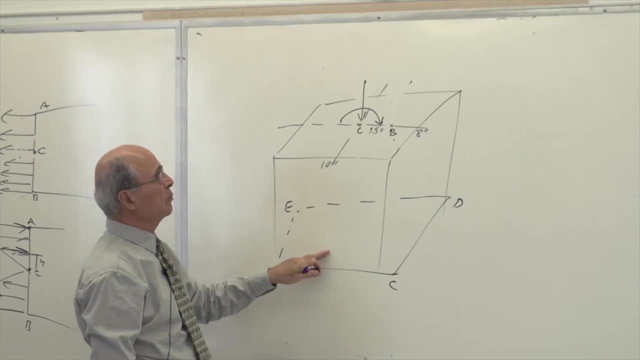 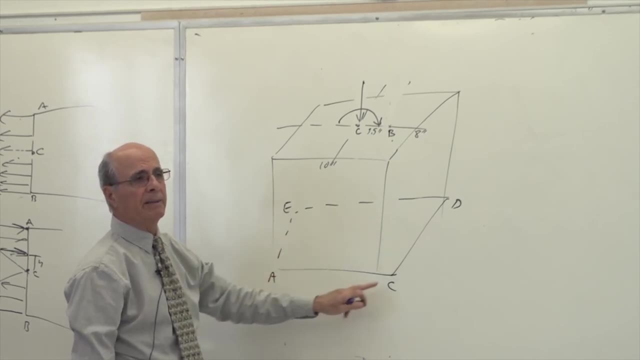 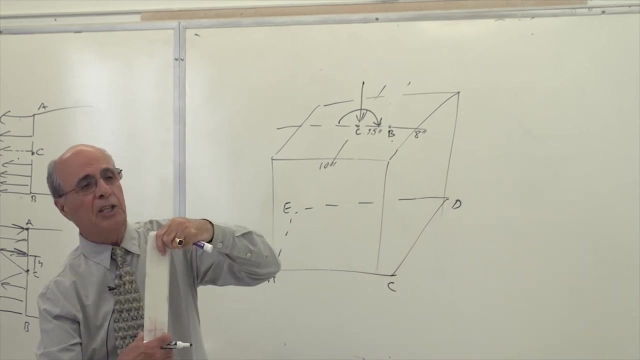 sorry, not B, A's, E, C, D. they are under uniformly pressure of P over A, Yes or no, All of them Negative, Correct In every part, Here, here, here, here. So in other words, I have here a force at the center. Everything here would be under. 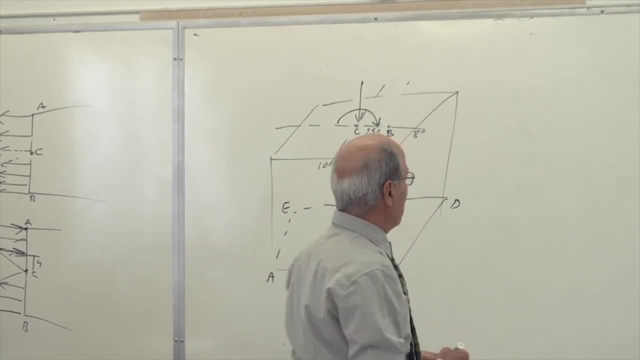 compression. That's a no brainer. Is that clear? Yes, But if I come to point C or D, what about the moment? what should I do? Is it tension or is it compression, Compression? Where is the compression? This is all is in. This is all in. 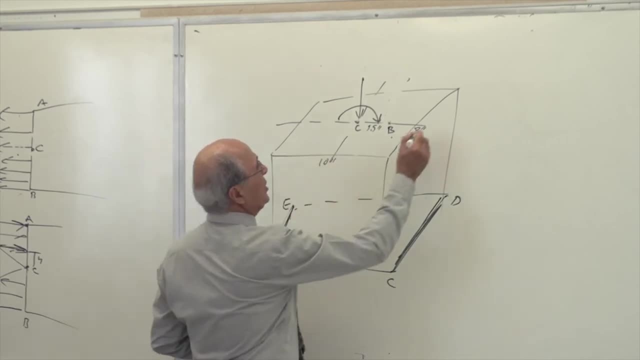 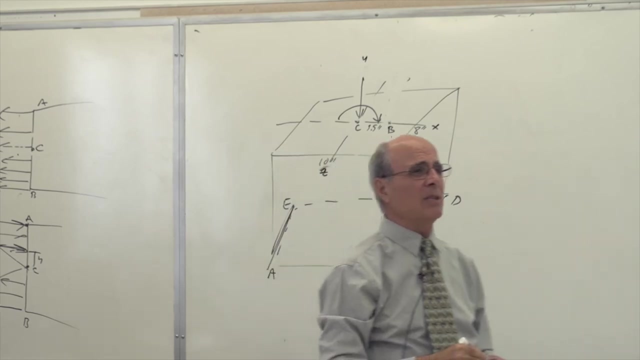 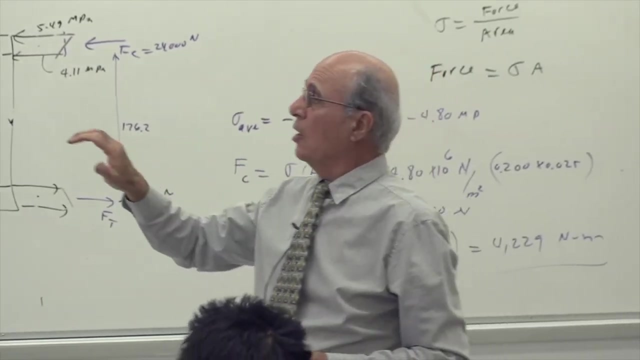 Tension. Where is the neutral axis? Is it X axis or this is, let's call it, this is X, Y, Z. Is the neutral axis is X axis or it is Z axis, Z, Z, Absolutely, Everybody with me. The neutral axis right now is: 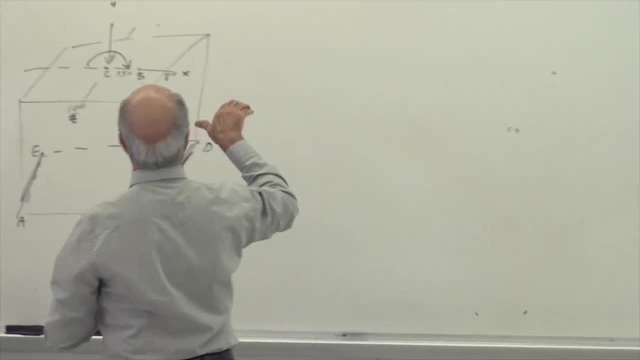 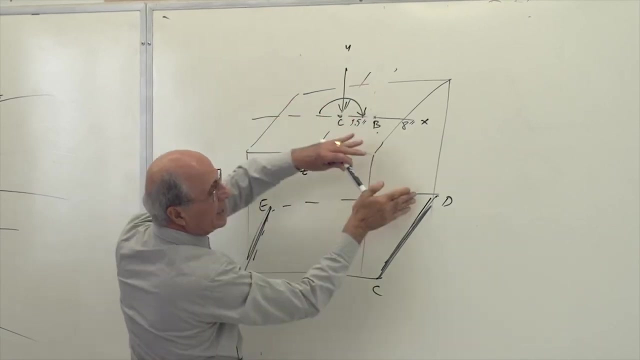 Yes, The Z, because all you have to do, guys, put your right hand rule here. Yes, The thumb indicator, so that this is not the neutral axis. This is because you are bending it this way. Is that correct or no? Yes, Everybody with me, statically. 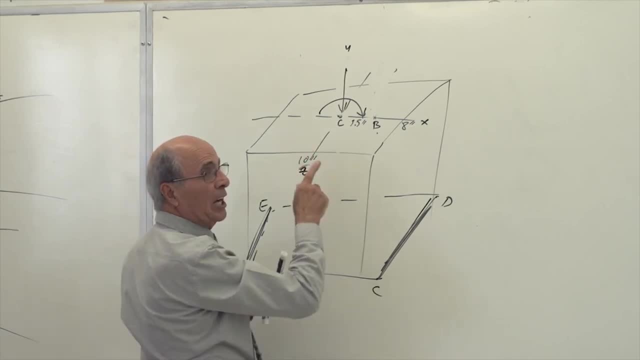 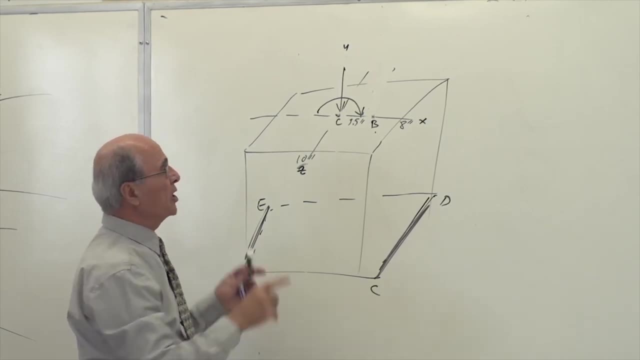 Back there. Okay, All right, right, Because this problem I have seen in ME219: people make mistake. I'm just teaching you the way. I want nobody to make mistake Because I give them this, I give them a cross section like that, And 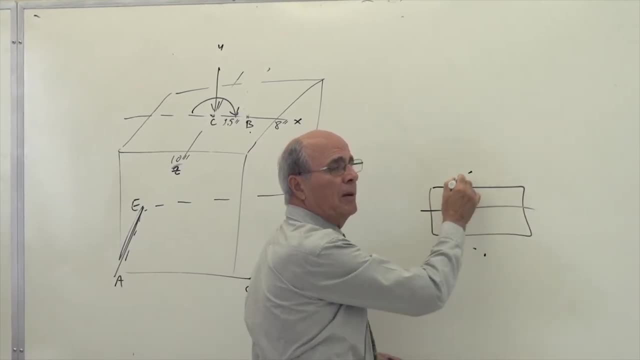 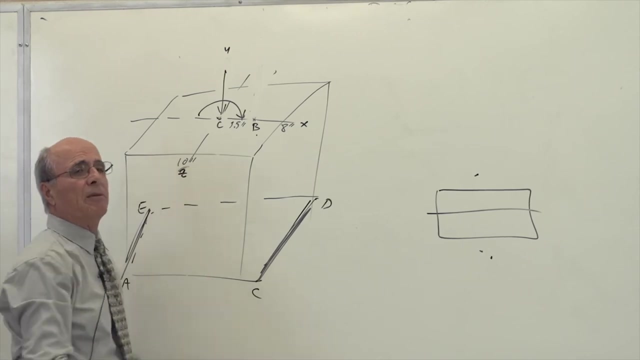 I give them a cross section like that, No matter what, they use 1, 12 of base time For this problem. base is here, height there, Because this is your neutral axis. Everybody see what I'm talking about. Yes, Okay. However, if I put the 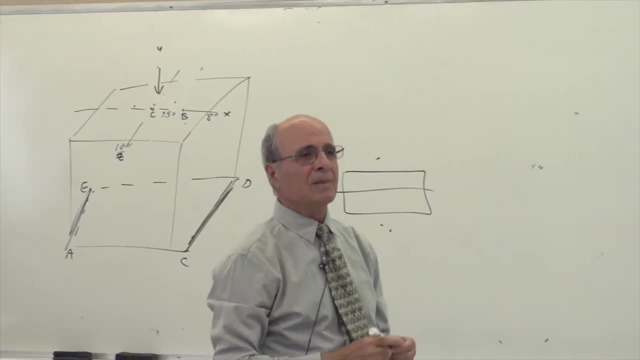 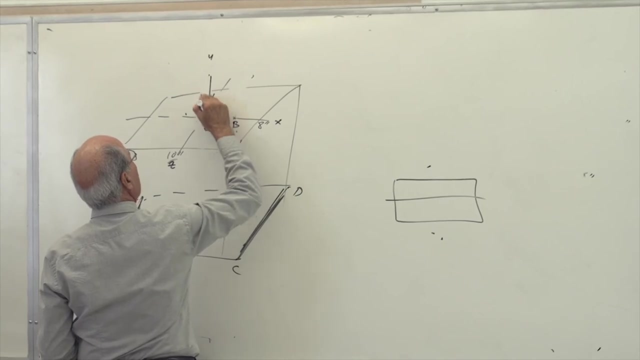 load here. now what I have done. I create a bending. that way, Everybody understand that. In that case, the bending will be like that: The load comes here Again. the same thing, But this time this is the same. This is the same. 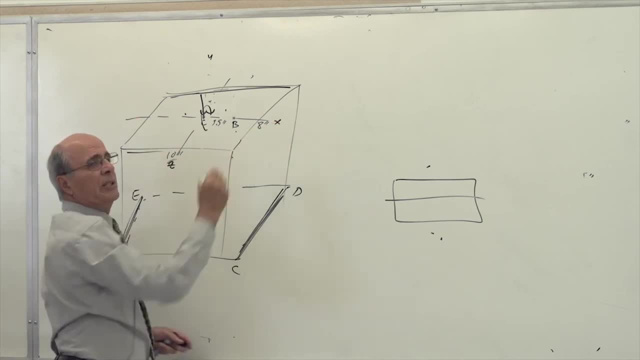 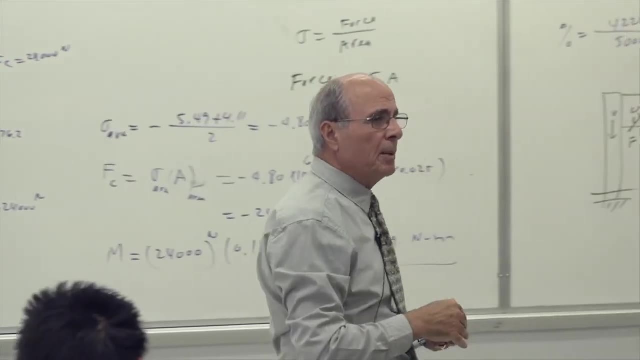 This is in compression, This is in And this is the neutral axis. Everybody understand. So we have a bending. So when you go to your homework problem, just see which way it is Bending and take the proper neutral axis, you are done Is. 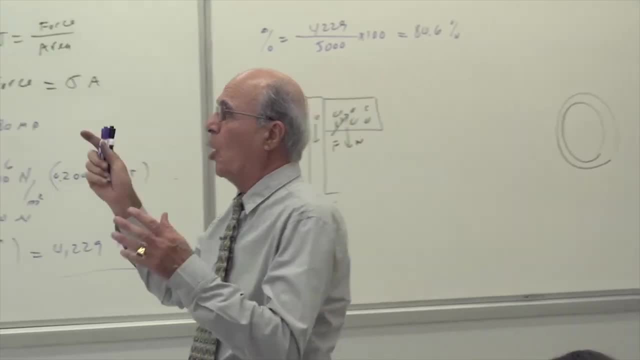 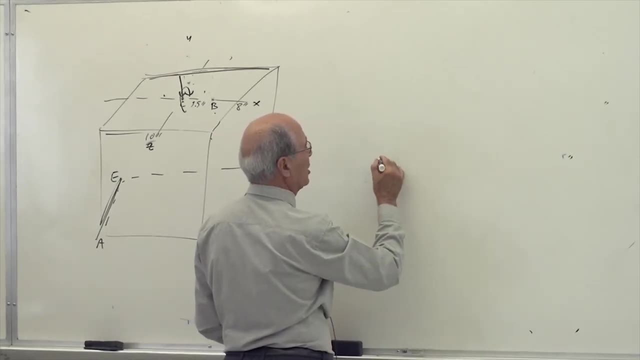 that understood. So please do not make a mistake, Don't assume always because the cross section given like that- This is what people make a mistake- It's cross section given like a rectangular cross section like this. Don't assume this is the base, This is height, This is the base, This is the base, This is the 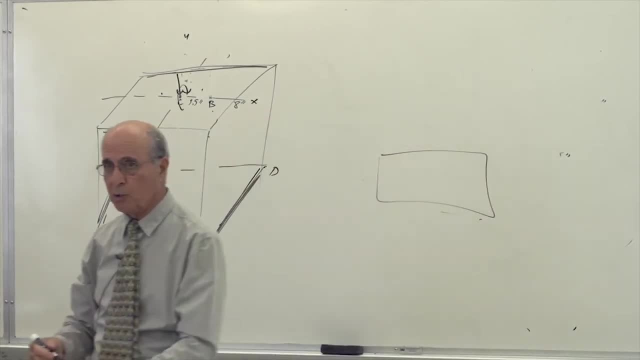 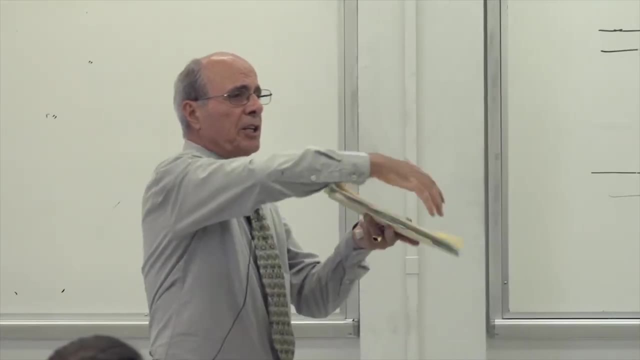 height Depend whether you have bending like that or not. In other words, this is. I can show you one more time. Just give me a couple of more minutes. I have one more problem to this just to discuss with you. Here it is. I do this way. 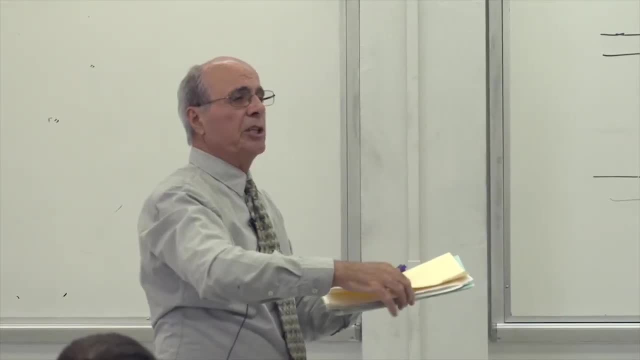 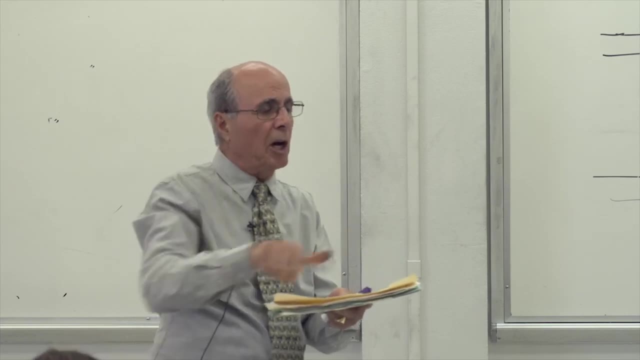 Here is compression, Here is tension. This is the neutral axis. I do it this way: Here is compression, Here is the head of this head is the compression of, And the thumb is always is the neutral. One more problem before you go, because I 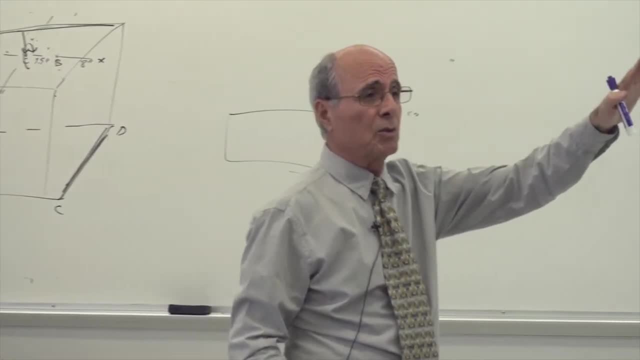 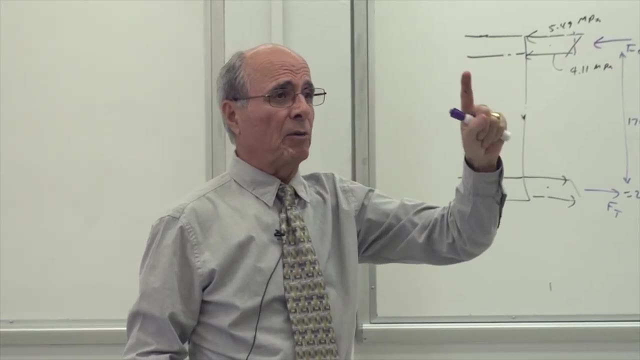 want you to do all your homework. Today is the. nobody has quiz today, So just nobody has quiz today, So office hours is very, very probably empty. As I said, you come and see me there, Plus the fact- one more thing- Many of you are going to 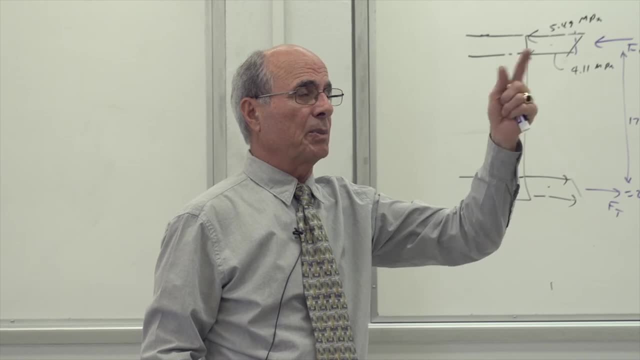 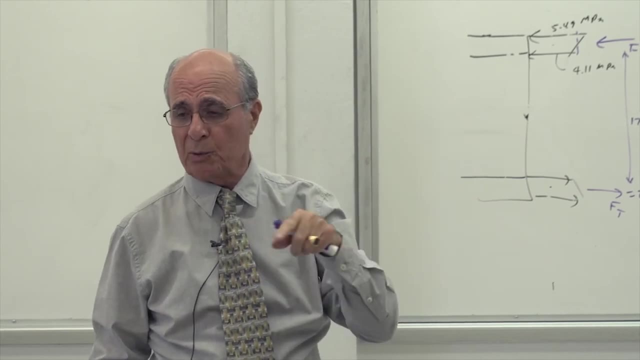 pass this course next summer, next spring, next fall? What course? Somebody asked me that. What course are you going to take? I checked it with the department. You are going to take the 219 cap. Go for mechanical engineer, Or are you going to? 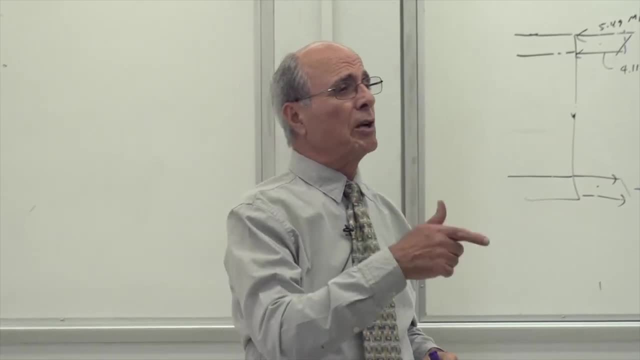 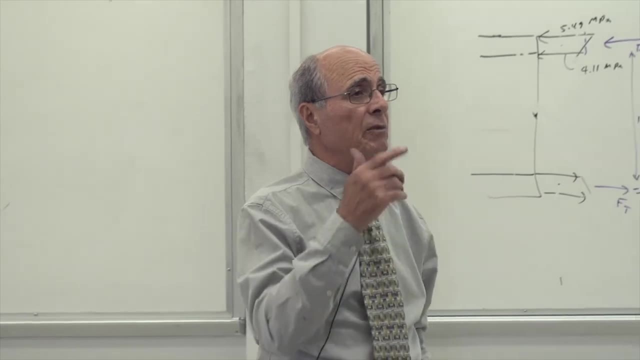 take 219 regular. I suggest you take 219 regular because in that course, my students, we are going to repeat chapter 5, 6, 7 of this string one more time And it's very important for you to review that. But I asked the department. They 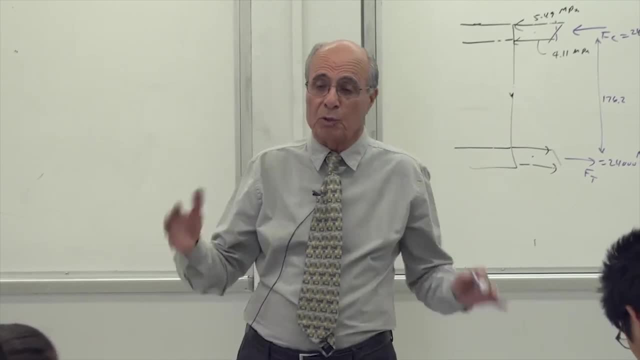 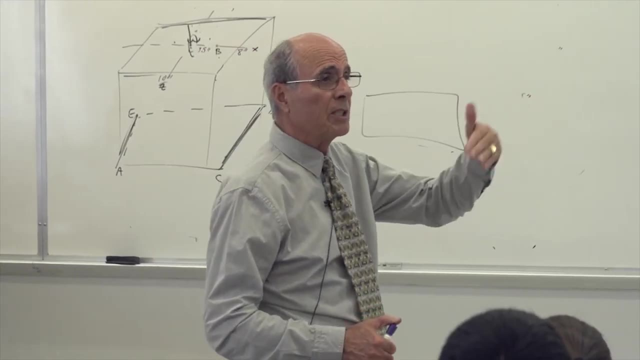 said you are allowed. you already asked it. They said you can take it. Actually, that's you should. everybody, even you are a student here. I would suggest that you don't take the cap. Take the ME 219 one more time, which is 15 weeks, Part of 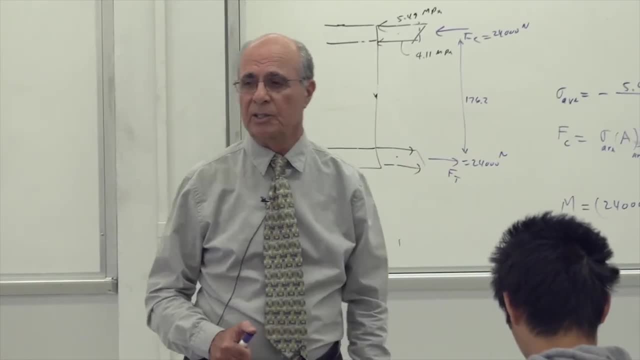 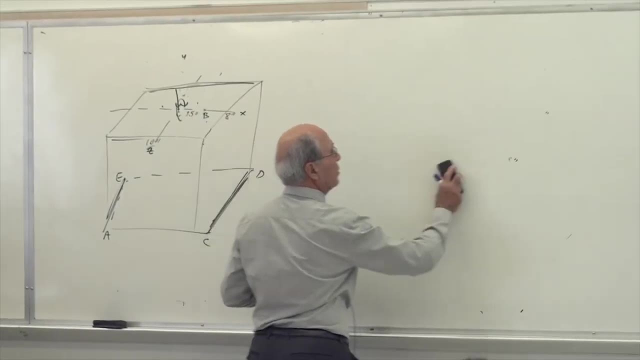 it is two: this is for mechanical engineers, This is only for mechanical. So take that course, because it gives you extra, extra work. Now one more question before I leave that I want to. there is another problem Quickly I want to mention. 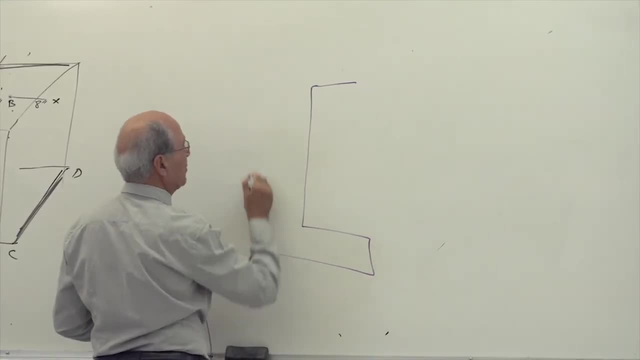 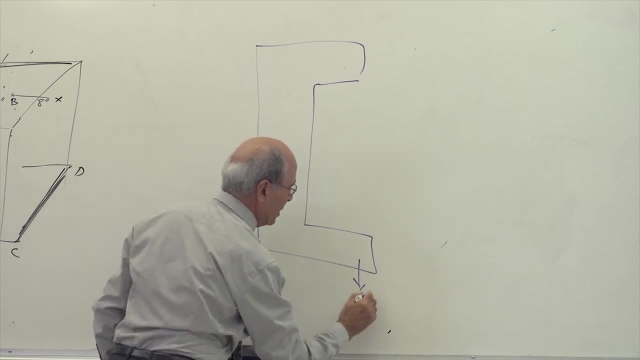 that There is another clamp-like system like that, which is exactly like the way I did Remember this clamp. They changed the direction of it. Is that understood? So they put here. they put the P here. They put a P here, which is exactly what I 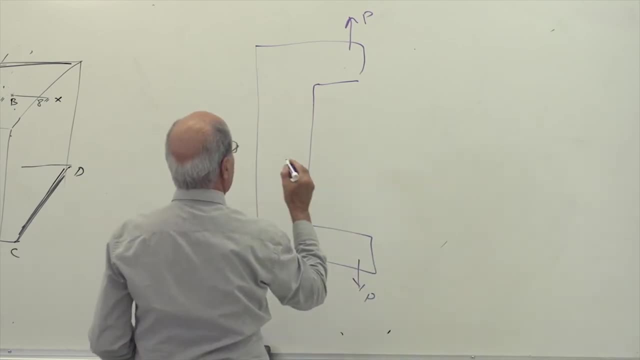 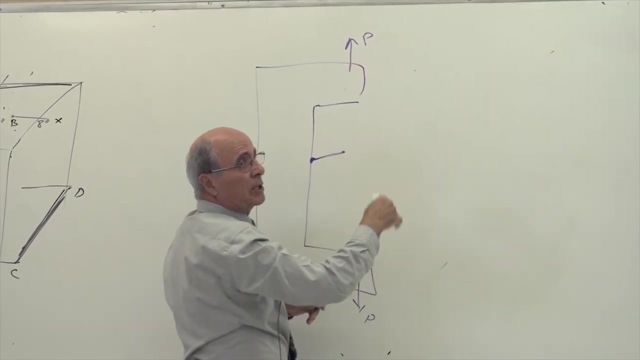 did at the beginning. Remember that. And then they said this. They said here: that's the only difference between these two: The P is not given. this time The P is not given, but sigma max is given. So sigma max is given. So sigma max is given. 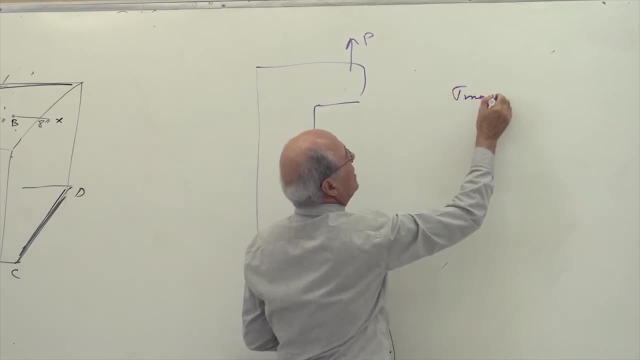 But P is question. You have to answer that. But instead of that they put here. you see, they said strain. Strain is epsilon. There is a gauge there. The epsilon is measured, let's say, equal to 1,000 micro, either plus or minus. That's beside.